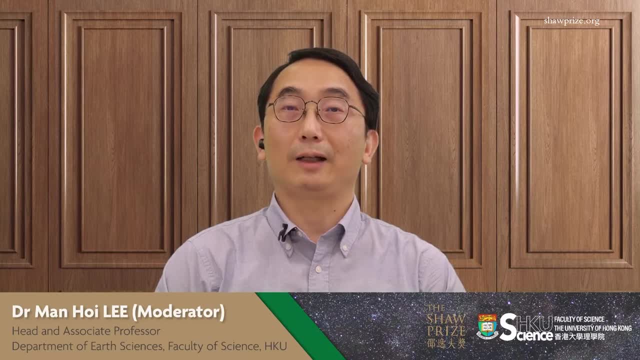 one of the two independent teams that carry out the data analysis for Hipparcos. He was a member of the Hipparcos science team for two decades and the Gaia science team for two decades after that. Professor Michael Perryman was project scientist for Hipparcos from 1981 to 1997,. 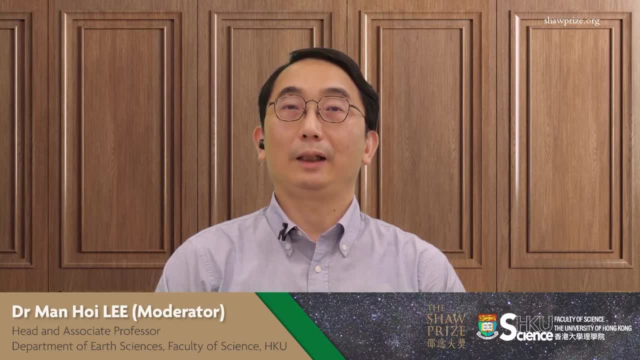 chair of the Hipparcos science team for the same period and lead author on the 1997 paper describing the Hipparcos catalog. He was also project scientist for the Gaia mission from 1995 to 2008.. Chair of the Gaia science advisory group from 1995 to 2000 and chair of the Gaia science team. 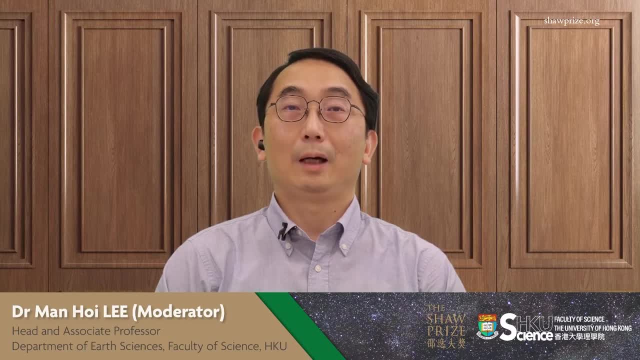 from 2001 to 2008.. Professor Lindegren and Professor Perryman collaboratively proposed the concept for Gaia in the 1990s and were instrumental in the scientific and technical design, Before inviting our SHORE laureates to share their insights on space astrometry. 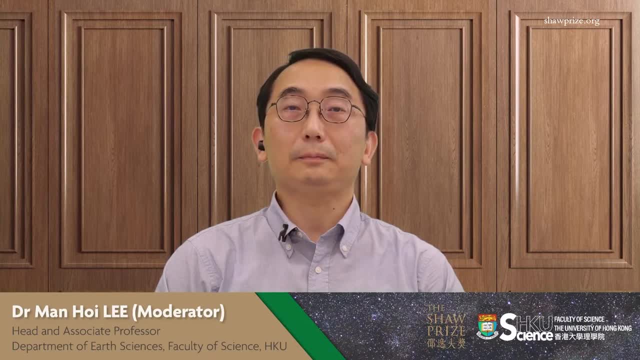 briefly introduce their academic background. Born in 1954 in Luton, UK, Professor Perryman is currently adjunct professor of the school of physics at University College Dublin in Ireland. He received his bachelor's degree in mathematics and theoretical physics in 1976. 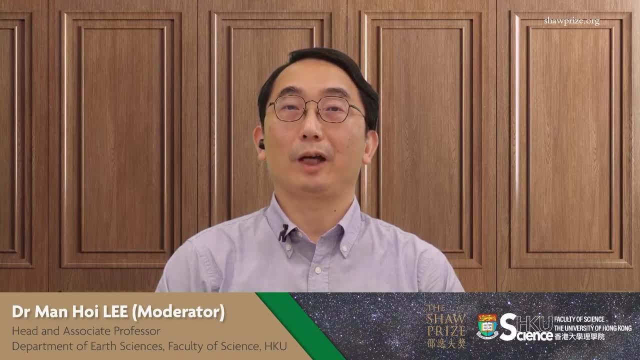 and obtained a PhD in 1980 from the University of Cambridge, UK. He joined the European Space Agency in 1980 and was nominated as project scientist for the Hipparcos mission and subsequently study scientist and project scientist for the Gaia mission. During his 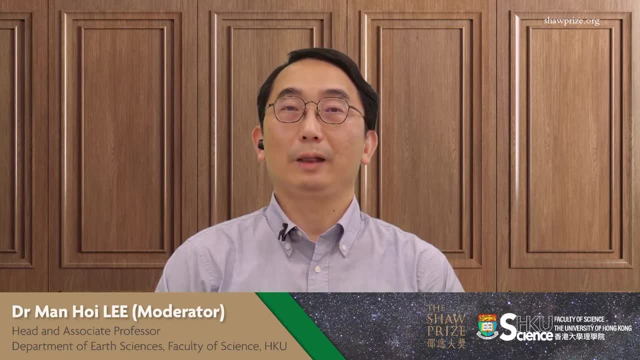 service in ESA. he has been professor of astronomy at Leiden University in the Netherlands. He held a joint position at the University of Heidelberg and the Max Planck Institute for Astronomy, Germany in 2010.. A year later, he joined. 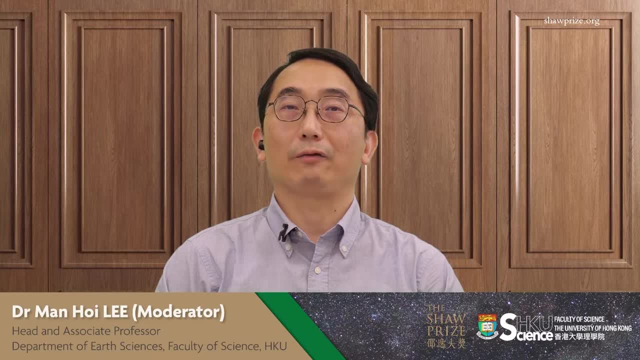 the University of Bristol in UK as visiting professor of physics. He has been adjunct professor at the University College Dublin since 2012.. In the upcoming lecture presented by Professor Perryman, he will look at the scientific aspects of this exciting journey. First, he will put their modern space. 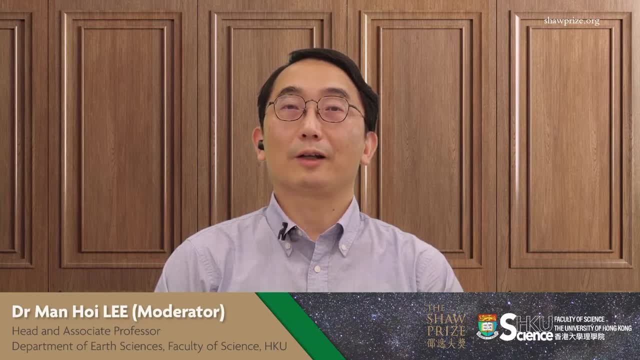 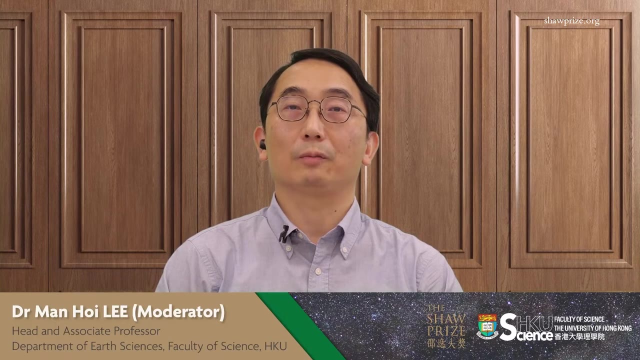 measurements in the historical context and summarize what astronomers have learned from measuring the positions of celestial bodies over the past few hundred years. After that, a few of the remarkable scientific advances which are resulting from the extremely accurate measurements of positions from space, and also a little of what this is telling us about our 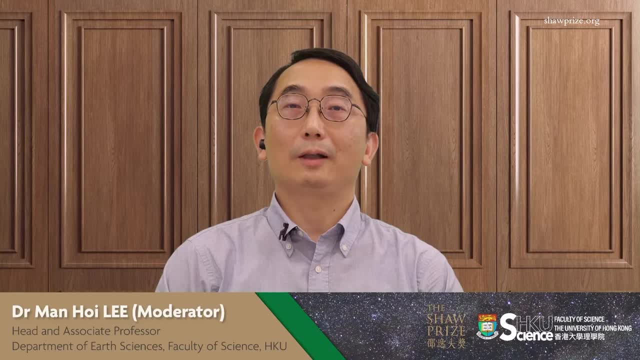 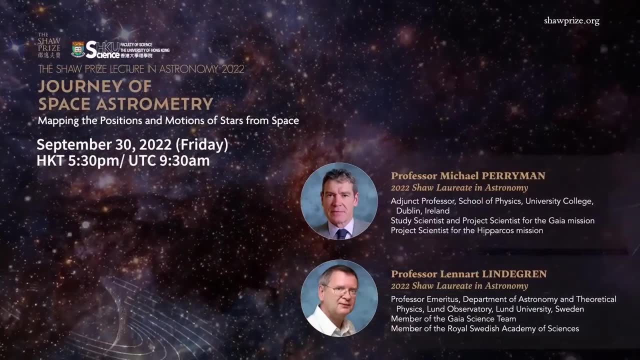 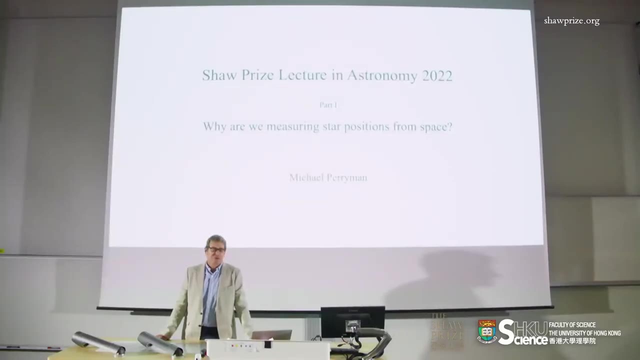 place in the universe will be covered. Now let us join professor Perryman's lecture in this exciting field. Thank you for the opportunity to speak with professor Perryman and for having to give this Shaw Prize lecture in Astronomy 2022. 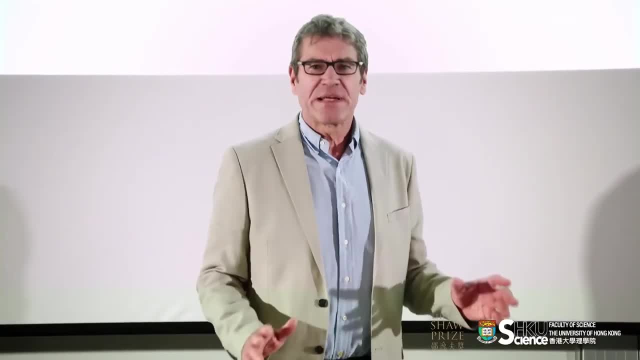 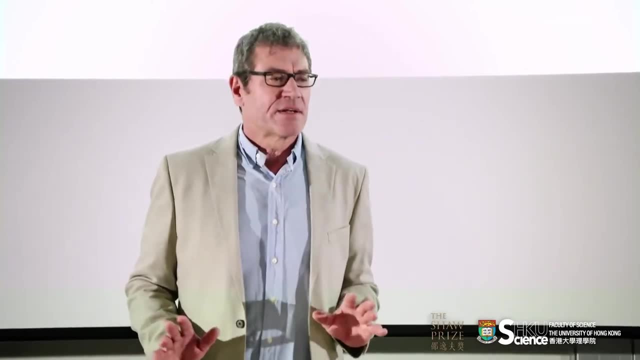 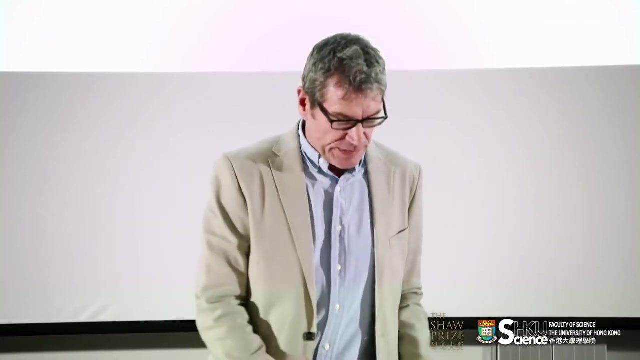 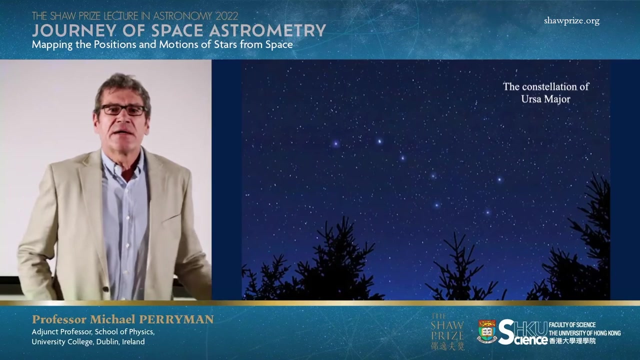 My colleague Lennart Lindegren and I are going to split this introduction to the projects that concern us into two parts, And my part- the introductory part, is to tell you why we're measuring star positions from space. First, imagine you're looking up into the night sky and the well-known constellation of Ursa Major. 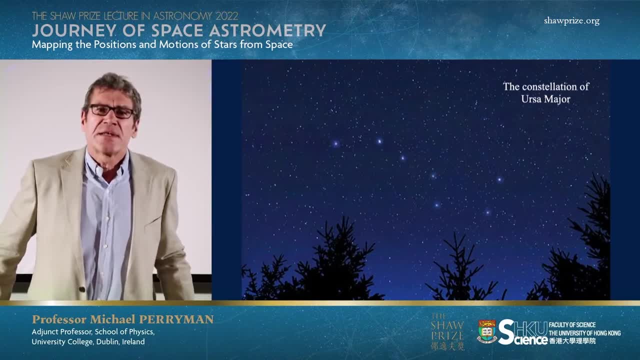 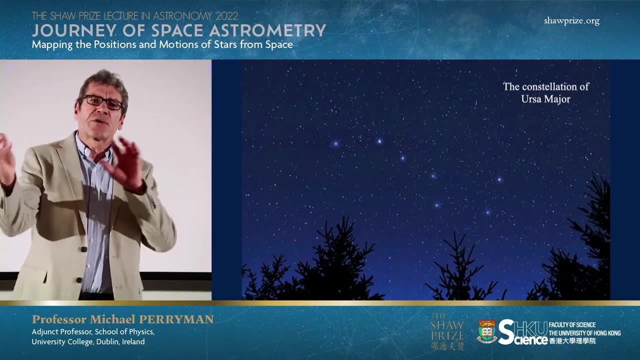 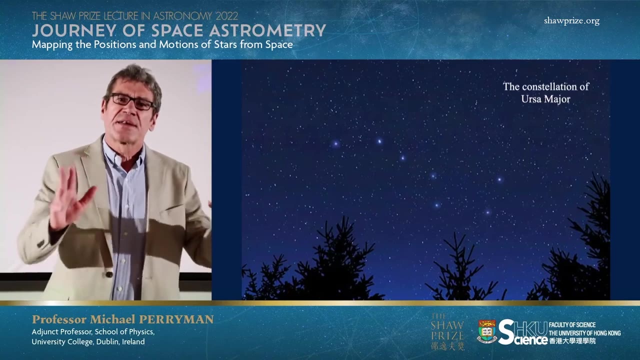 and it will look the same to you now as it did to humanity 10,000 years or even 100,000 years ago. The heavens rotate night after night as the Earth spins on its own axis, but the stars stay stationary one with respect to the other. 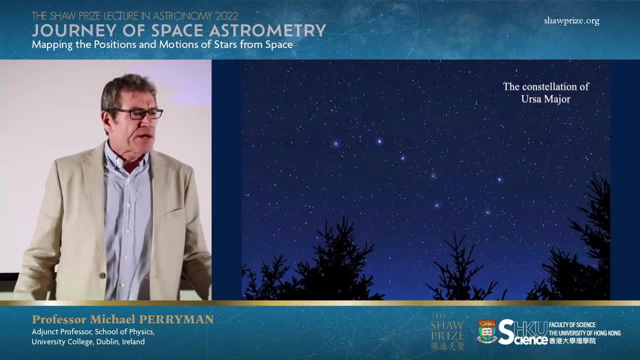 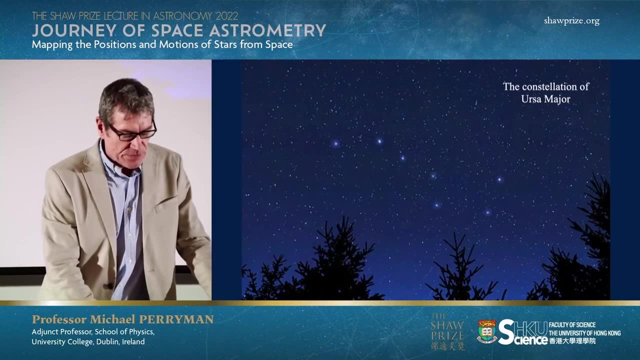 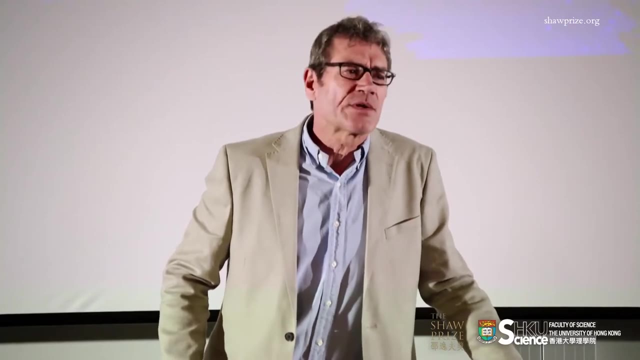 Amongst them, moving in a way which was extremely puzzling to the ancient Greeks, were the Sun, the Moon and the small number of planets that were known to them at the time. How far are these stars away from us? What do they tell us? What are these stars? 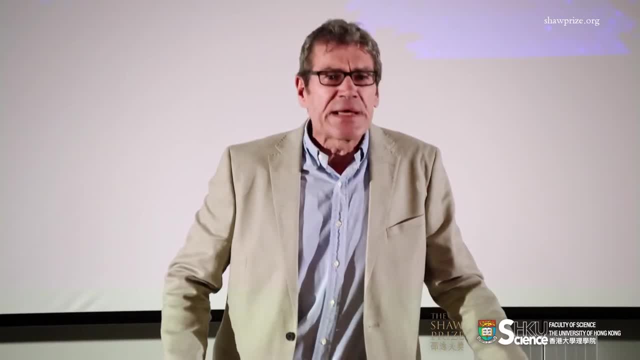 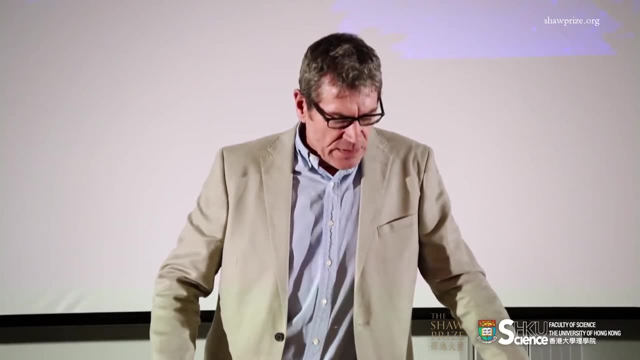 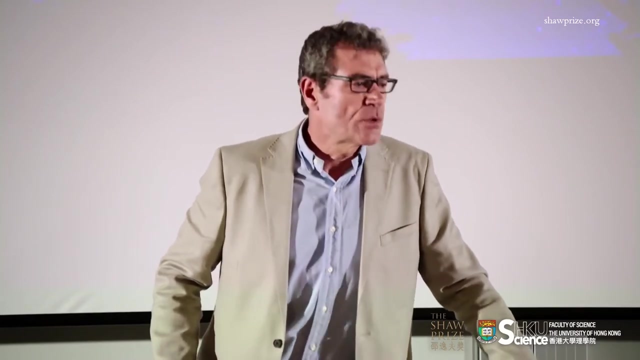 What is the nature of the universe? This has been a subject of scientific inquiry for 2,000 years, since the time of the ancient Greeks. Surprisingly, it was only less than 100 years ago that we knew what the stars were, what fueled them, what powered them? 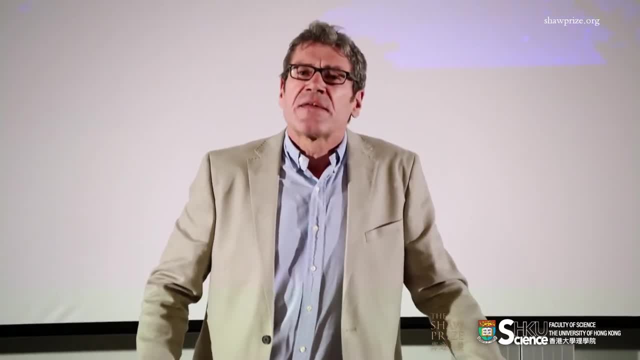 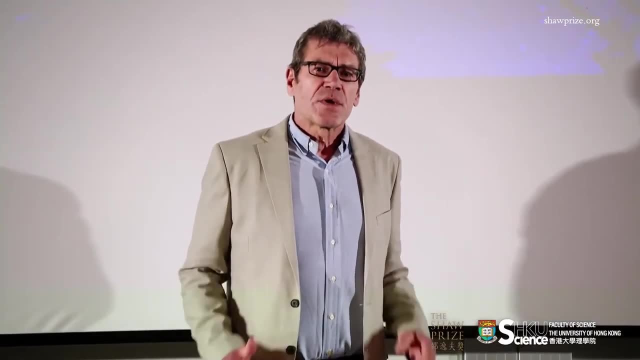 But over the course of the past 400 or 500 years there has been a great advance in understanding their distance, how they move through space, and this has told us, in turn, an enormous amount about the nature of the universe around us. 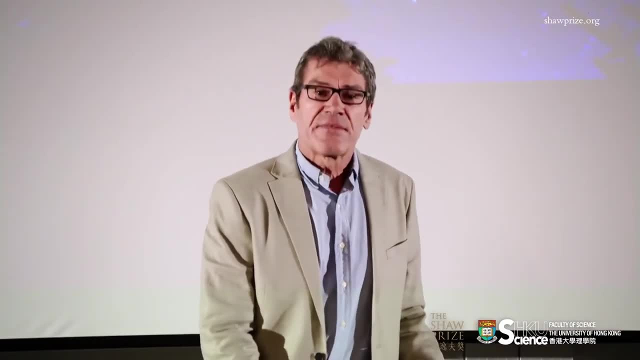 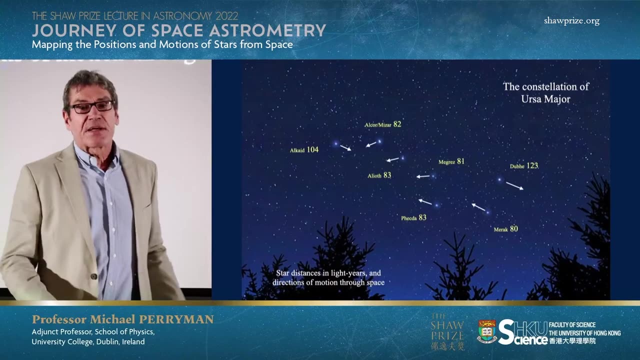 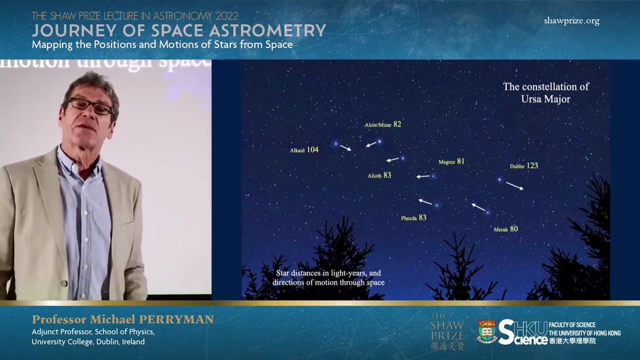 And what we know today, for example, is that The stars in the Ursa Major constellation are not all at the same distance. They are in light years- I put the numbers here- about 80 light years, but notice Al-Qa'id on the left and Dubey on the right are about 120 light years. 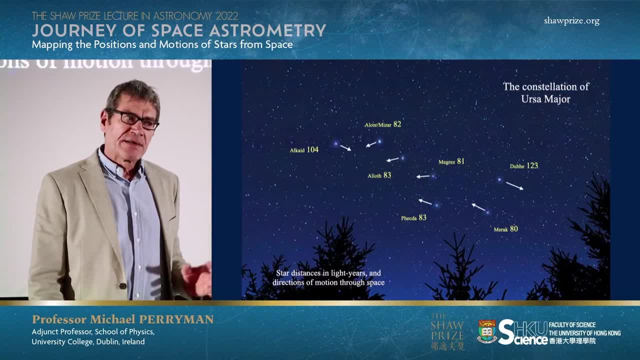 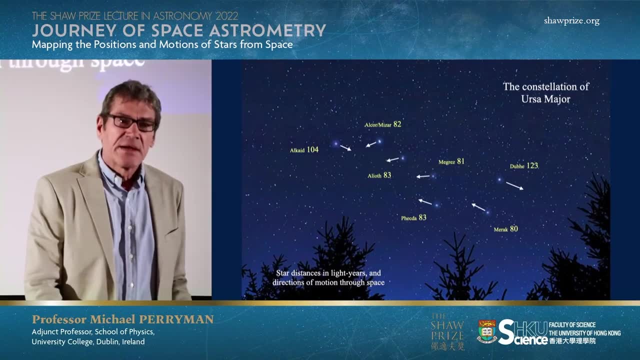 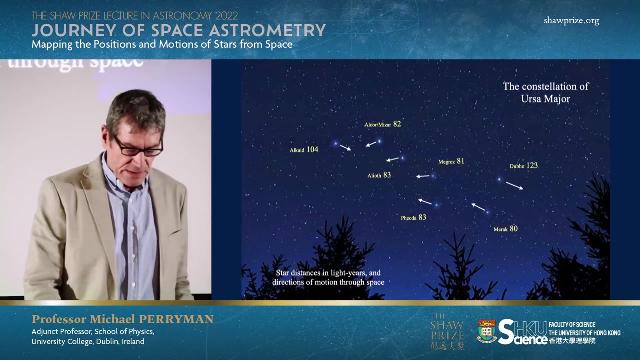 much more distant, and they're moving in different ways as well. So, although they're moving, space is so vast that even at the end of our lifetime, the constellation of Ursa Major will look exactly the same as it did at the beginning of our life. 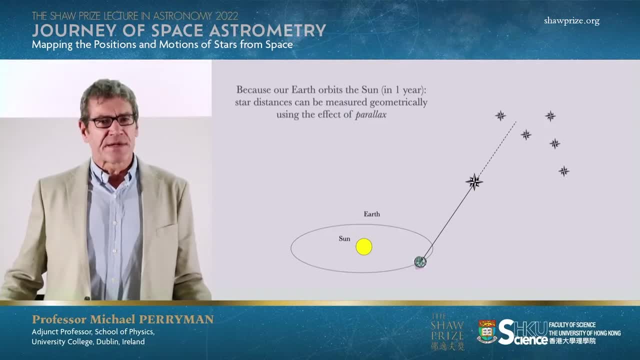 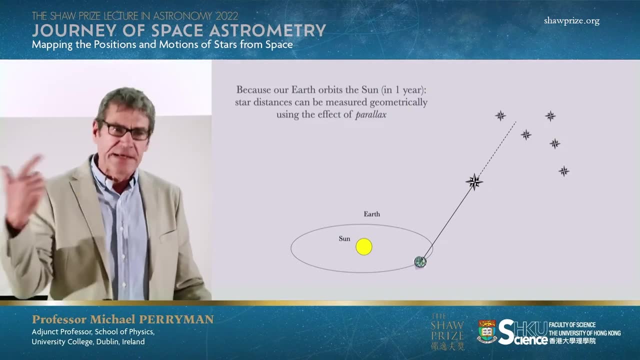 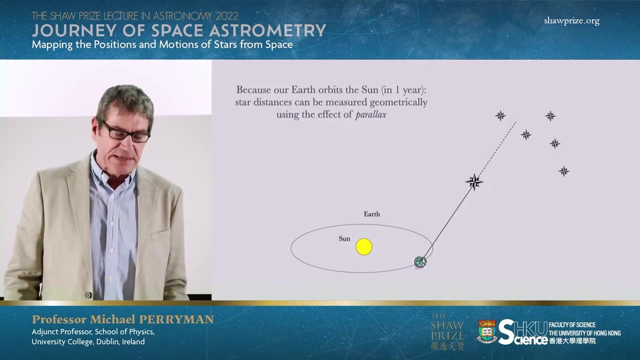 But there is a way of measuring the distance to the stars, and this utilizes the fact that the Earth moves in its annual orbit around the Sun. It takes one year, That's the definition of a year- And from its different positions as the Earth orbits the Sun. 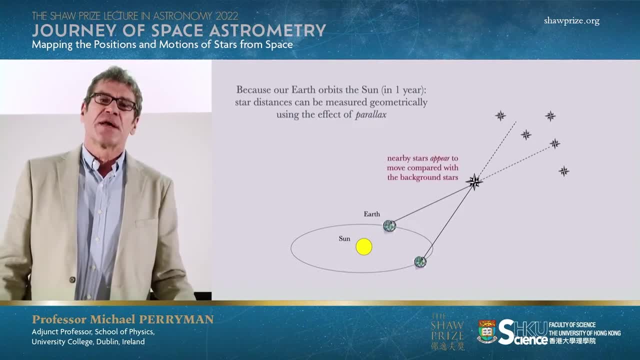 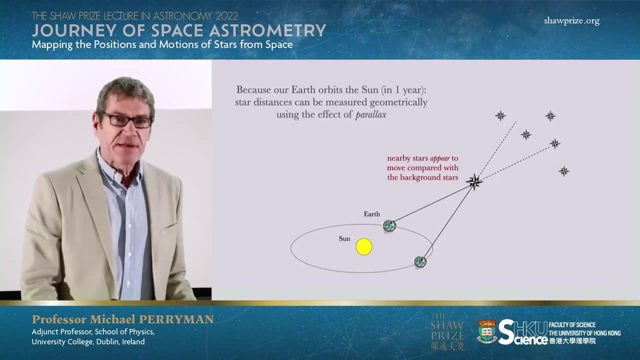 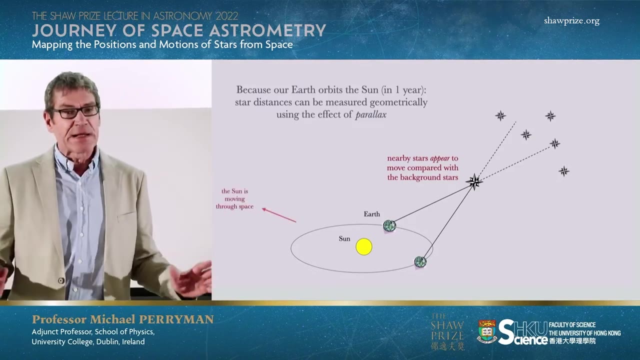 a nearby star will appear to move slightly with respect to the background stars, And this gives us the key to measuring the distance to the stars and revealing the nature of the stars. Now, of course, there's many complications. The Sun is moving through space. the stars themselves are moving through space. 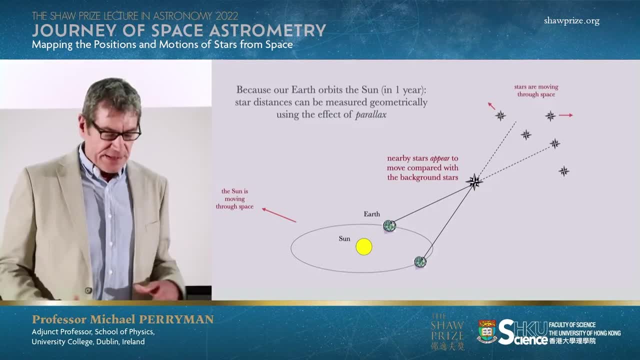 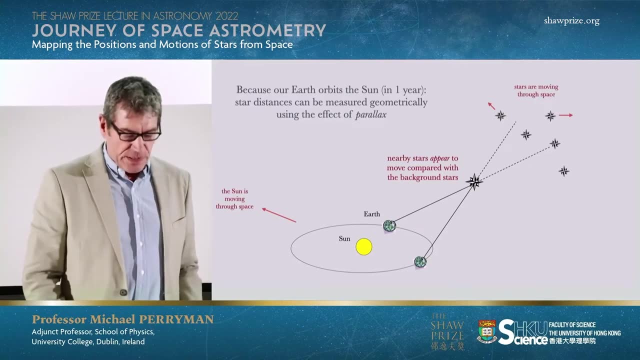 and there are many other details, but the key fact is that we can exploit the fact that the Earth moves around the Sun and if we can measure these angles accurately enough, we can hope to determine the distance to the Sun. So we can know the distance to the stars if we know the Earth-Sun distance. 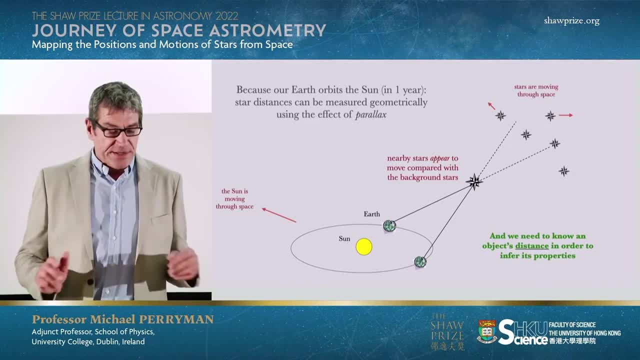 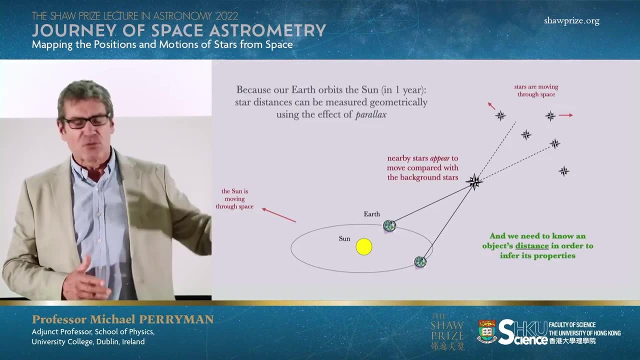 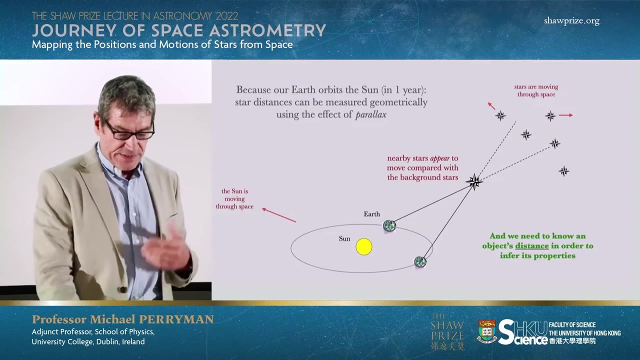 And why are we doing this? It's only by knowing the distance to the stars that we can convert their apparent properties, things like their brightness, their angular radius or whatever, to more physical quantities like their luminosities, their masses, their radiuses, and so on. 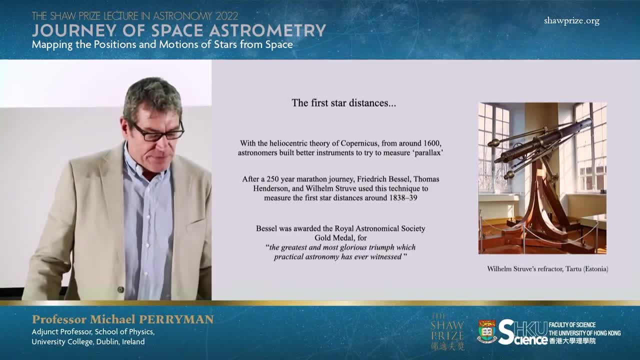 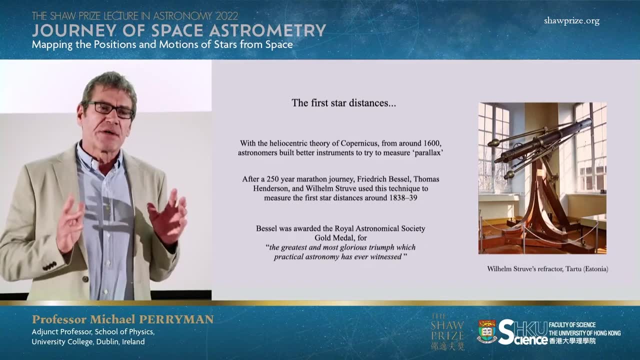 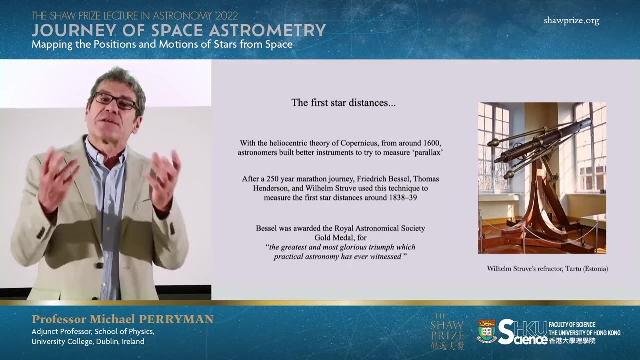 Along with the idea of the heliocentric concept of Copernicus, the fact that the Sun is at the centre of the Earth-Sun system. from around 1600, astronomers realised that if they could measure these angles accurately enough, they could determine the distance to the stars. 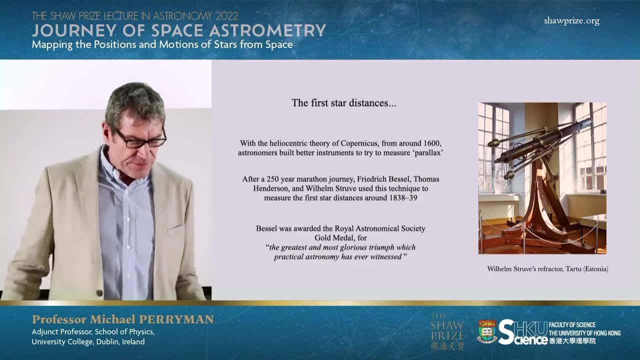 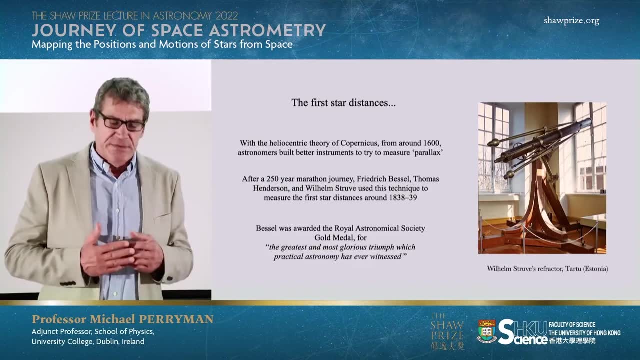 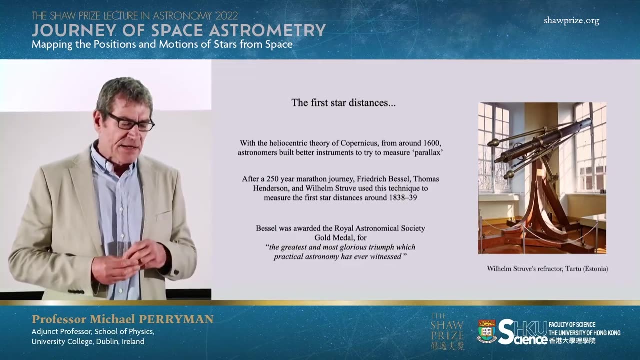 And this started a journey of about 250 years, a real marathon journey, in which astronomers built better and better scientific instruments, pushing the angular accuracy of their instruments to better and better luminosities, And after something like 250 years, around 1830, 1840,. 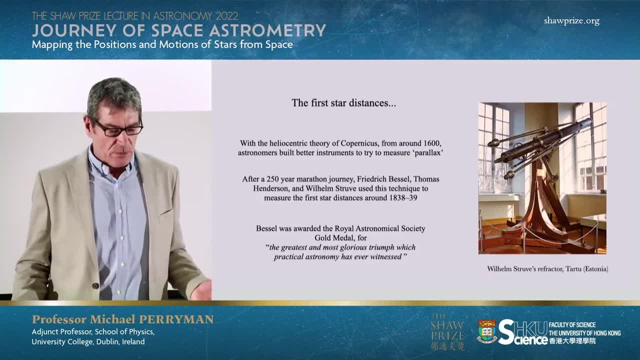 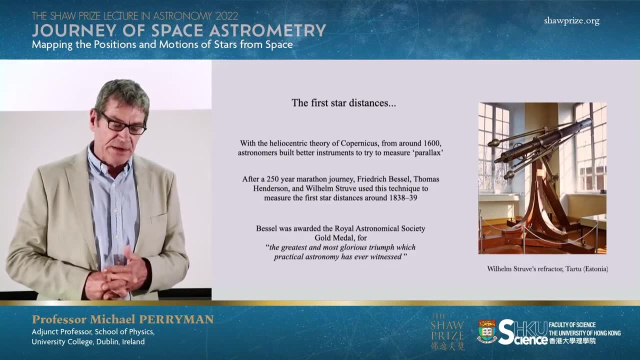 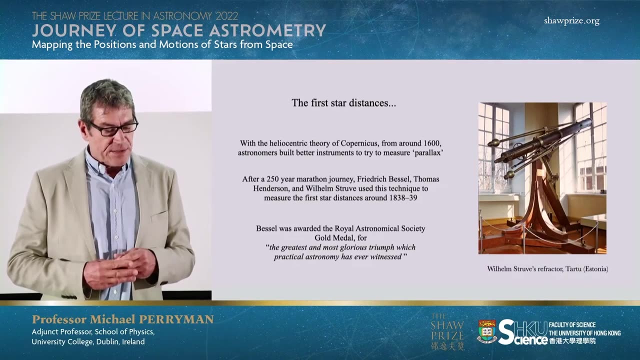 the first distances to the stars were measured using this technique, And this is the refractor used by Wilhelm Struve at his observatory in Estonia. The determination of the first star distances was recognised as a major achievement in astronomy, and Bessel was awarded the Royal Astronomy Award. 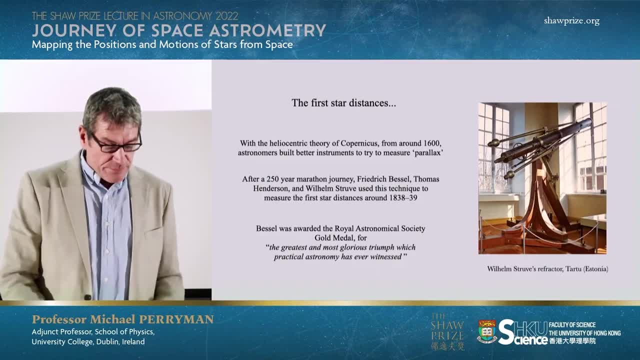 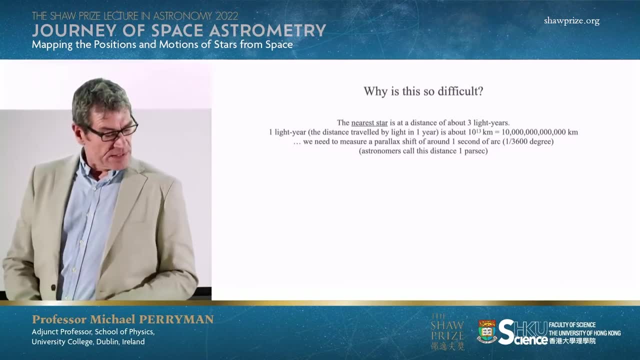 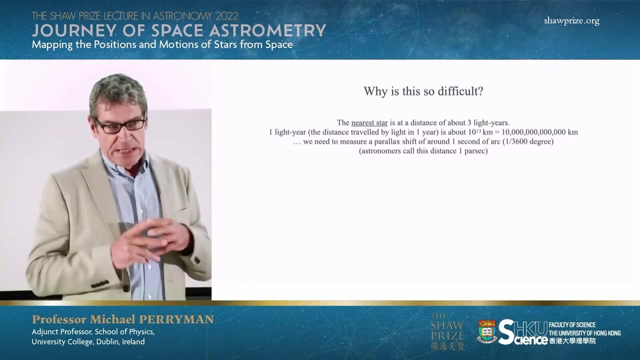 The Royal Astronomical Society's gold medal for this most glorious triumph, as the president of the Society reported at the time. Now, why is this so difficult? It's difficult because even the nearest star lies at colossal distances. Most of you will have heard of a light year. 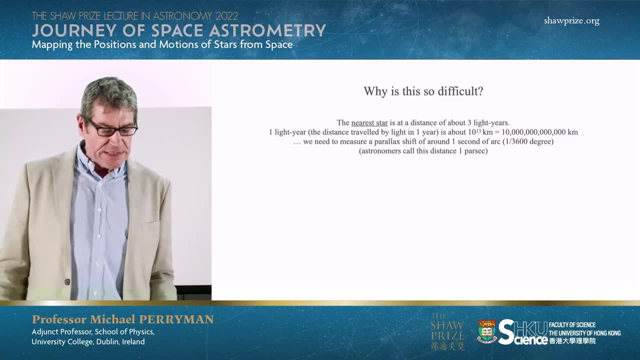 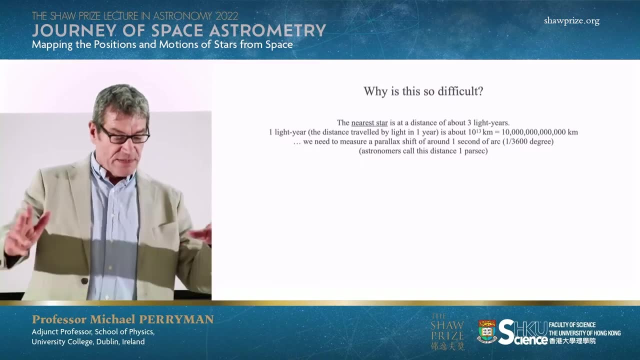 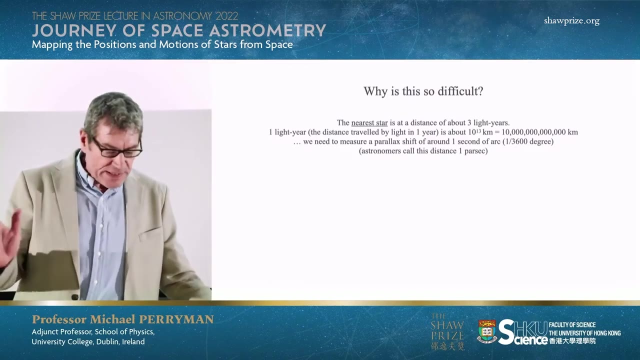 A light year is the distance that light travels in one year. It's about 10 to the power of 13 kilometres, 10 million kilometres, And we need to measure that angle, one arc second or thereabouts, in order to be able to measure the distance to the nearest stars. 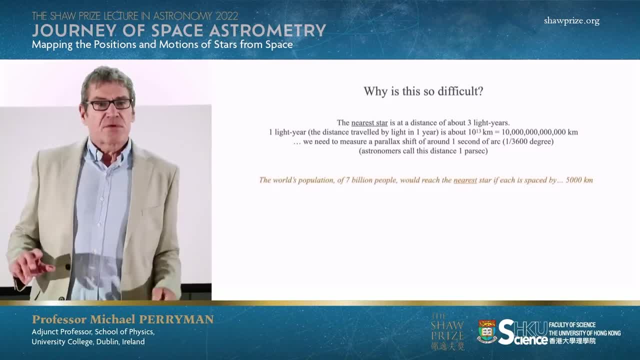 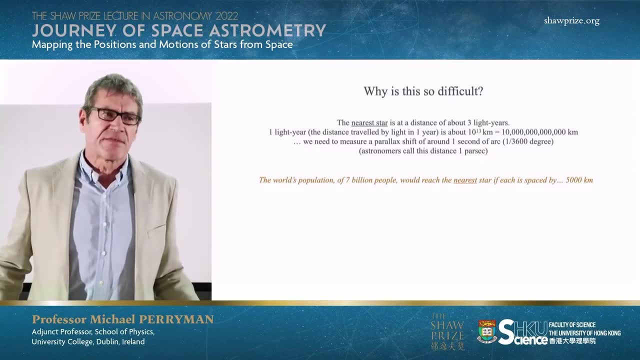 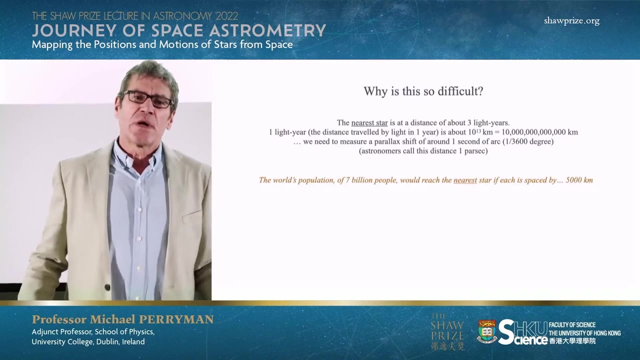 I've tried to come up with my own analogy of how can we comprehend the distance, say, to the nearest stars, And I don't think it's easy for humans to appreciate that. but here is an analogy If we took the world's population of 7 billion people. 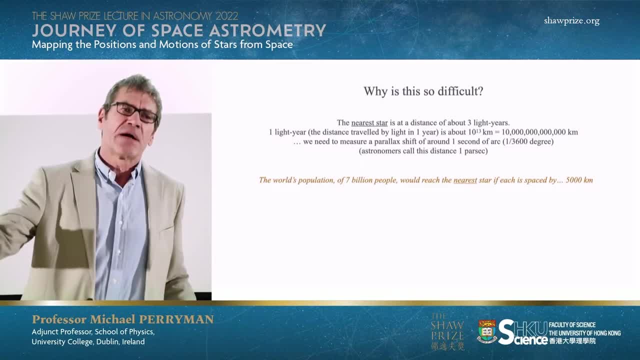 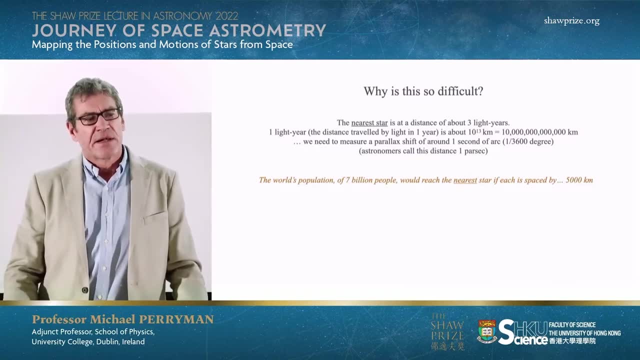 and we spaced them out at regular intervals. how far would we need to space them to get to the nearest star? And the answer is about 5,000 kilometres. So 7 billion people each spaced at 5,000 kilometres. would get us to the nearest star, And the problem becomes much more serious if we want to measure distances to the more distant stars. For example, the centre of our own galaxy is a distance of about 30,000 light years, so 300,000 billion kilometres. 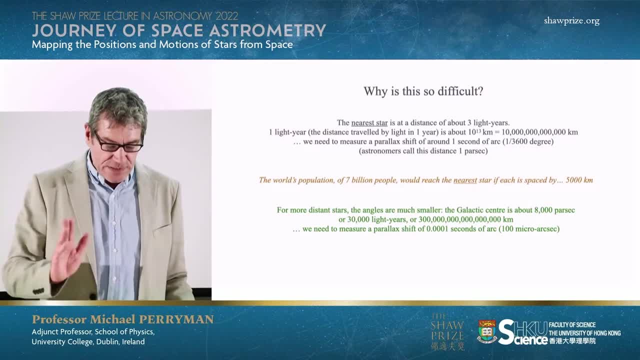 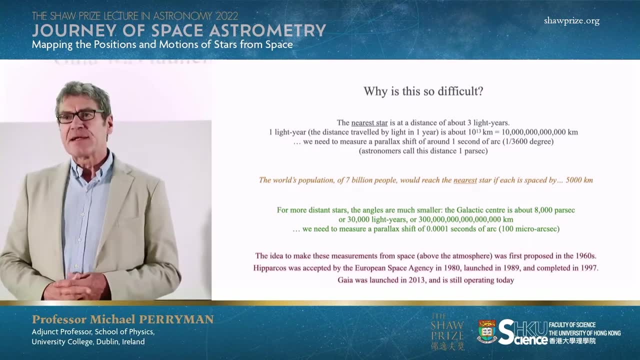 And we'd need to measure angles getting down to levels of a millionth or a few millionths of a second of arc in order to be able to do that. Now, the idea to make these measurements from space came about in the mid-1960s. 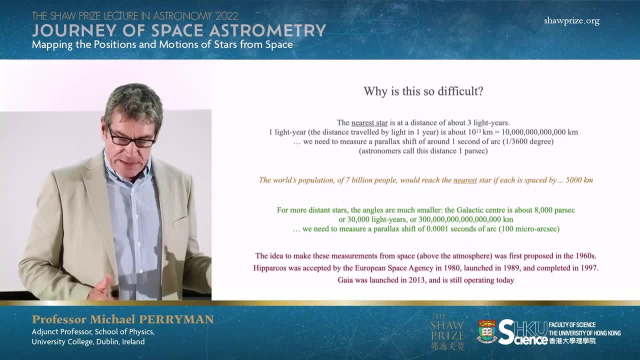 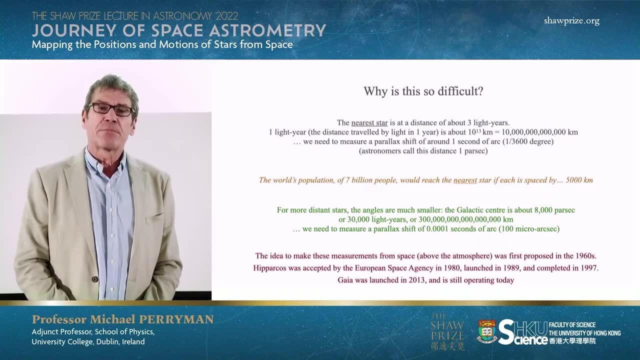 The idea was to get above the atmosphere so that we can reduce the perturbations that the atmosphere brings to these measurements, And Hipparcos was really a trailblazing experiment adopted by the European Space Agency in 1980.. It was launched in 1989. 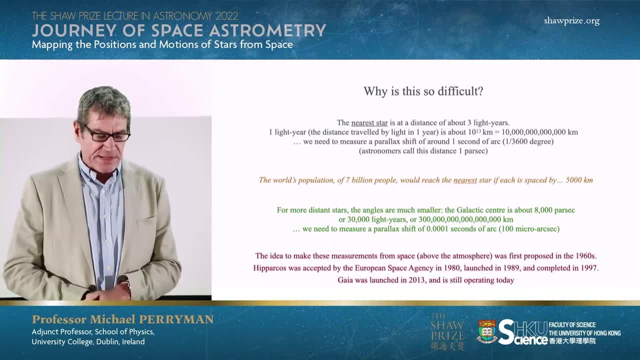 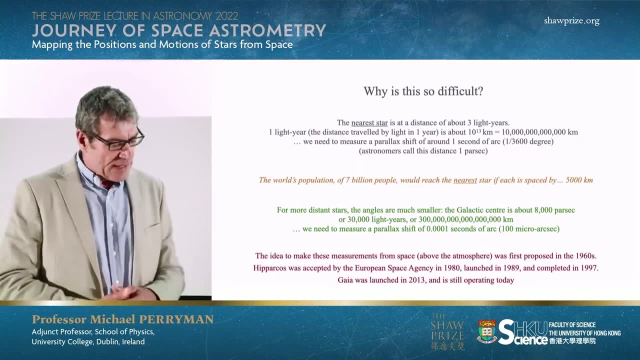 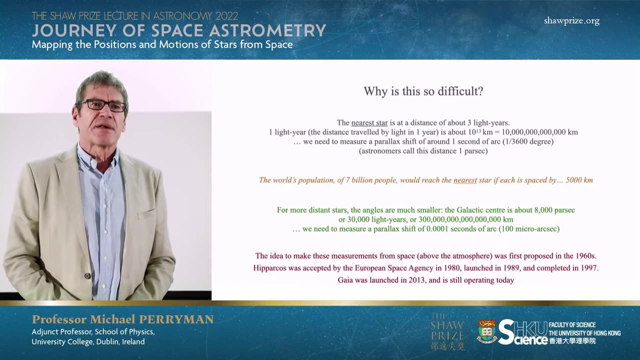 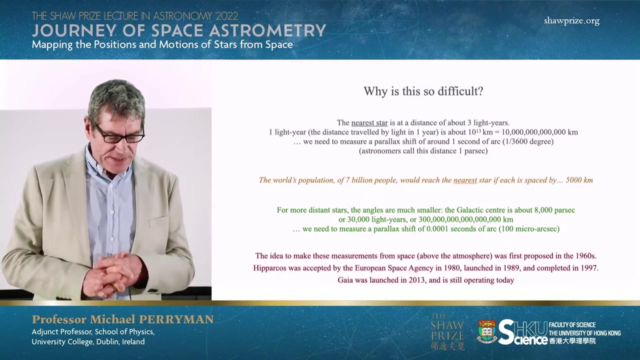 The mission completed its activities in 1997.. And it enabled the measurement of the distances to something like 100,000 stars, So that's just over 20 years ago. Hipparcos was so successful, so illuminating, that a second mission was accepted. 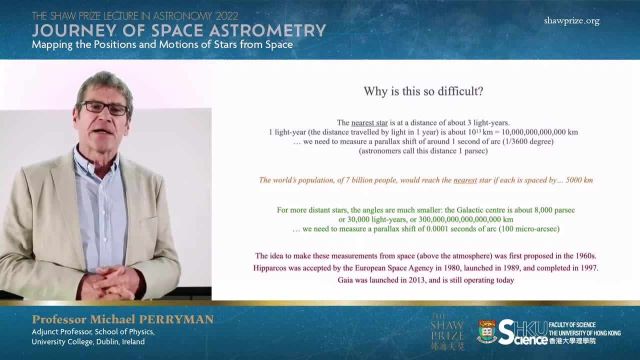 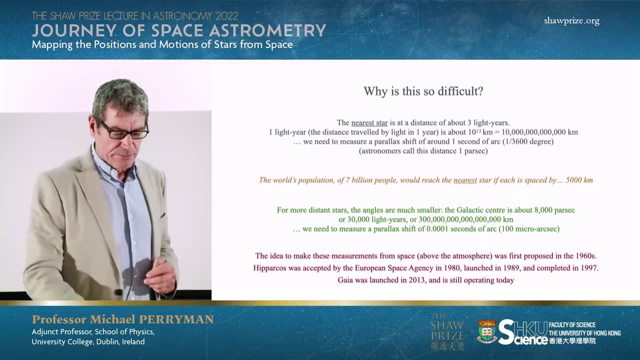 by the European Space Agency very quickly afterwards. Gaia. Gaia was launched in 2013, and it's still operating today And it's taking these measurements to much, much greater levels and much, much greater distances. So, from a dark sky location. 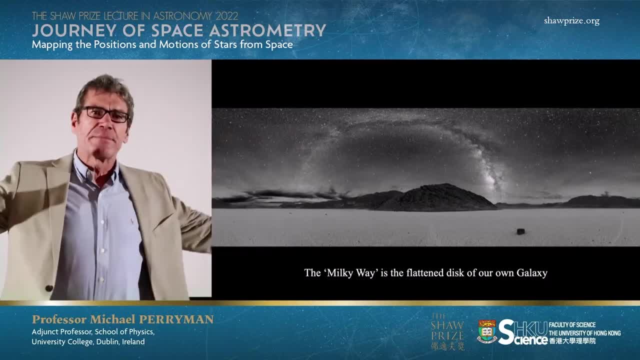 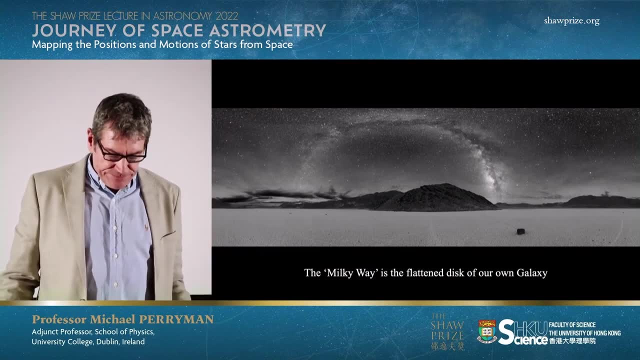 you can look up into the sky and you see this band, the Milky Way. And the Milky Way we now know is the flattened disk of our own galaxy. So if we could step outside of our galaxy, it would look something like this: 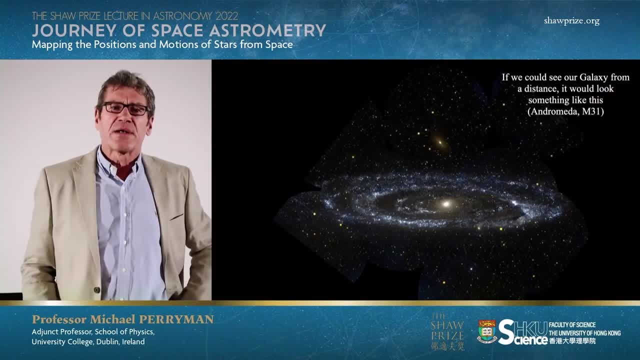 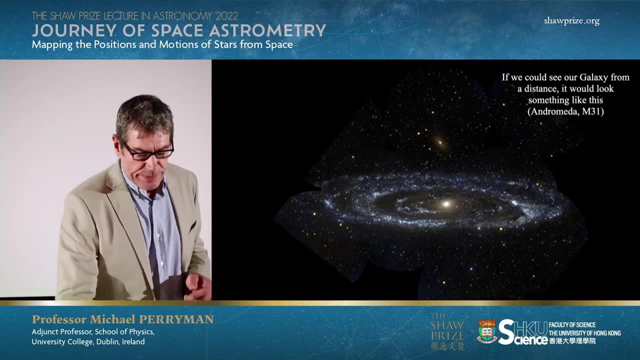 This is the Andromeda Galaxy M31. It's part of our local group of galaxies And we think our own galaxy looks something like this: We would be sitting the Sun and the planets around it would be sitting somewhere out here. 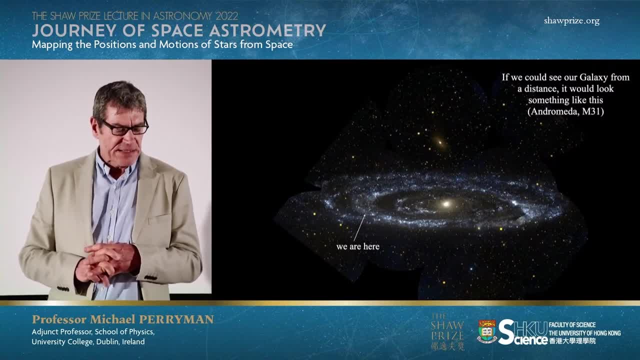 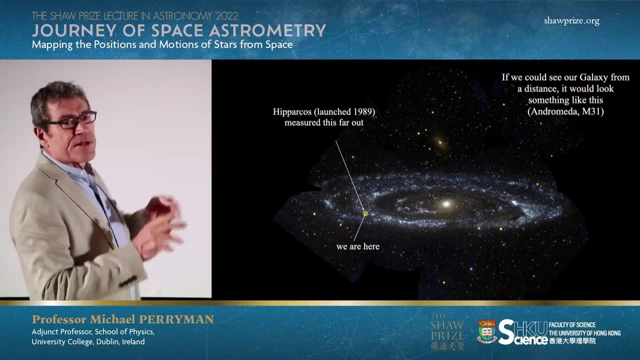 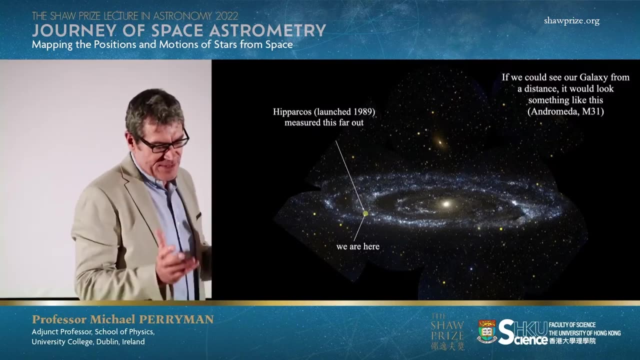 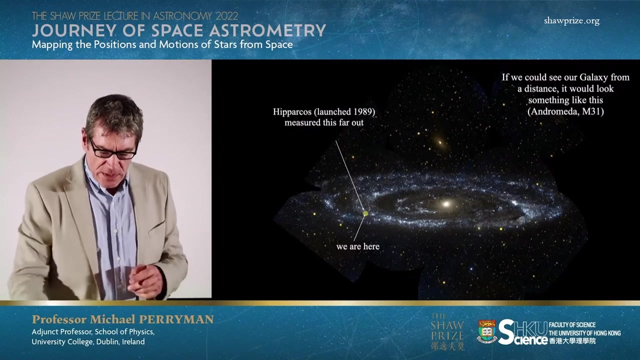 30,000 light years from the center, And this circle shows very roughly the sphere that we're able to access with Hipparcos. This small region around our Sun is the region out to which we could measure accurate distances and star motions, What Gaia has been able to do. 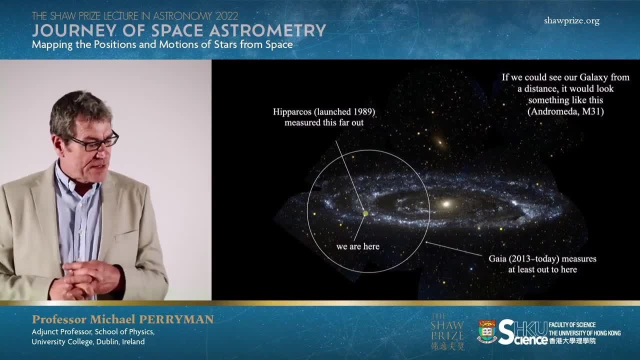 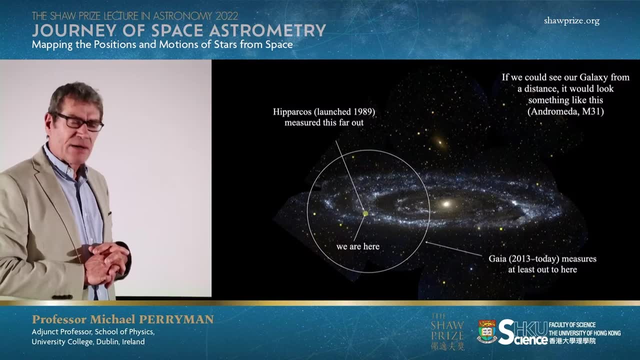 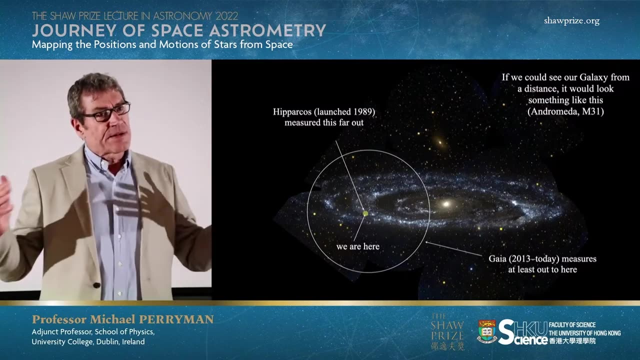 by improving enormously the accuracy that we can measure from space, is to expand our distance horizons out to much greater distances, out to distances something like the center of our own galaxy, And this means that we can measure the distances, the full stereoscopic. 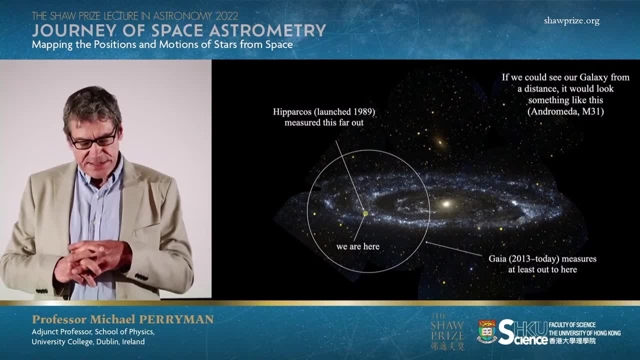 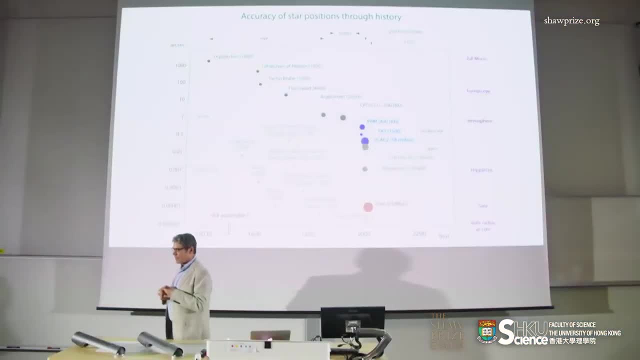 distribution of stars in our galaxy and also how they're moving through space. Now just to put this in a little bit of a historical context. there's a lot of information on here, but I show here the accuracy of measurements over time. 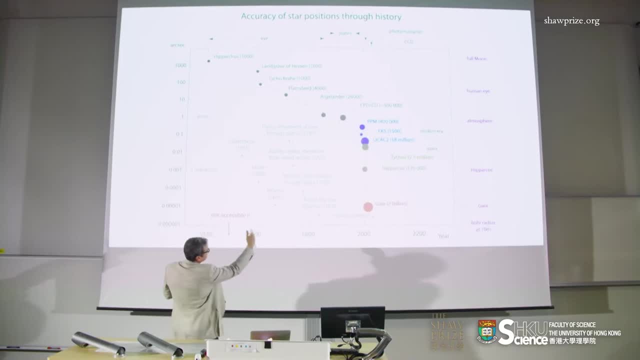 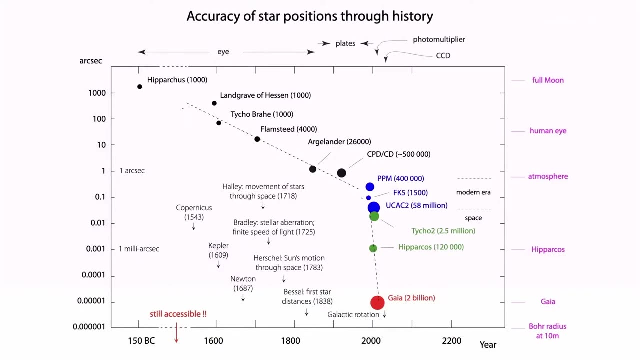 And this is going back to say 1500,, 1600,, 1800, and the year 2000.. And there's a logarithmic scale on the left and it shows how the accuracies have improved over time. 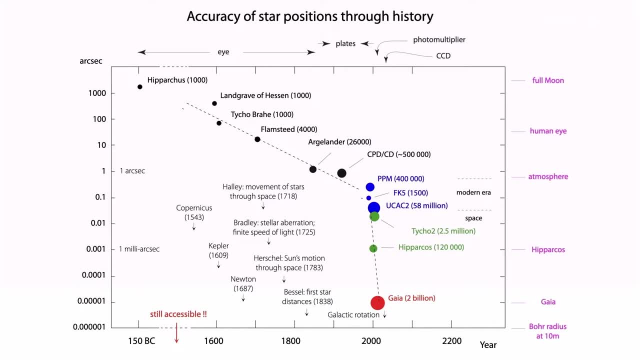 You see this dashed line going down And about 20 years ago, with the advent of space techniques, you can see Hipparcos suddenly moves the accuracies well down, and Gaia even much further still. And if we go back through history, 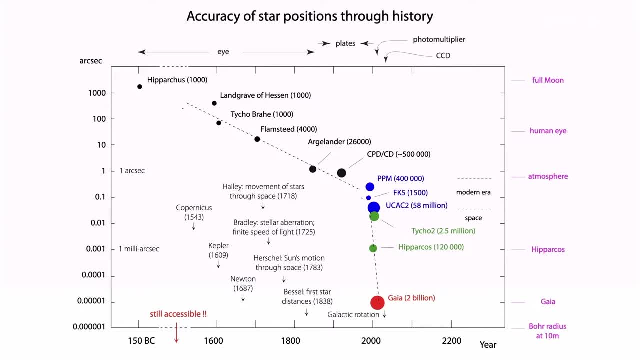 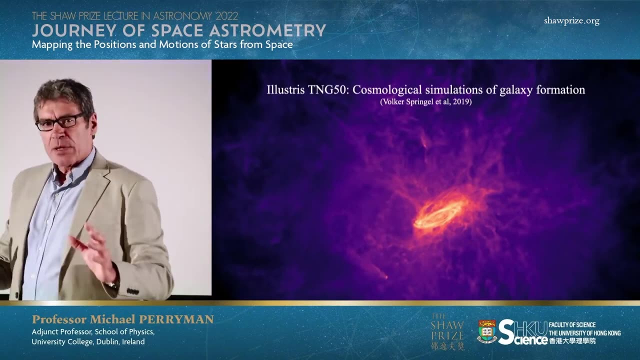 we can see that each of these improvements in accuracies has led to considerable insights into the nature of our galaxy and the universe surrounding us. I'm just going to come at the problem from a slightly different direction momentarily. This is nothing to do with Gaia. 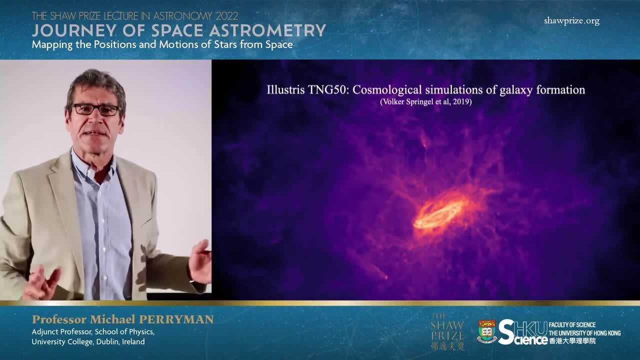 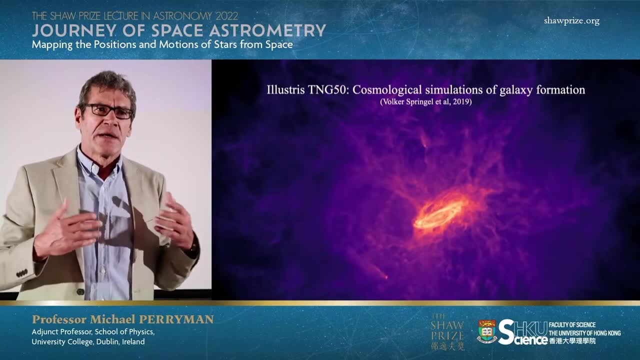 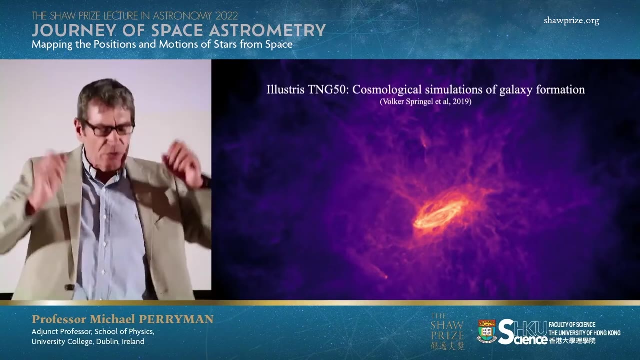 but it shows the state-of-the-art understanding of how our universe formed and how the galaxies within our universe formed, And it's from very extensive cosmological simulations that use all the ingredients that we understand today apply to our universe: The Big Bang, visible matter, dark matter, 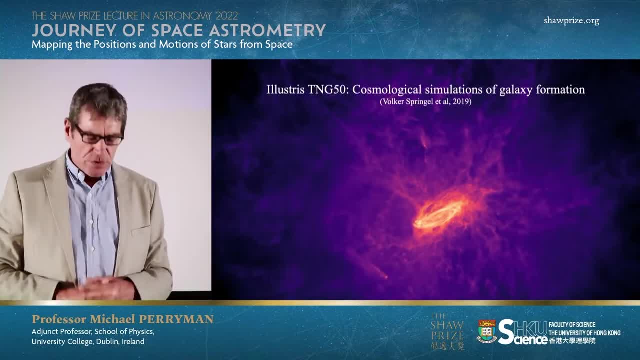 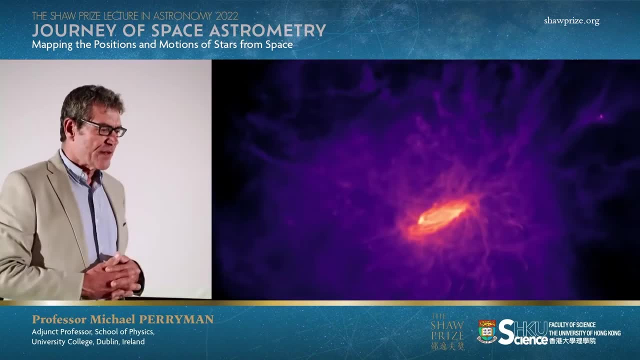 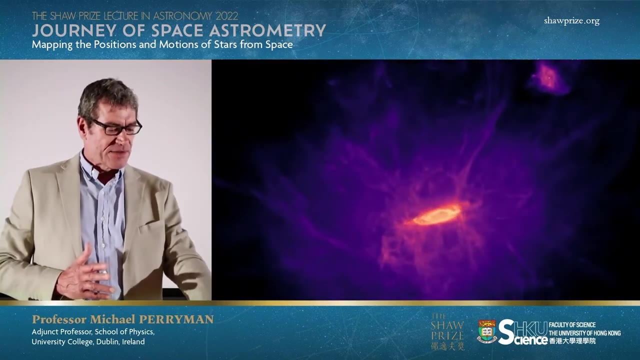 dark energy and so on. And these models are so detailed and so comprehensive that, setting this in motion, you can see over billions of years. you can see structure forming in there which looks a little bit like our own galaxy and satellite galaxies. 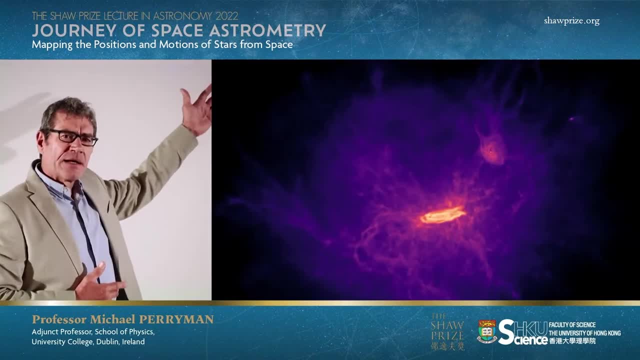 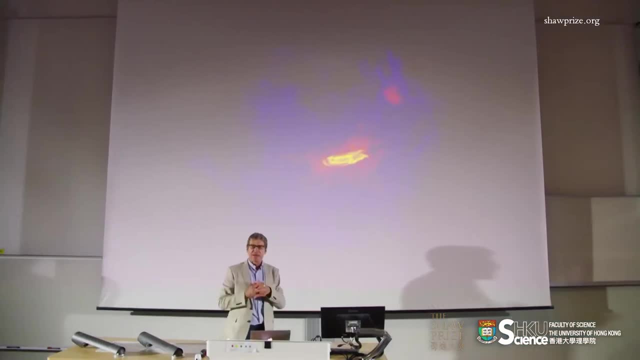 which are moving into the frame of the picture, which look very much like the Large Magellanic Cloud, one of our neighboring galaxies. The importance of this little animation is that it shows you that in any understanding of how our own galaxy formed, there's going to be an enormous amount. 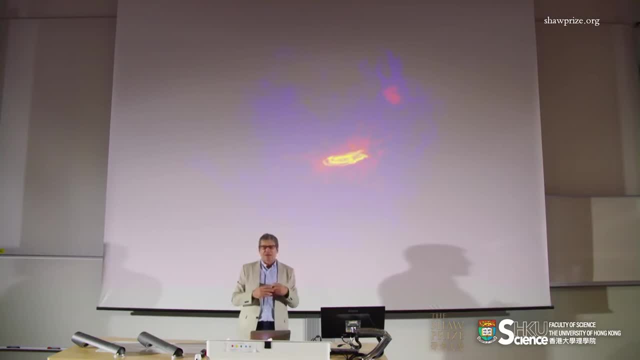 of structure in there, Concentrations of stars and complex motions of stars- And what Gaia is all about is really measuring huge numbers of stars and trying to put together a more complete picture of how our own galaxy formed. Now I'm going to just drop back. 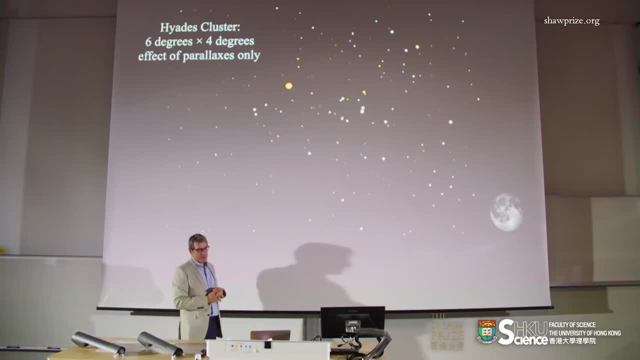 and show three little animations coming from the work on Hipparcos, so 20 years ago, And these, I think, still show quite effectively what it is we're trying to measure. This is a region of the sky about six degrees by four degrees. 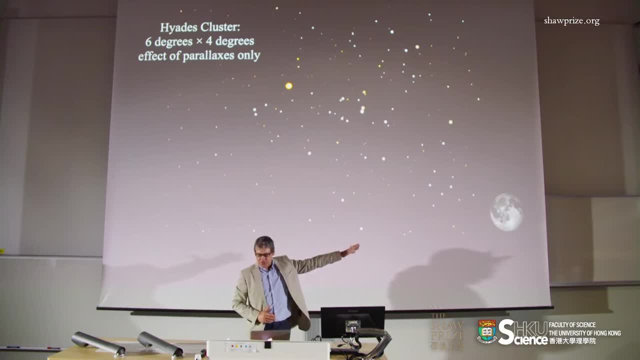 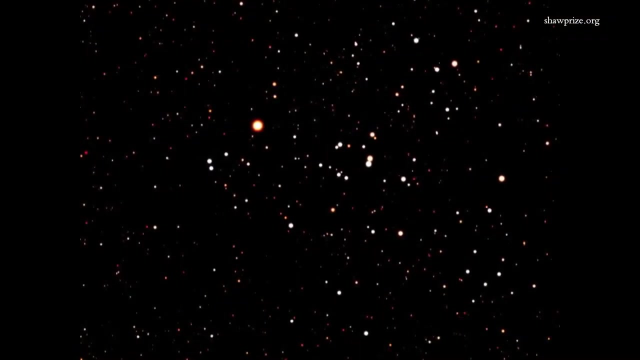 So in this the moon would occupy a region of sky, something like that, And what I've done in this animation is just to swing backwards and forwards around those stars to show you the effect of the distances. It's very difficult to communicate the idea of distances. 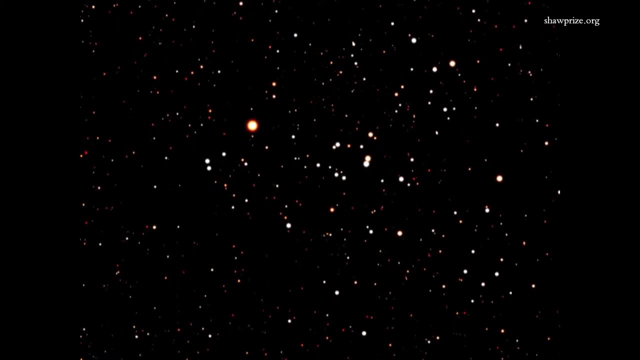 in a two-dimensional presentation, But by making sure that we're making this animation that swings backwards and forwards. the stars that are moving most are the stars nearest to us and the stars that are moving least are the background stars, And that is illustrating the effect of parallax. 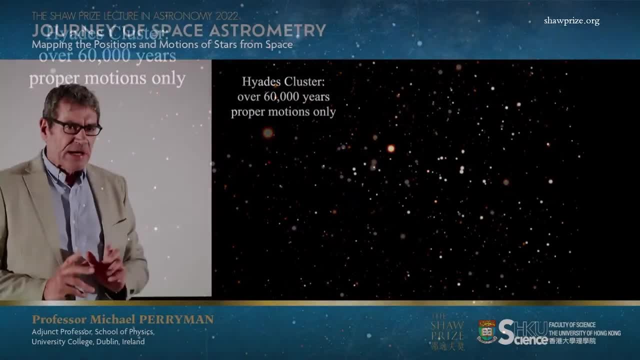 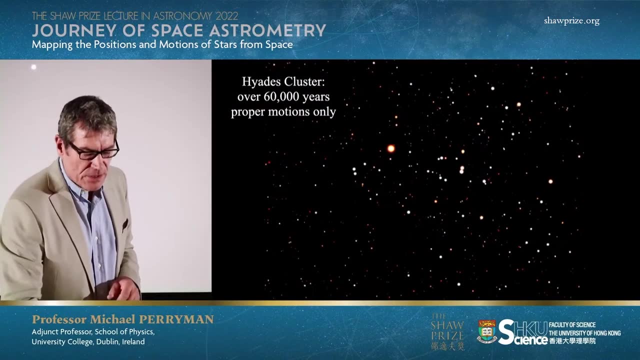 that I talked about earlier on. Now, at the same time, it turns out that we can measure how the stars are moving through space, And this shows the same region of sky- It's the Hyades Cluster- And it shows how the stars would be moving. 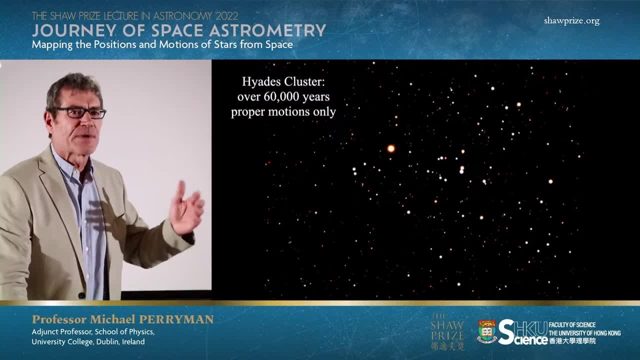 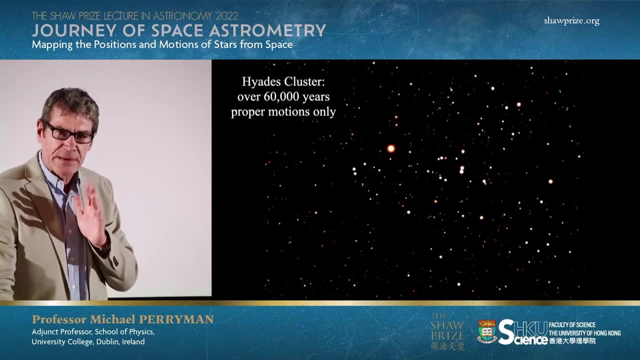 over 60,000 years on the basis of the measurements made from this satellite. over just three or four years, We can measure them so accurately that we can propagate their motions forward And you can see there that over the 60,000 years. 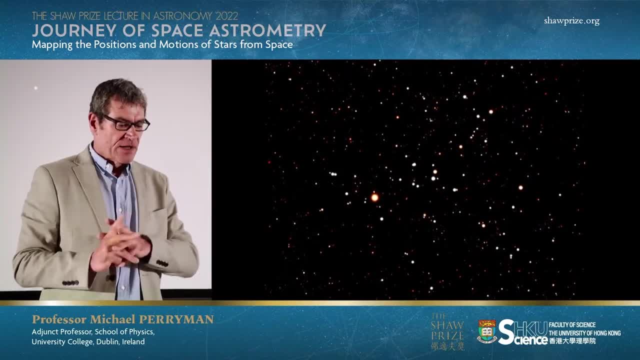 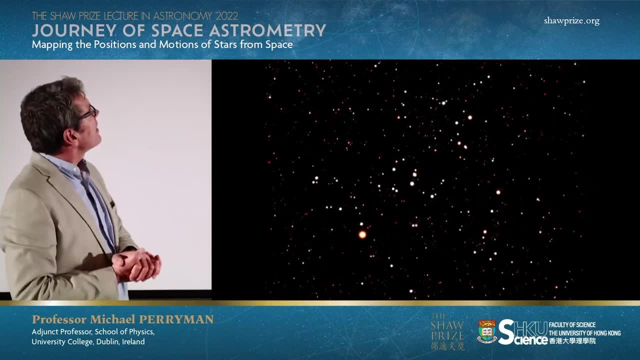 stars are not moving the same way at all through space. Some of them are. Most of them are moving right to left as we look at this. This is the bright star, Aldebaran, and it's moving from top to bottom, But other stars are in the background. 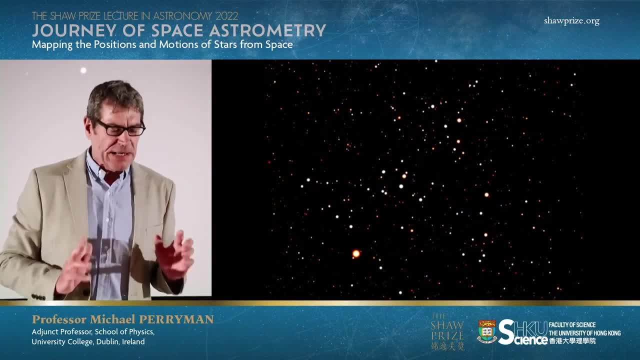 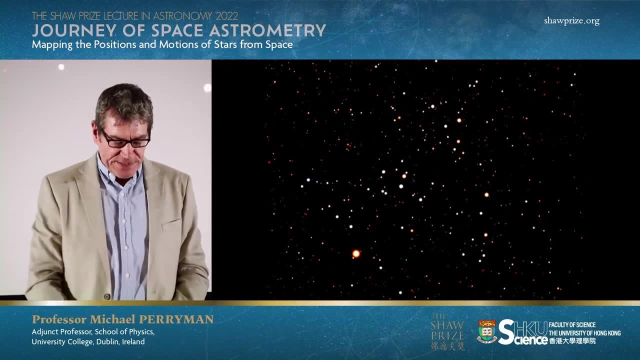 and moving in very different ways. This is trying to explain that if we can measure simultaneously the distance to the stars and also the way the stars are moving through space, we can infer a lot about the structure of our galaxy And we can put those two effects together. 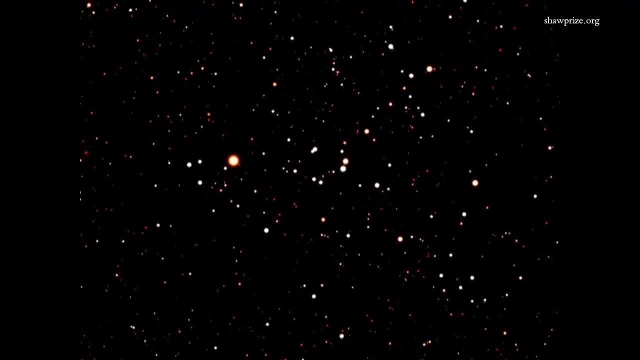 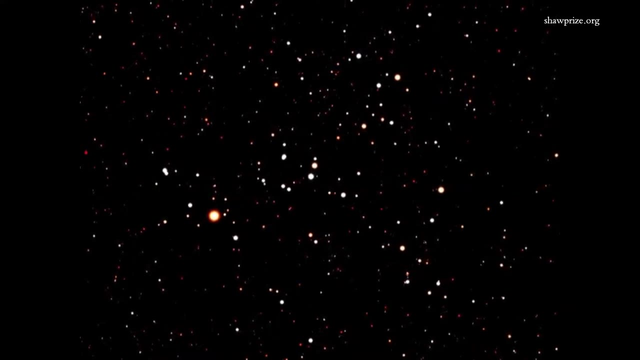 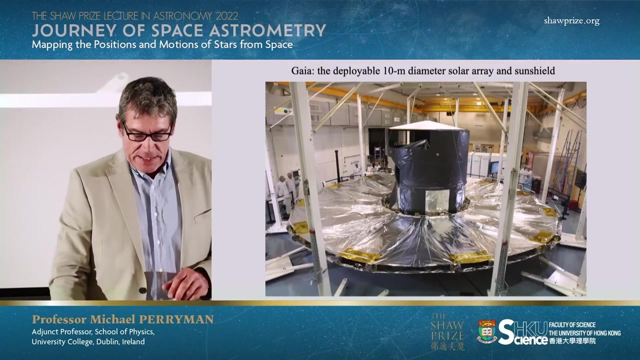 combine the parallax motion and the proper motion and you can see that these stars are moving in apparently very complex ways And they're encoding the information about their distance and their motion through space. I will just show. It's not my goal today. 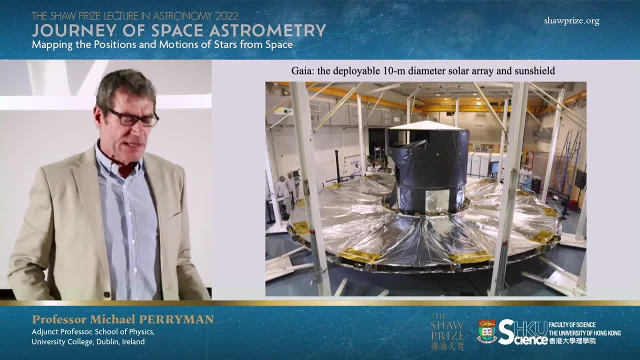 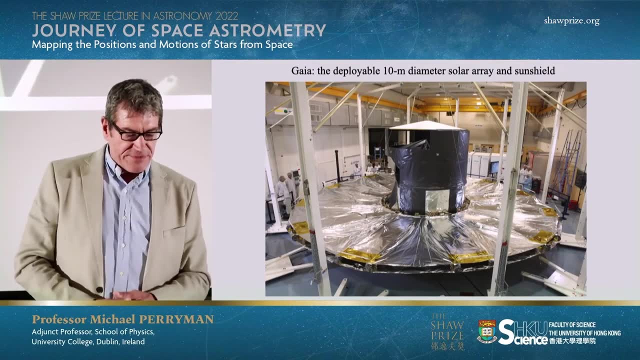 to tell you in detail how this is done or to tell you in detail about the Gaia satellite, but I think it's a nice opportunity to just show you a couple of pictures. Here is Gaia in the test facilities: assembly facilities before launch. 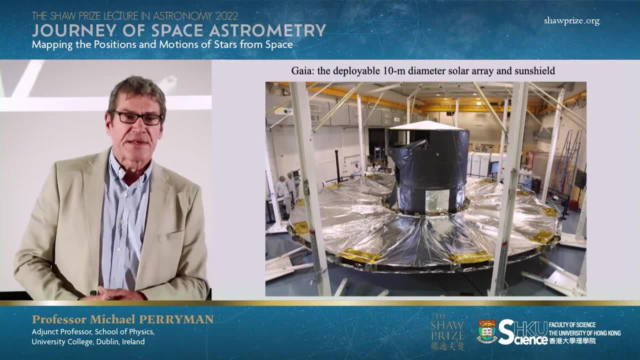 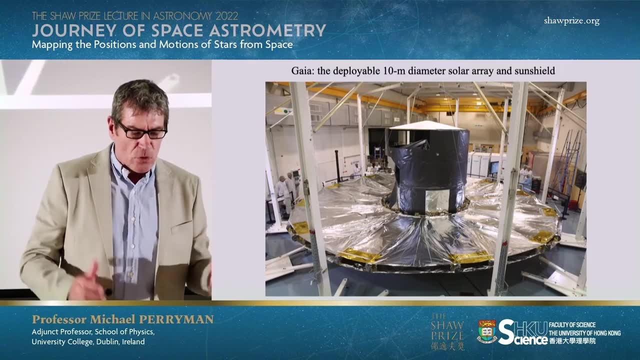 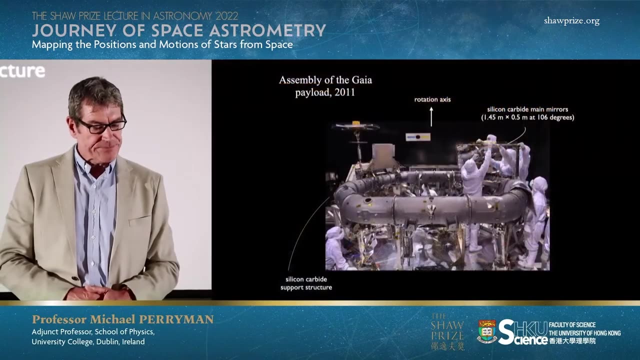 There are people around the side of it. It's a sun shield which is very much like the sun shield that you've seen with James Webb Space Telescope. It was deployable And it shields this very delicate payload assembly from the intense radiation from the sun. 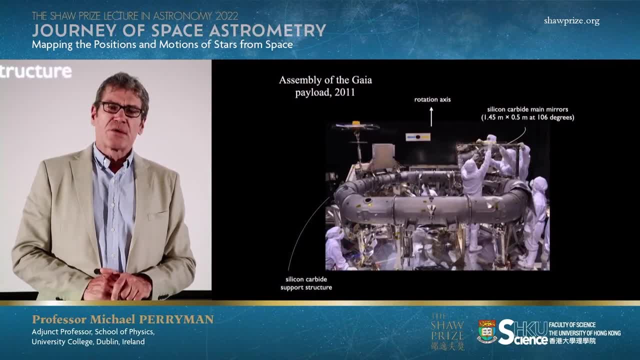 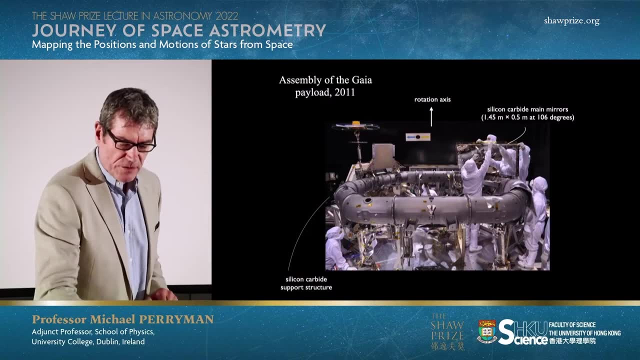 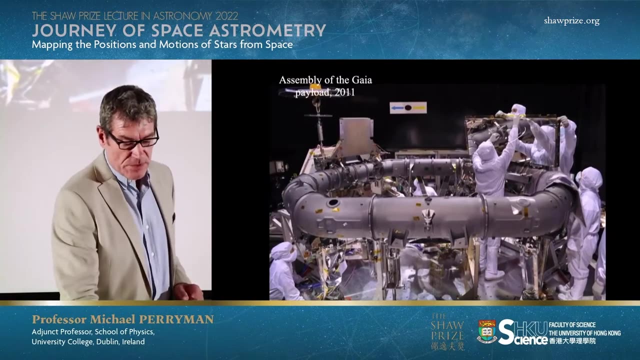 The telescope is a huge and very, very accurate system. It's built around a very stable torus structure and you can see one of the two main mirrors there being assembled back in 2011,, shortly before launch. That's all I'm going to say. 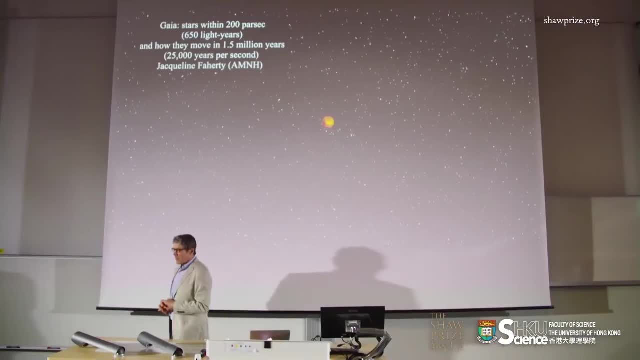 on the Gaia satellite itself. Where are we with the results from Gaia? Well, what we can start to do now is to put together a little animation, and this is one created by Jacqueline Flaherty at the American Museum of Natural History. 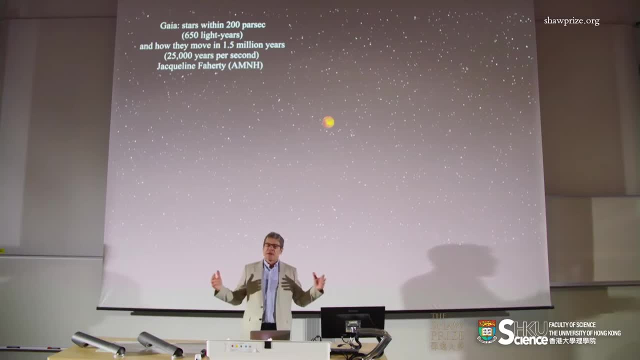 And what she's done is to take the stars within 200 parsecs. It's about 500, 600 light years, so it's still very close to us in absolute terms, And she's just made this little animation which shows how the stars move. 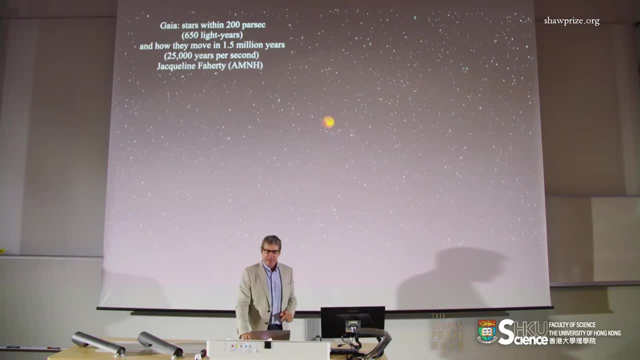 over a period of 1.5 million years. Again, we can't possibly measure them over 1.5 million years, but we can measure them sufficiently accurately that we can predict how they will move through space over 1.5 million years. 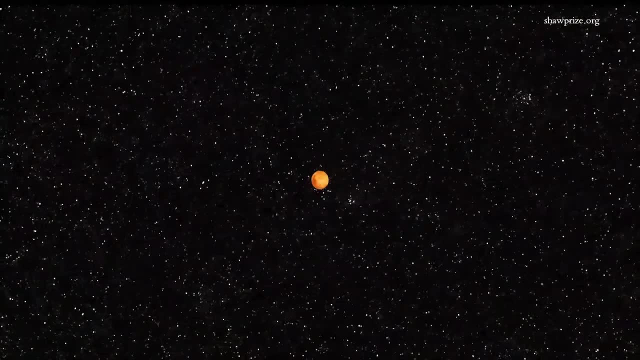 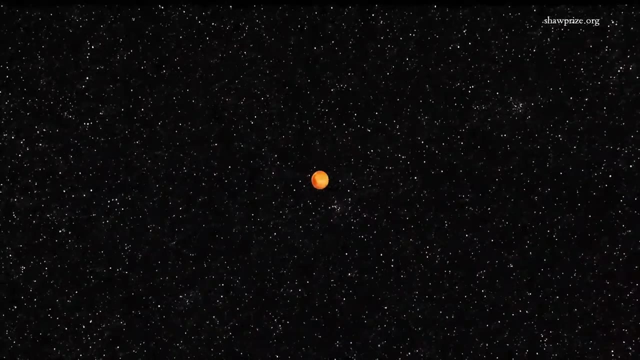 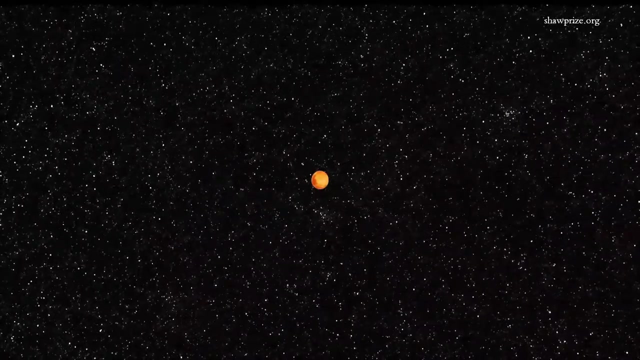 And if we watch that little animation unfolding, you'll see all sorts of complex structures. We've got clusters of stars, open clusters moving in different ways, stars moving in very complex ways, And you can see from time to time stars shooting through the. 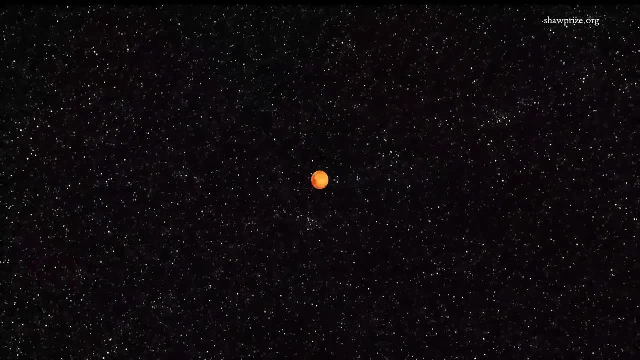 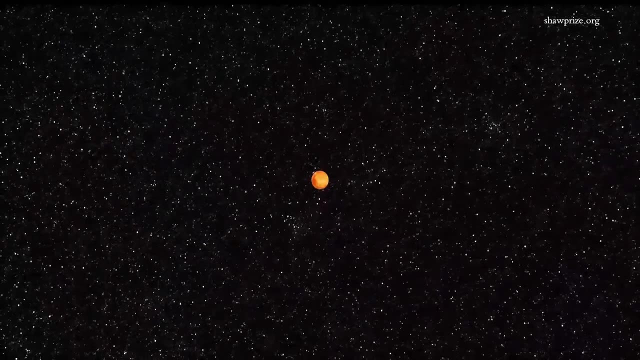 animation at very high speed. These are stars which are in the halo of our galaxy and just passing through very close to us and very rapidly. So this is just a little, one little snapshot of the Gaia results, but it gives you a clue. 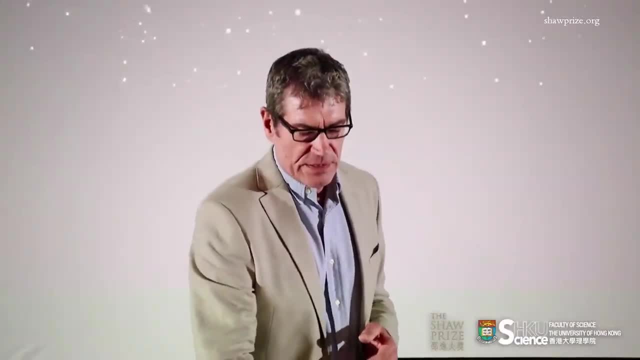 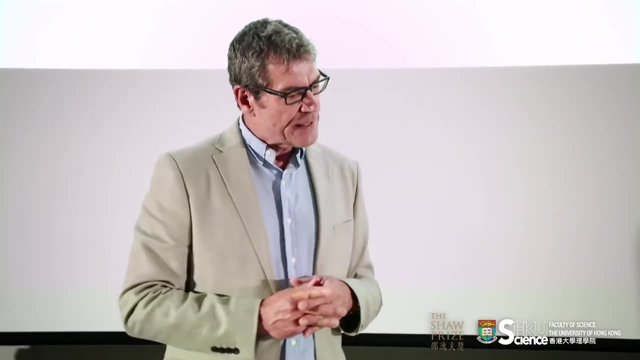 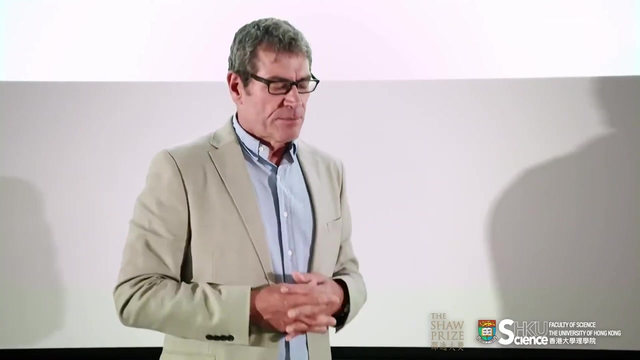 as to how we are piecing together these stellar motions in our region of the galaxy. Now, what I'm going to do in the remainder of my talk is just to pick out five or six of some of the things that are emerging from these investigations. 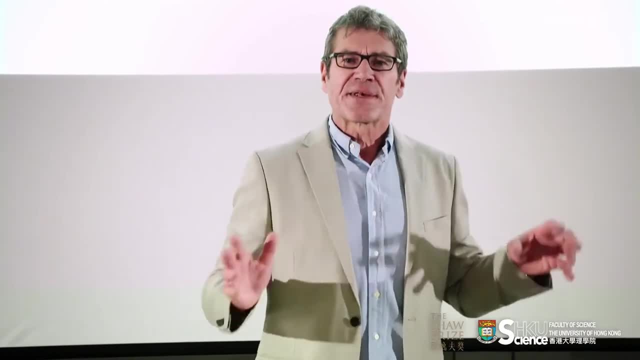 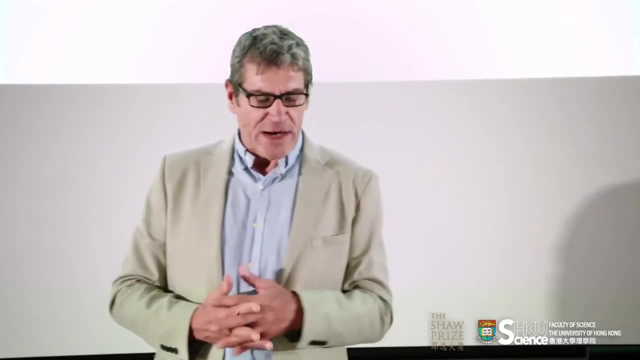 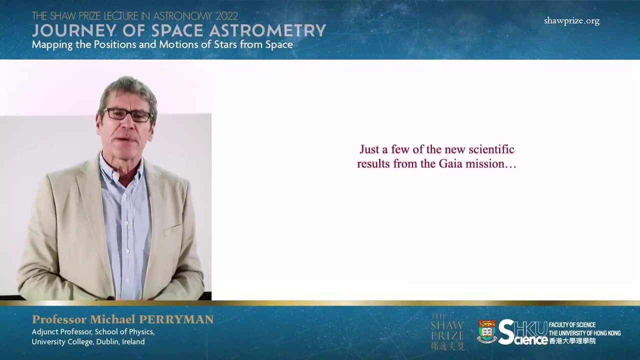 Now you may imagine that, with 2 billion stars being measured by Gaia, Gaia is really impacting almost all areas of astronomy, so it's pretty much impossible to give you a detailed insight into what's coming on, but I hope I can give you a little bit of a flavour. 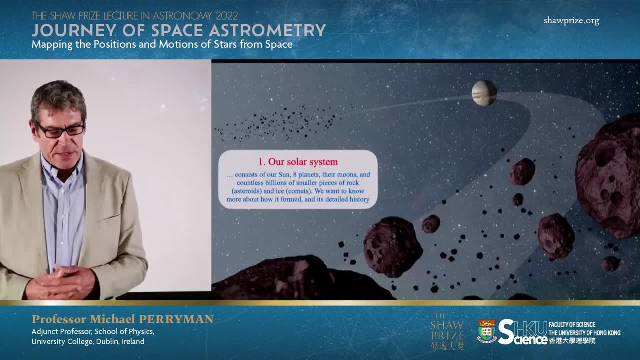 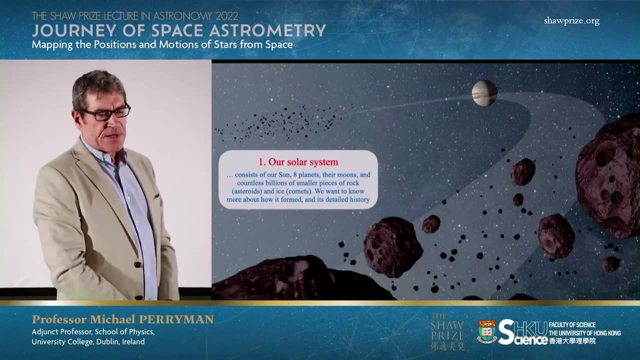 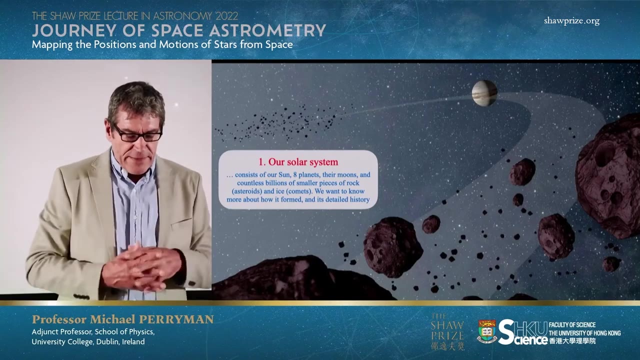 of what we are discovering. So I'm going to start with the nearby and move outwards. go through each of these quite quickly. The first is the solar system. It turns out that Gaia is not only measuring stars in our galaxy, but we're also measuring 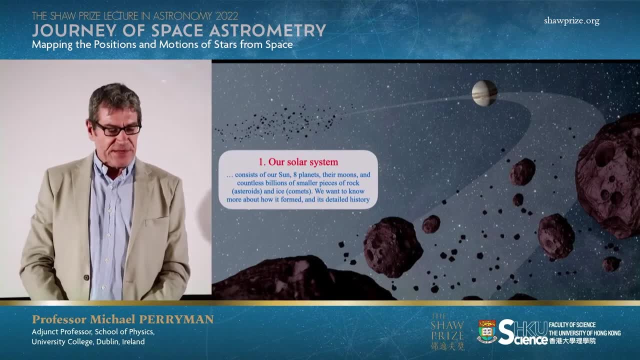 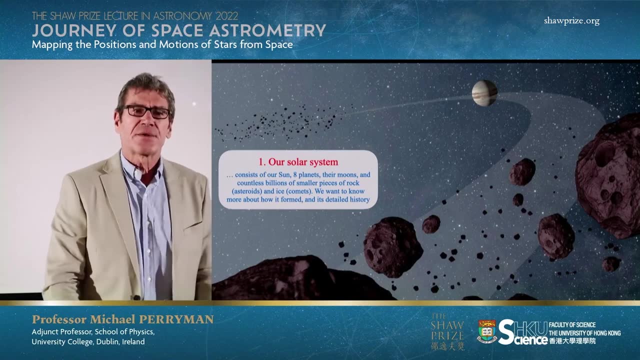 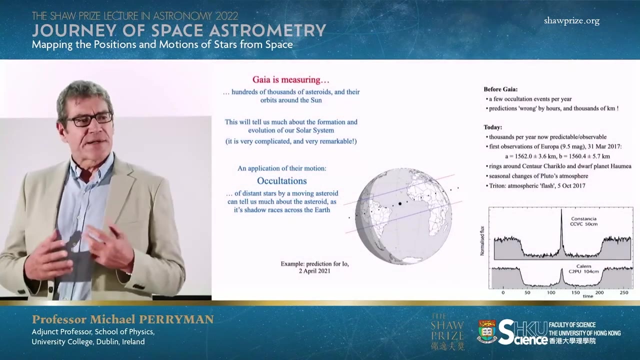 asteroids and other bodies in the solar system, And Gaia will eventually, in the final catalogue, contain several hundred thousand of these rocky bodies in our solar system. What are we using this for? We're using this to try and understand the history of the formation and the evolution. 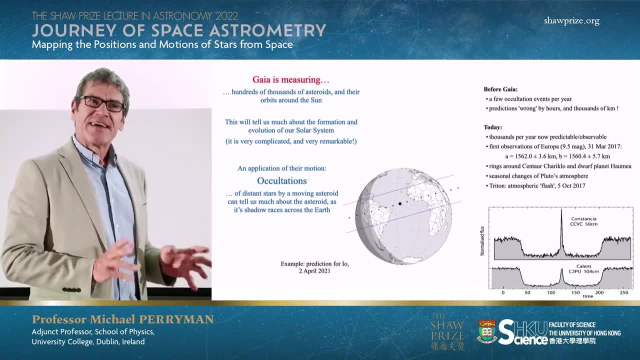 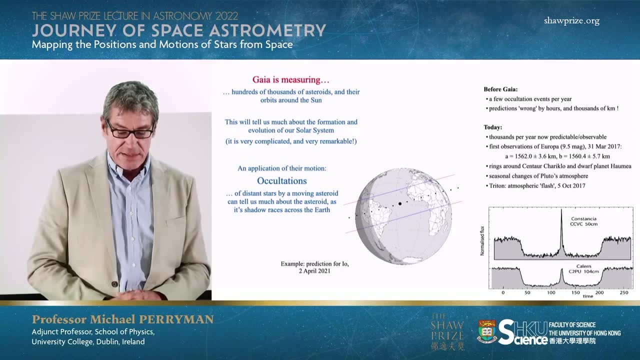 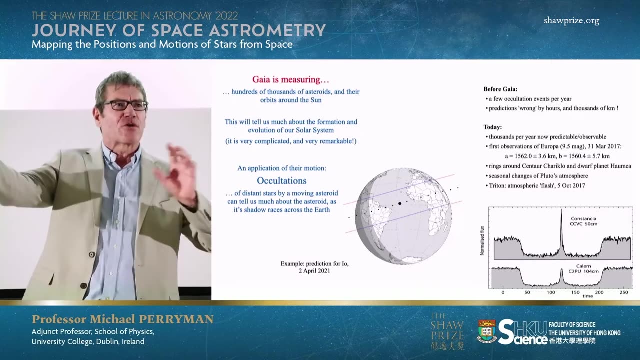 of our own solar system, And one of the very beautiful, clever techniques that's actually being used as well by amateurs who are assisting the Gaia scientists with this is the occultations of stars as the asteroid bodies move across them. Now I ask you to imagine. 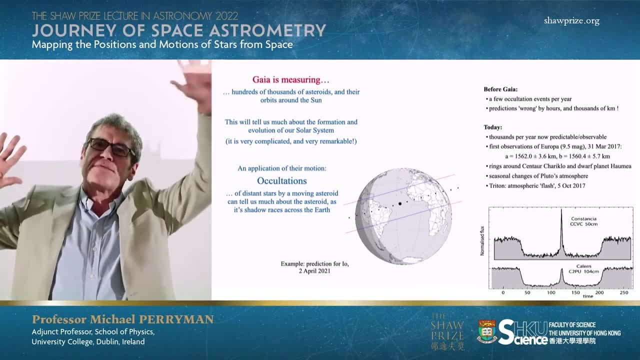 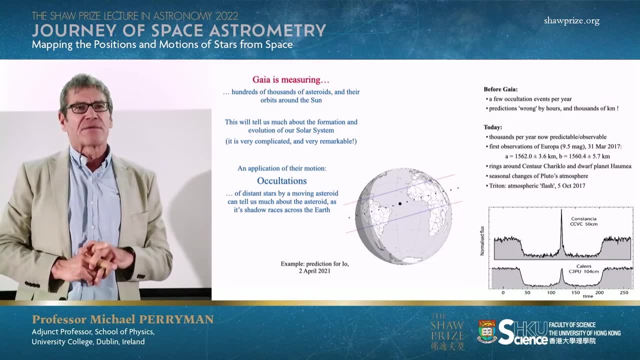 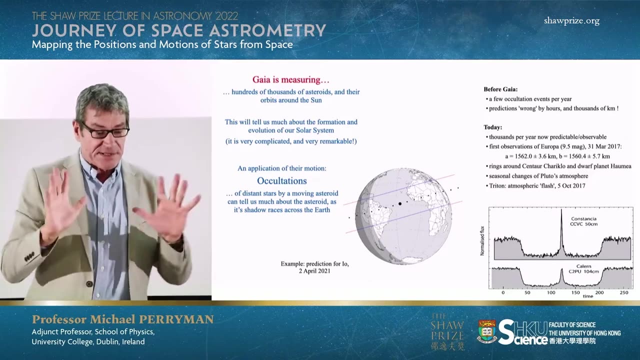 hundreds of thousands of rocky bodies moving in front of billions, millions or billions of stars that are also moving slowly through space, and you may imagine that from time to time, one of these rocky bodies passes in front of the star, A star- And when it does that, 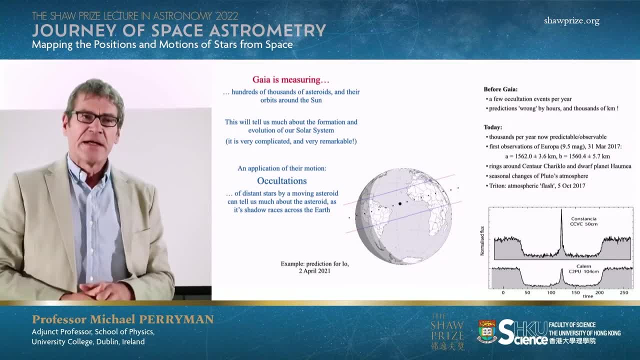 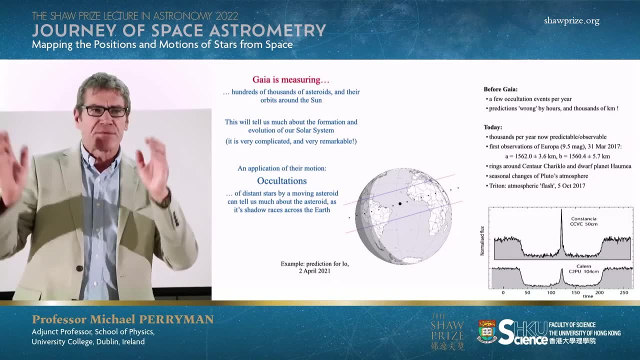 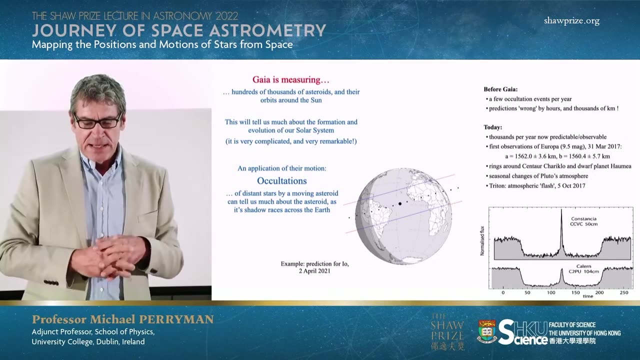 the light is diminished coming from the star and if we can predict where these occultations are going to happen on Earth. astronomers can watch this, look out for them and measure the attenuation in light as the rocky body passes across the face of this star. And now? 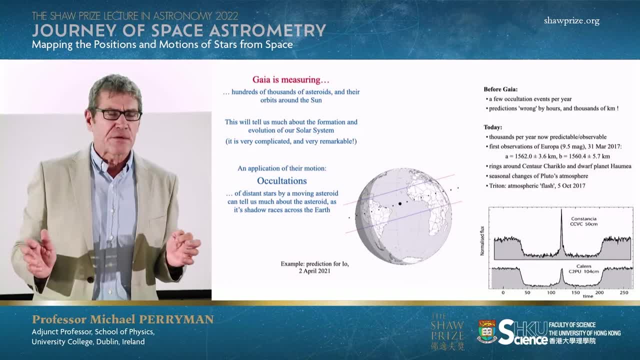 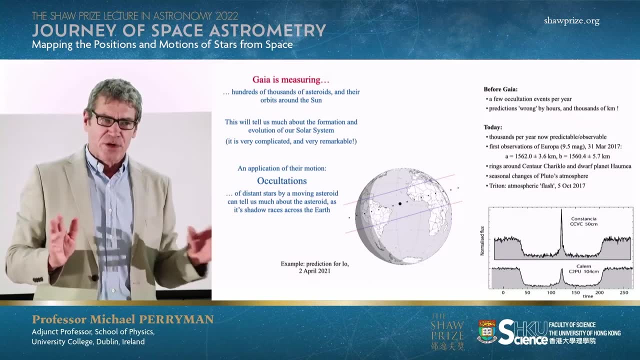 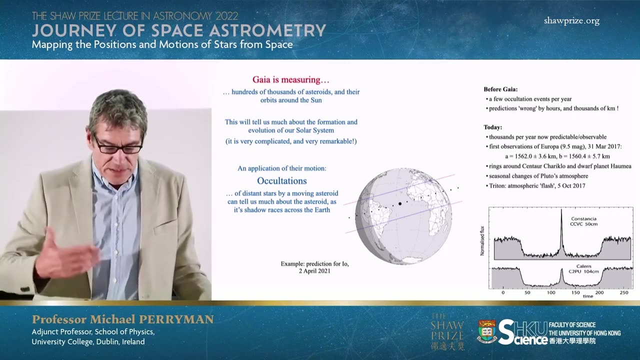 we're in a position to predict thousands of these each year, to get the occultation time accurate to a few seconds and to start saying an awful lot about the sizes of these rocky asteroidal bodies, or even if the body has an atmosphere, for example. 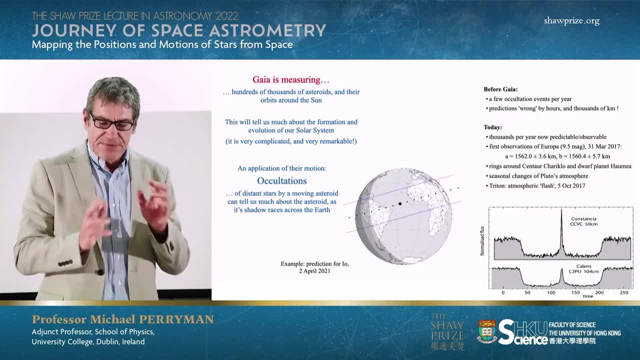 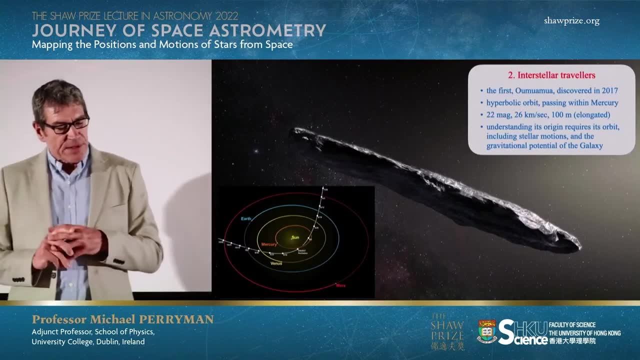 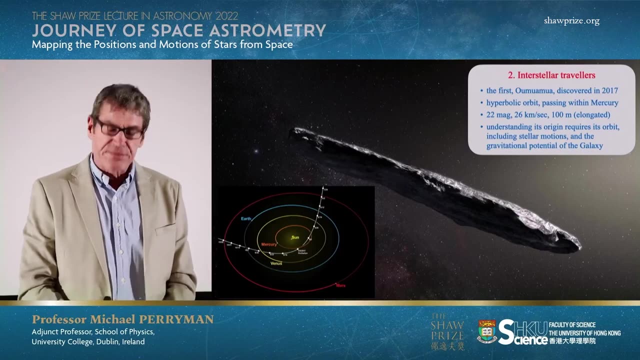 Pluto. we can see the effects of the atmosphere as the asteroid passes across the star. My next example is something which emerged into great excitement five years ago: the discovery of the first interstellar traveler, or interstellar vagabond. This is a piece of rock that is passing. 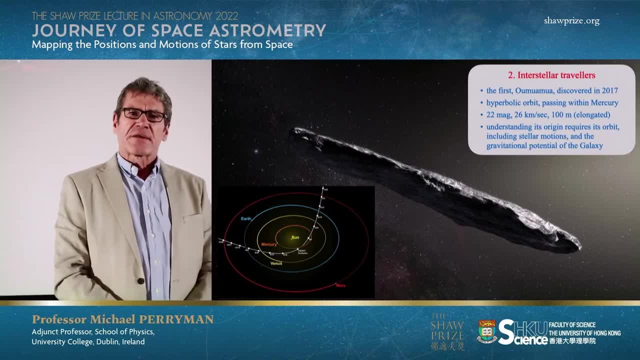 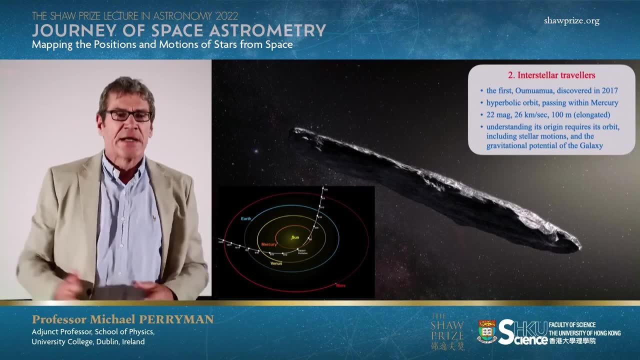 through the solar system which has an orbit such that we can say definitively it's not bound to the solar system. It must have come in from somewhere and it's going to fly past the sun and it's going to head off into. 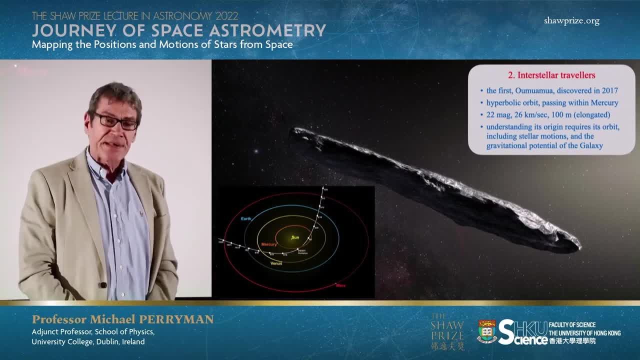 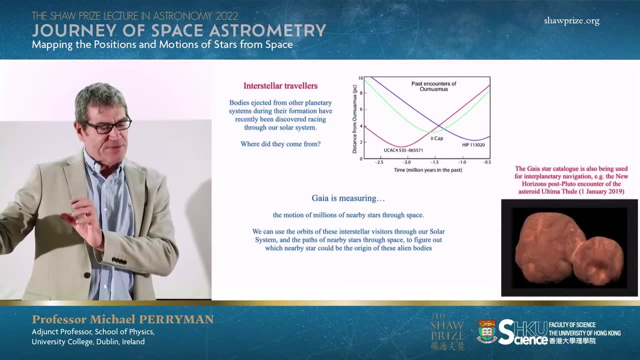 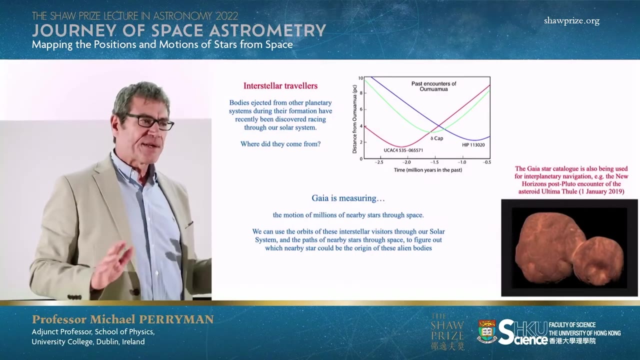 space And there was a great excitement with this, and one of the things that Gaia is now doing is to taking the orbit of these interstellar travelers and piecing it together with the orbits of the stars, is to figure out which star system close. 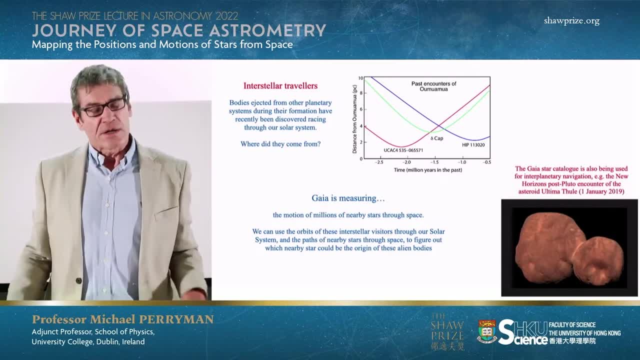 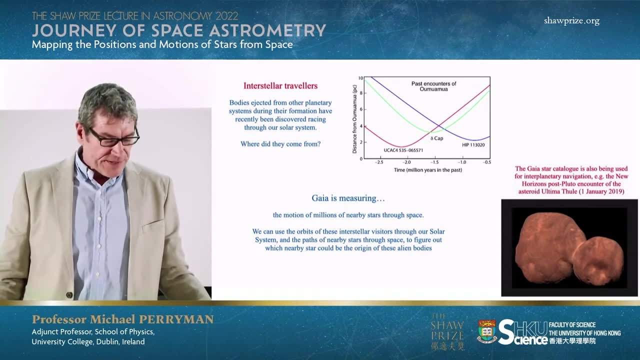 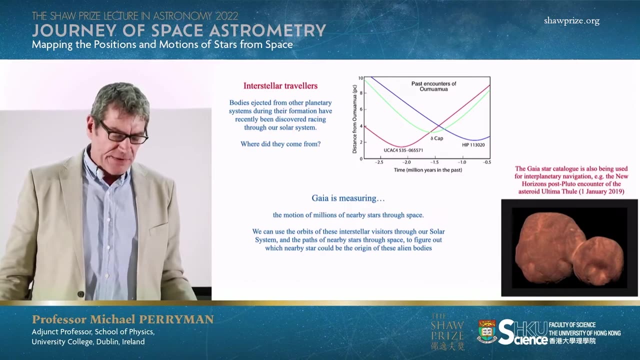 to us. this particular piece of rock was ejected from, So there's a greater excitement. there's more of these interstellar travelers been discovered since The Gaia system. the stars in the catalog are so accurately placed that they're being used as well. 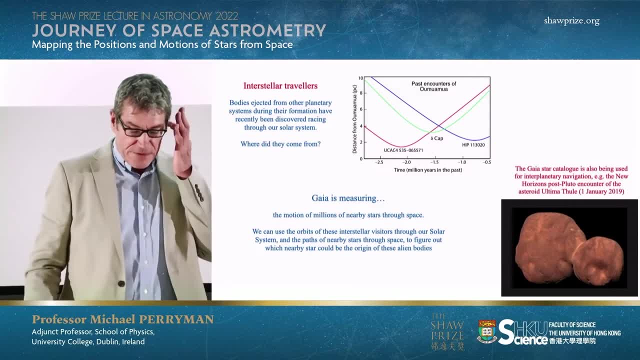 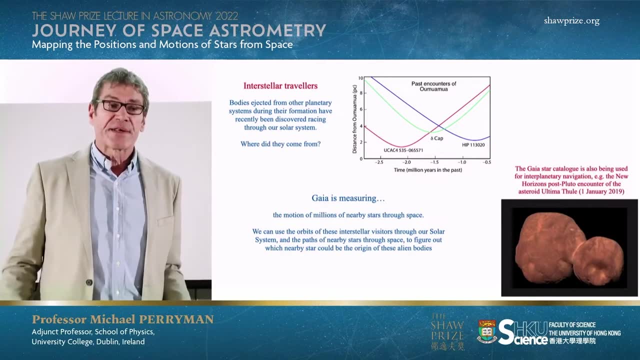 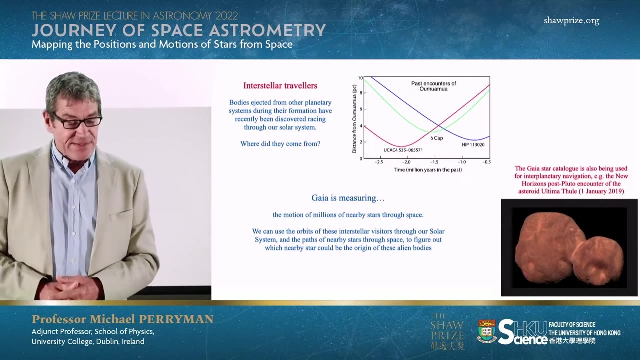 for interstellar navigation- sorry, interplanetary navigation. and a highlight three years ago was the reorientation of the New Horizons spacecraft by NASA in its close encounter with an asteroid called Ultima Thule and using the reference system from Gaia, enabled. 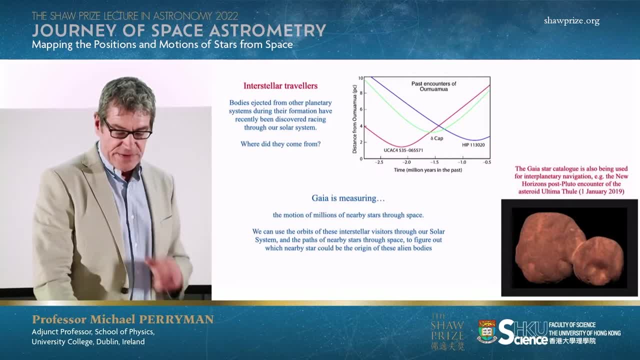 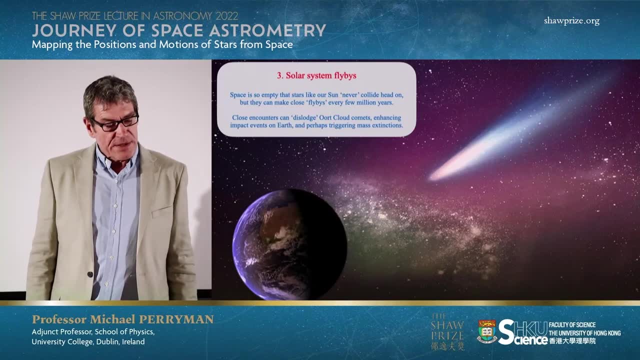 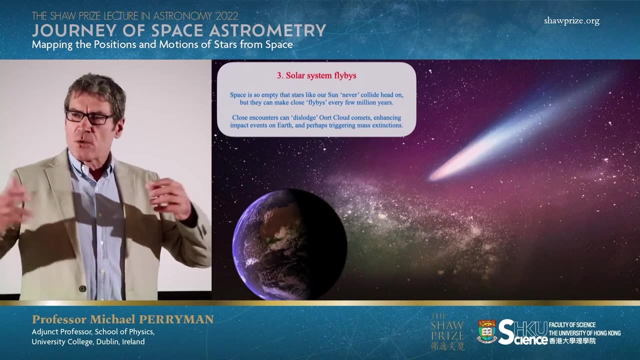 the imaging camera to be pointed directly and get this great snapshot of Ultima Thule. I move on to the third topic which I want to mention, which is solar system flybys. Our own sun is moving through the galaxy. all the other stars are moving through the galaxy. 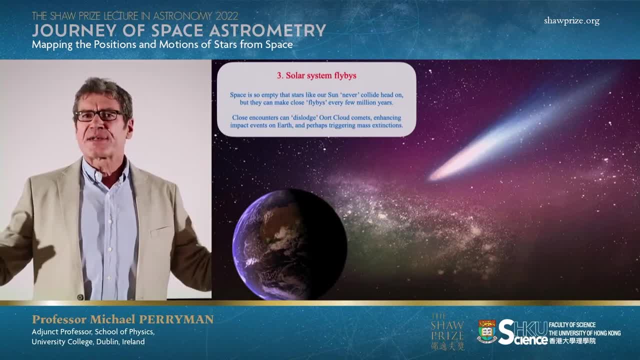 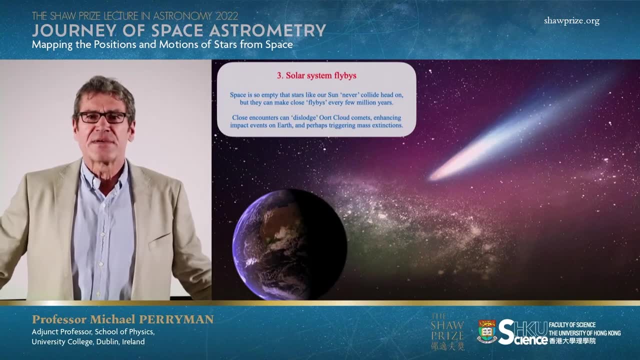 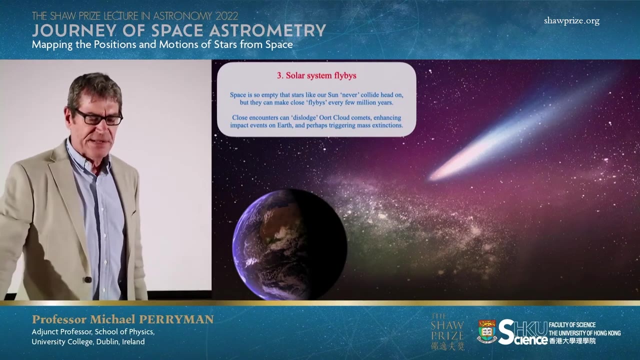 You may ask the question: how long will it take our sun to collide with a nearby star? Well, the answer is fortunately never, or effectively never. It will take thousands of times the age of the universe for our sun to stand any chance of hitting. 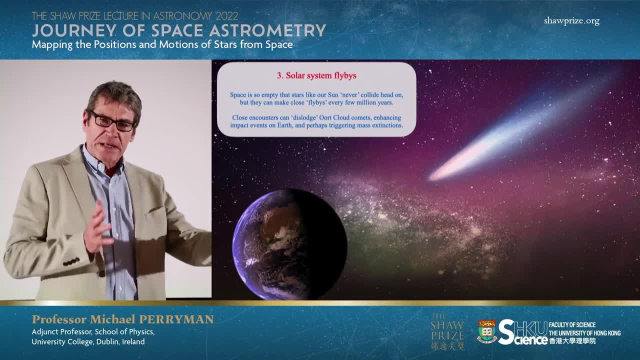 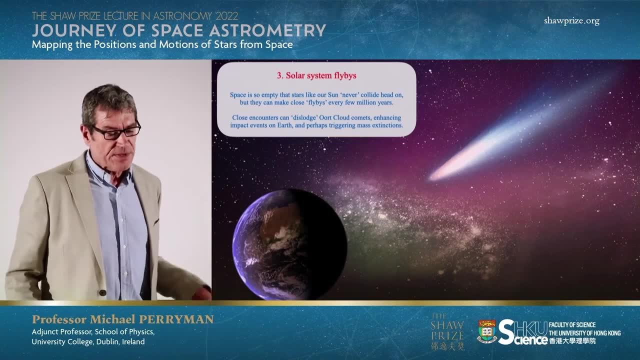 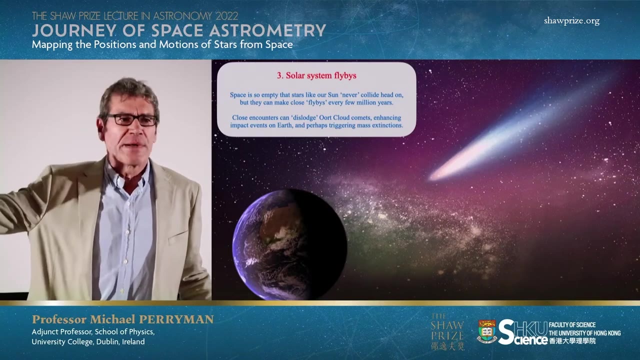 one of the other moving stars. but what can happen is that nearby stars which are moving through space can come close to our own star, relatively close to our own star. our own sun and this, turns out, dislodges some of the icy comets that are. 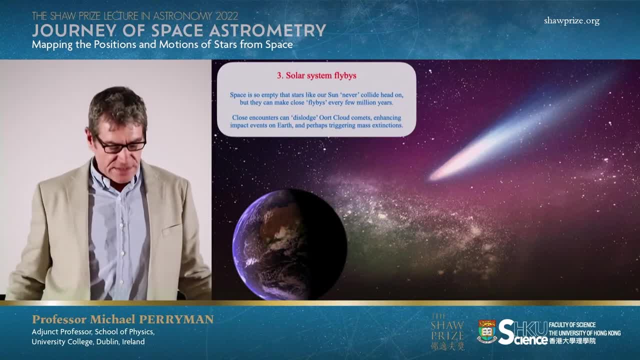 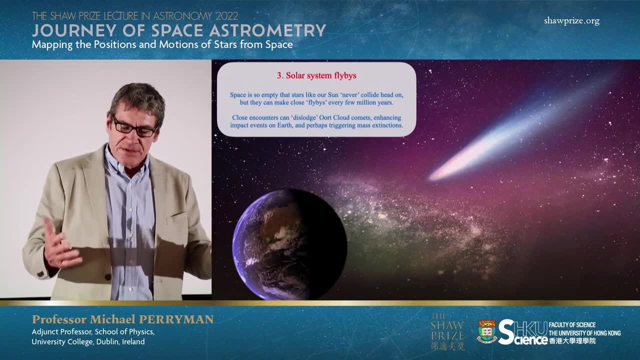 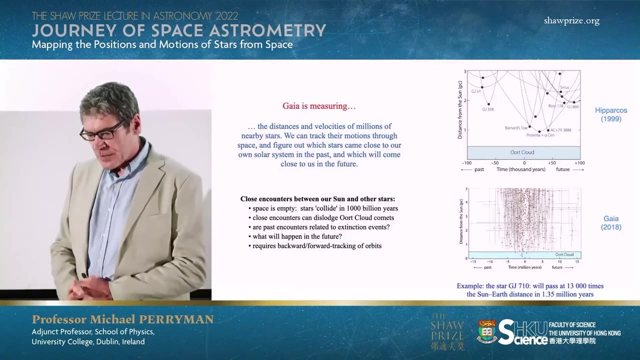 sitting far out in the solar system, remnants of its early formation, and they can be deflected inwards and create cometary clouds that are timed with these close passages of these stars. So one of the scientific topics that was started with Hipparchos. results, and has now become a lot more precise and rigorous with the accuracy of Gaia- is to look at the stars in our neighboring region of the galaxy and see which ones could have come close to us in the past and which ones will come close to us in the future. 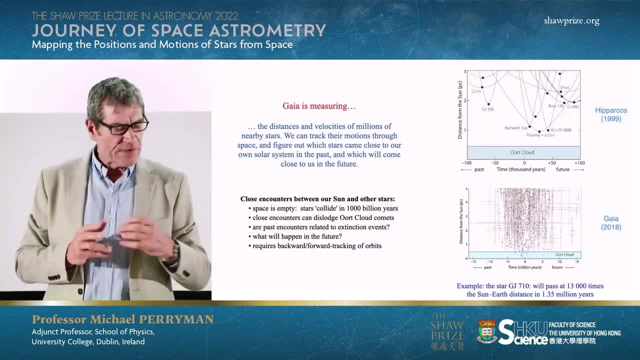 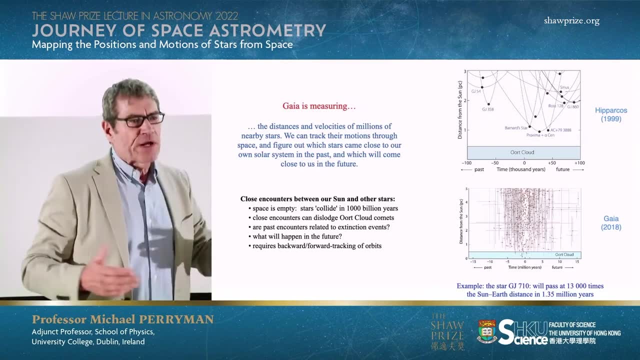 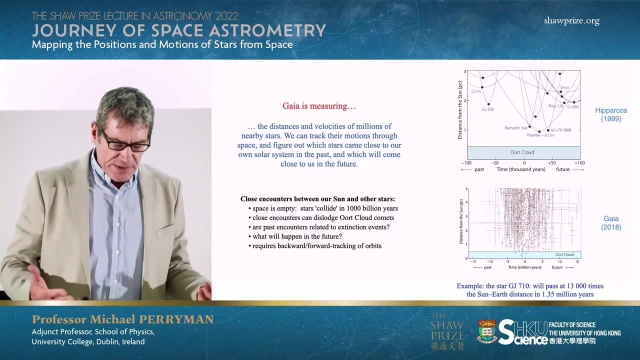 And some groups. what they're trying to do is to figure out whether these close stellar passages might have created the kind of cometary impacts that, for example, could have led to the extinction of the dinosaurs 63 million years ago. So stars don't collide. 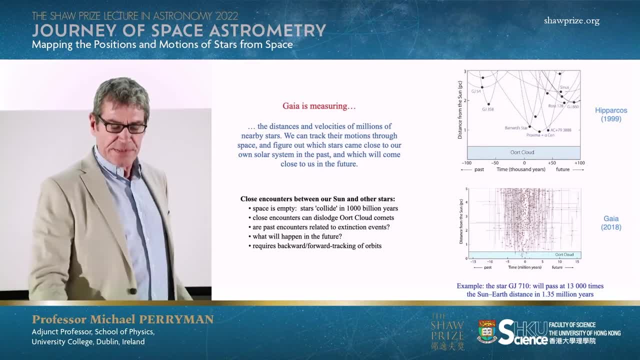 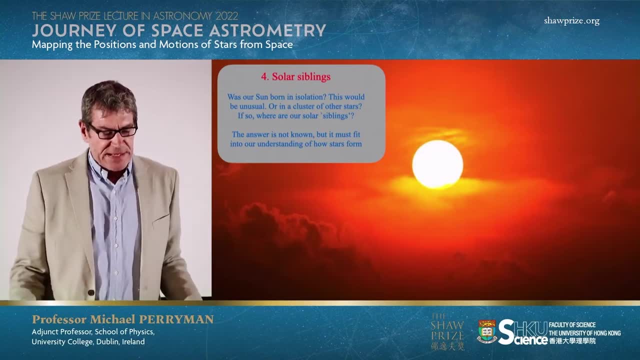 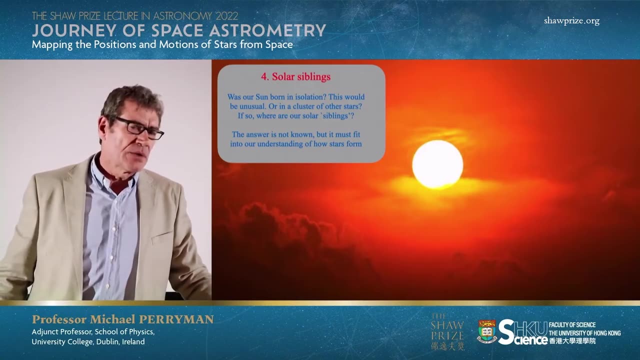 but they can come close enough to disrupt the other bodies in the solar system. The fourth topic that I've selected is to ask a very interesting question in astronomy: Was our sun born alone? Was it formed on its own? This would be very unusual. in astronomy. This is not the way stars are believed to form. Stars are believed to form in groups, clusters and so on. Our sun almost certainly formed in a cluster of other stars, but they're not there now. so where are they? 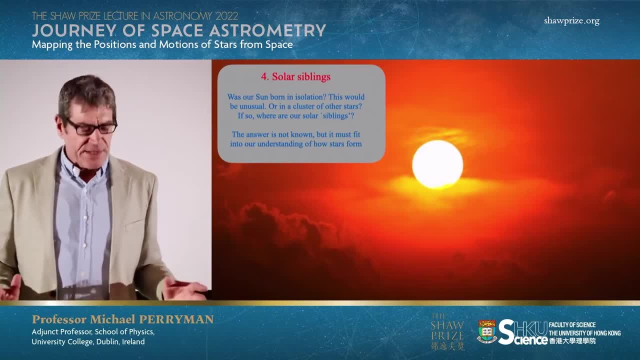 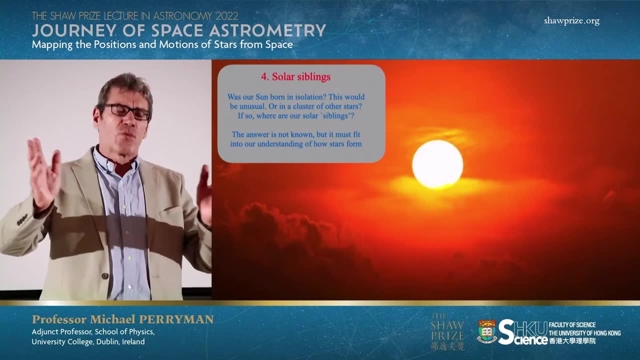 We have sufficiently good models of how clusters disrupt under the influence of the rest of the galaxy and so on, to know that these stars, after they've been formed, will move away from us slowly, But the interesting thing is that they will continue to move on orbits. 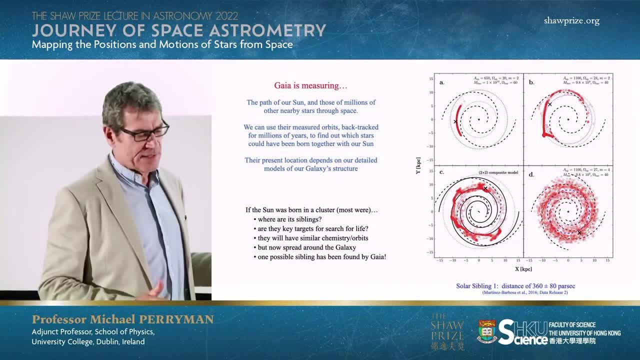 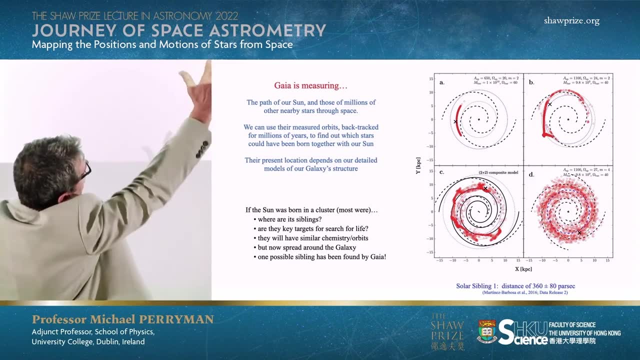 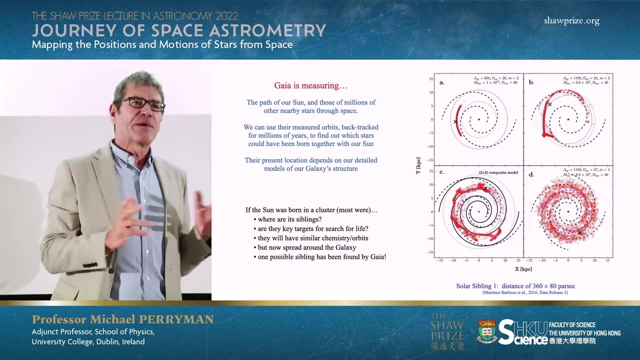 very, very similar to the orbit of our own sun around the galaxy, And what some groups are now doing is trying to develop different models. These are four different models: looking down on the face of our galaxy and trying to figure out where these stars that could have been formed. 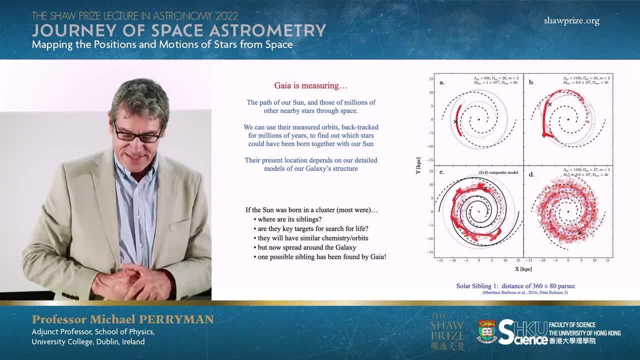 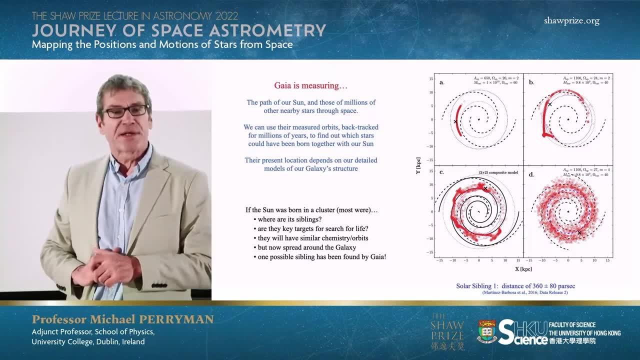 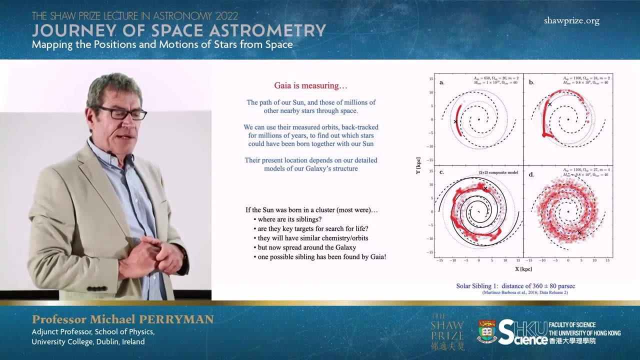 in the same nursery as our sun. where are they now, And with some success? the first of these candidates- Solar Sibling 1, was announced five years ago already. And the interesting thing is that not only these objects share the same dynamical. 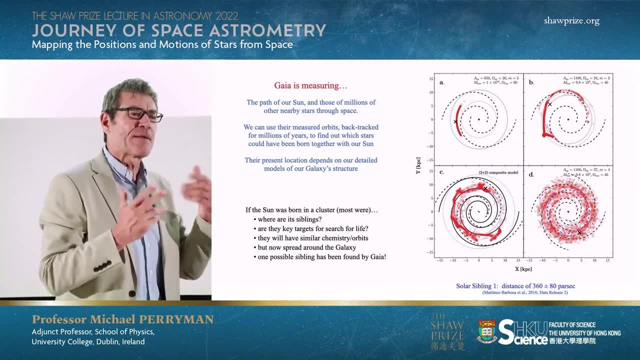 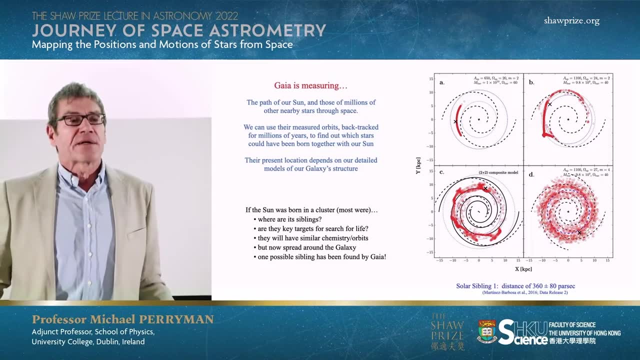 motion as our sun around the galaxy, but they have a very similar chemical composition. So people are starting to look at these stars they're about. this one is about a thousand light years away from us, but they're probably formed in the same stellar cloud. 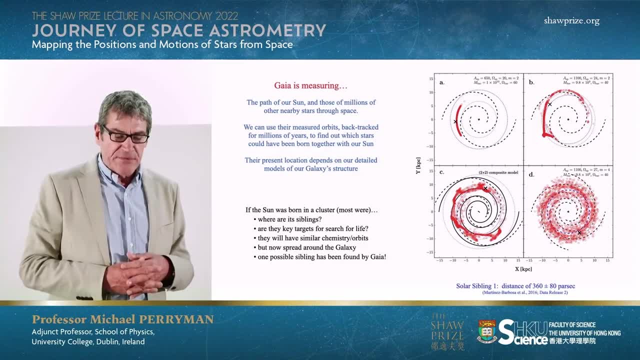 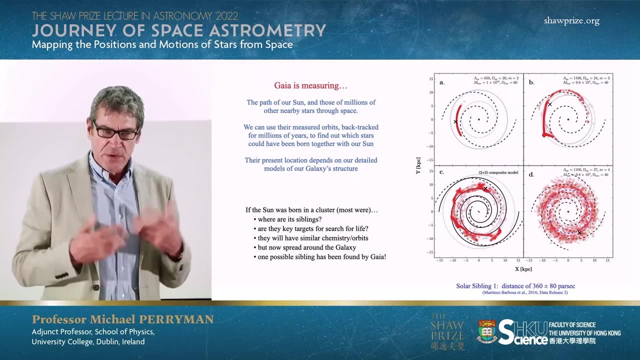 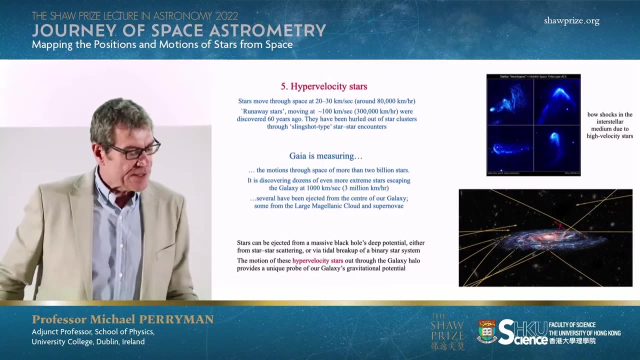 And the idea is, perhaps there are signs of life in these stellar systems that life formed at a similar time, in a similar way to life in our own solar system. So this is the search for solar siblings. Our next example: hypervelocity stars. Stars move through space at about 20 kilometers per second. 20 kilometers per second doesn't sound too much, but that's 80,000 kilometers an hour. There are stars that have been known for 50 or 60 years, that move at even. 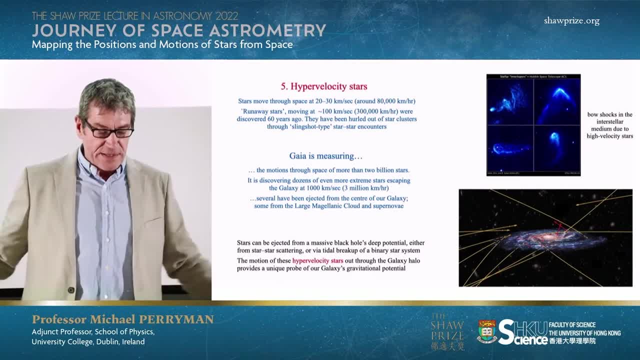 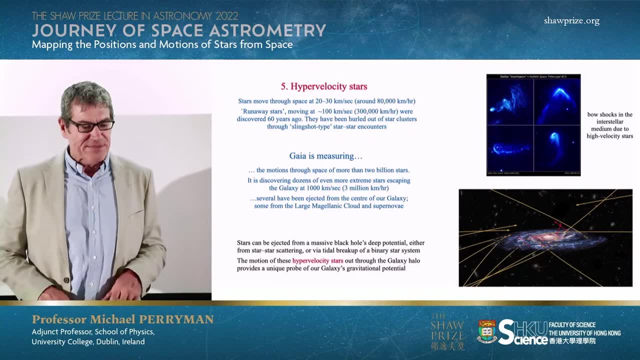 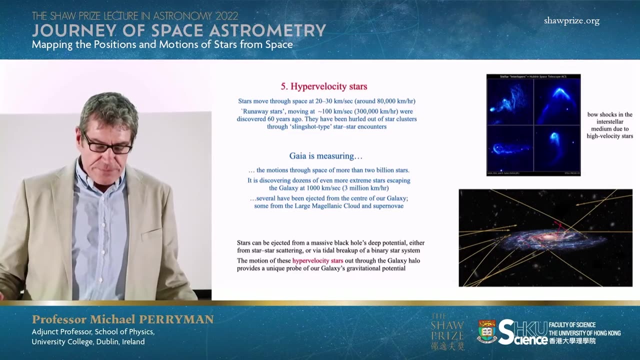 greater speeds: 100 kilometers per second. runaway stars, 300,000 kilometers per hour. In the last few years, even faster stars have been discovered, hypervelocity stars. The first was discovered before Gaia, but Gaia is discovering many more of them. 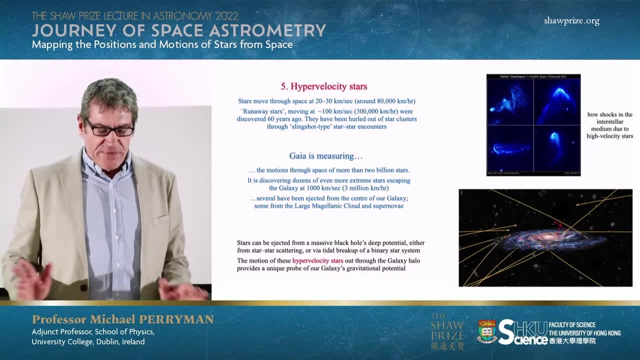 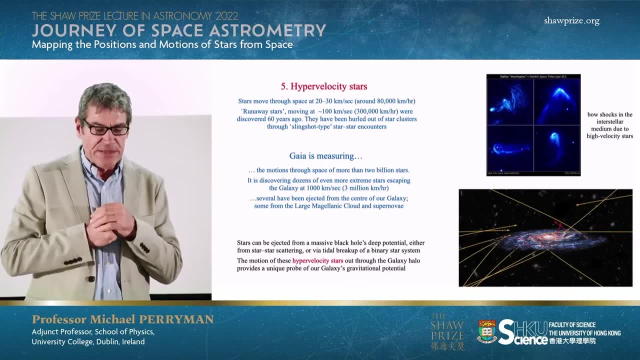 And the interesting thing is that it's being able to show where these stars are coming from. We can measure their distances and we can measure their velocity through space and we can trace back where they're coming from. And it does seem that most of these hypervelocity. 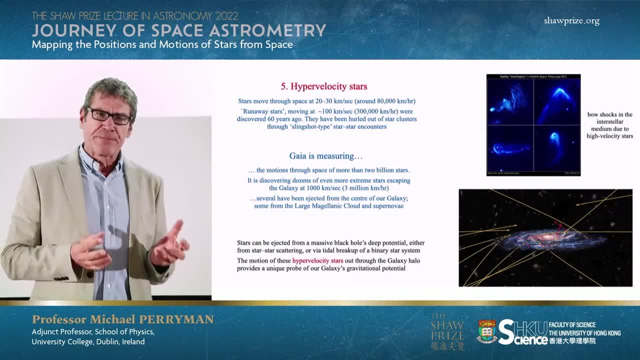 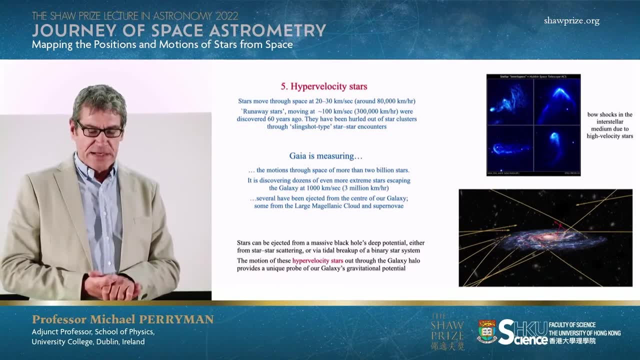 stars are coming from the center of our galaxy, and theoreticians have been busy working on this, figuring out that disruption of stellar systems in the vicinity of the black hole at the center of our galaxy can tear binary systems apart and eject them at very high velocities through space. 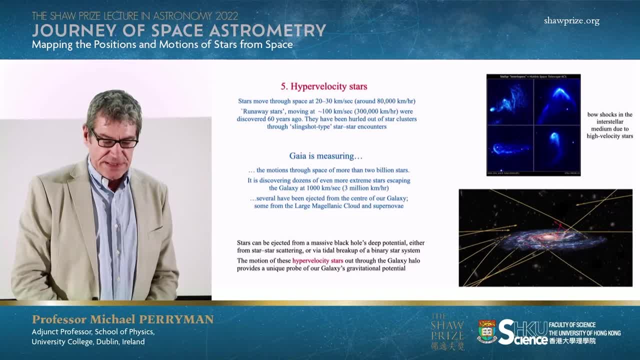 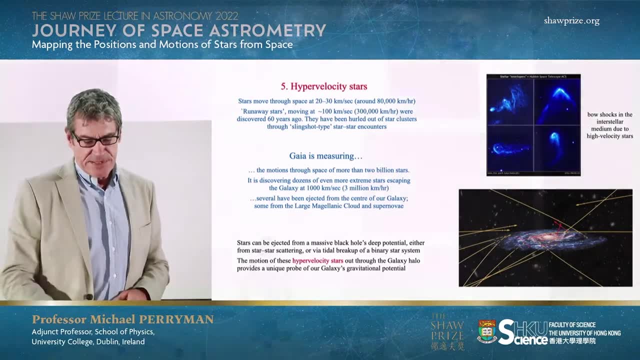 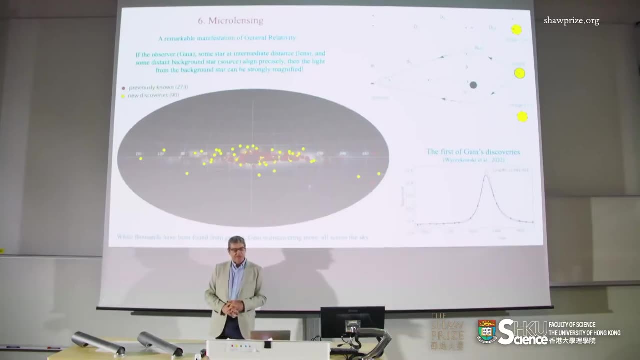 Again, there are very interesting applications of these, figuring out the mass of our own galaxy and figuring out the halo properties of our galaxy. My penultimate example: microlensing, a very bizarre manifestation of general relativity If you have a star. 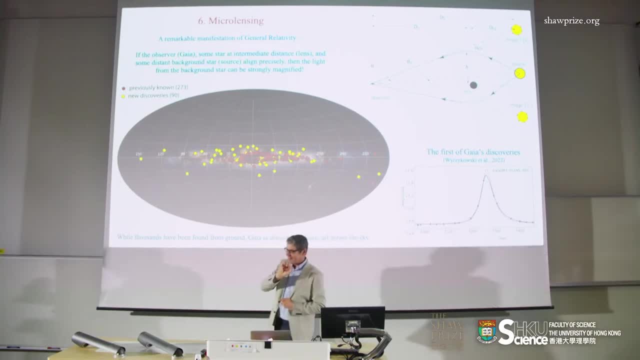 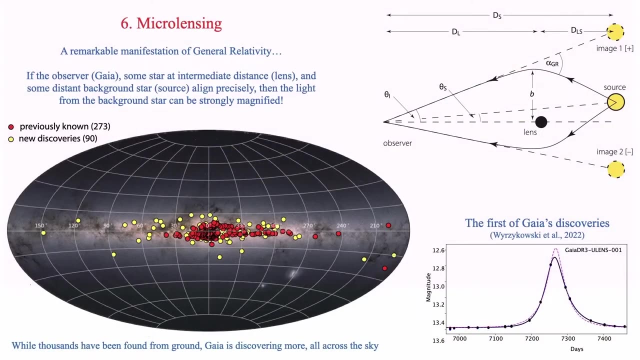 lined up with another star on the path to us as an observer. if it happens that those stars- the observer and the distant star and the foreground star- if it happens that they're lined up almost exactly, then the foreground star acts as a kind of gravitational lens. 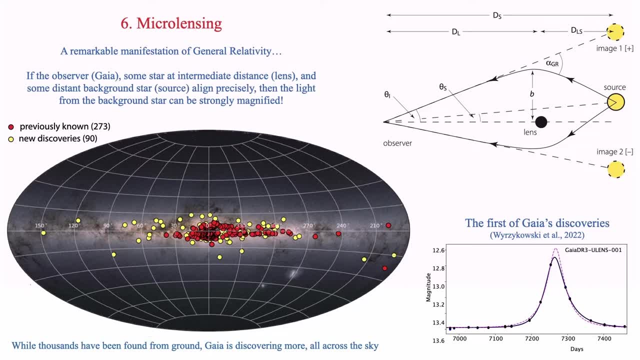 and the background star suddenly increases in brightness as it's lensed by the foreground star. Now again, this is not something that was pioneered by Gaia- not at all, and there are several thousand of these microlensing events that are known already. 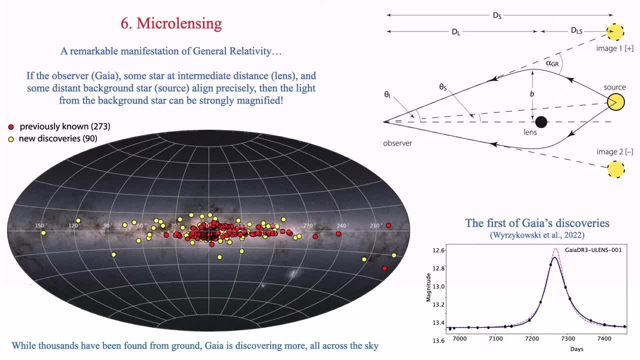 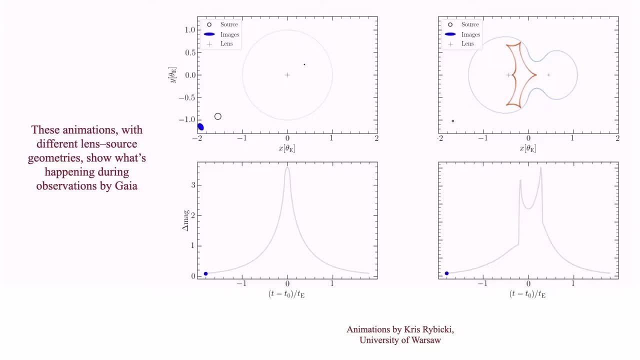 but what Gaia is doing is searching over the entire sky and it should be able to measure also the motions of the stars as they're deflected by these lenses. And in these little animations here- which I should go just very quickly, but at the bottom you can see the light. 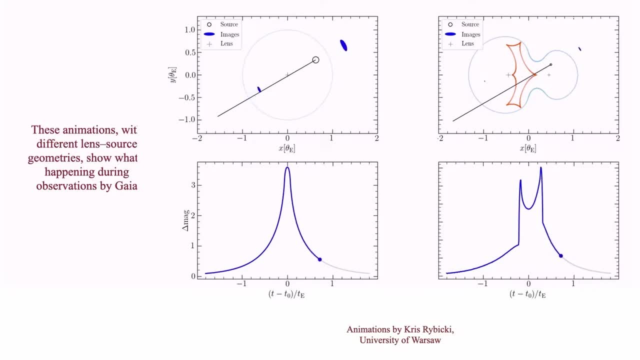 curves that result from the passage of the background star or the foreground star compared to the background star. So again, I've covered that topic very, very quickly. but it's one of the bizarre manifestations of nature, this curious alignment that can occur and give. 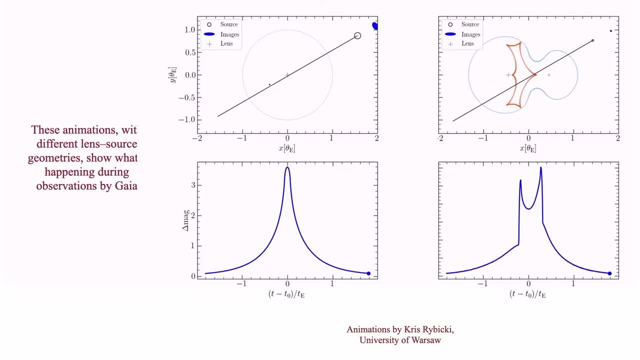 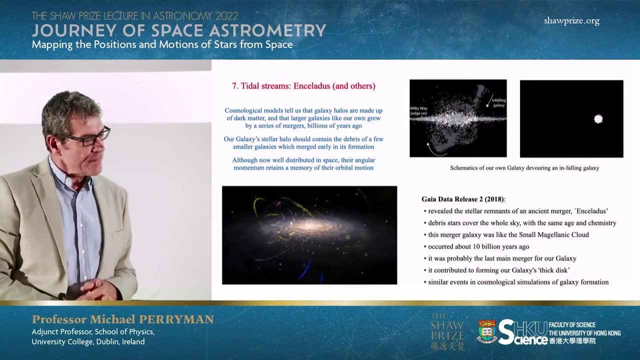 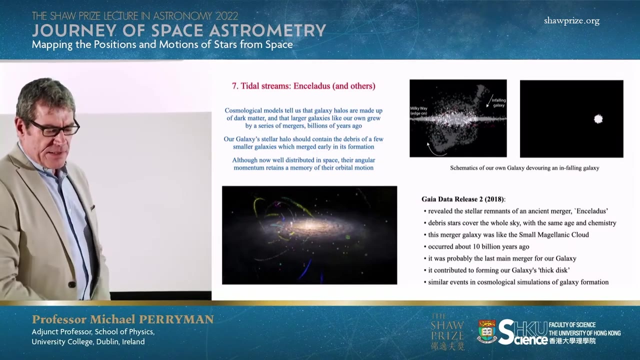 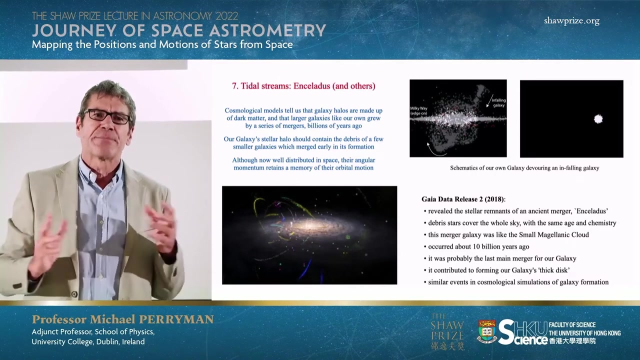 rise to observable phenomena that we can measure and disentangle a lot about the nature of these stars. My final example is on a much bigger scale. It started to become apparent perhaps 20, 30 years ago that our own galaxy formed by cannibalizing other. galaxies. Our own galaxy is quite large. When the universe was created, there were smaller galaxies there- many smaller galaxies in our local group, And the idea that cosmologists have put together in their models is that our own galaxy will have grown by devouring. 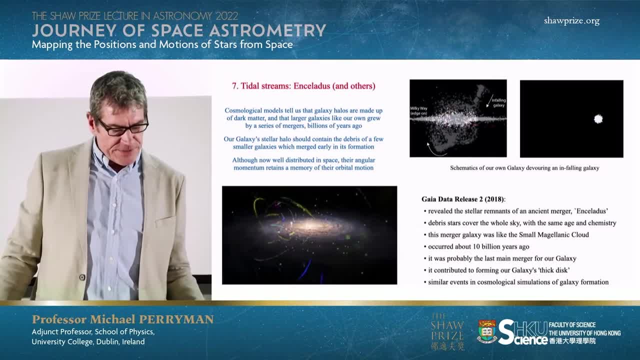 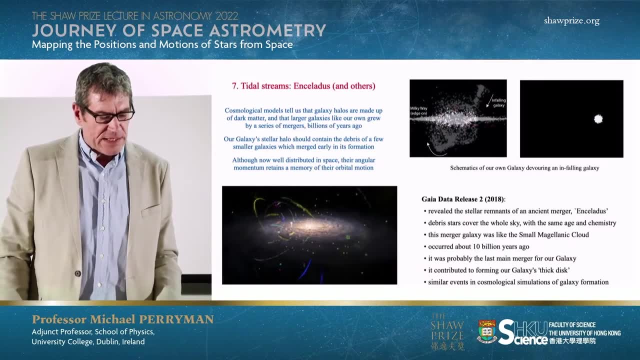 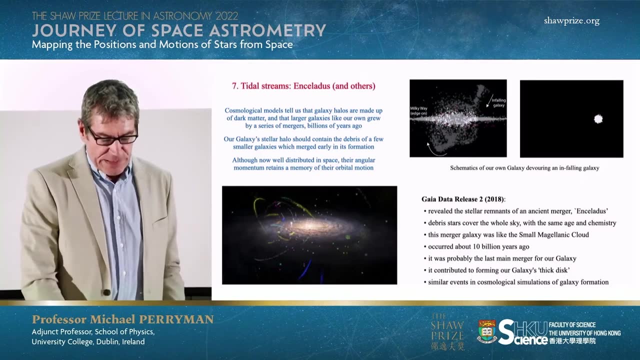 some of these smaller galaxies in the distant past. The first signs of this came already from Hipparchos, and with Gaia there are many more of these streams being discovered. The first of them is called Enceladus. It's believed to be 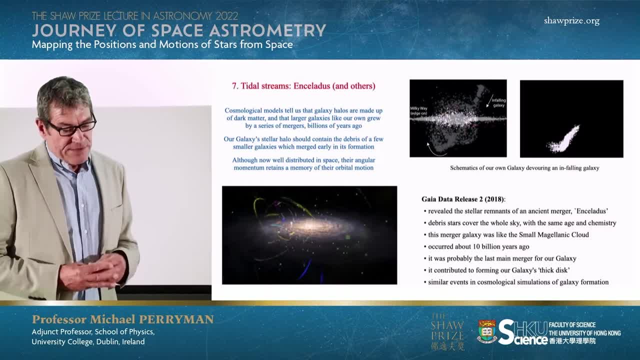 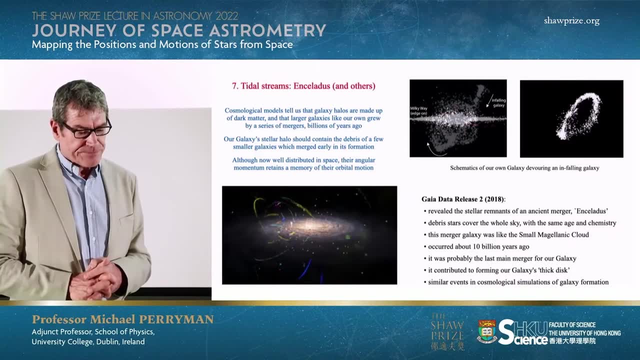 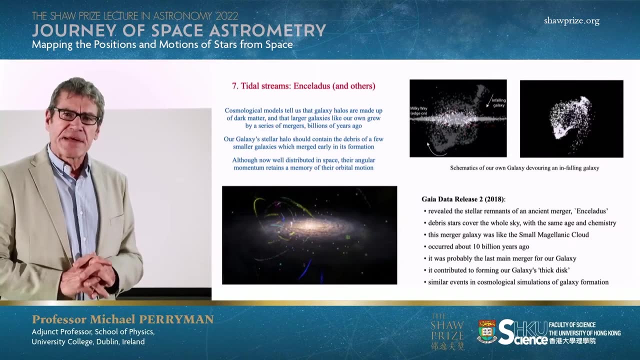 the last major merging event that took place between our galaxy and a precursor galaxy something like 10 billion years ago. And the more of these systems that we can measure, the more secure we can be about piecing together the history of the formation of our own galaxy. 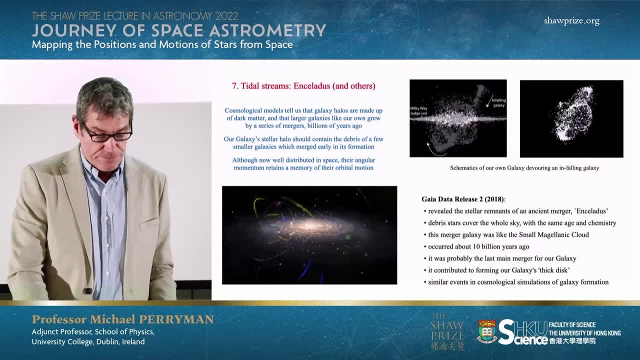 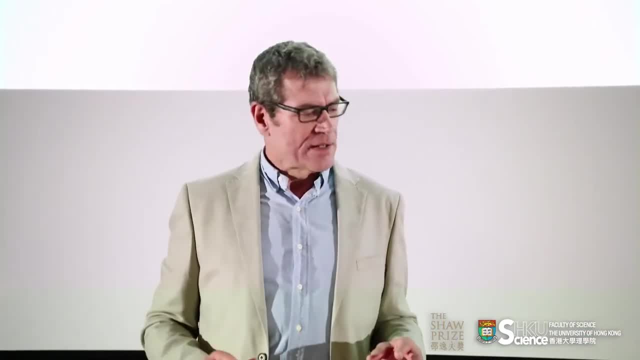 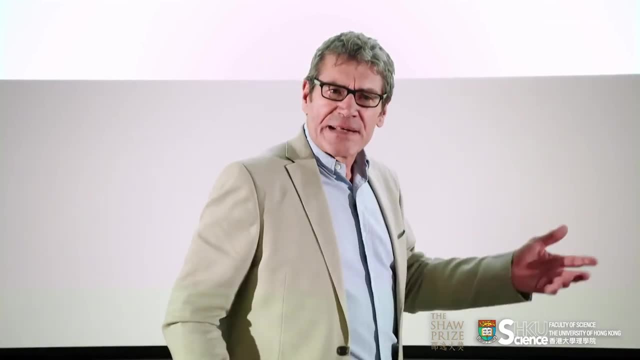 and the history of the evolution of our universe as a whole. So these are really just a few quick, short examples. I've gone over them far too quickly for you to be able to understand many of the details, but I hope this is just this little snapshot. 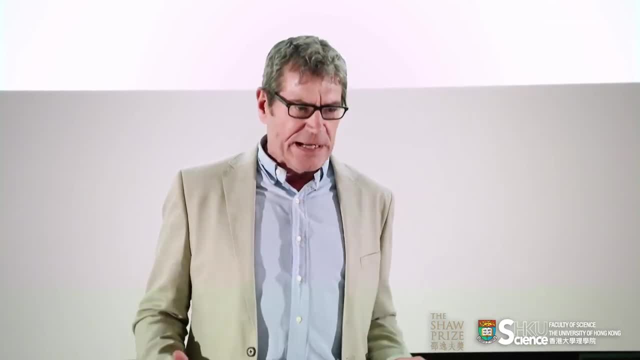 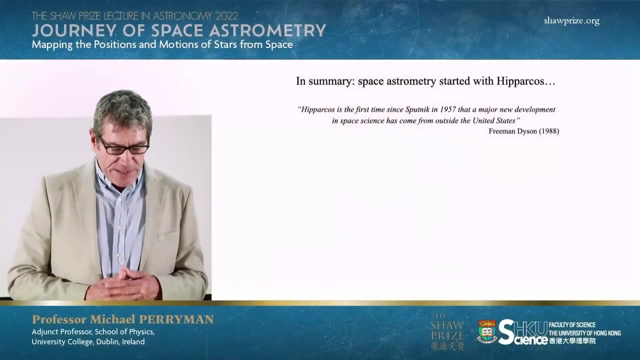 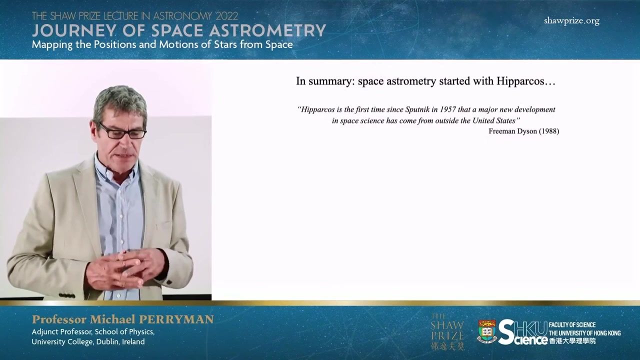 is giving you a clearer picture of some of the science that is going to come out of an advanced technological mission like this. In my summary, then, I'll say space astrometry- measuring the positions of the stars. Space astrometry started with Hipparchos. 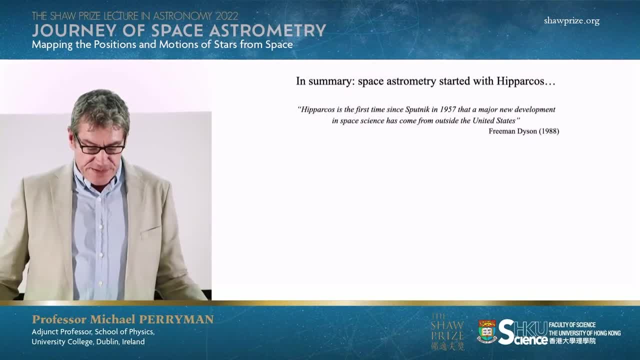 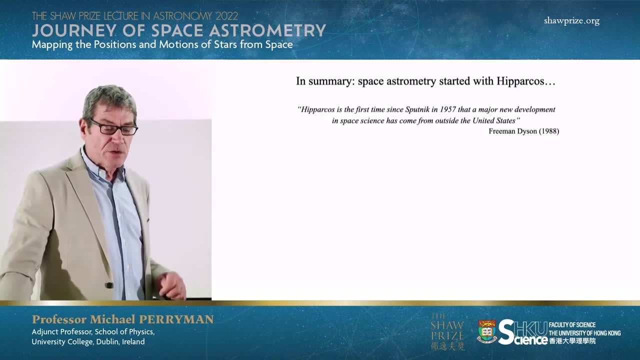 with the European Space Agency and in fact a very eminent physicist, Freeman Dyson, wrote in 1988 that Hipparchos was the first time since Sputnik in 1957 that a major new development in space science has come from outside the United States. 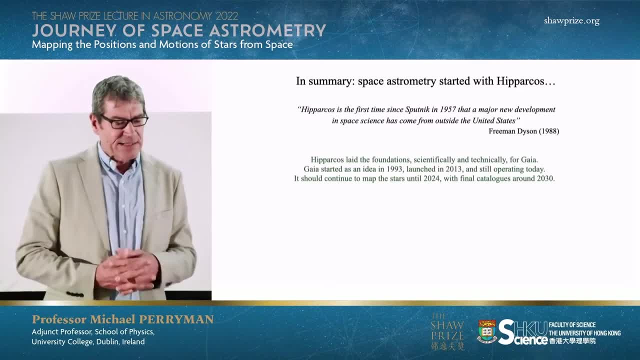 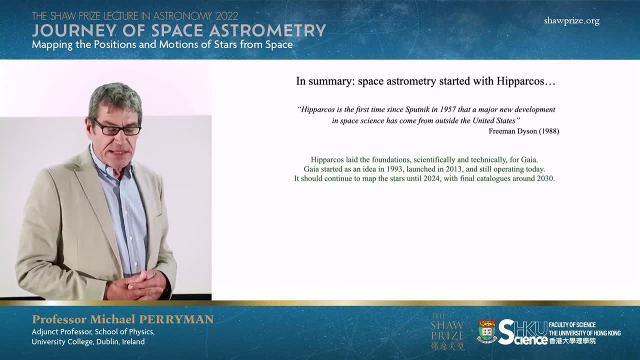 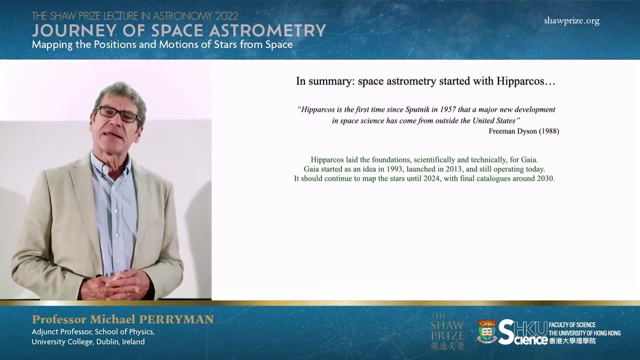 Hipparchos really laid the foundations, scientifically and technically, for Gaia. Gaia started as an idea back in 1993, it was launched in 2013, it's still operating today and it should continue to map the stars until 2024 or thereabouts, with final catalogues. 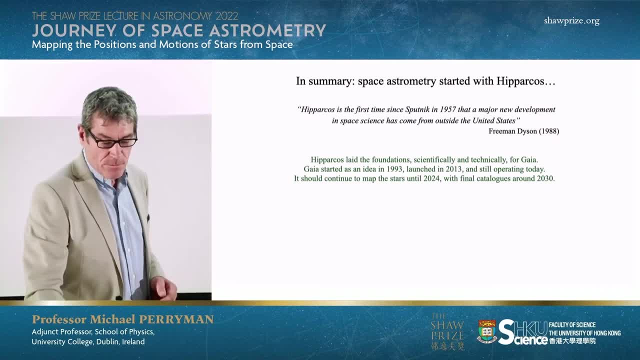 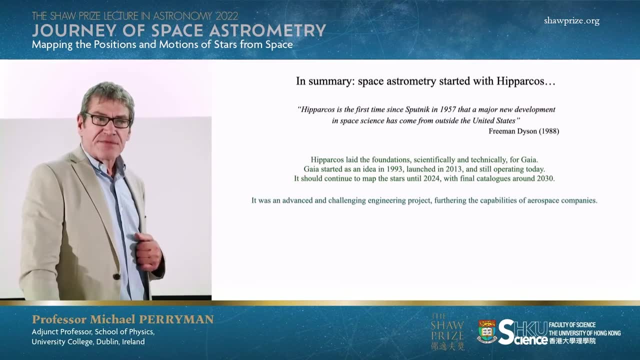 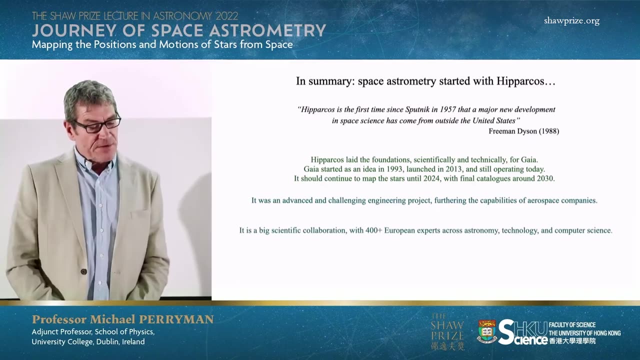 coming out in about 2030.. It was an advanced and very challenging engineering project, furthering the capabilities of aerospace companies as well as pushing forward the boundaries of science. I should stress that it's a huge scientific collaboration. there are four hundred or more. 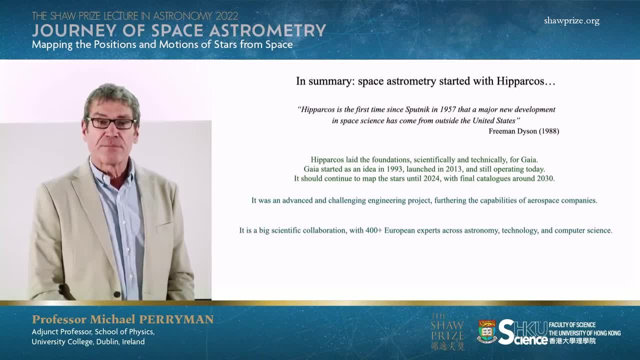 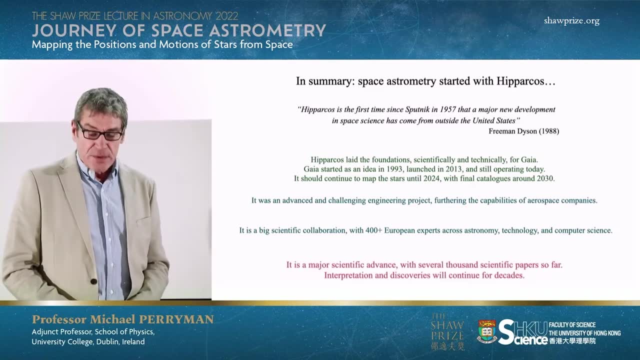 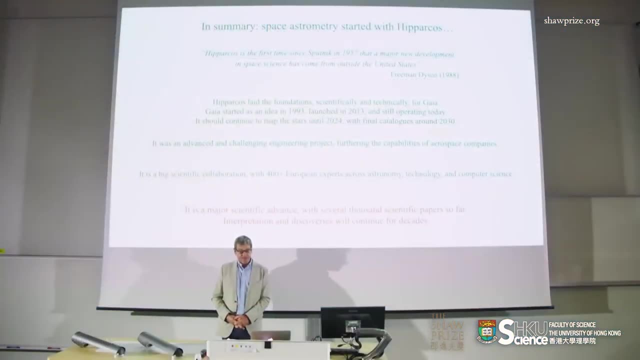 European experts across the fields of astronomy, technology and computer science working on it today. It's a major scientific advance. several thousand scientific papers have been published so far and the interpretation and discoveries will continue for decades. I'm going to play out with a video. 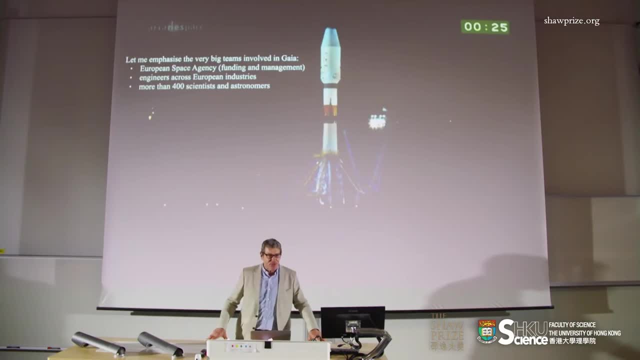 I haven't told you how Gaia works. I haven't told you the great challenges in building it. I haven't told you how the data is analysed on the ground. I've just given you this snapshot of what it is we're trying to achieve scientifically. but 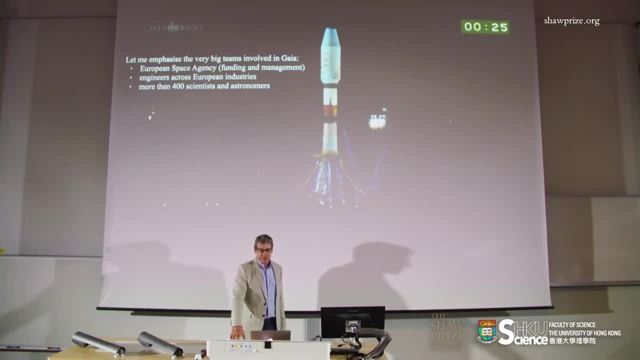 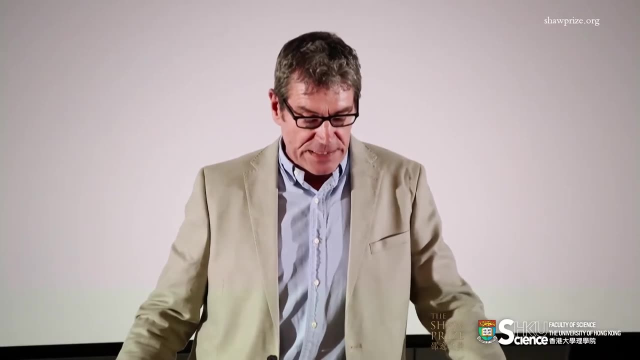 let me just show you the launch of this, a very spectacular event in December 2013, and as I play it out, let me emphasise again that very big teams are involved in these space missions like Gaia, and one must credit the European Space Agency. 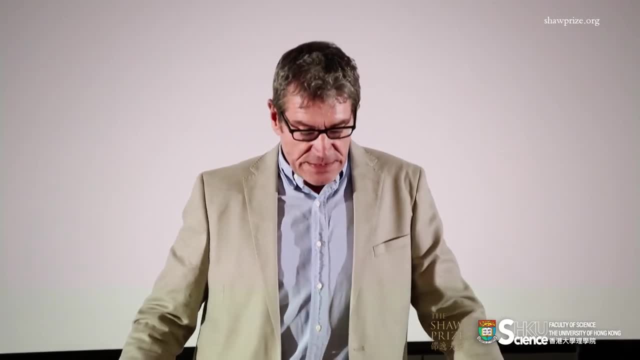 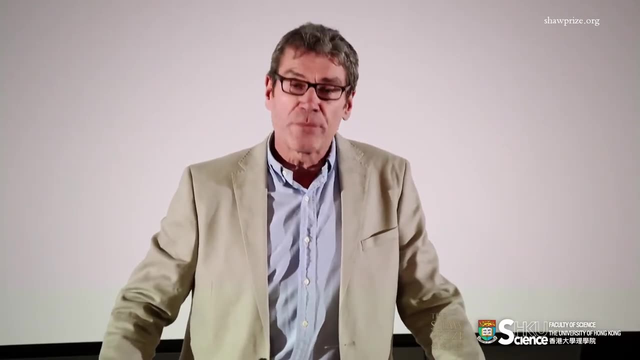 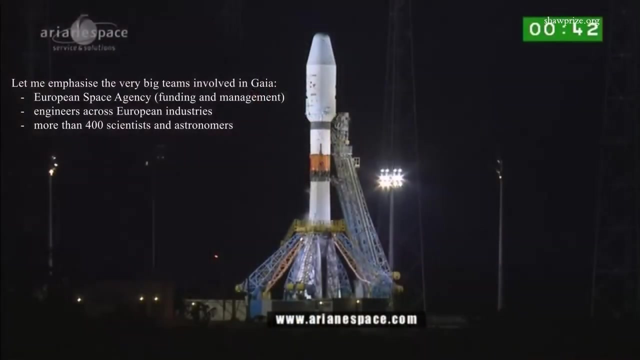 for the funding, the management, the innovation and the initial acceptance of these ideas. Tremendously skilled engineers across European space industries that are able to put these kind of missions together and, as I said, more than 400 scientists and astronomers throughout Europe working on the data. 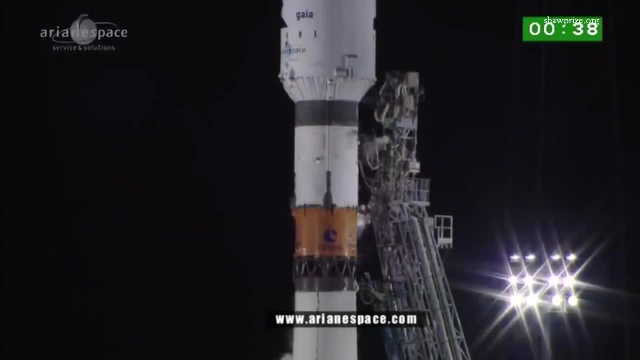 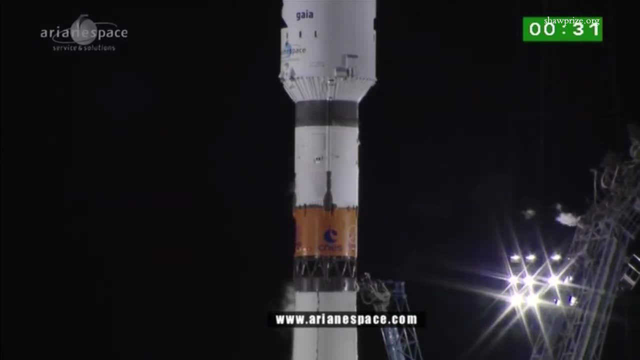 The ignition sequence is in three stages. part of it is a sequence from minus 17 seconds down to minus 6 seconds, during which the engines are tested. there are the arms rolling away. that's one of the final moments. at minus 15 seconds is the first controlled. 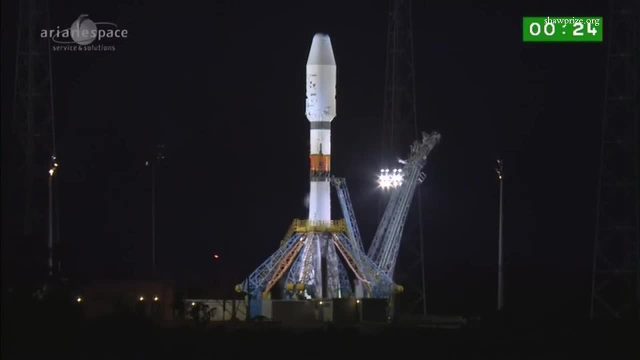 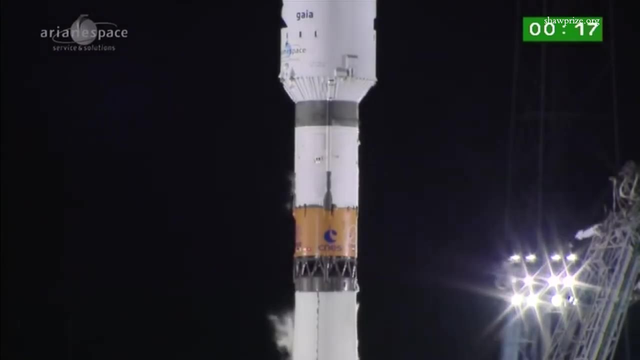 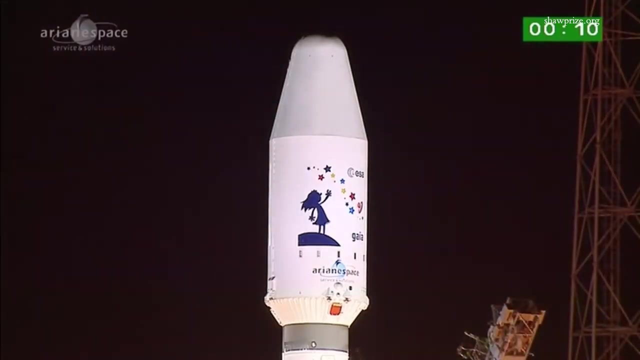 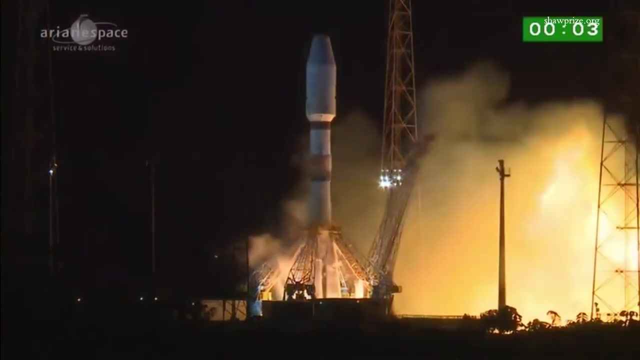 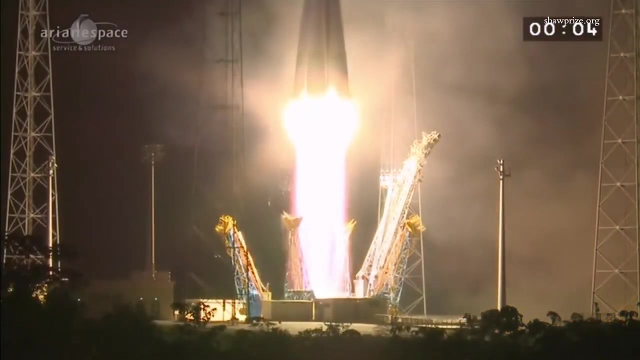 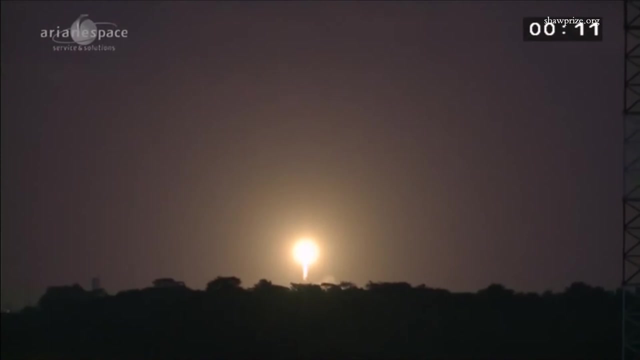 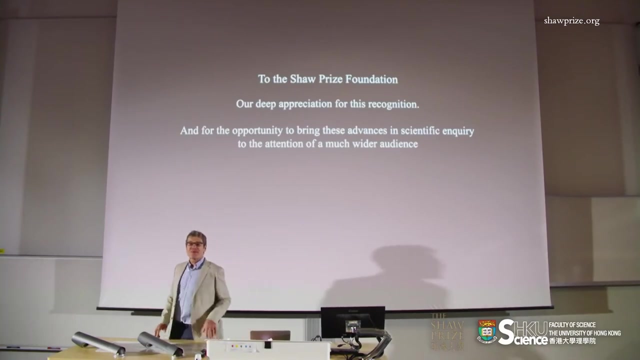 ignition at minus 7 seconds is another one at about half pressure and then at minus 3 seconds the order is given for the third and final phase. there's the gantry arms going back and forth. it's still very emotional watching that launch, knowing that. 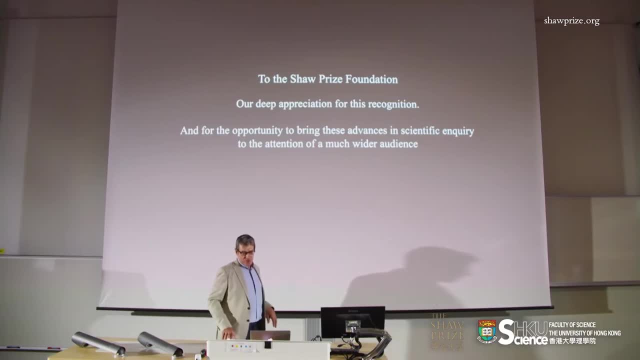 you've consigned this delicate piece of engineering to the top of these massive rockets. That brings me to the end of my presentation. may I say finally, of course to the Shaw Price Foundation, our deep gratitude and appreciation for this recognition and really for the opportunity to bring these. 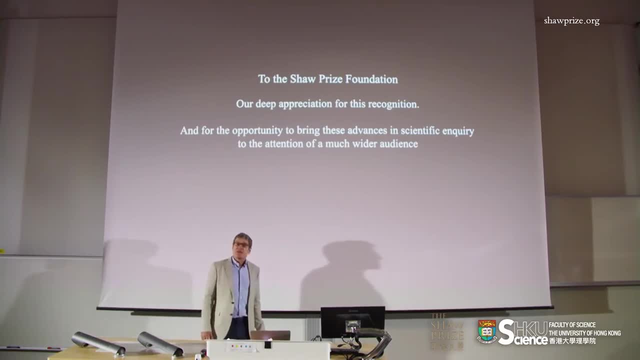 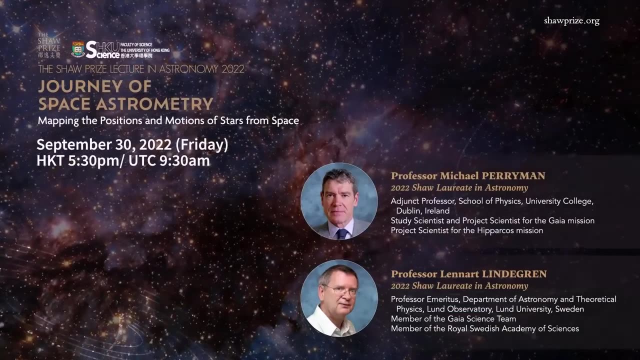 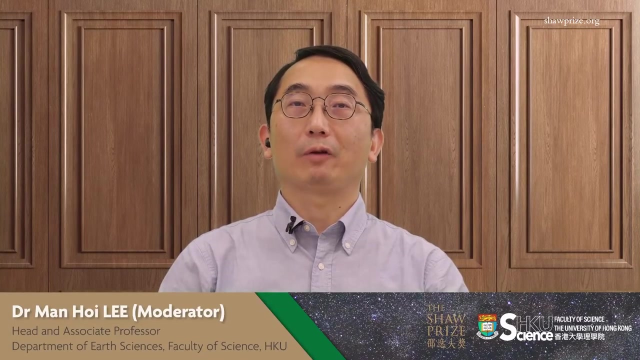 advances in scientific inquiry to the attention of a much, much wider audience. Thank you, It is a truly inspiring lecture. Thank you, Professor Perryman. Next, we are very glad to have Professor Lindegren to share his insight on fundamental concepts of global astrometry. 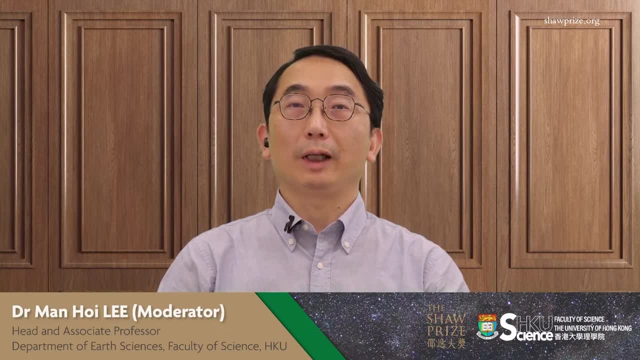 Professor Lennart Lindegren was born in 1950 in Sweden and is currently Professor Emeritus of Lund Observatory Department of Astronomy and Theoretical Physics at Lund University in Sweden. He received his PhD in 1980 from Lund University. he then joined as a member of the 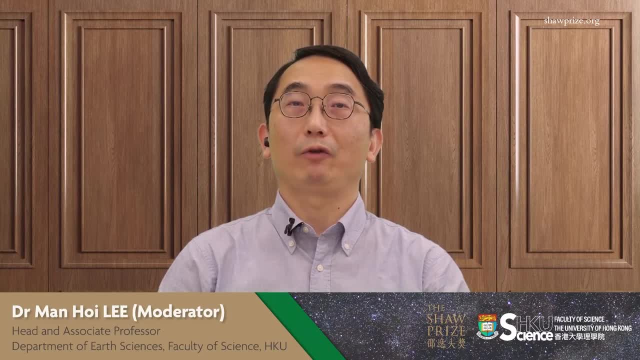 teaching staff at Lund University and became Professor of Astronomy in 2000, serving until his retirement in 2017.. During this time at Lund Observatory, Professor Lindegren had served as the director for six years. He was a member of the European Space Agency's 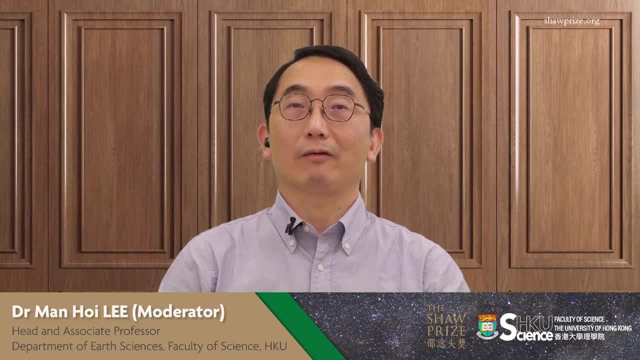 Hipparchos Science Team and Gaia Science Advisory Group. He leads the scientific implementation of the astrometric global iterative solution in the Gaia Data Processing and Analysis Consortium and is also a member of the Gaia Science Team. He also served as project coordinator. 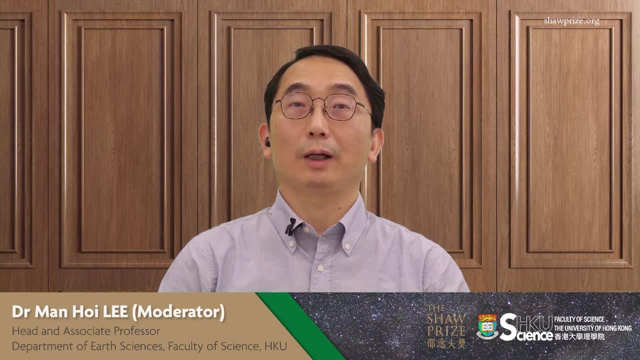 for the Marie Curie Research Training Network, ELSA. he is a member of the Royal Swedish Academy of Sciences. In the following lecture, Professor Lindegren will describe how optical observations using a scanning satellite allow us to measure accurate absolute parallaxes and proper motions. 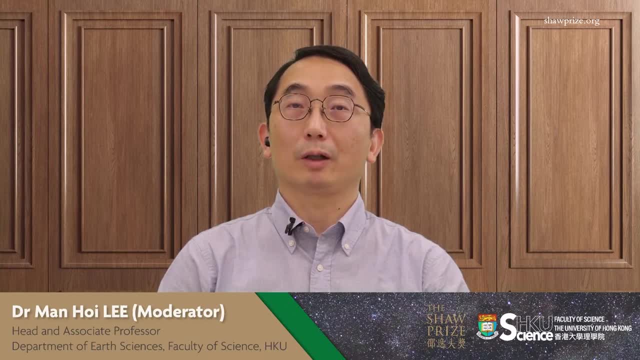 and to build a rigid reference frame over the whole celestial sphere. The principle was first applied to Hipparchos data in the 1990s, and the same principle is now used for Gaia. The intertwined measurements of all objects bring formidable data processing challenges. 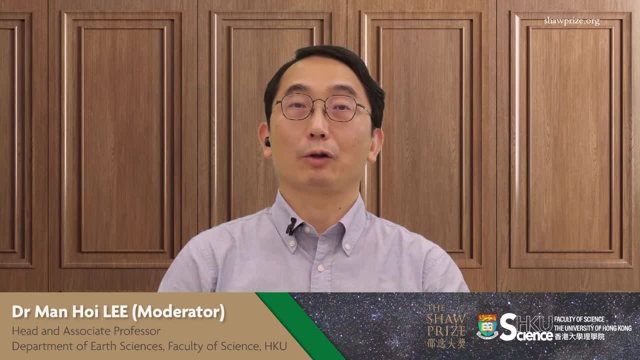 that could not be mastered for Hipparchos without certain approximations. The exponential growth in computing power since then makes it possible to treat the Gaia data much more rigorously, in spite of the immensely larger data volume. Now please join Professor Lindegren's lecture. 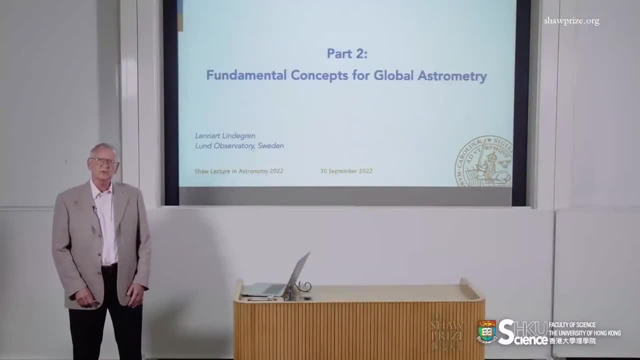 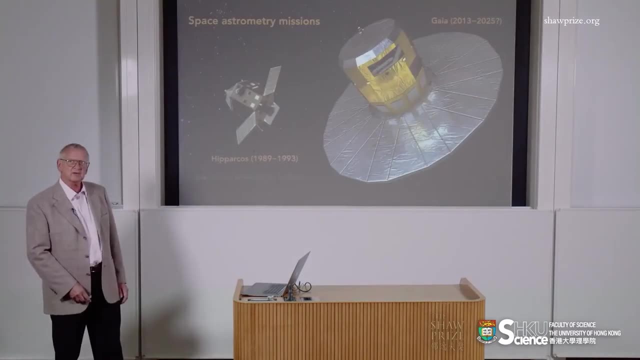 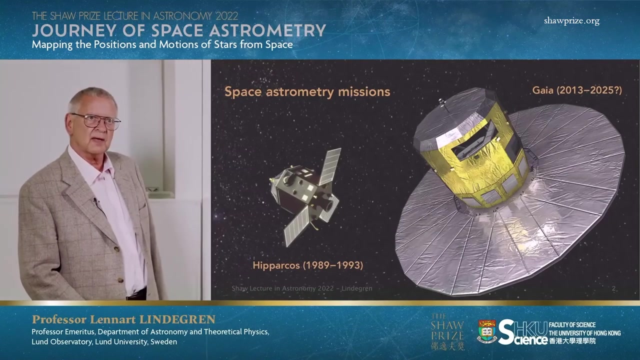 In this second part of the lecture, I want to explain some fundamental concepts underlying the two very successful space astrometry missions Hipparchos and Gaia. Hipparchos was launched in 1989 and the data came out eight years later. Gaia was launched. 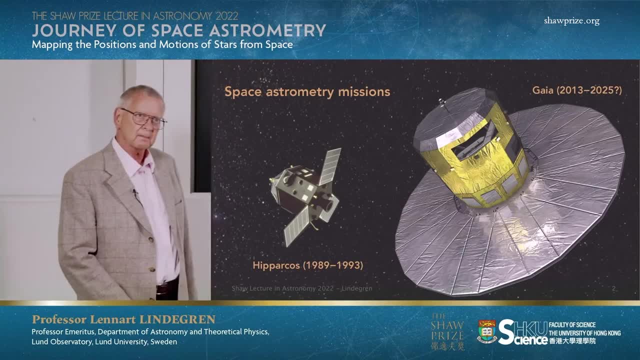 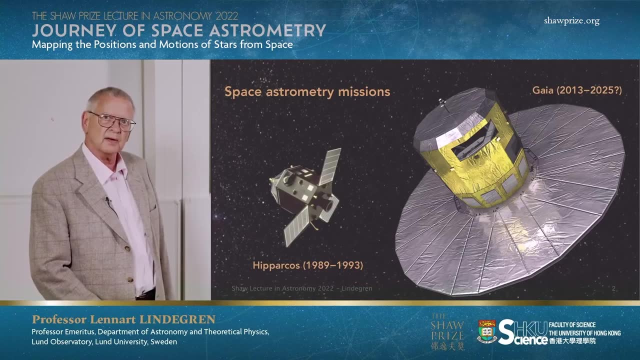 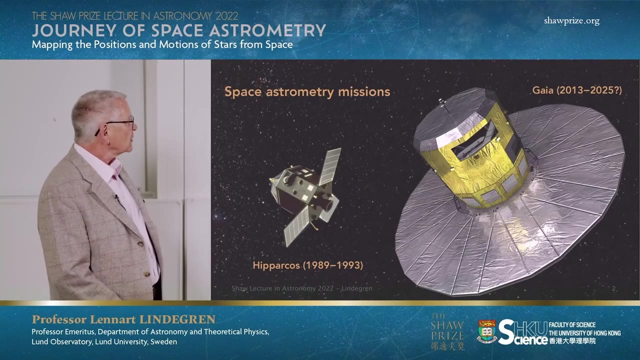 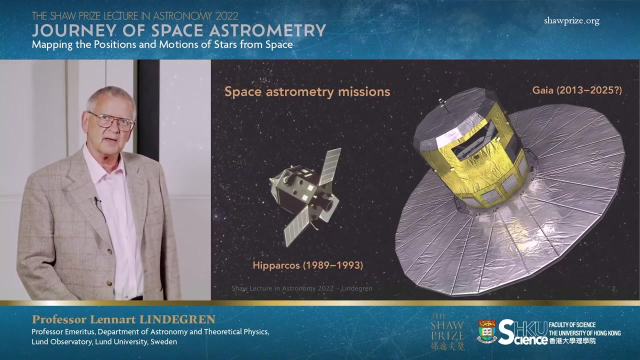 in 2013 and it is still operating. Gaia is, of course, much bigger, both in size, as shown in this drawing, and in scope and in accuracy and in almost every respect, But the two missions are actually fundamentally very similar because they are using the same principles for. 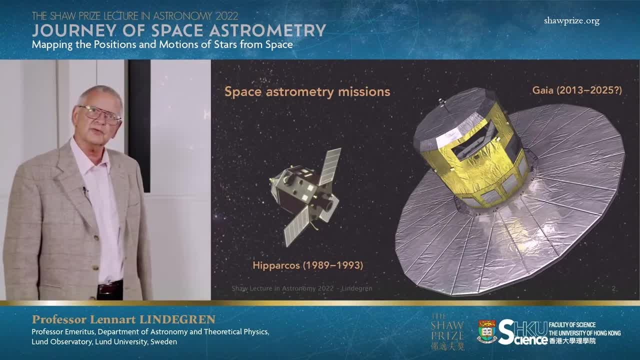 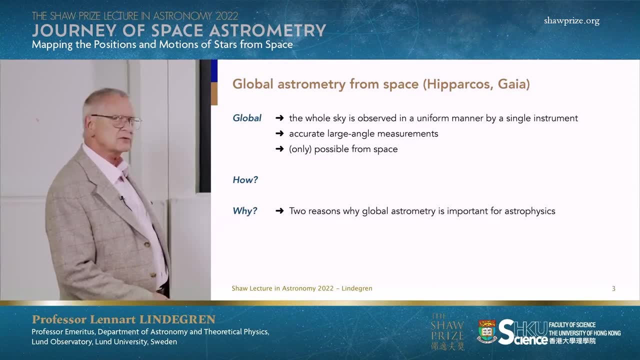 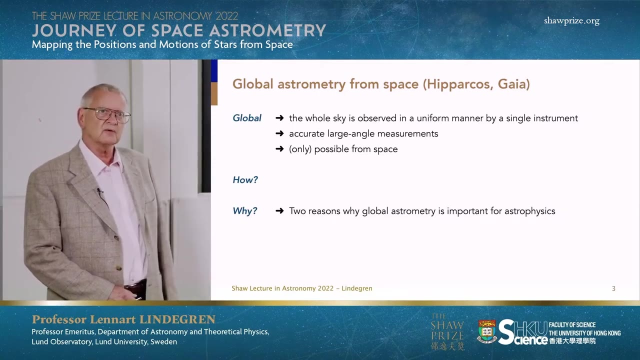 doing astrometry from space, And that is what I want to explain in this talk. I will focus on the global nature of these missions. Global means that the whole sky is observed in a uniform manner from a single instrument. This requires accurate large scale measurements. 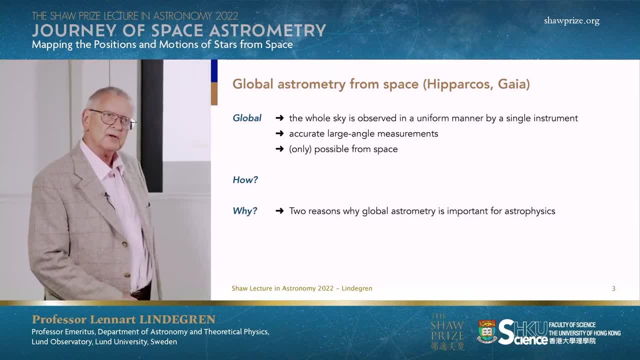 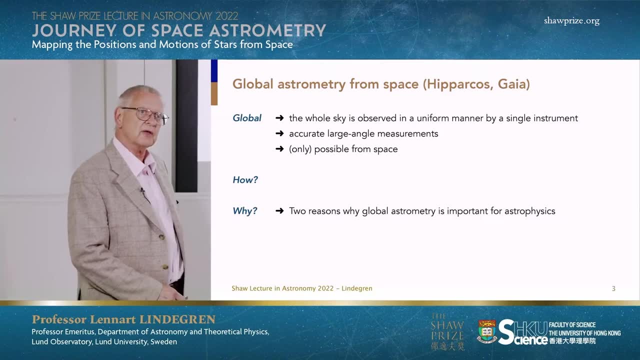 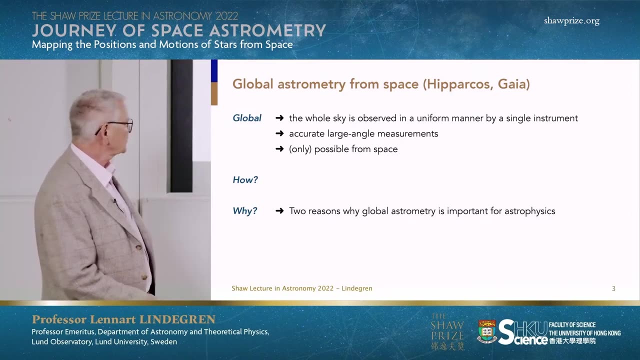 over the whole sky, Which, as we will see, is only possible from space. I will explain how this is possible, but first I will give two good reasons why such global astrometry is important in astrophysics. The first reason is that 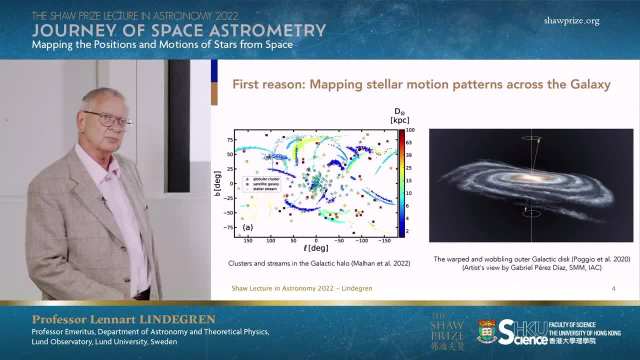 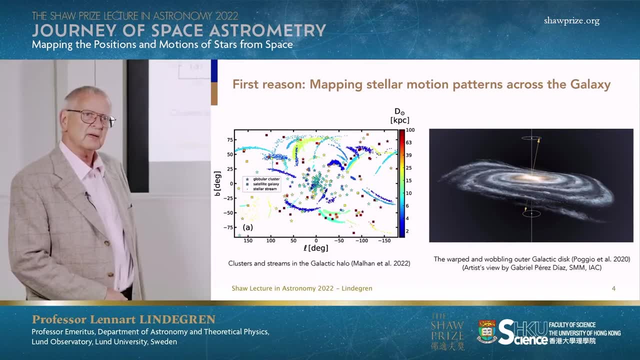 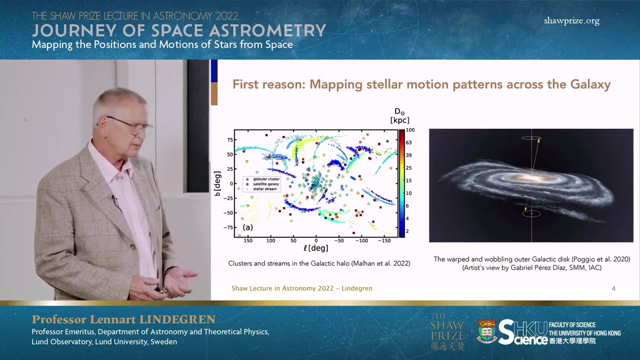 in order to understand how our galaxy is built, how it is formed and how it works, we need to map stellar motions across the whole galaxy, And because we are sitting inside the galaxy, it means we have to measure these motions across the whole sky. That means global astrometry. 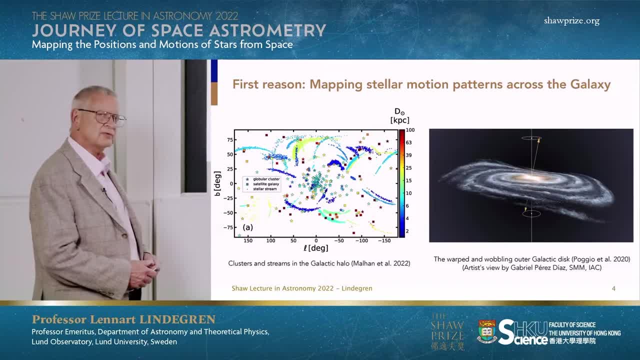 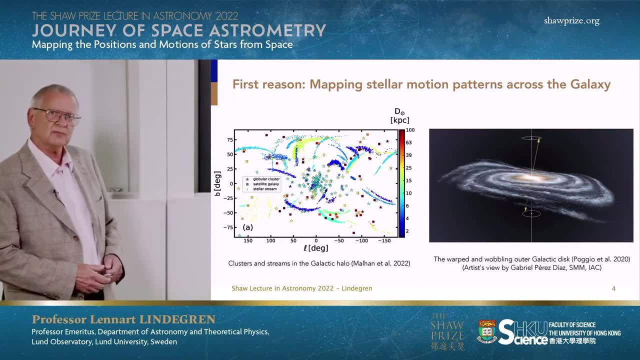 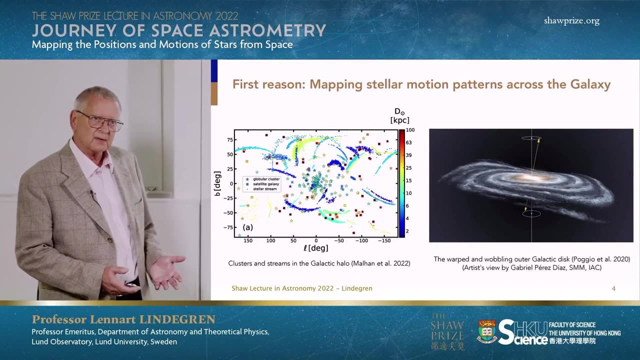 These diagrams show two examples of why we want to map these global patterns. In the left diagram we have the clusters and streams in the outer part of the galaxy, the halo, which tell us a lot about our galaxy. They make it possible to weigh the galaxy. 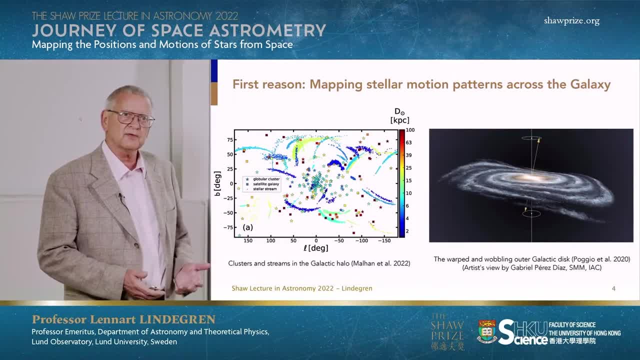 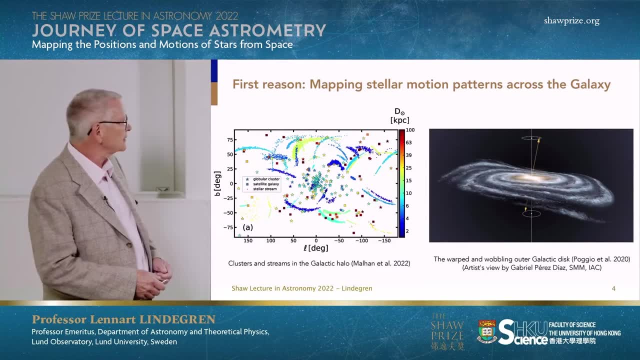 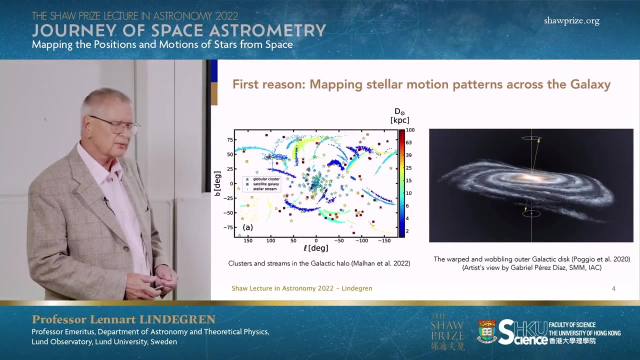 and tell us how much dark matter there is, for example, But they also tell us how much light there is. The drawing to the right is illustrated that our galaxy is not just a flat rotating disk. This disk is warped and it is processing in a complicated way. 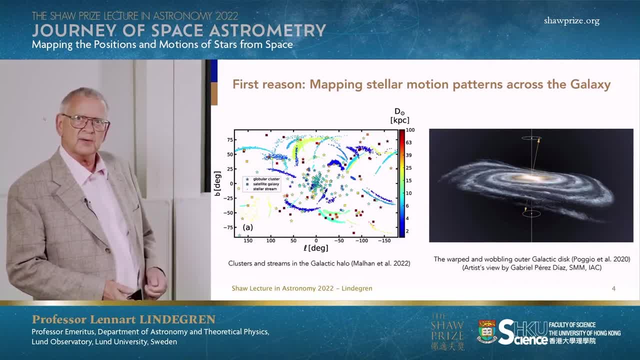 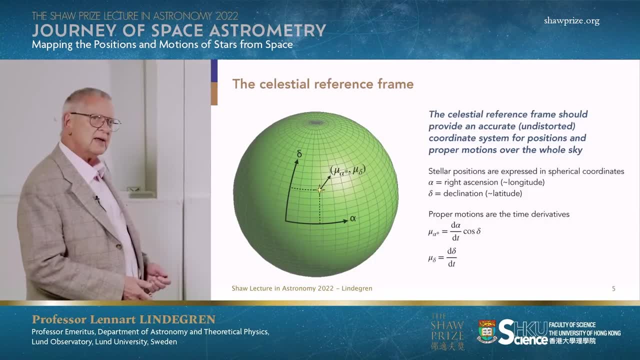 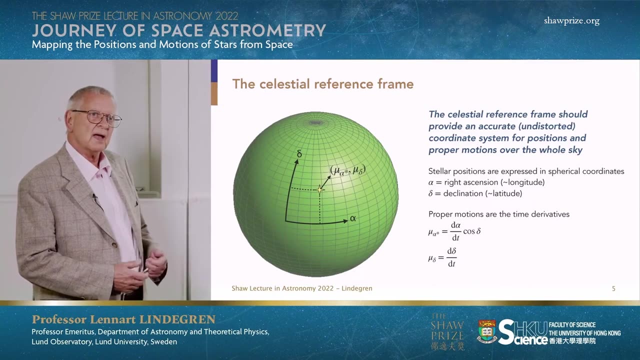 much like a spinning top, And this again tells us something about the dynamical history of the galaxy. In more technical terms, what we need is a celestial system that is very accurate, which means has no distortions, So it provides a coordinate system for positions and 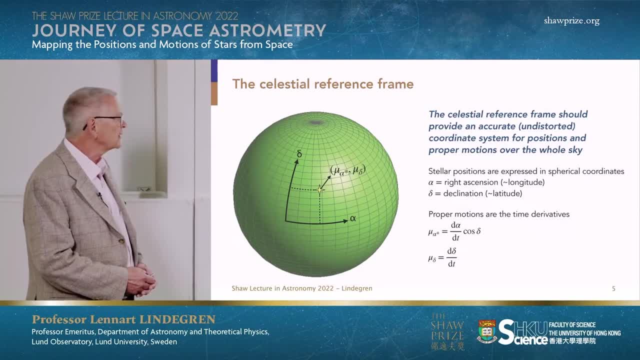 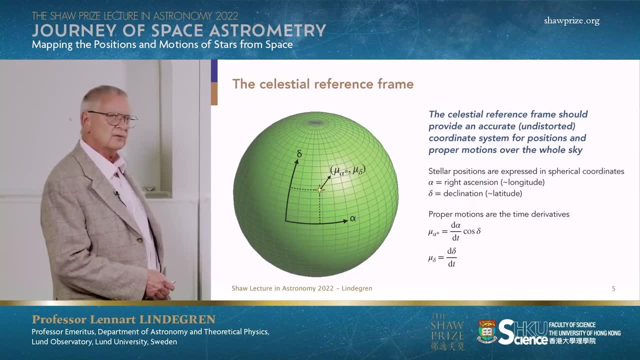 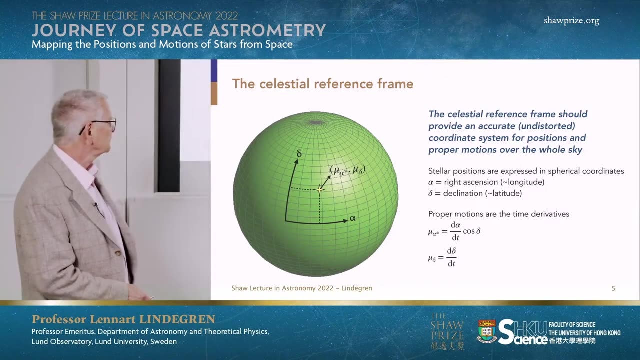 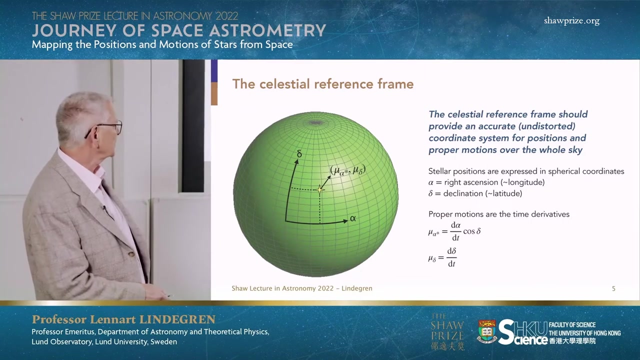 proper motions over the whole sky. Stellar positions are normally expressed in spherical coordinates called right ascension and declination and denoted with the Greek letters alpha and delta. Proper motions are the time derivatives. of these derivatives And we know very slowly that there is seldom any. 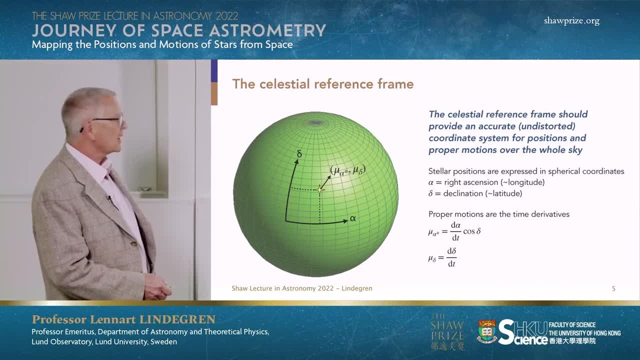 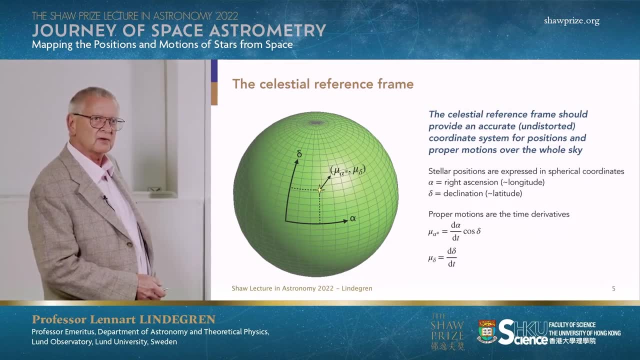 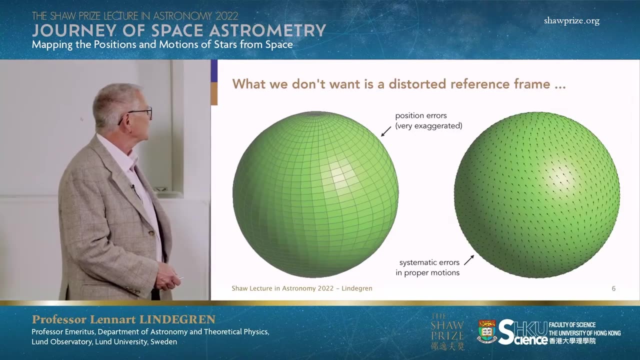 reason to use higher derivatives than the first derivative. The proper motions can be visualized as vectors on the celestial sphere showing the motion of stars perpendicular to the line of sight. What we don't want is a distorted reference frame, that is, that the positions of the 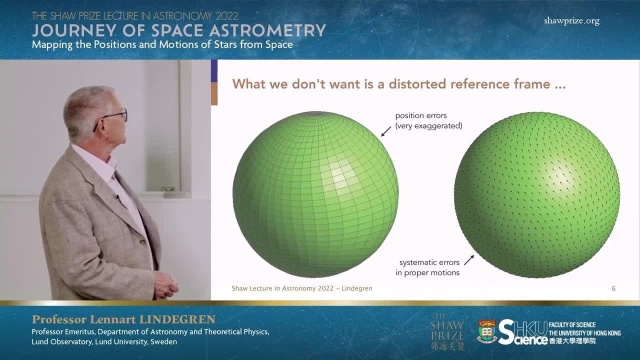 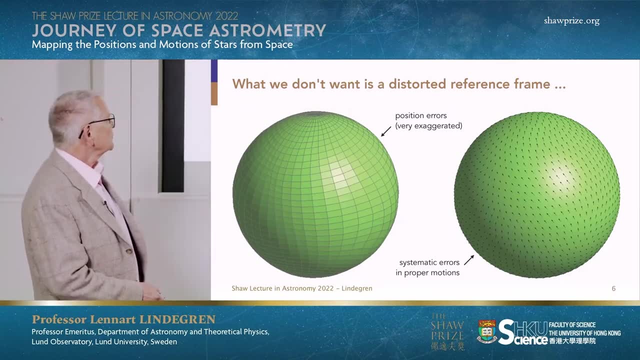 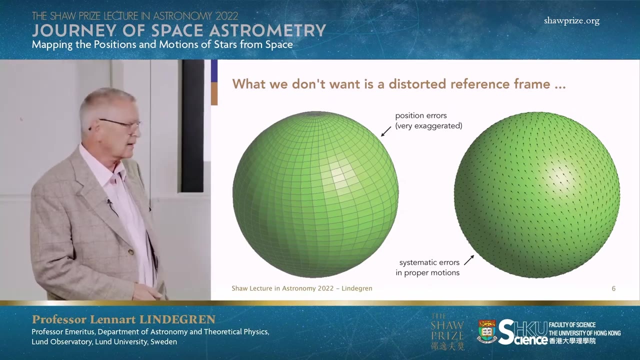 stars are not a regular grid on the sky, but a distorted pattern, like illustrated in the left figure, And similarly the proper motions should be undistorted, which means that they don't make large scale patterns in their eras. But that is not what we have. 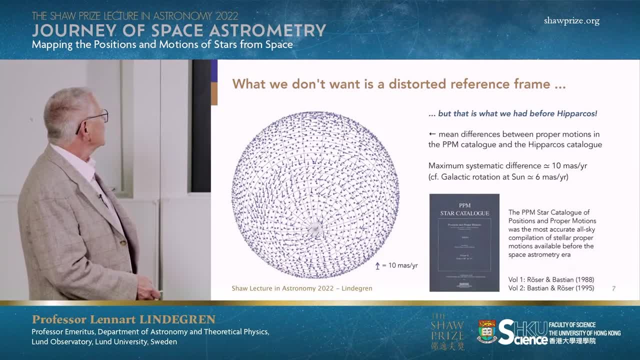 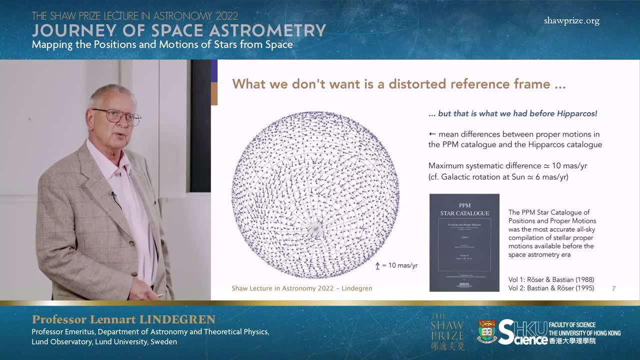 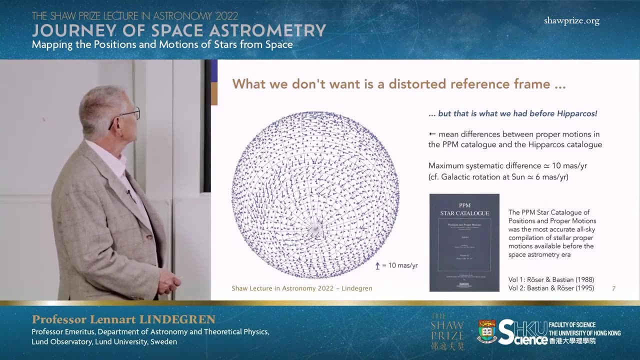 in the data before Hipparchus. This diagram here shows the errors in proper motions in the best compilation of stellar proper motions before Hipparchus, the PPM catalog. What you can see from this vector plot is that in some areas of the sky the errors are rather small, but in others they are as much as 10 ms per year. This is not a big, proper motion, but it is large compared to the patterns that we want to measure, For example the galactic rotation itself around the galactic center. 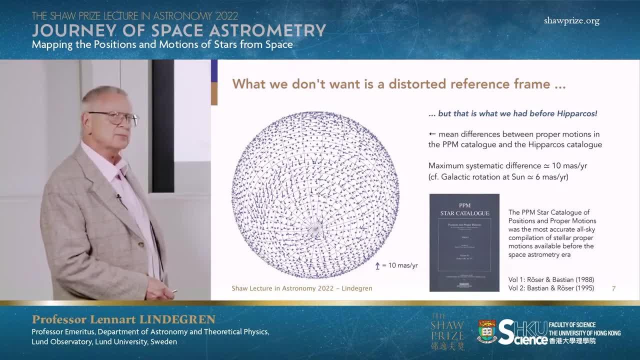 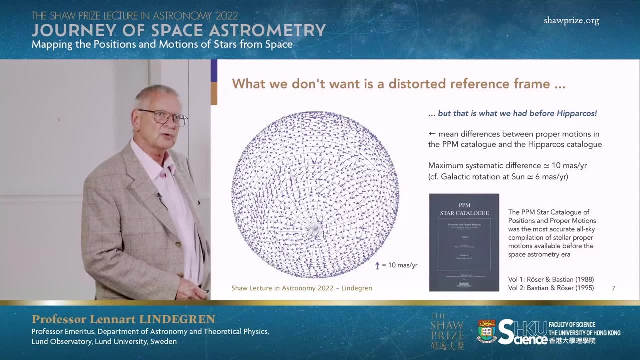 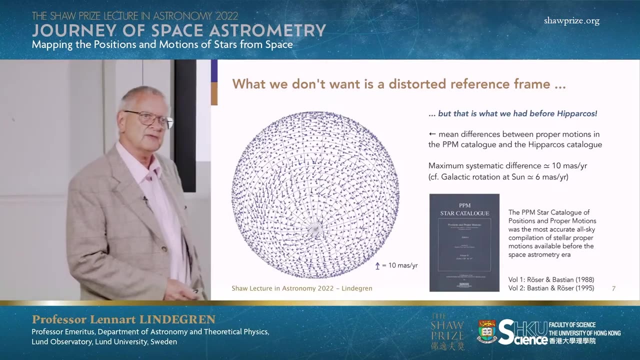 as seen from the sun is only about 6 ms per year, and it is clear that if we have this kind of systematic errors in our proper motions, we would not be able to see the much more subtle patterns corresponding to the halo streams or the processing warp I talked about before. 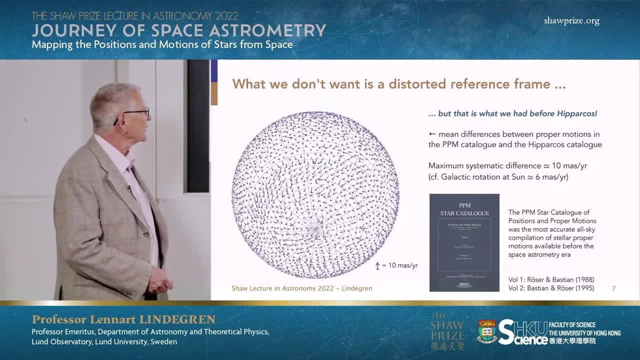 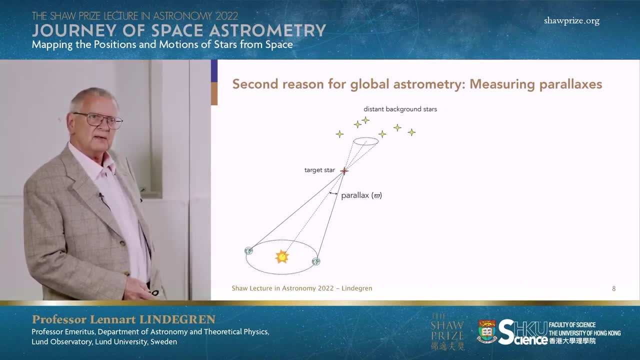 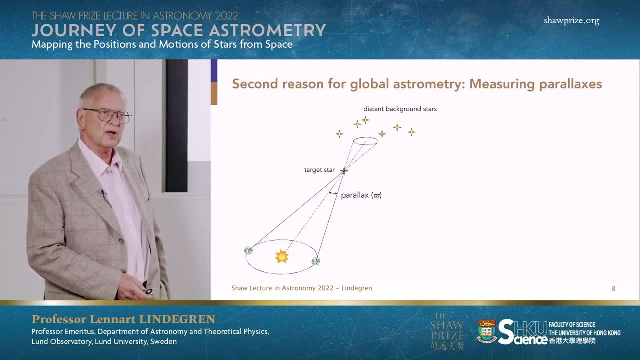 So with this kind of systematic errors in the proper motions, we could not do that kind of science. The other reason why we need global astrometry is in order to measure parallaxes. This could come as a surprise to you perhaps, since it is well known. 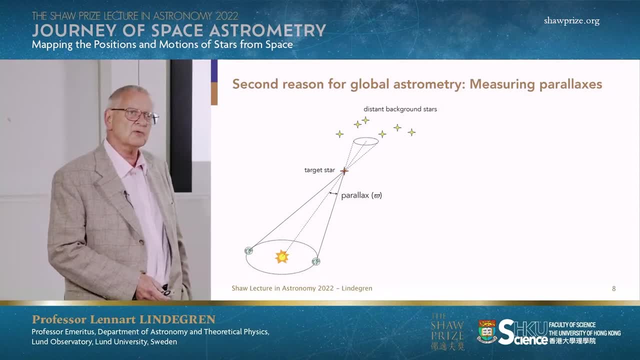 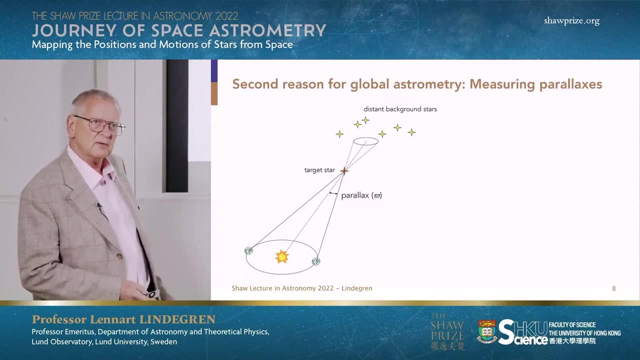 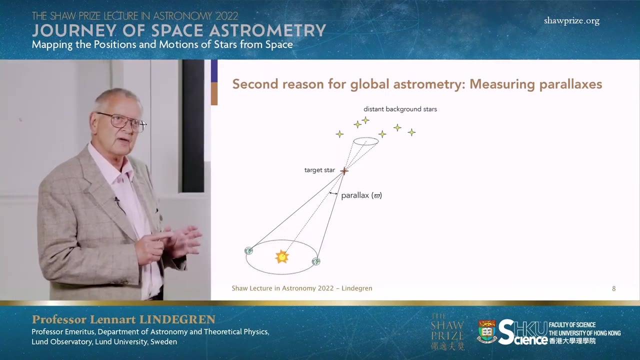 that we have been able to measure parallaxes from the ground for almost 200 years with quite a lot of success, But these parallaxes were always measured within the field of view of a big telescope, which means that we only measured angles between stars. 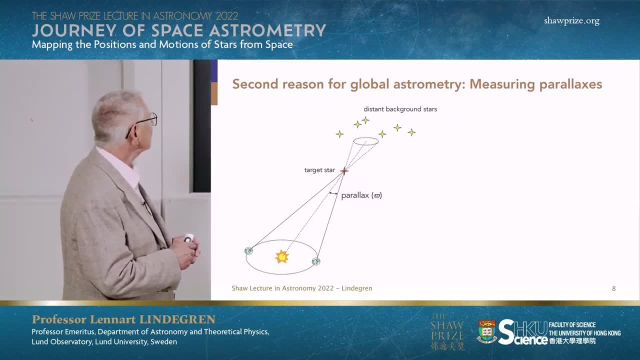 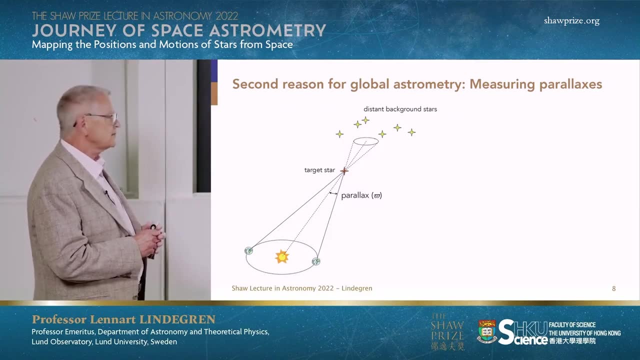 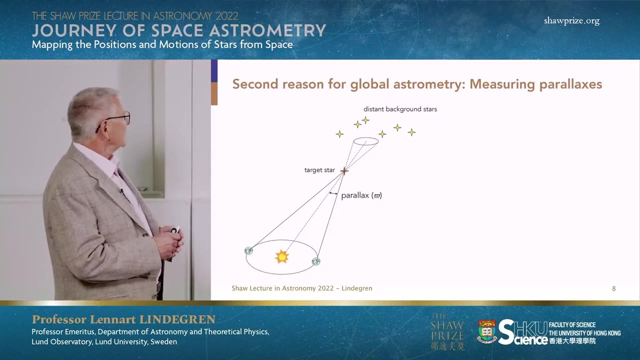 that were very close to each other on the sky, Parallax is usually described by means of a diagram like that to the left. So as the earth moves around the sun over the year, a nearby star, the target star imaged here, appears to move in a small ellipse. 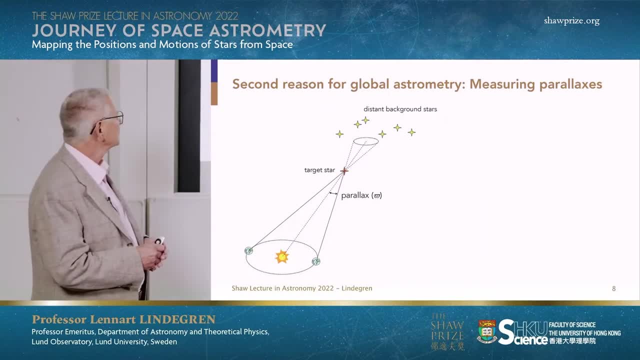 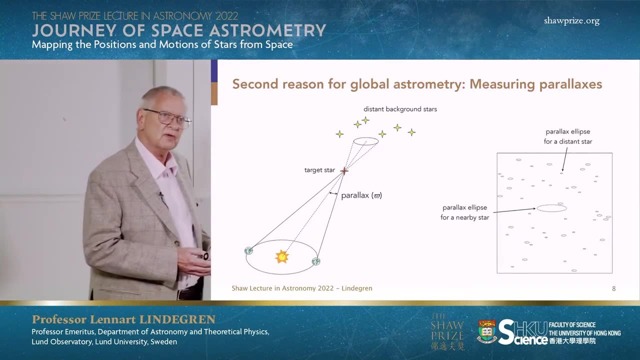 compared to the background stars. This is the parallax. This parallax ellipse is actually the mirror image of the earth's motion around the sun as seen from the star, And the more distant the star is, the smaller this ellipse is. But even the background stars 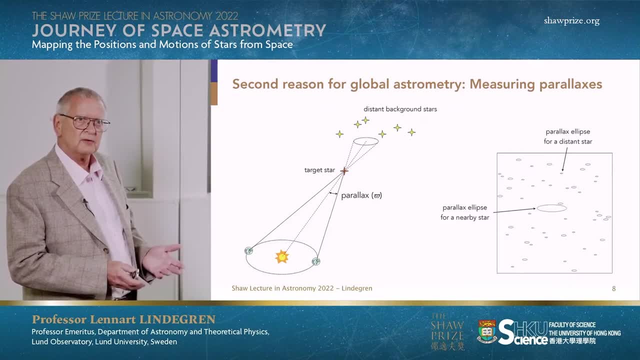 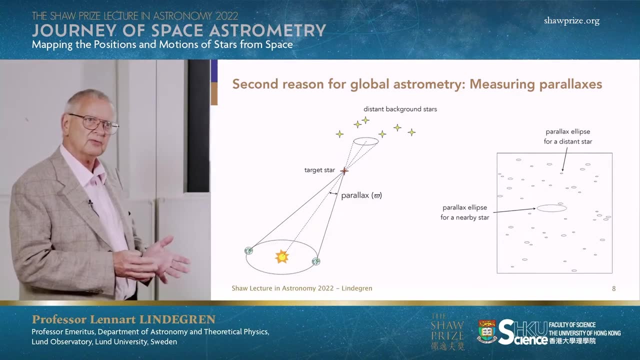 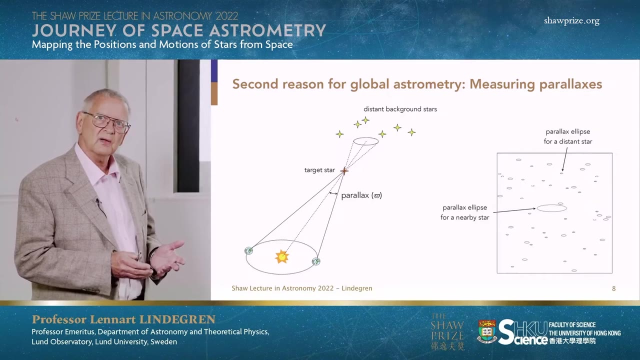 are not at infinite distance, which means that they too have a parallax. They also move in small ellipses, And when we do measurements in a small field, then we will not see the whole parallax of this nearby target star. we will only see the difference. 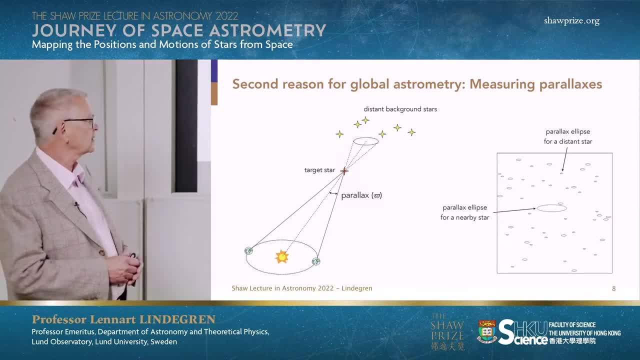 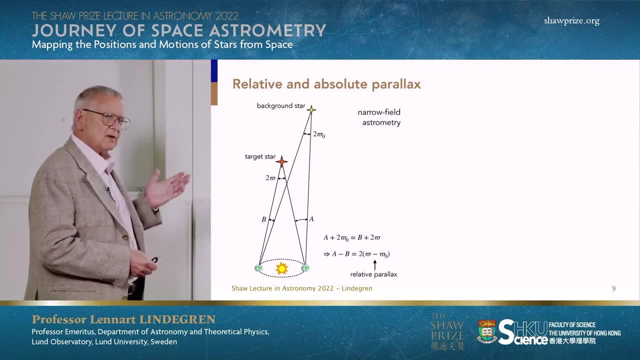 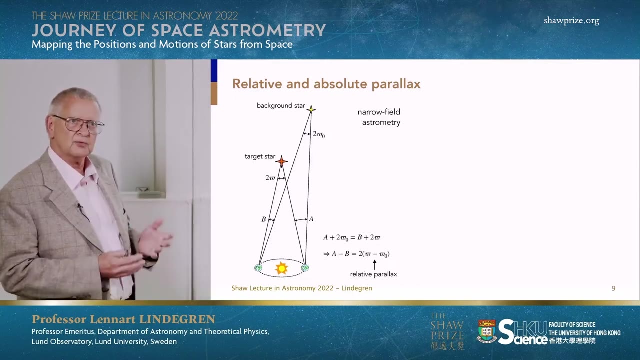 in parallax between its parallax and the mean parallax of the background stars. This diagram illustrates the same thing in a slightly different way. We can see here that by measuring the angles A and B, which are small angles on the sky between the target star and the background star, 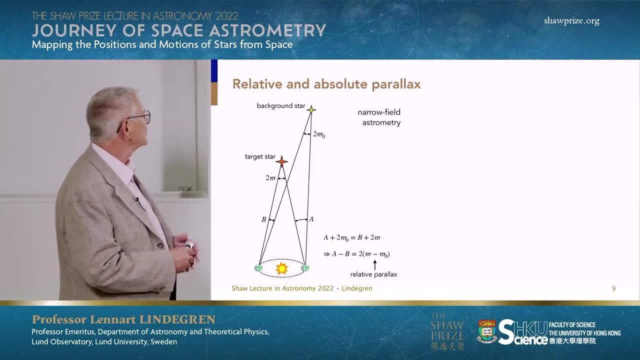 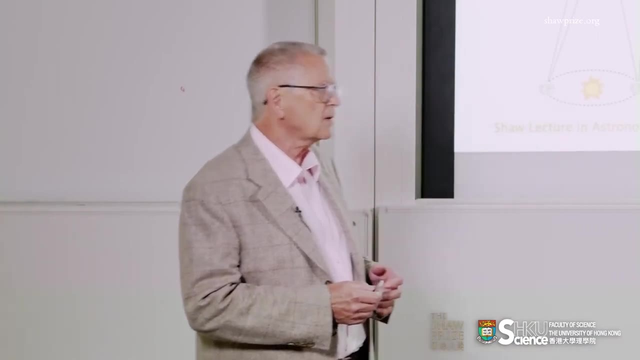 we, by taking the difference between these two angles, what we get is twice the difference in parallax between the two stars, And that is what I call the relative parallax. This is okay as long as we are only looking at some of the most nearby stars. 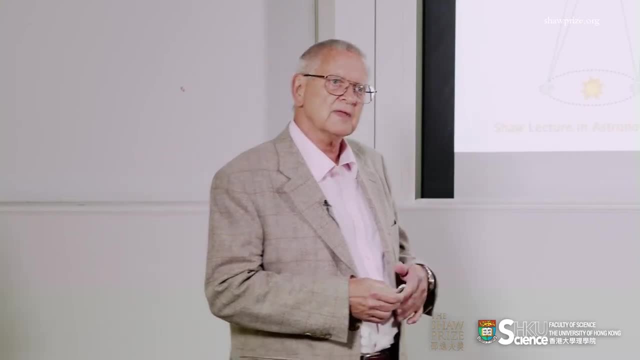 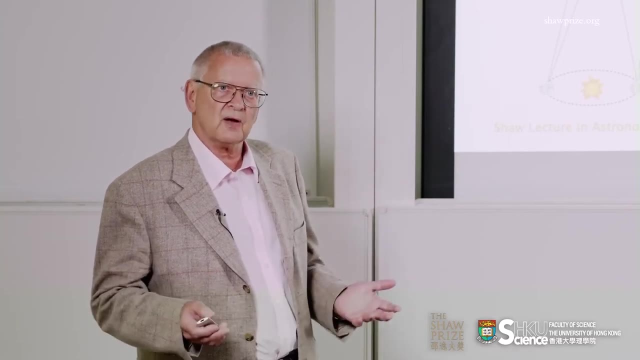 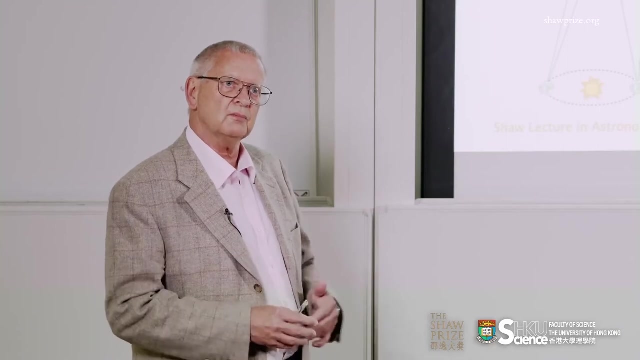 to our solar system, But if we want to map stellar distances throughout our galaxy, this method will not work anymore, Simply because most of the stars are background stars. They are at such great distances that there are no more stars sufficiently more further away that they can be used as a background. 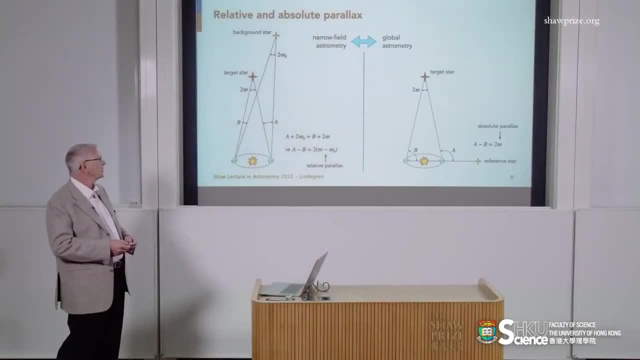 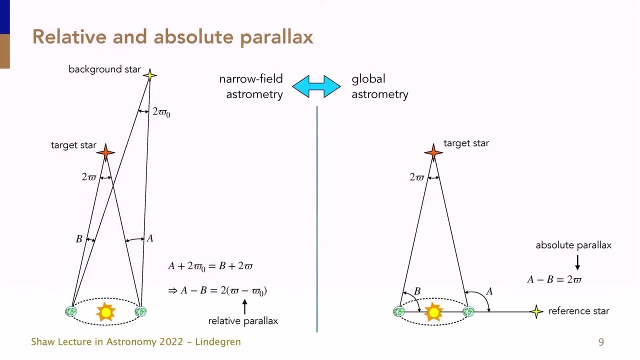 So the solution to this problem is, again, global astrometry. With global astrometry we can measure not only small angles on the sky but also large angles of the order of 90 degrees. So suppose we measure the angle between the target star and the reference star. 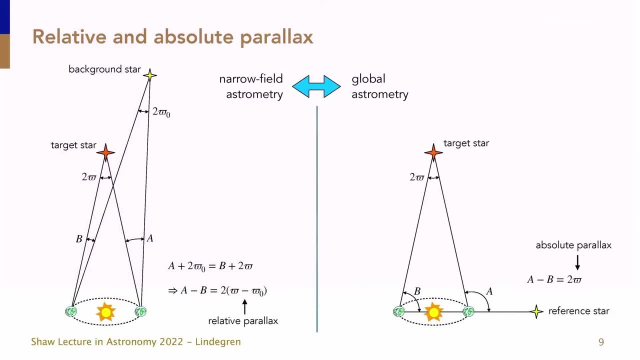 90 degrees away from it at two different times, when the Earth is in opposite points in its orbit around the Sun. Then by taking the difference between these two angles, we get twice the parallax of the target star, And this result is independent of the distance to the reference star. 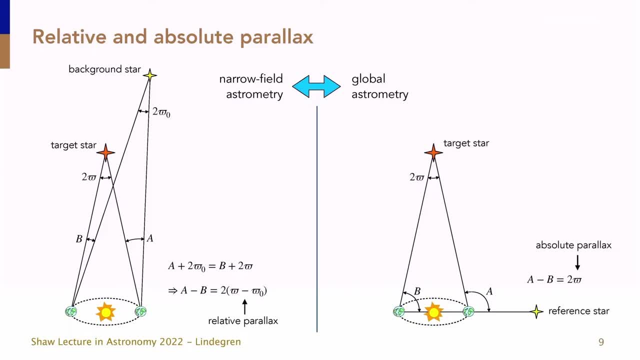 We can even have a reference star that is not at all in the background, but even closer to us than the target star. In this way we get absolute parallaxes, But it requires to measure large angles of the order of 90 degrees. So now I give you. 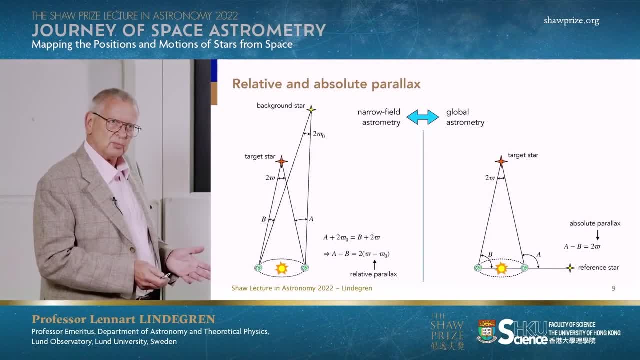 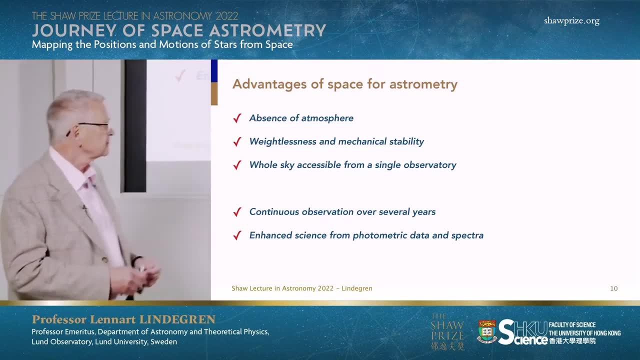 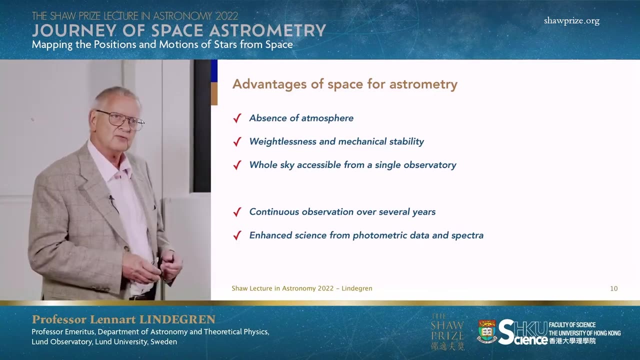 some good reasons why we need global astrometry. Now I have to tell you why we have to do it from space. Space offers some very important advantages for astrometry, and especially for global astrometry. First of all, we have the absence of atmosphere. 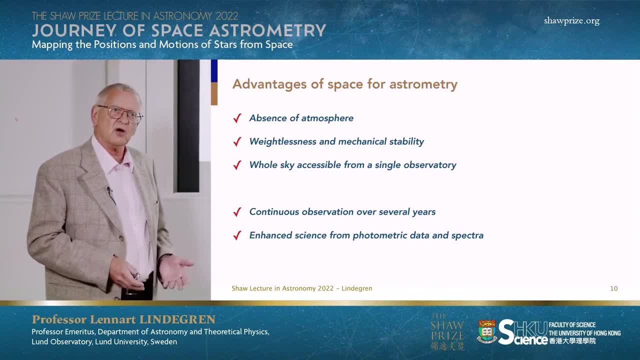 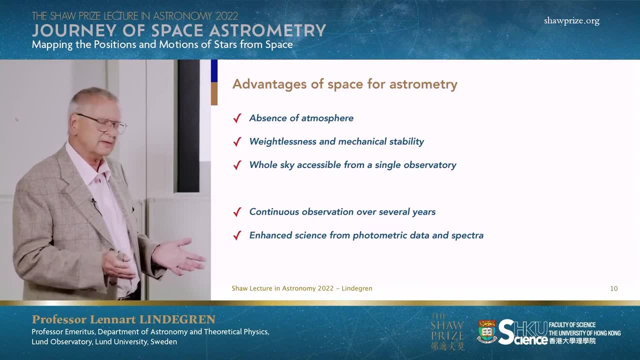 which means that the images of stars are very sharp and stable and we don't have a refraction in the atmosphere that changes their directions. We also have weightlessness, which means that we can turn the instrument in different directions without it being distorted by gravity. 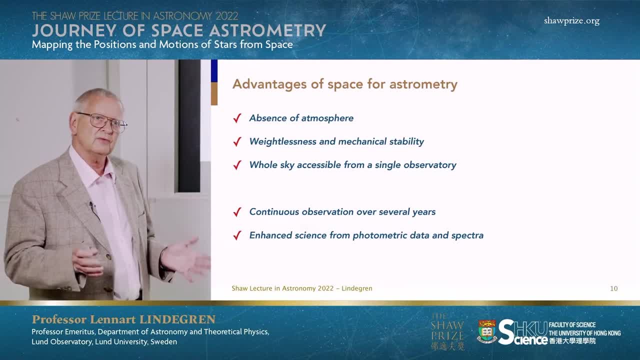 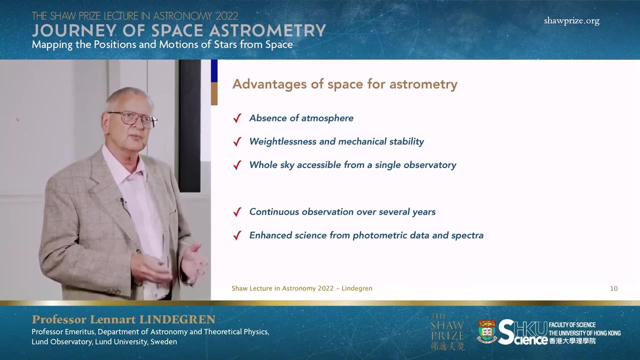 And we also have a stable thermal environment in space, which means that we can also have mechanical stability in the instrument. And the final point, which is very important for global astrometry, is that we can access the whole sky from a single point, from a single instrument. 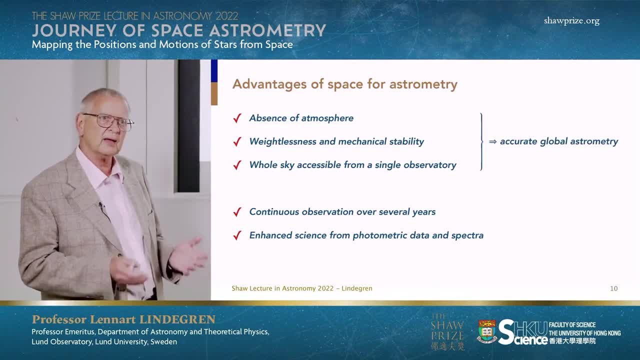 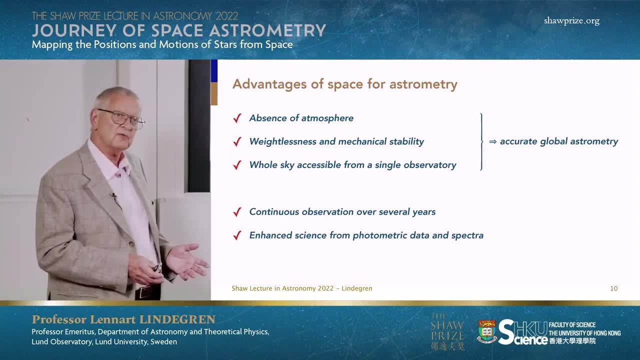 These three points together means that we can do accurate global astrometry from space. There are other advantages as well from observing from space, For example, that we can observe more or less continuously, 24 hours per day over several years, And we can also collect additional. 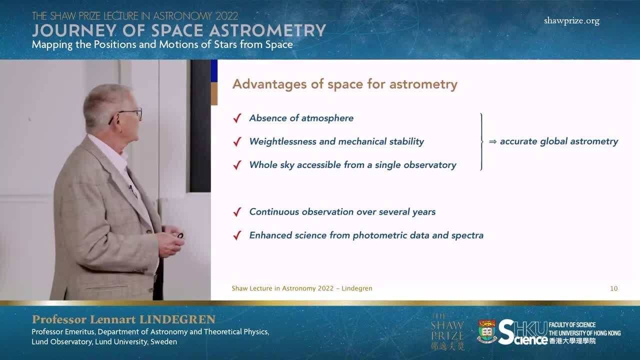 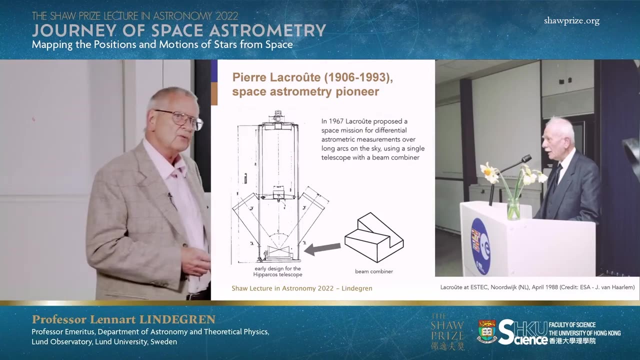 data like photometry and spectra that are extremely useful for the astrophysics and we get them almost for free. The idea to use space for astrometry was first put forward by the French astrometrist Pierre Lacoute In 1967. 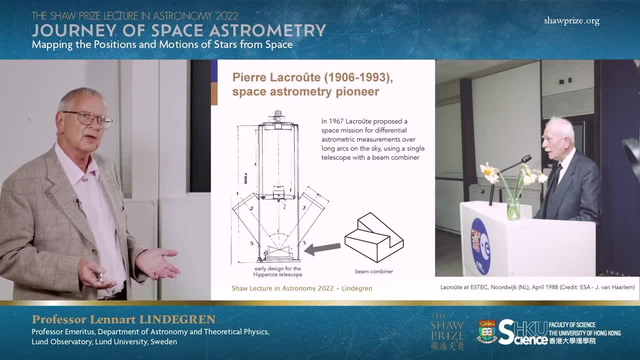 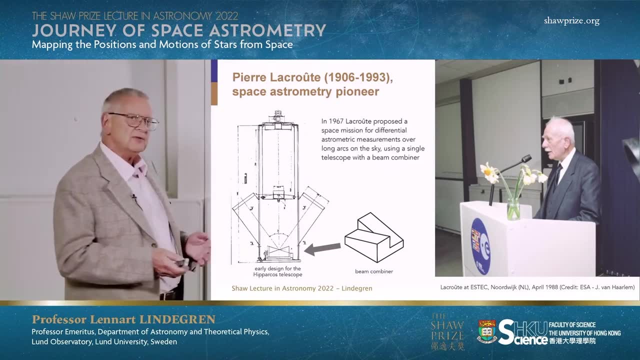 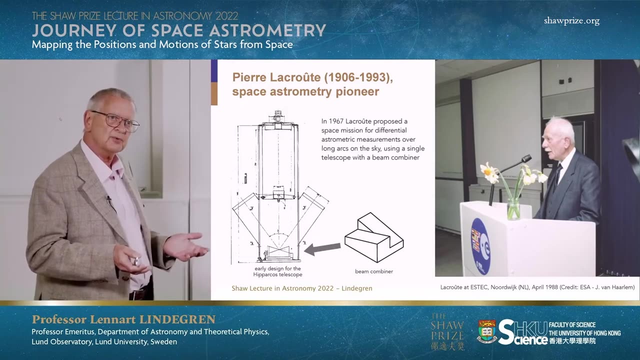 he proposed a space telescope that was able to do differential measurements over long arcs on the sky And using a single telescope and a beam combiner in front of it. This beam combiner makes it possible for the telescope to look simultaneously in two different directions. 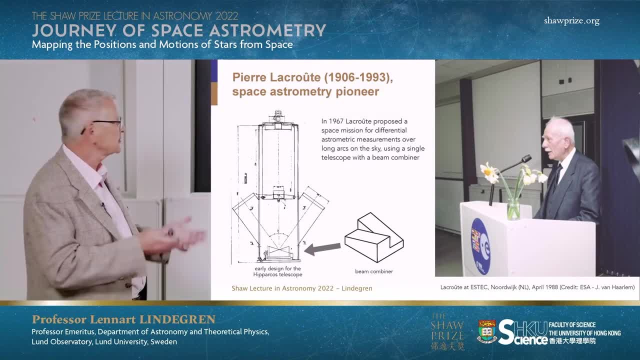 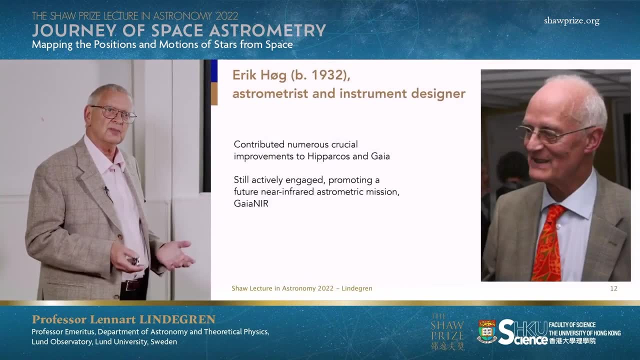 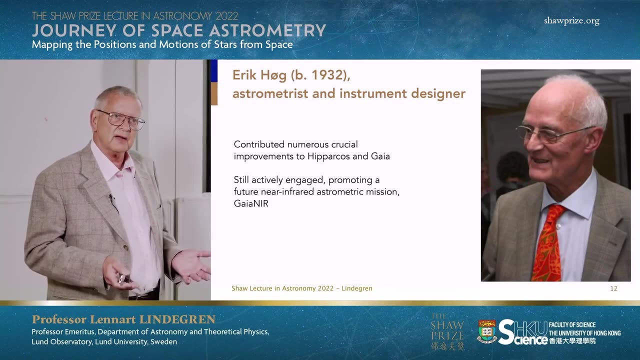 And that enables us to do these large angle measurements. It took more than 20 years for this idea to be realized before Hipparchus was launched, And this development was the result of many people contributing to this mission. I will mention only one of them. 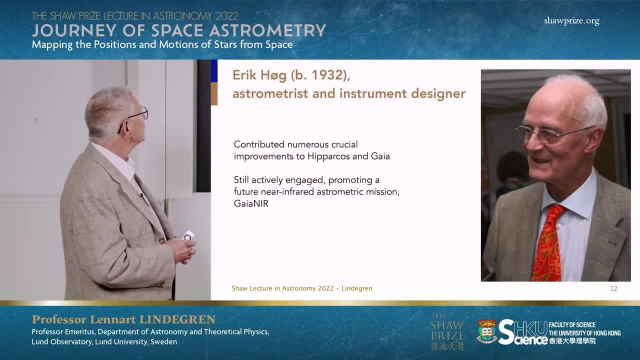 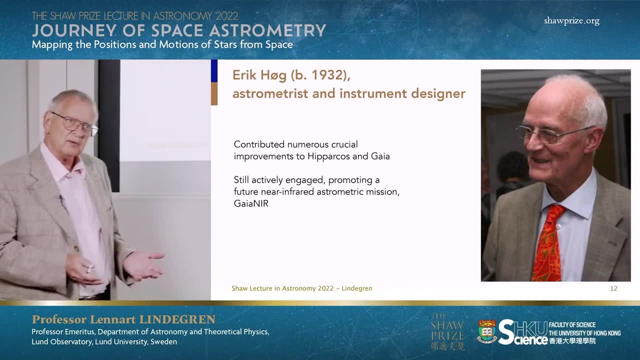 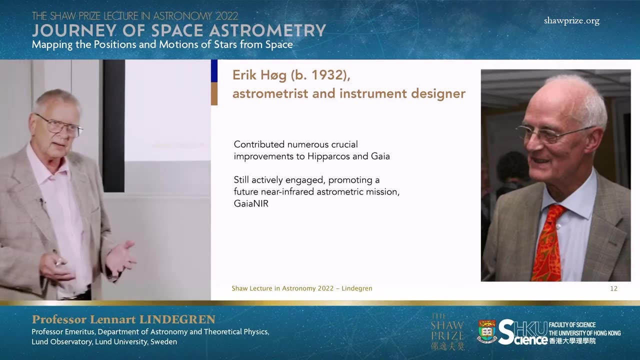 The Danish astronomer Erik Kerg, who contributed many crucial improvements to the original ideas, First to Hipparchus and then also to the Gaia project. It was the dedicated work over many years by people like Erik Kerg that transformed Lacoute's vision. 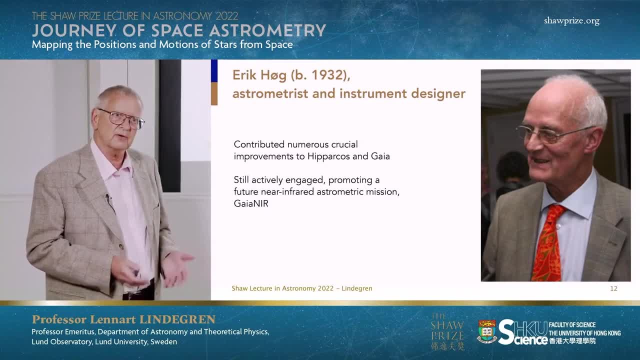 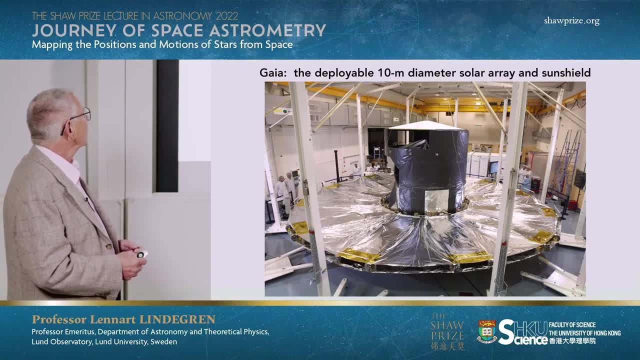 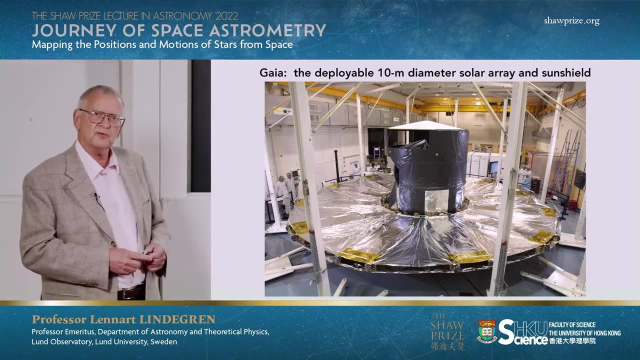 into a real mission, Or actually two missions: Hipparchus and Gaia. Now let's take a look how this actually works in Gaia. This picture shows the Gaia satellite shortly before launch, when the deployable sun shield was tested Inside the central. 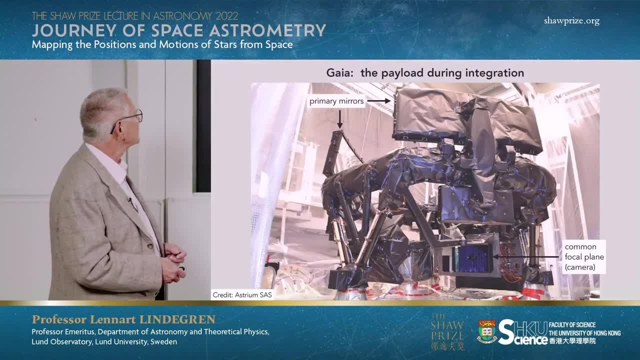 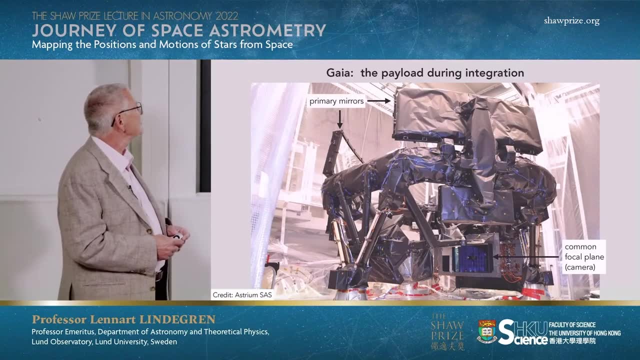 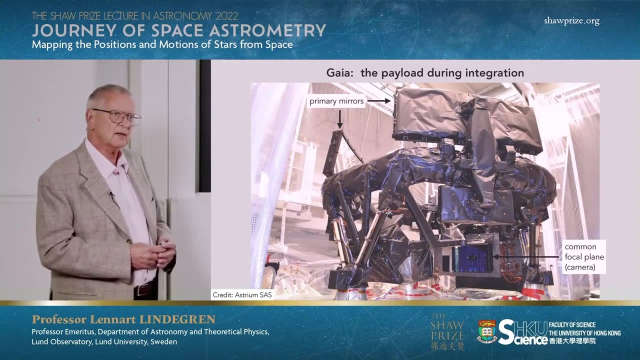 hut. there is the instrument, the payload, which is shown in this picture during integration. In the top part of the picture you see the two primary mirrors that look in two directions And at the bottom right you see the focal plane, the common focal plane for the. 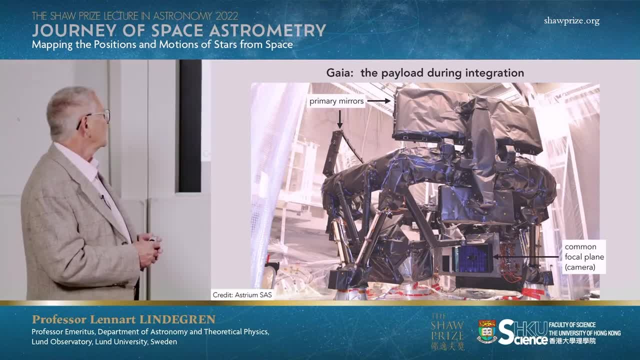 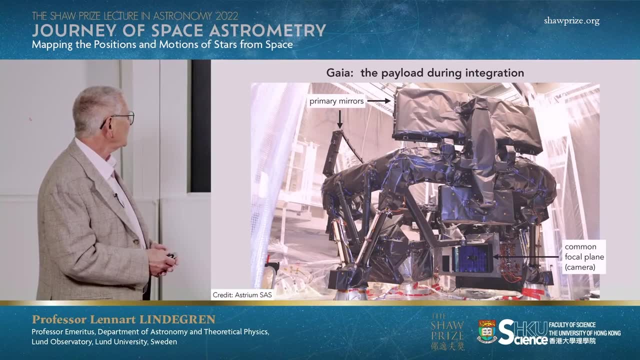 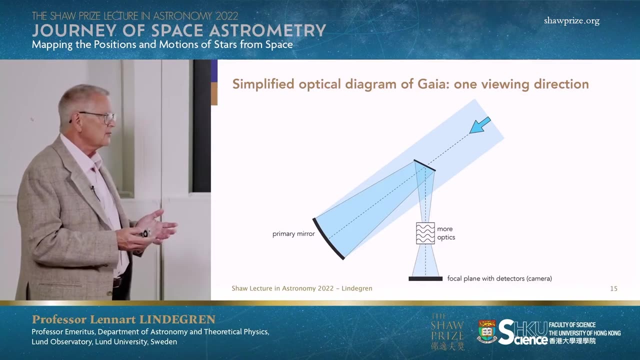 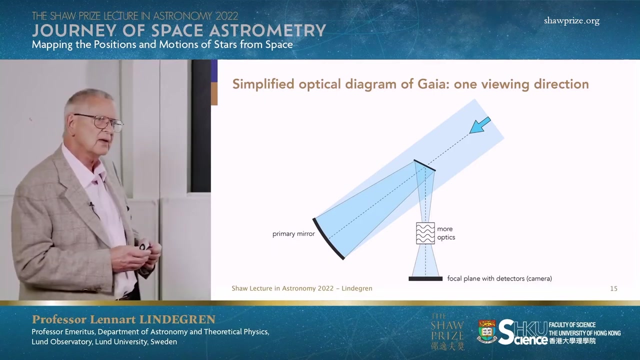 two mirrors- or the camera, if you like- Consisting of more than 100 CCVs covering almost one square meter. This is how the telescope works. Light from one direction is collected by one of the primary mirrors and is then reflected by a flat mirror into. 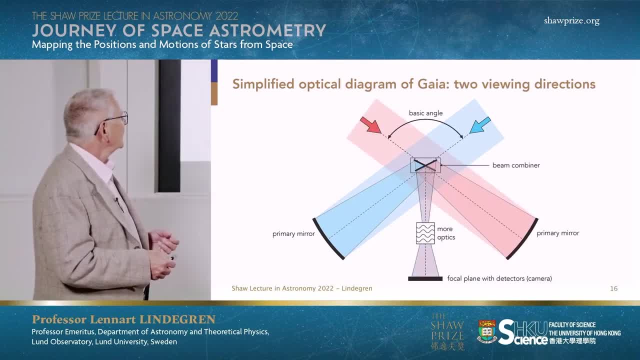 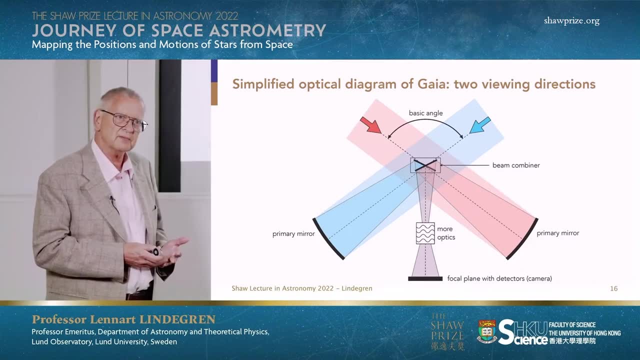 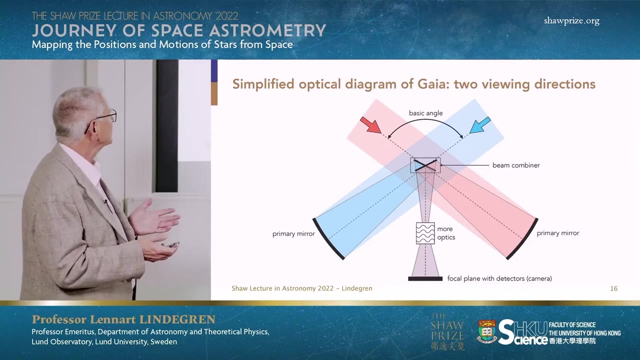 some additional optics and onto the camera. Light from the other direction goes to the other primary mirror and is then reflected to the same focal plane, the same detectors. This means that the telescope can simultaneously look in two directions, separated by a large angle called the basic angle. 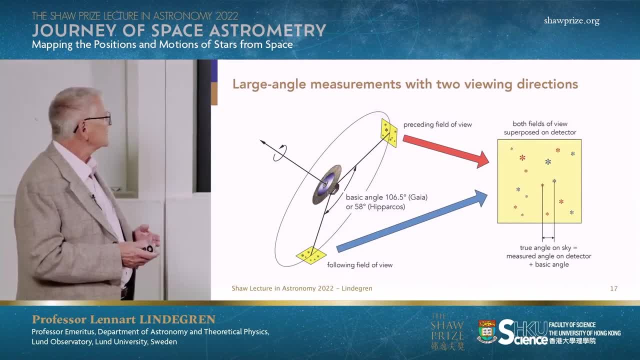 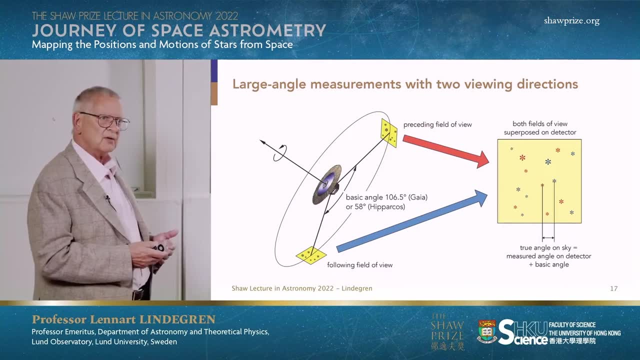 The overall effect is that the satellite Gaia can look in two different directions on the sky at the same time, With some stars coming from one of the fields of view, here called the preceding field of view, and some stars from the other field. 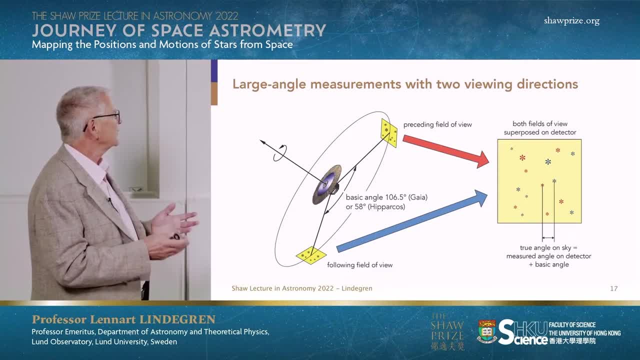 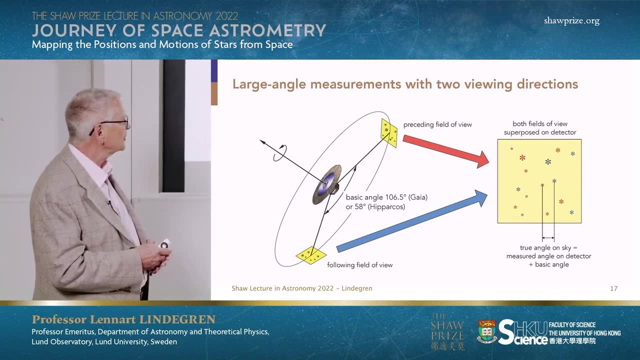 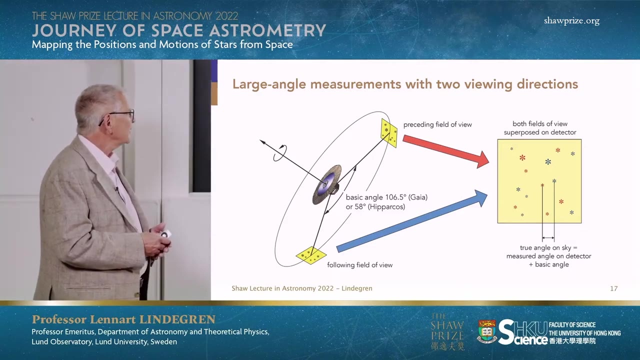 the following field of view, But they are all seen on the same detectors. In the image to the right, the stars coming from the preceding field of view are shown in red and in blue are shown as the stars coming from the other field of view. 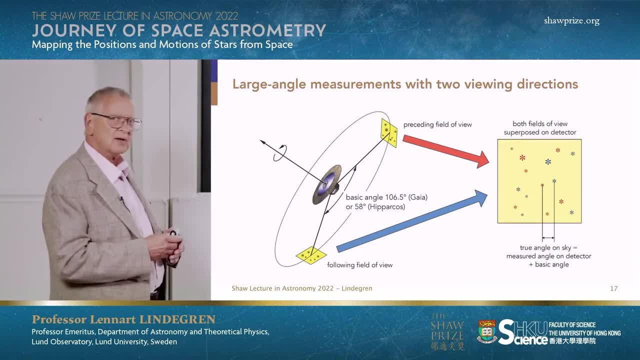 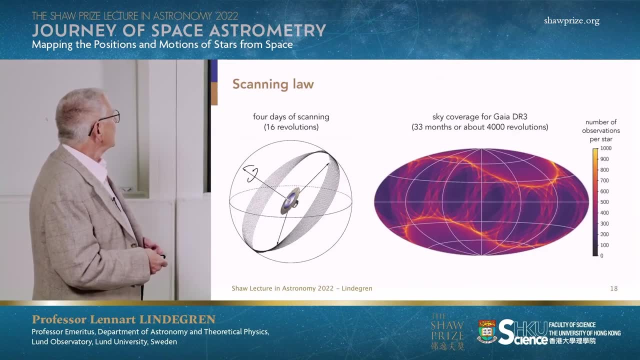 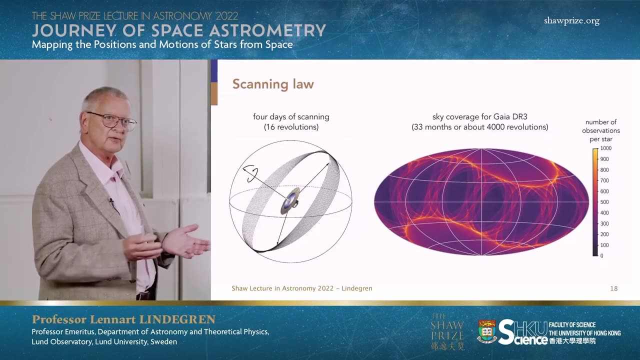 On the detector you can measure the angle between these images, But to get the true angle on the sky you have to add the basic angle. The satellite is slowly rotating around its axis, which means that the two fields of view sweep roughly along a great circle. 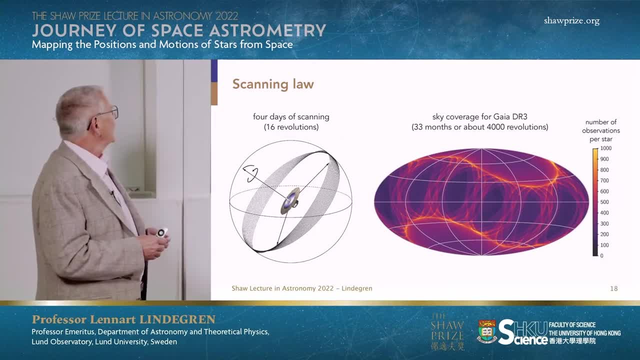 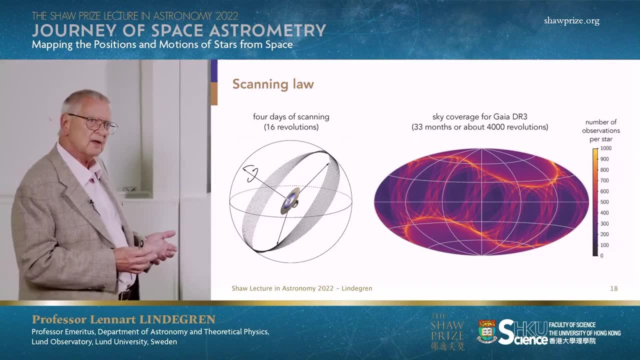 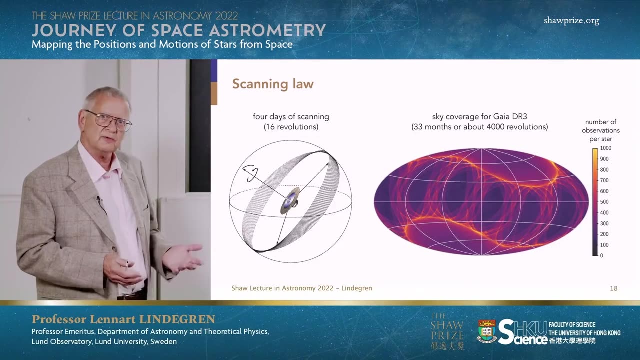 on the sky in six hours. But the rotation axis is not fixed in space but is slowly changing its direction, which means that a successively larger part of the sky is covered by the two fields of view And after a few months you have covered all the sky. 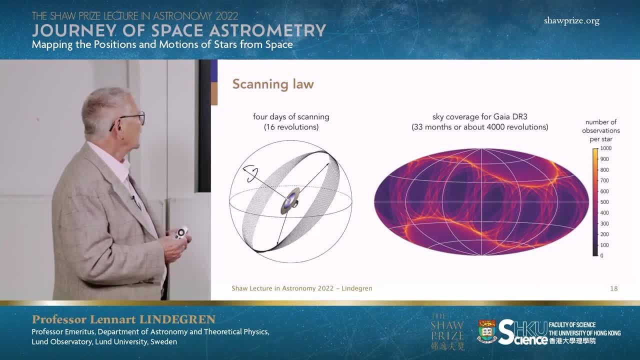 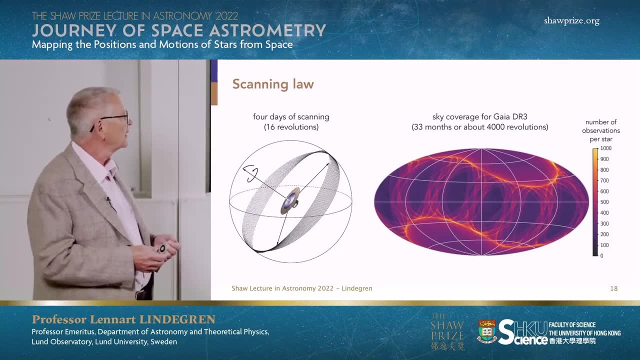 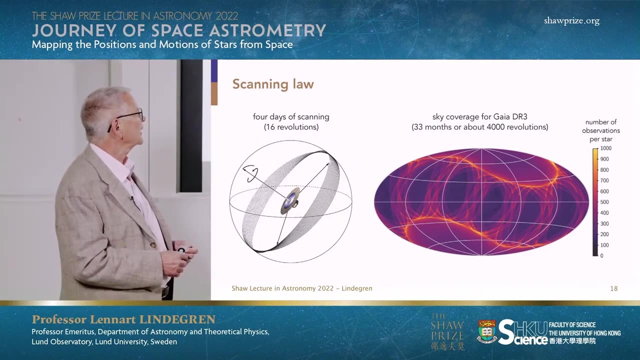 And this is then repeated many times over the years. The diagram to the right shows the number of observations obtained at each point on the sky after nearly three years of observations, namely the observations that were used for the third release of Gaia data, Gaia DR3. 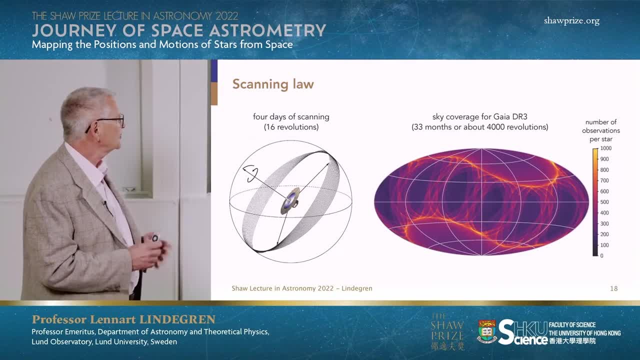 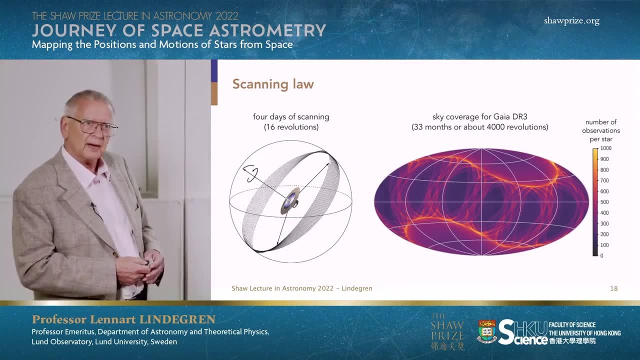 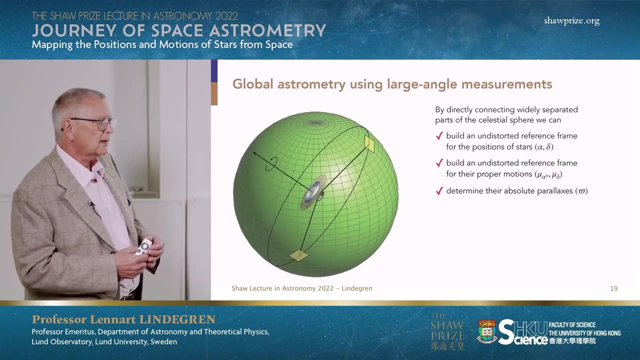 You can see that the number of observations per point on the sky varies from a few hundred up to about a thousand. This is the so-called scanning law, for Gaia and Hipparchos used a very similar scanning law. Now I will try to explain how this. 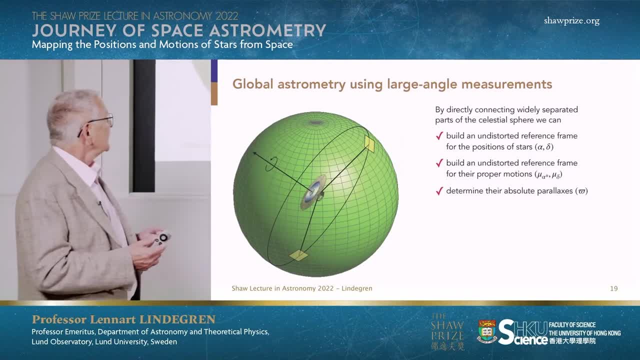 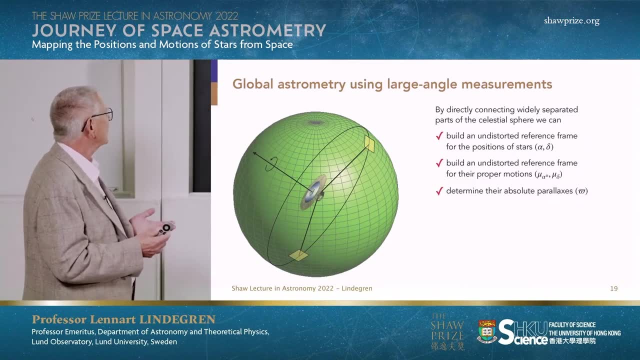 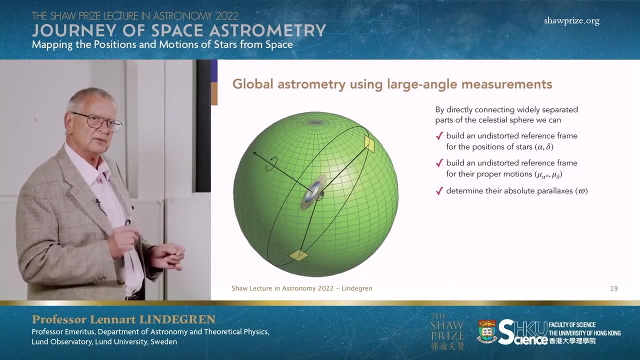 makes it possible to do global astrometry. The point is that we want to construct a celestial reference frame that is undistorted, as I mentioned before. If it is undistorted, there will be errors in the two fields of view that are not the same at all the time. 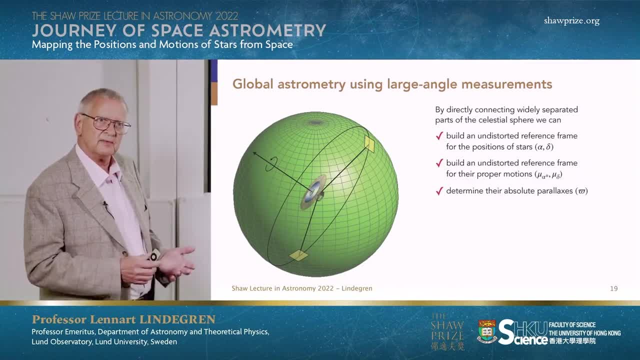 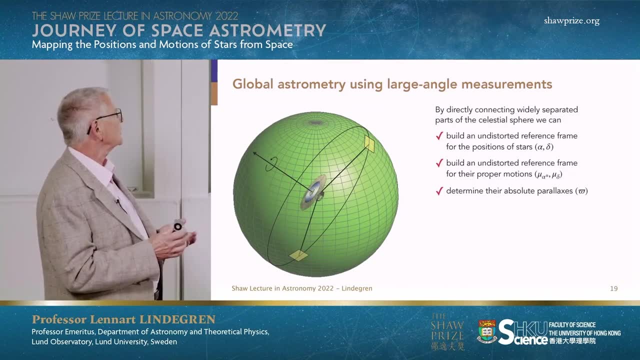 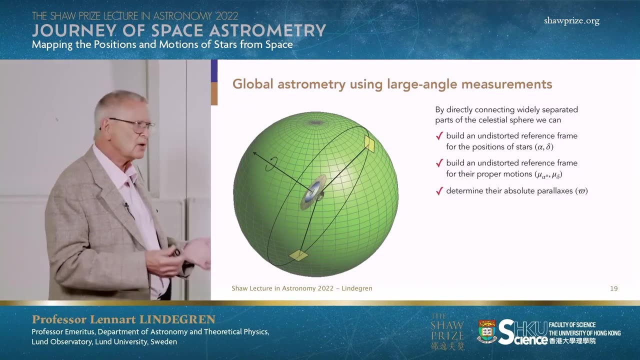 And these differences can be measured by the satellite, and that makes it possible to construct an undistorted reference frame. So we obtain this reference frame for the positions, but in a similar way also for the proper motions we get an undistorted reference frame. 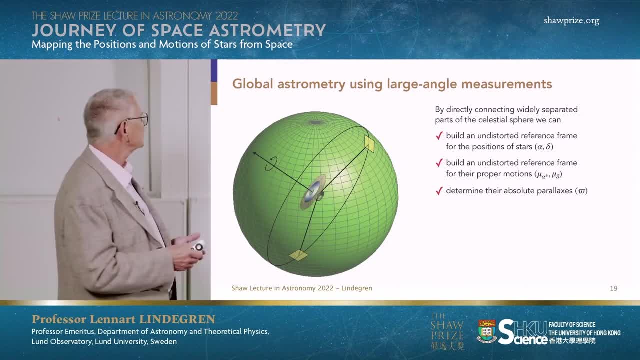 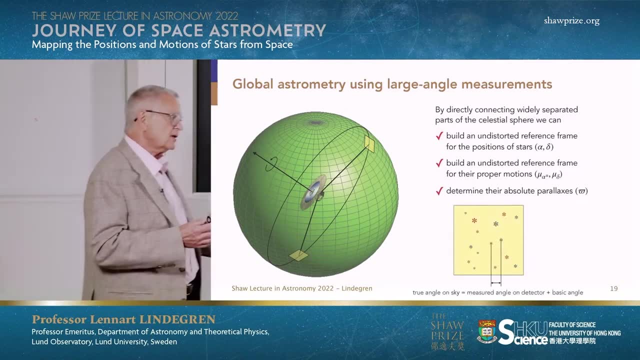 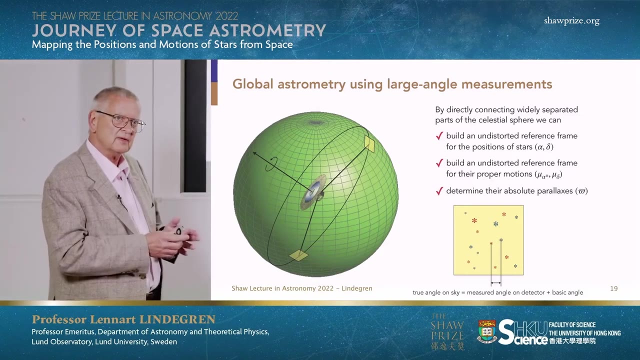 And at the same time we can also determine the parallaxes using the large angles between the stars. But there is one problem, of course. As I said before, to get the true angle on the sky you have to take the angle that is measured on the detectors. 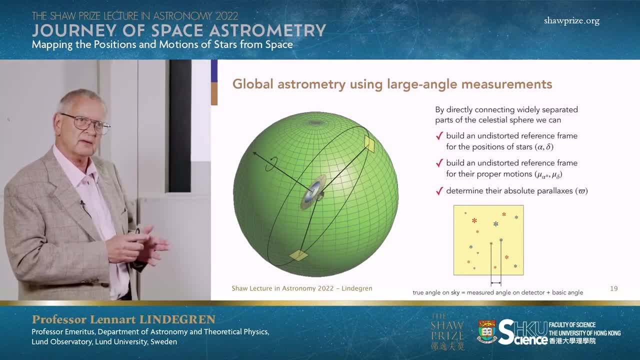 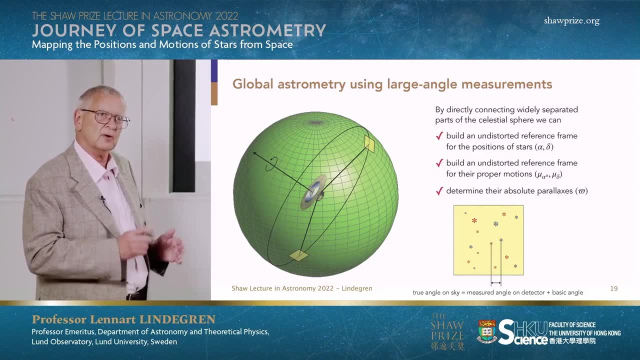 and add the basic angle. So how can we know the basic angle? We need to know it to the same precision that we aim for in the final astrometric data. That is the micro-arcsecond precision, And no device on board the satellite. 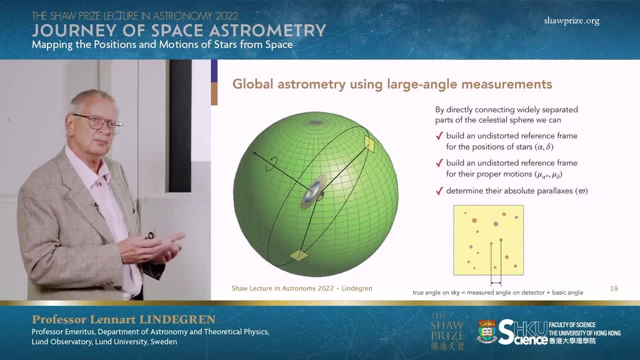 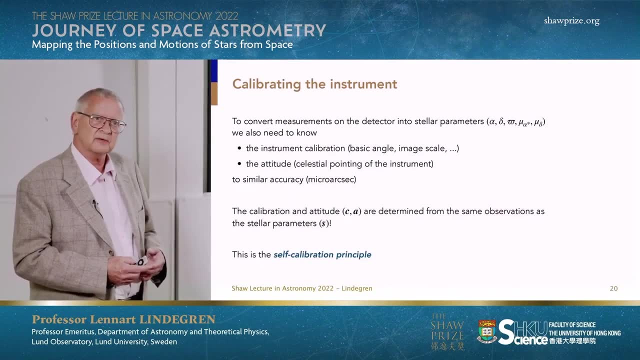 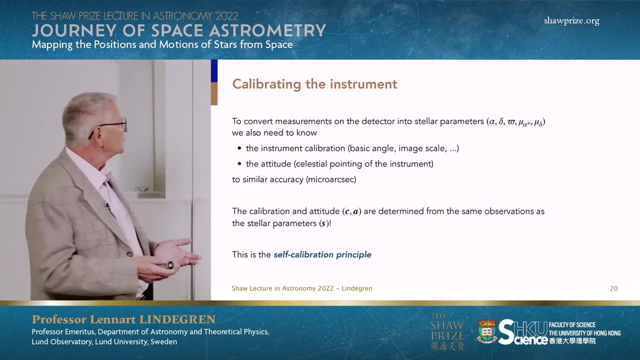 is able to measure this basic angle to that kind of precision. So the answer to that is something called the self-calibration. We need to calibrate the instrument, like the basic angle, image scale and so on, but we also need to know exactly. 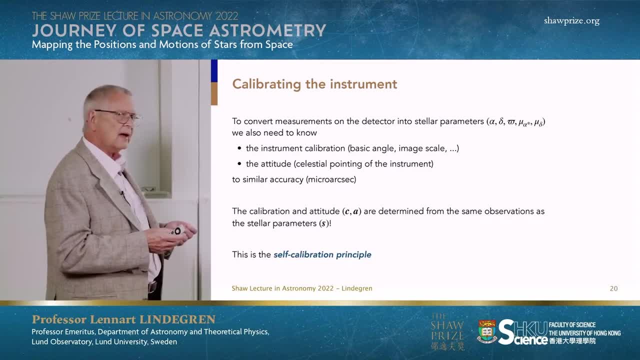 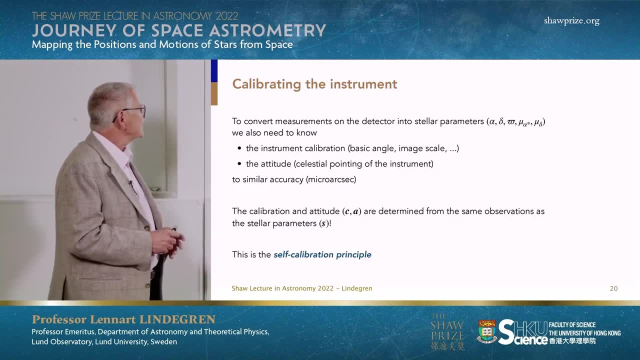 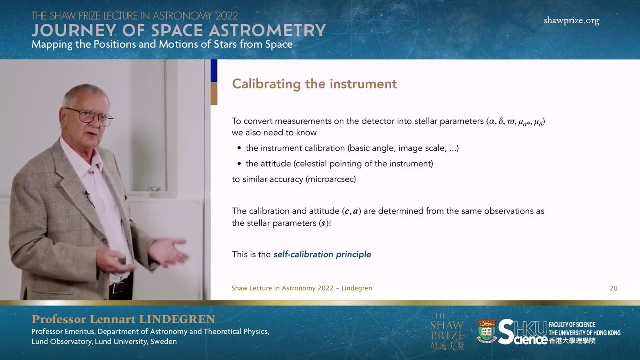 where it is pointing on the sky at each point in time. This has to be done to similar accuracy to micro-arcsecond accuracy. Self-calibration means that the calibration and attitude parameters are determined from the same observations as are collected to do the astrometry. 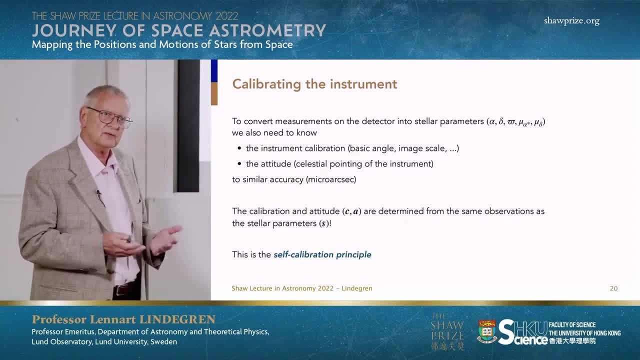 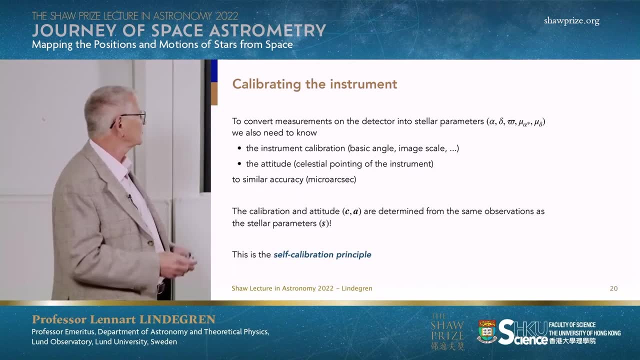 We don't need any special device for the calibration or attitude determination and we don't need any special observations for that. We use the same observations as are collected for the astrometry, So it is a self-calibrating instrument. To illustrate how this works: 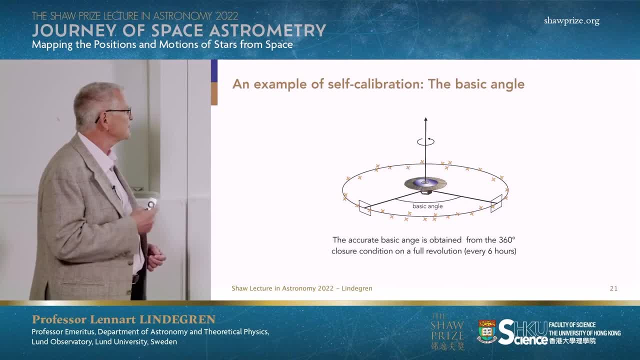 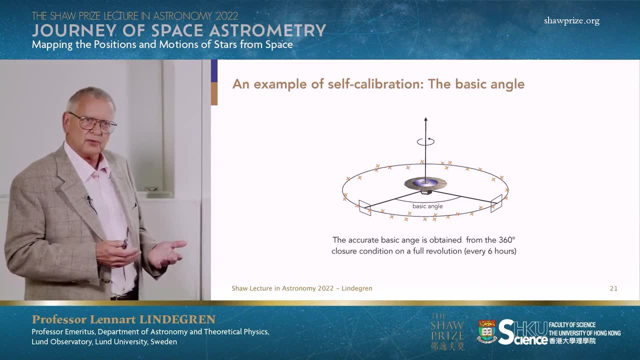 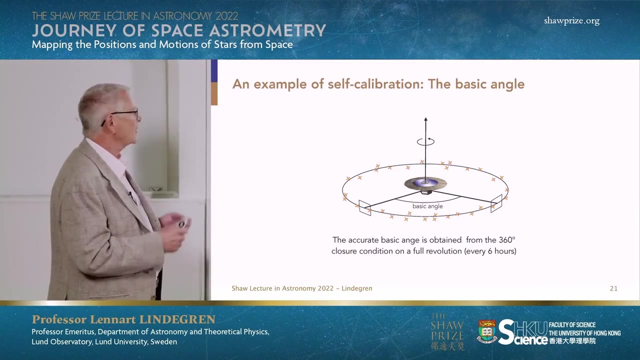 in practice. let me just take the example how the basic angle is determined. Assume that we know approximately what the basic angle is, We can use this value to compute the angles between pairs of stars in the two fields of view And as a satellite turns. 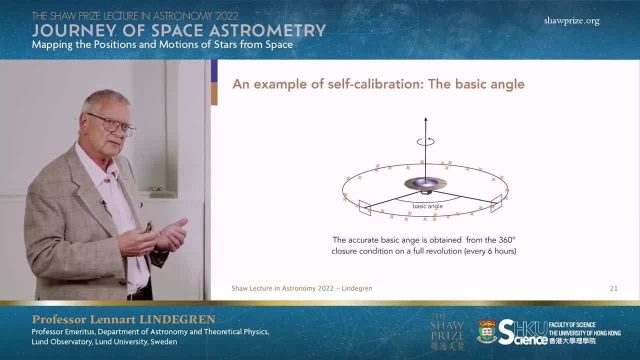 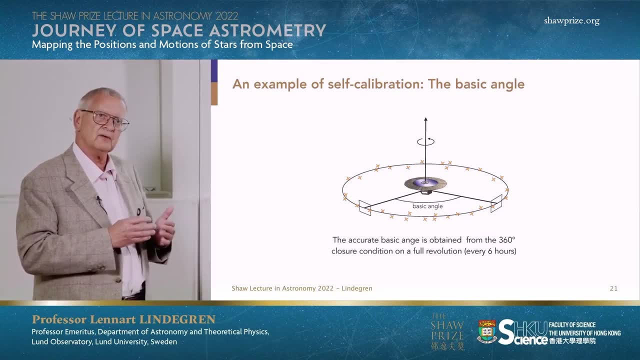 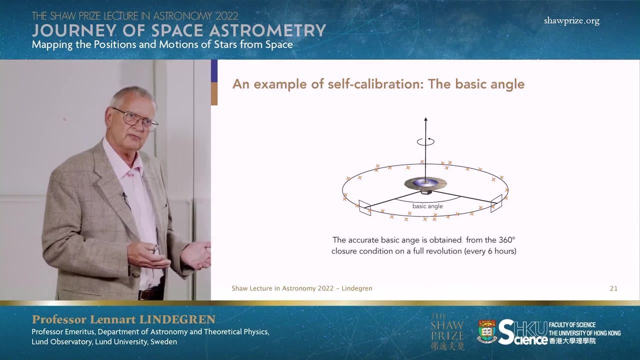 a full revolution in six hours. we get angles between different pairs of stars And if we add up all these angles along the great circle they should add up to 360 degrees. But if we use the wrong value for the basic angle they will not add up to 360 degrees. 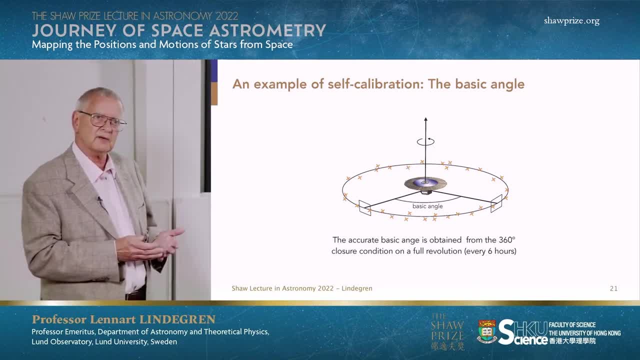 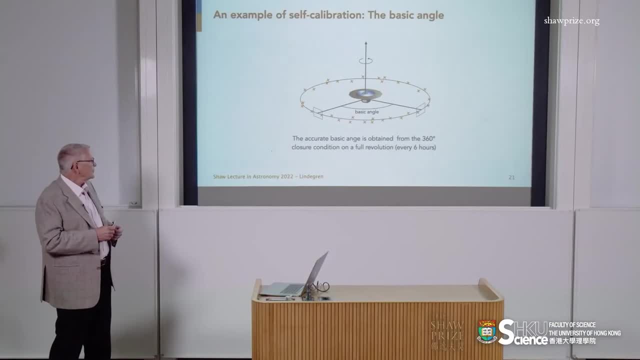 but to something different, And that allows us to compute what the basic angle actually was, And the result will be as accurate as the measurements are. So effectively we get the calibration every time the satellite completes a complete revolution over six hours. In a similar way, 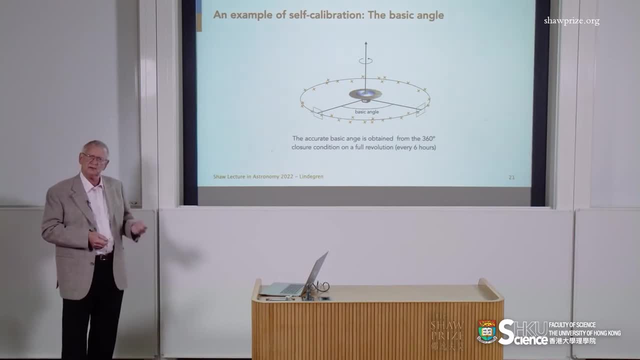 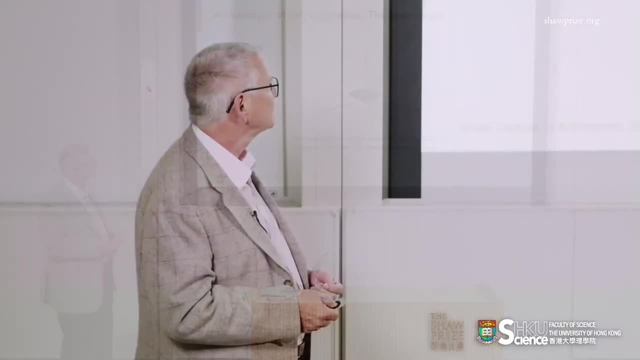 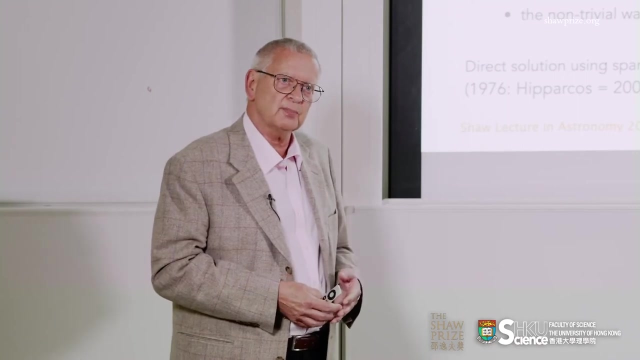 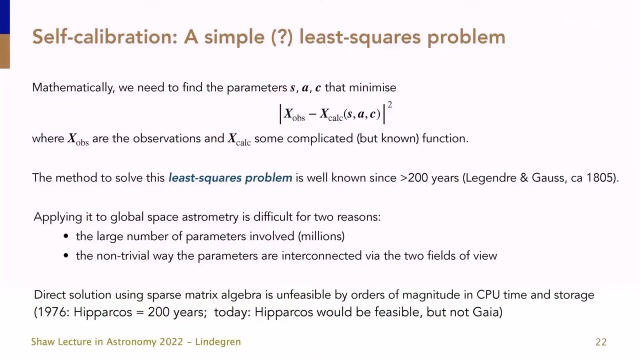 other parameters, like the image scale and the attitude, are obtained from the observations basically by the equivalent procedures. It is actually not difficult to formulate these self-calibrating principles in mathematical terms. The observations here denoted x, obs. They can be described in terms of all these parameters. 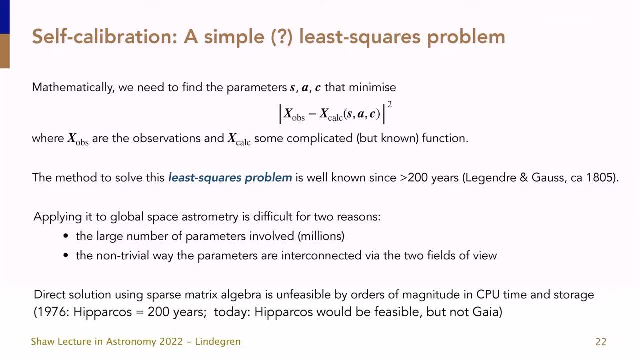 The stellar parameters as the attitude a and the calibration parameter c by means of some complicated function: x, calc. It is complicated but known. What is not known is the values of the parameters s, a and c. What we have to do is to adjust. 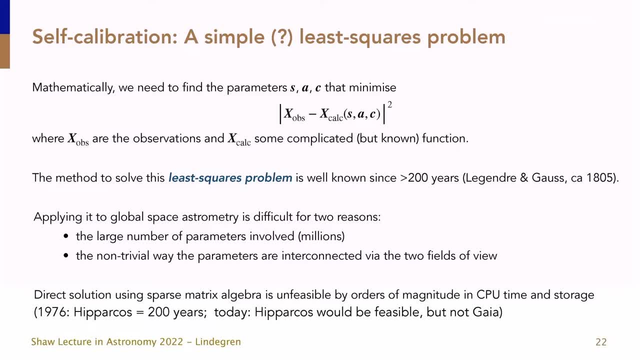 these observations as measured by the sum of the squares of the differences between the measured values on the detector and the calculated values, assuming that we have the different parameters. This is what we call a least squares problem, And the way to solve it has been known for more than 200 years. 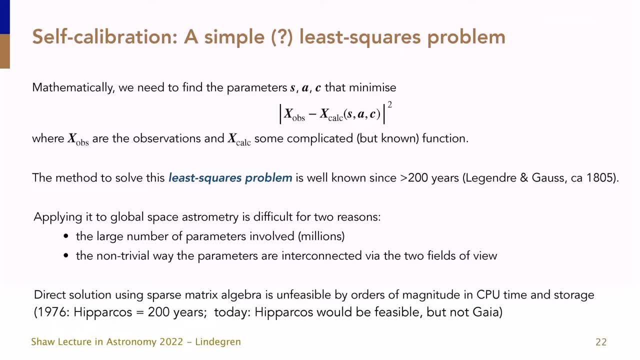 So, in principle, it is a simple problem. It is solved for two reasons: One is that there is a very large number of parameters to solve- Millions of them, Hundreds of millions even- And the other is that these parameters are interconnected in a very complicated way. 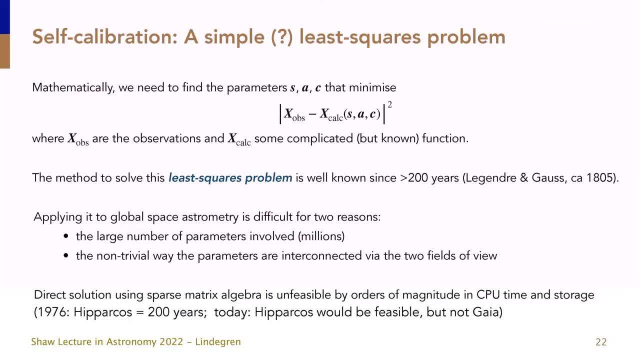 thanks to the two fields of view, where the observations are mixed, and also the scanning law, which makes a complicated pattern on the sky. If we try to do a direct solution of this problem, using sparse matrix algebra, for example, it would require far too much computing time. 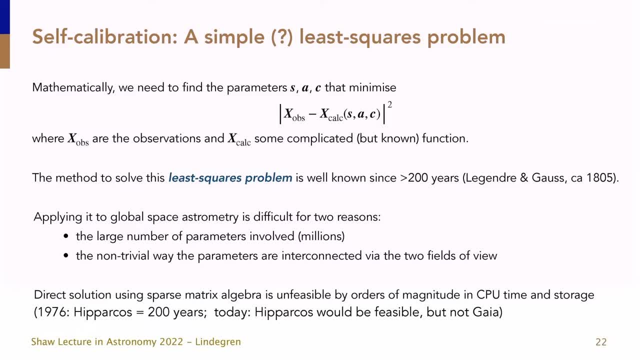 and computer memory to be solved even with the biggest computers available on earth today. Already in 1976 it was concluded that to solve these equations for Hipparchus would require 200 years to have a powerful computer available in those days. Today, this problem 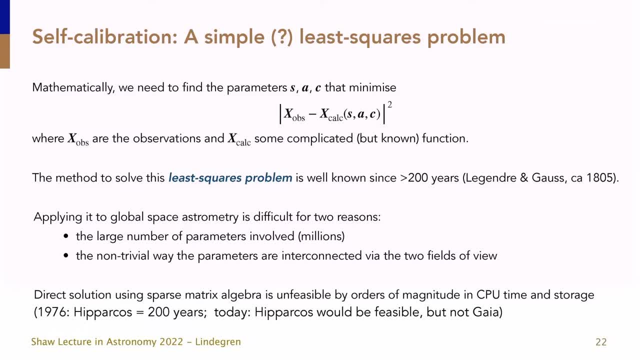 would probably be feasible for Gaia. It would probably be feasible for Hipparchus, but in Gaia we have so many more observations and so many more unknowns that it is certainly not feasible to do a direct solution For Hipparchus. we came up 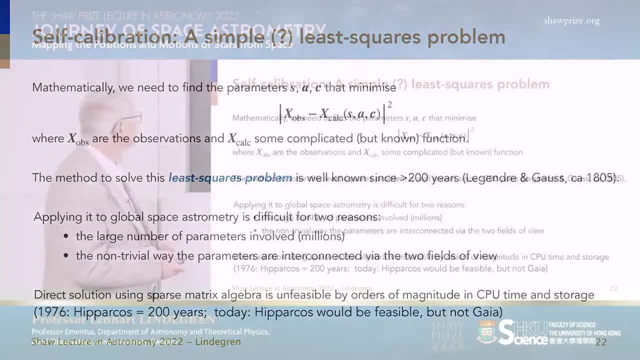 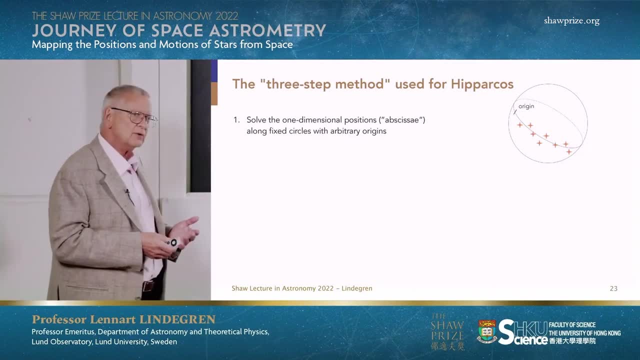 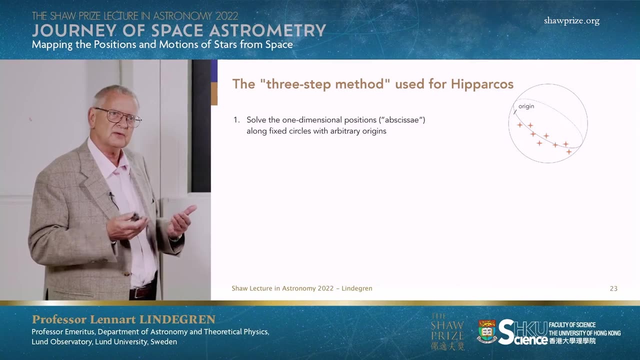 with an approximate solution in the 1980s. It is a three step method which I will briefly describe. The first step is that we use one dimensional measurements along a great circle on the sky, where we solve for the coordinates of stars along this great circle. 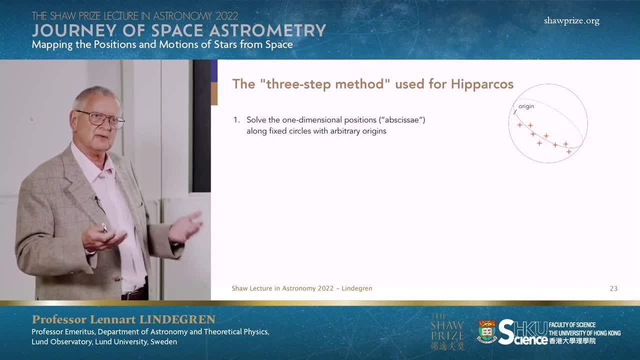 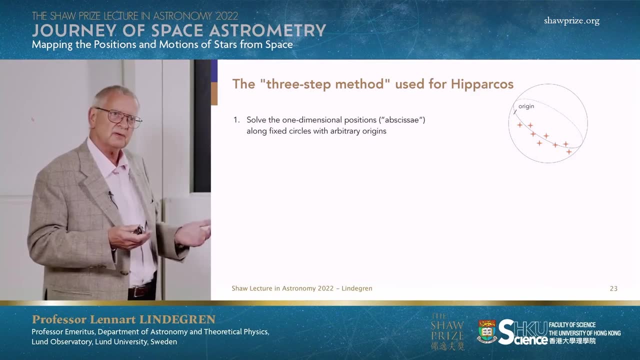 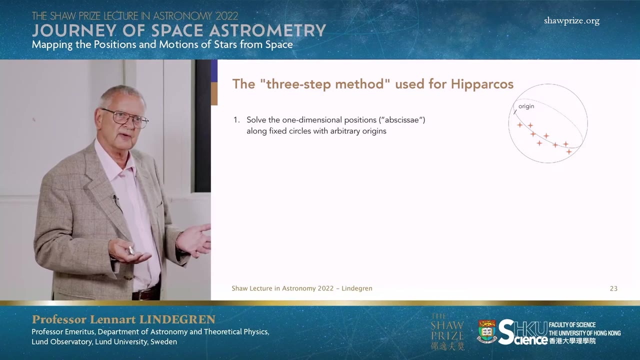 at the same time as we obtain the basic angle, image scale and so on. We can get these positions of the stars, but we don't know the origin, the zero point for these angles. that is only defined when we have the celestial reference frame, which we don't know yet. 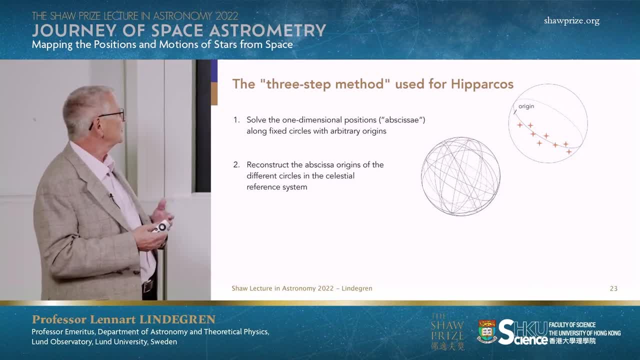 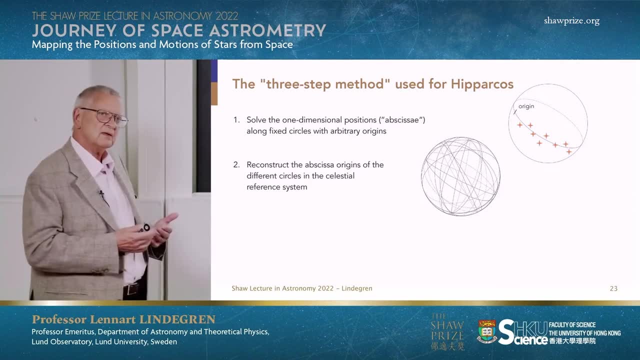 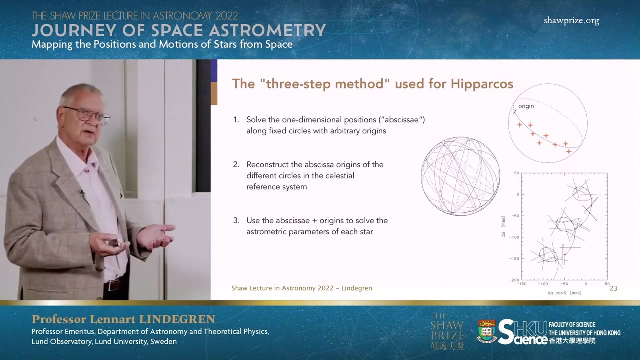 In the second step we solve the origins of all the few thousand great circles in such a way that the coordinates form a consistent reference frame over the whole sky. And then the third step is simply to combine the abscissa and the origin for each individual star. 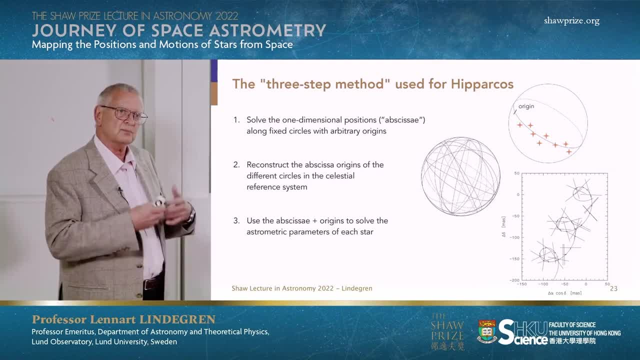 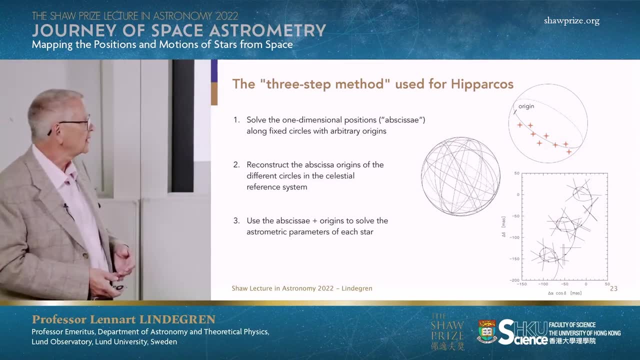 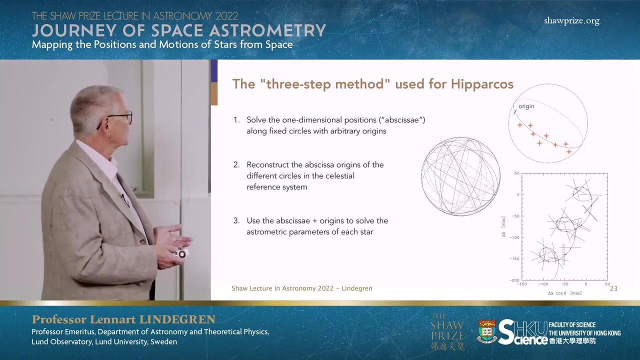 in such a way as to get its positions, proclamations and parallaxes. So this worked well for Hipparchos, because in each step you don't need to solve very big systems of equations. so it was quite- I wouldn't say- easy. 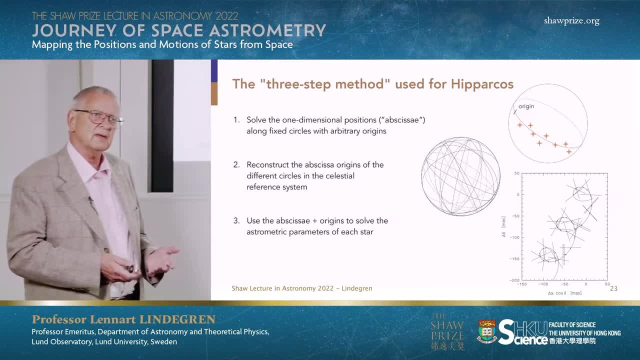 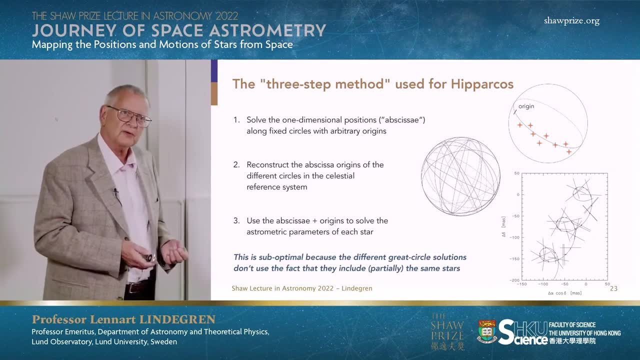 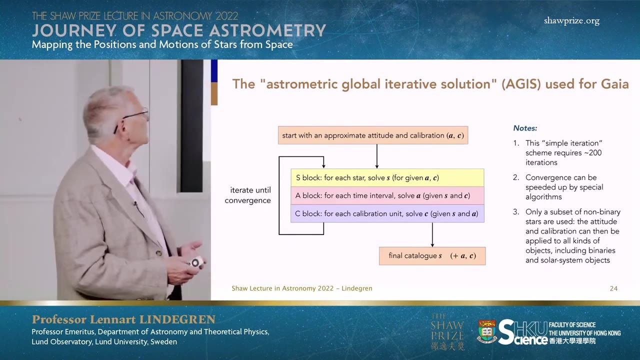 but definitely possible to do in those days. It is, however, an approximate method and therefore suboptimal, and for Gaia. we wanted to do something better, And what we came up with is what is called the astrometric global iterative solution, or AGES. 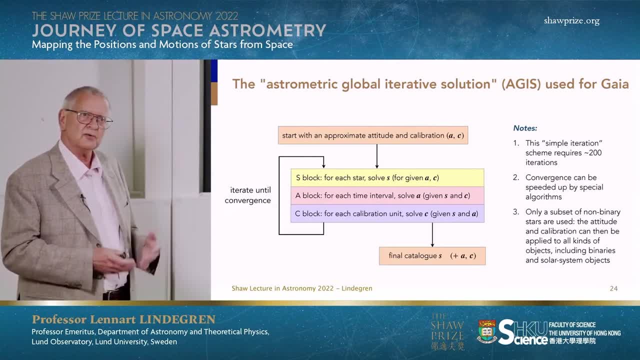 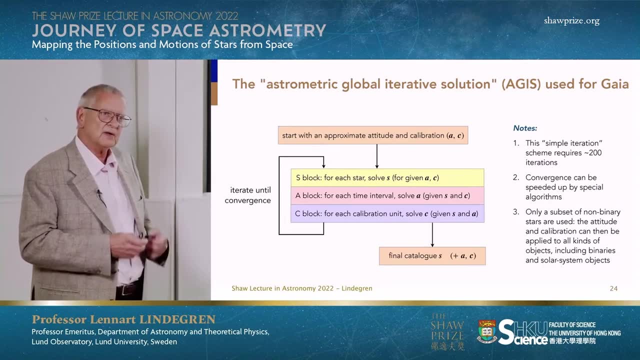 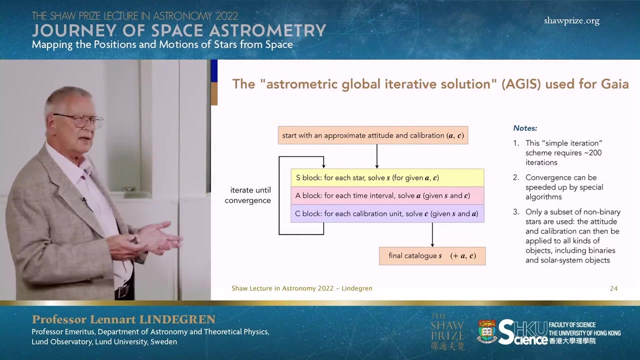 The idea is actually very simple and was around already at the time of the Hipparchos, although it was not used at that time. We already, from the beginning, have a good idea about what the attitude and the calibration parameters are, so we can use these initial estimates. 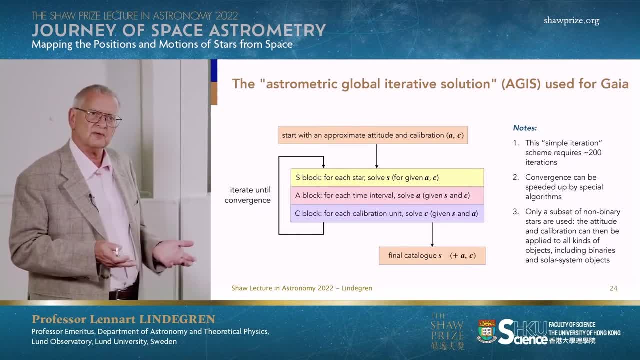 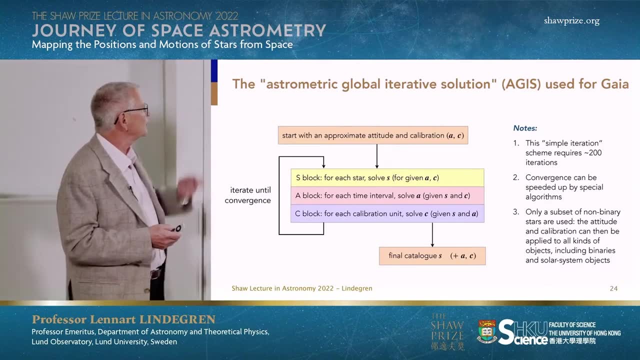 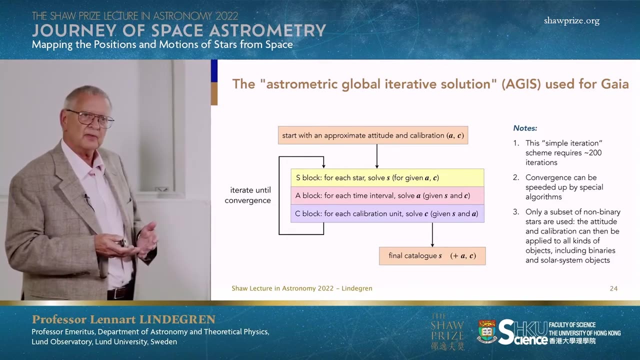 to compute the star parameters for all the stars observed. That is the S block in the three middle block here in yellow. Once we have the star parameters we can use them together with the initial calibration parameters to solve the attitude parameters. that is the pointing of the satellite. 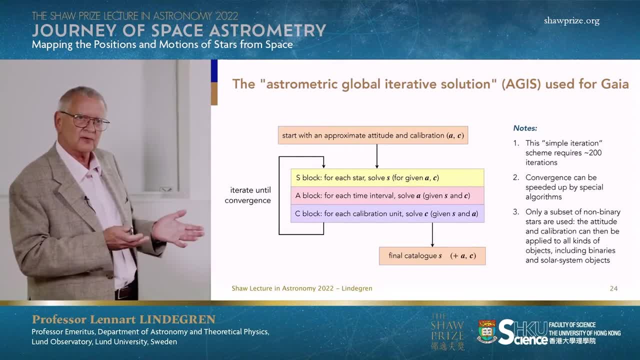 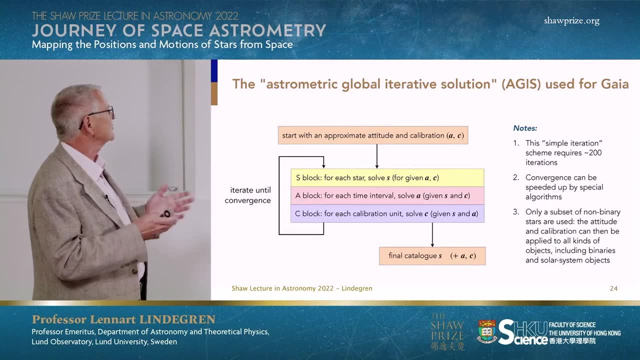 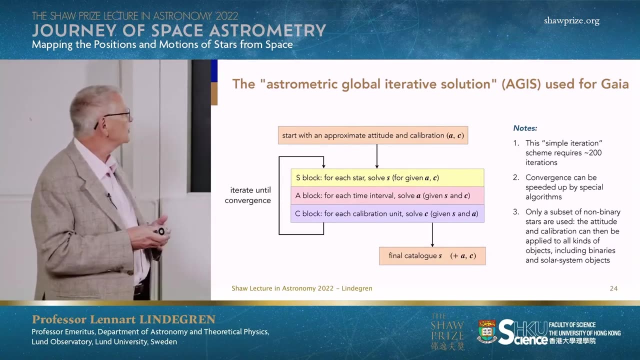 as a function of time. This will not be exact either, of course, because we have an approximate calibration and approximate stellar parameters, but it will be better than the original attitude that we started with And then in the C block we use the star parameters and this improved attitude. 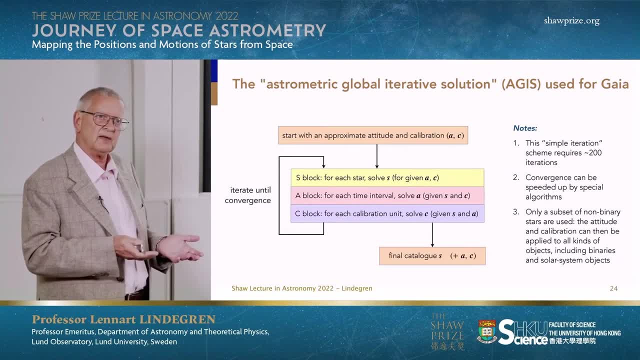 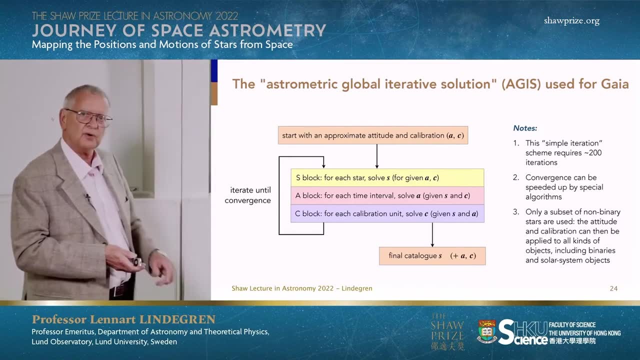 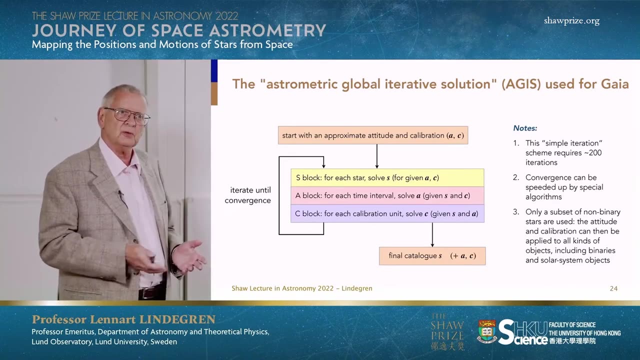 to solve the calibration parameters, And at this point we have improved both the attitude and the calibration and we can start again by doing the same loop once more. And each time we do the loop, all the parameters get a little bit better. It turns out that you need to do. 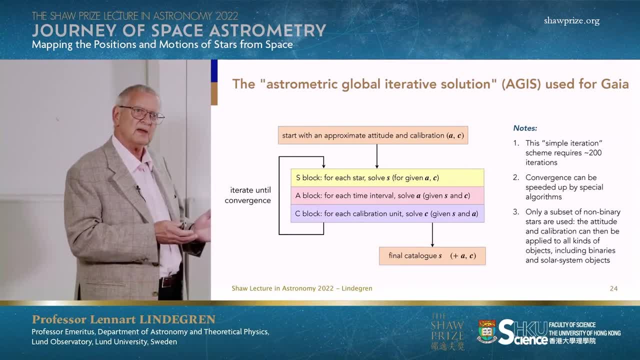 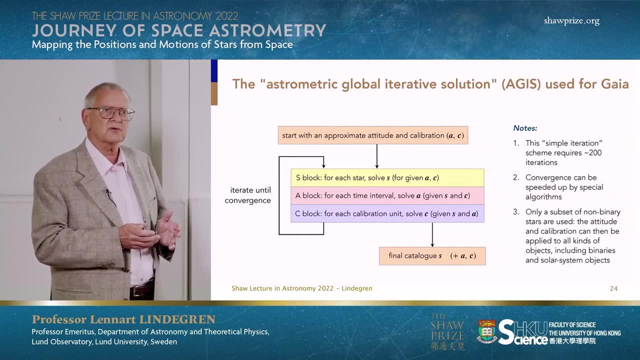 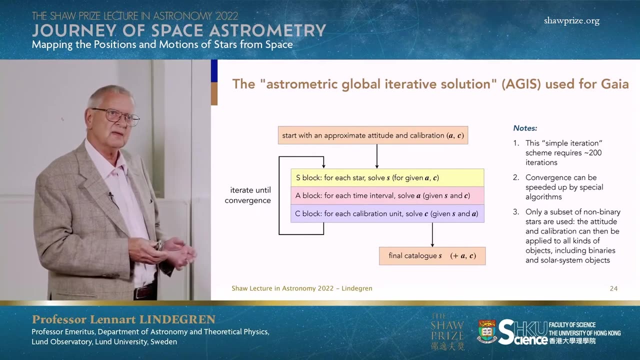 some 200 loops like this, but in the end the parameters don't change anymore and it turns out that you actually have the same solution then as from a direct solution of all the equations, But you get it for only a small fraction of the CPU time. 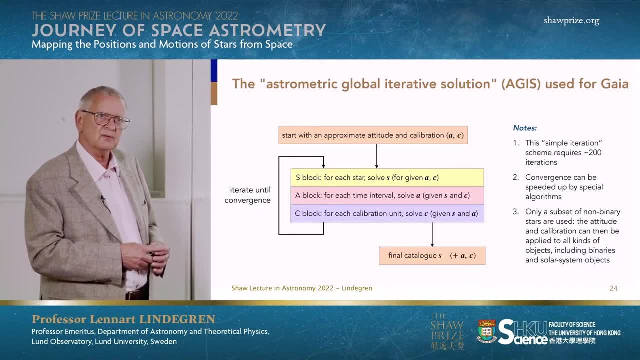 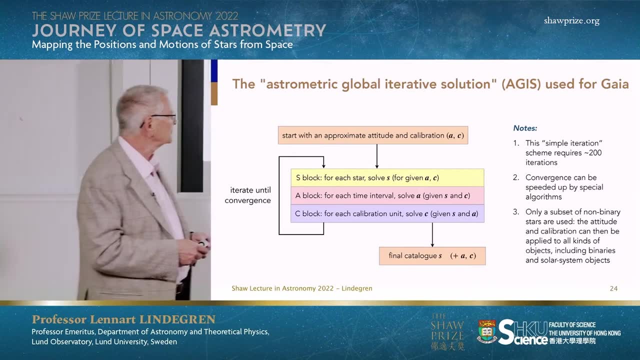 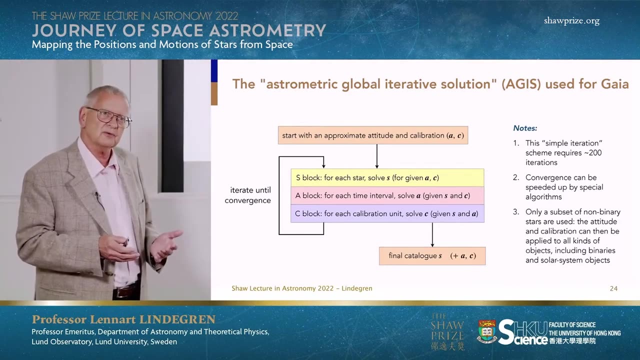 and memory requirements that would be required for a direct solution. So this gives you, in the end, the final catalogue And also, of course, the attitude and calibration parameters. There are several ways to simplify these shortcuts. For example, there are ways to speed up the. 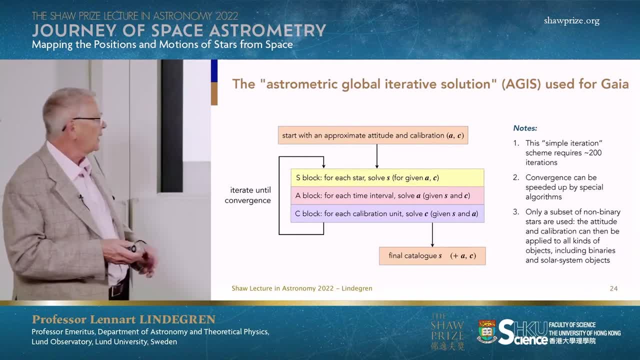 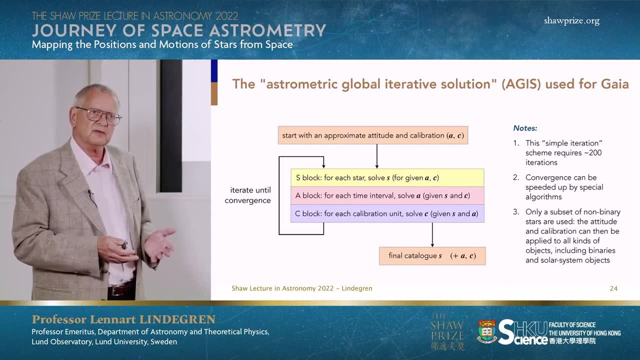 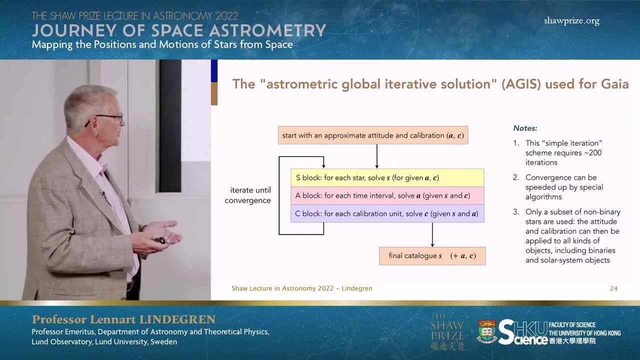 convergence of these iteration loops, and it is not necessary to do it for all the stars at once. You only need to do it for a subset of well observed and well behaved stars And, once you have done, got good estimates of the attitude and calibration using. 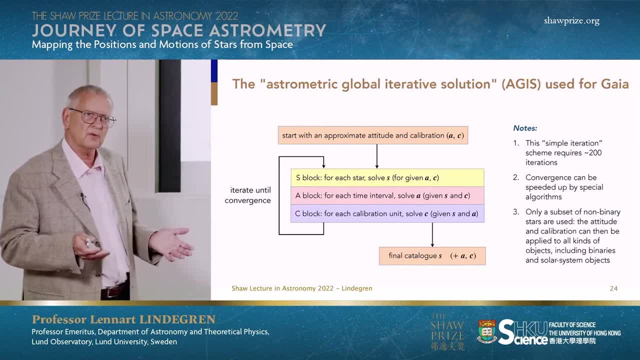 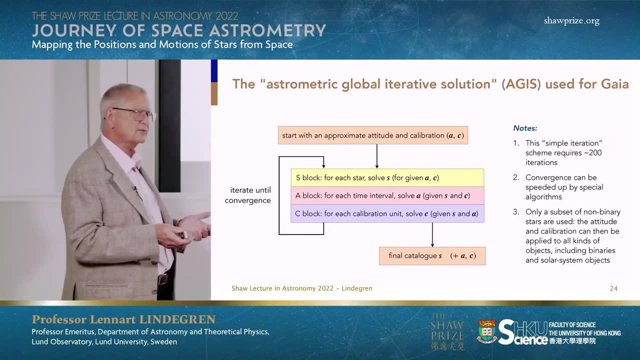 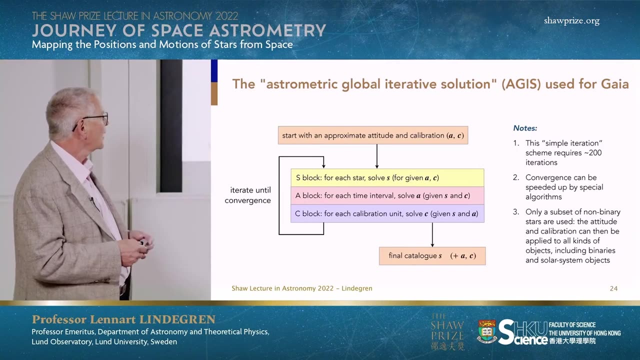 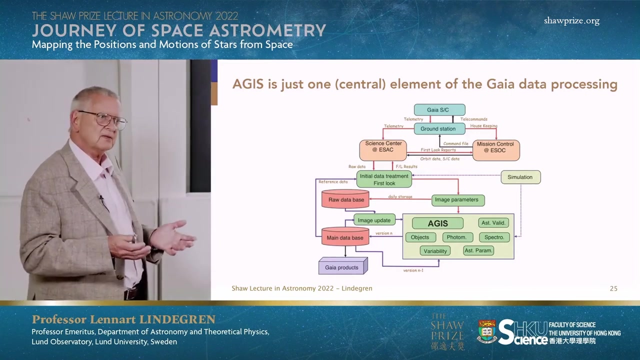 these stars. you can apply this attitude and calibration to all the observations and get stellar parameters for all the stars, but also other kinds of data, For example the positions of solar system bodies and galaxies and so on. In this talk I have completely talked only about the astrometric data. 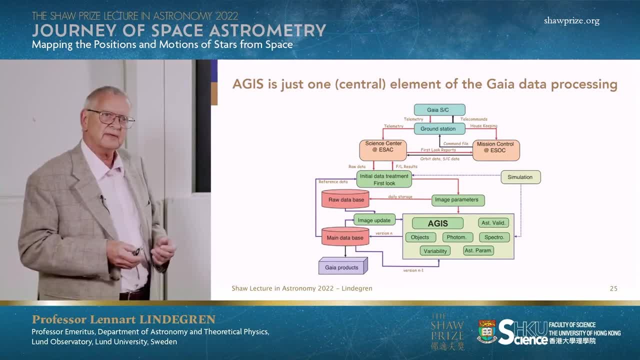 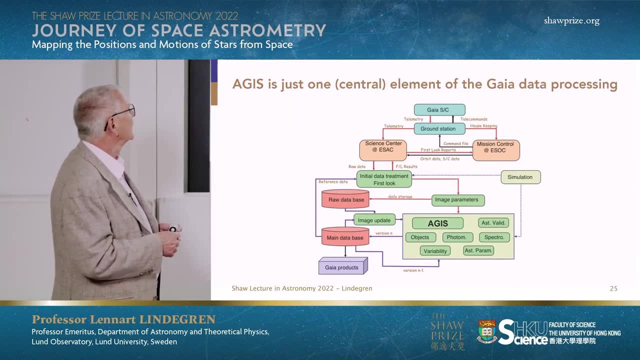 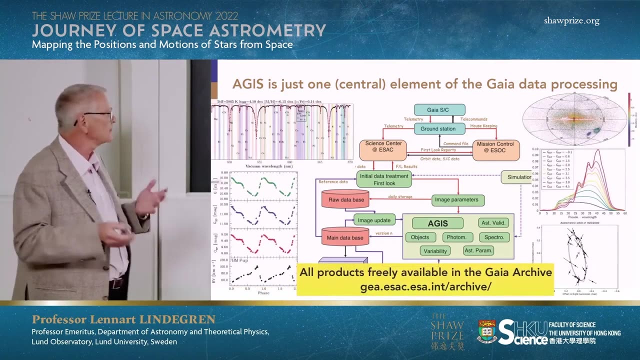 and the astrometric solution. But we should realize that that is only one element in a very big and very complex data processing task for Gaia. There are hundreds of scientists working on producing all other sorts of data: Photometric spectrometry for binary. 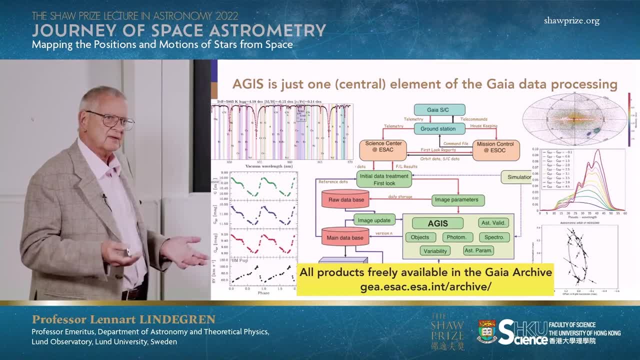 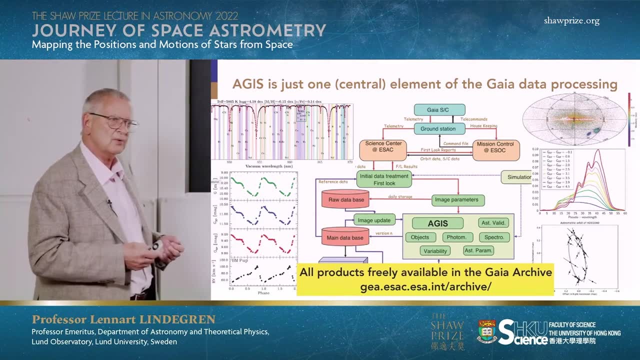 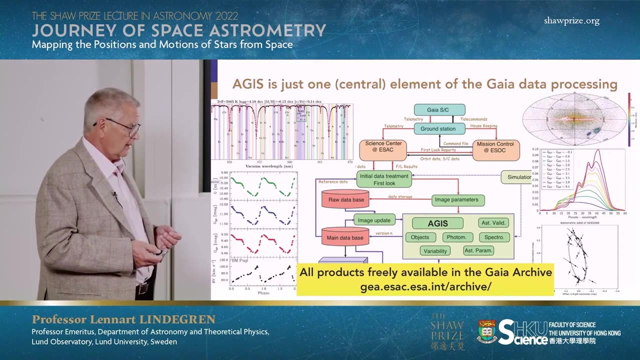 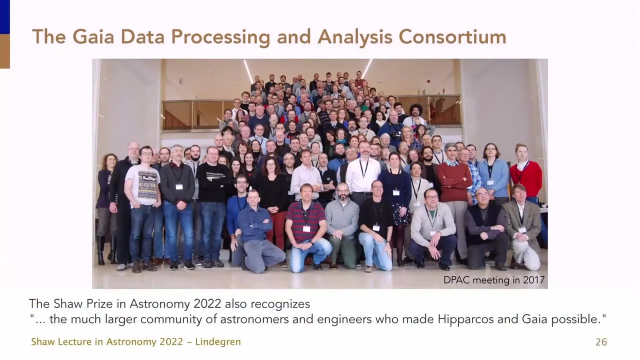 stars, galaxies, quasars and so on, And all of these products are freely available in the Gaia archive for everybody to use. I will end this talk with this picture, this photograph of members of the Gaia data processing and analysis consortium. 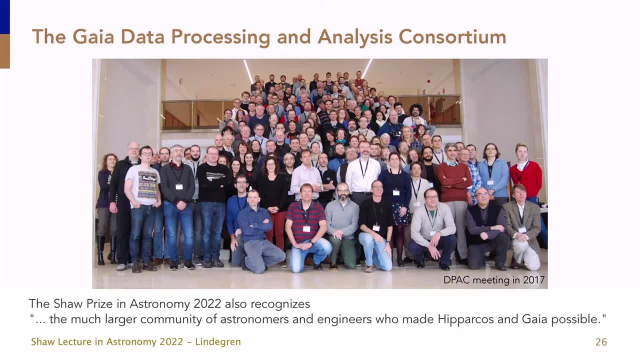 It is only a small fraction of all the people who have contributed to Gaia over the years, And many of the people contributing to Hipparchos are not here in this consortium. The Shaw Prize in Astronomy 2022 also recognizes the much larger community of astronomers. 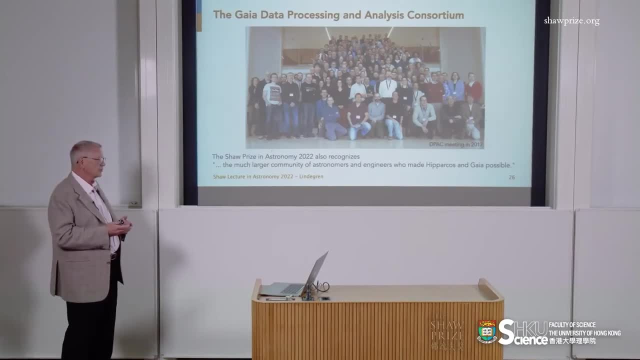 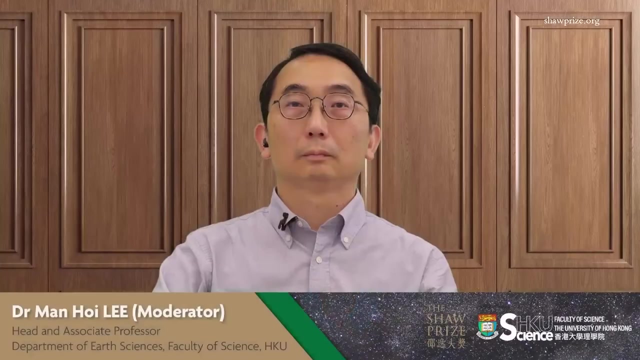 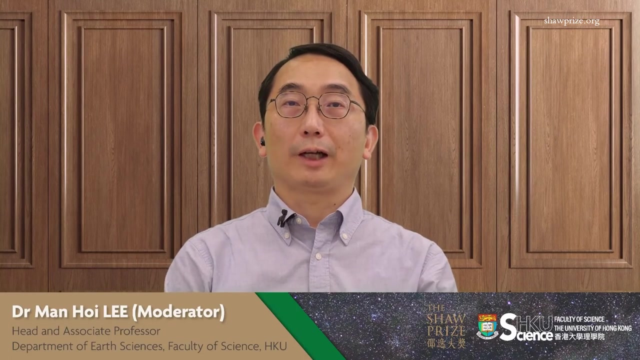 and engineers who made Hipparchos and Gaia possible, And I will let this image represent all of them. To them I say, and to the Shaw Prize Foundation I say, thank you. Thank you for your attention. Thank you, Professor Lindgren, for the lecture. 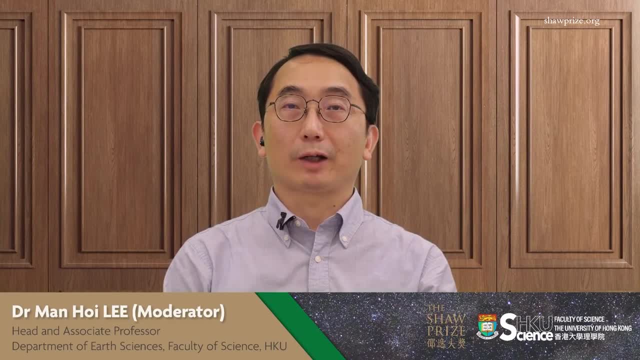 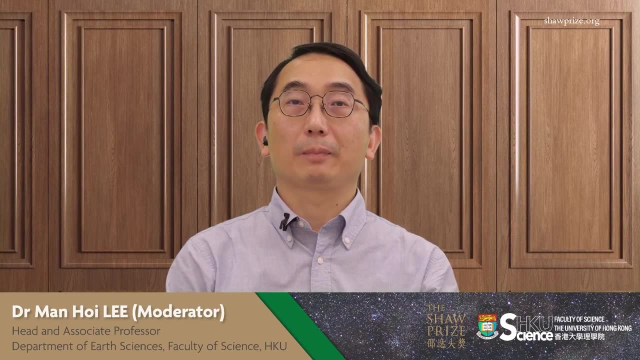 I am sure that all the audience benefited a lot from both lectures. For the audience: if you have any questions that you wish to ask our Shaw laureates, please take this opportunity to ask them now. Just feel free to unmute yourself or type in your questions in the chat. 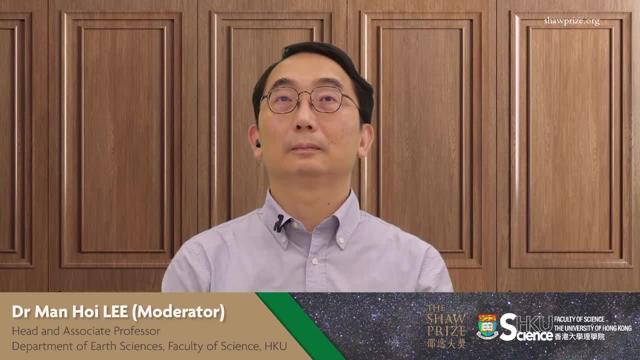 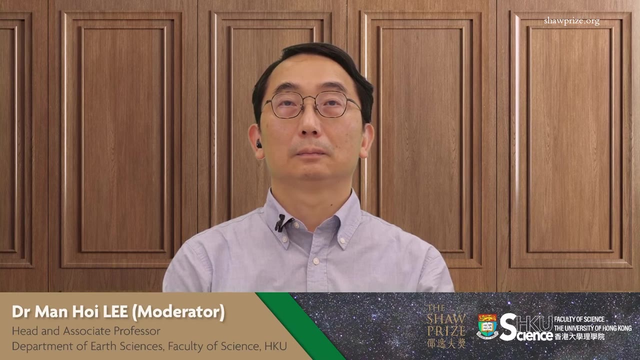 room here. So this is Mark Cropper. Can you hear me? Yes, we can. I wonder if Michael and Leonard can explain why the basic angle is not 90 degrees and why it was chosen to be the 106 degrees point five in Gaia. 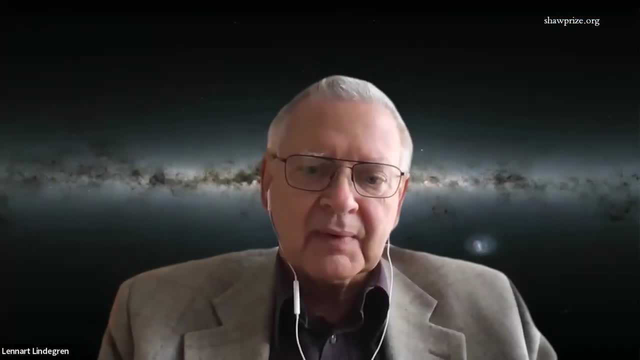 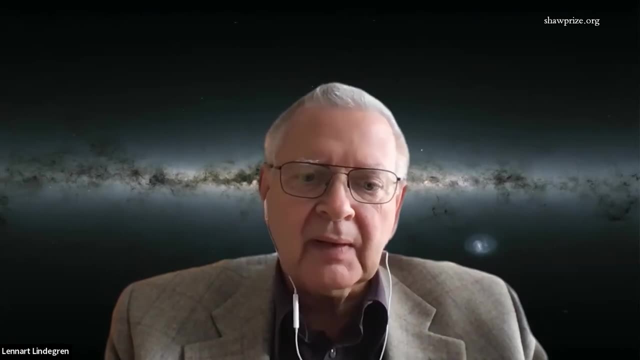 Yes, that's a good question. actually, It could have been quite a different angle. In fact, almost any angle, from about 30 degrees to 150 degrees, would have worked equally well for solving the global astrometric problem. But when you do this, 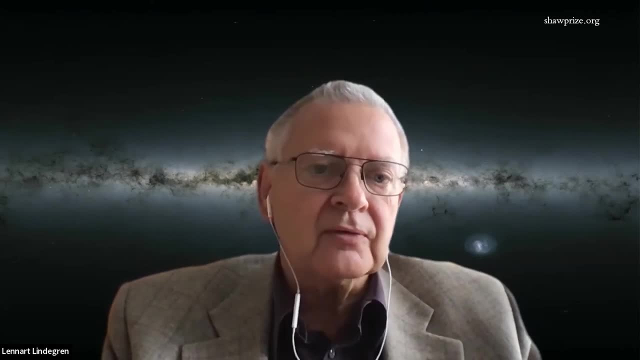 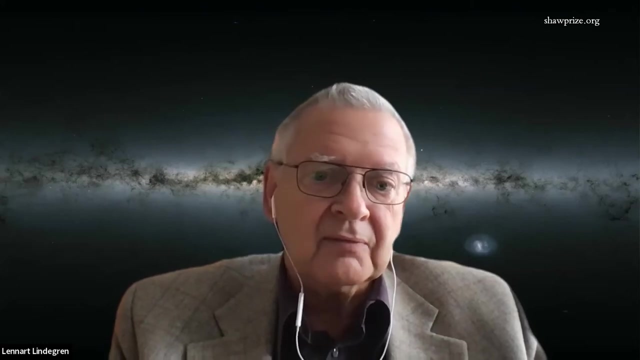 solution on a great circle to calibrate the basic angle and scale and so on. there are certain values that you should avoid and they are simple fractions of 360 degrees, Like 90 degrees is not a good angle, 72 degrees, which is one fifth. 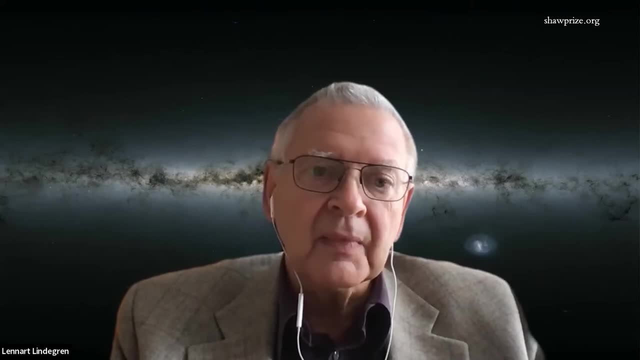 of a full circle is not a good angle, and so on, And this value, 106.5, is one of the values that just avoids these simple fractions. There was a whole range of possible values and the final choice, I believe, was up to the engineers. 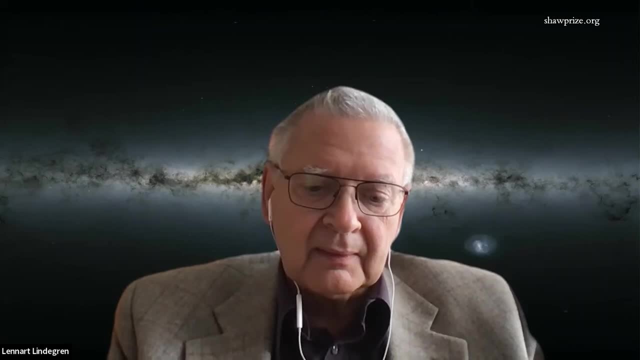 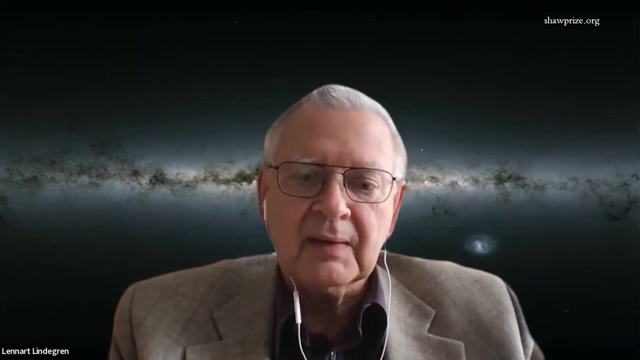 at that were going to design this instrument, They had to take into consideration that it could easily be accommodated and baffles and so on. So there were many constraints to be taken into account. Thank you, Leonard. So someone asked: can you? 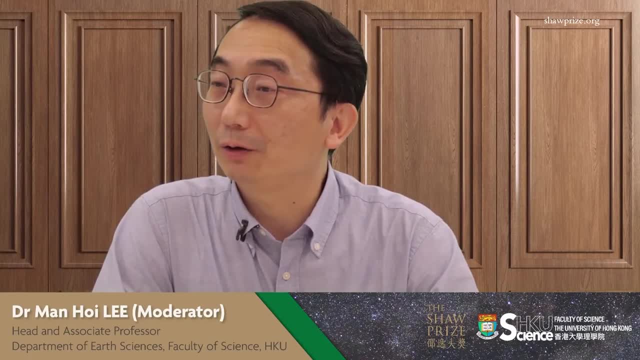 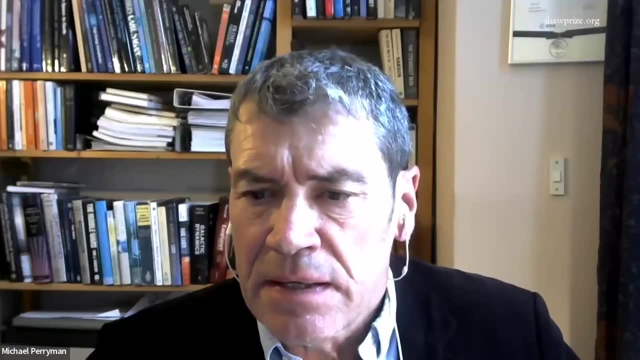 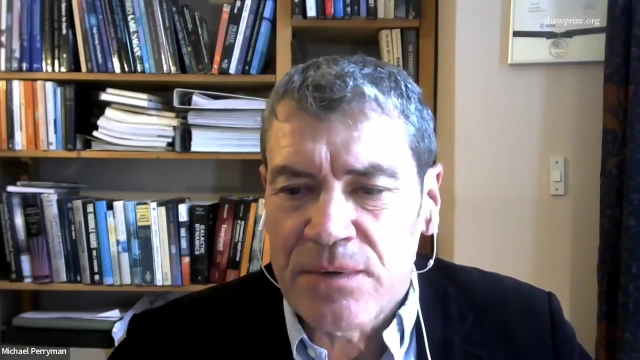 explain more about why we need to measure the star in two directions in the sky at the same time. Maybe shall I take that Go ahead Your question, Mr Fung. What we'd like to know is how each star is moving through. 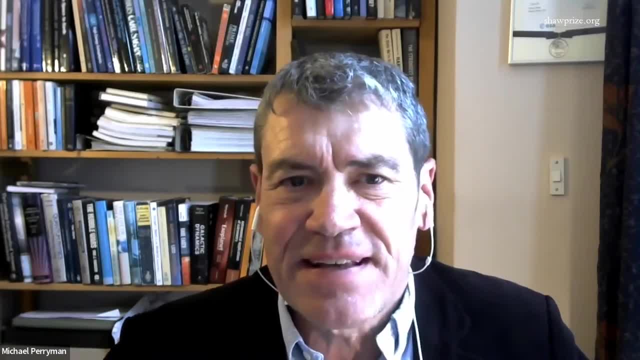 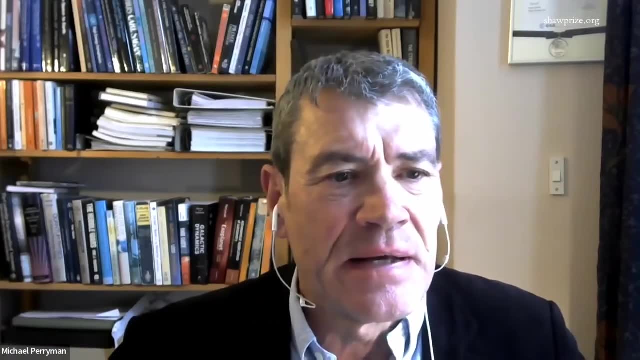 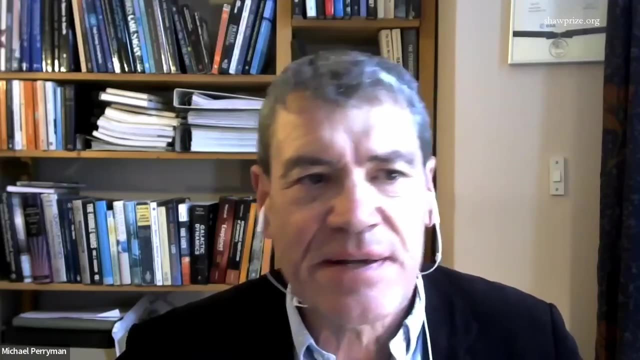 space. Forget any concept of coordinate directions. We'd like to know how the star is moving through space, And any motion through space can be described by three quantities in Cartesian coordinates: x, y, z coordinates. You want the x, y and z values. 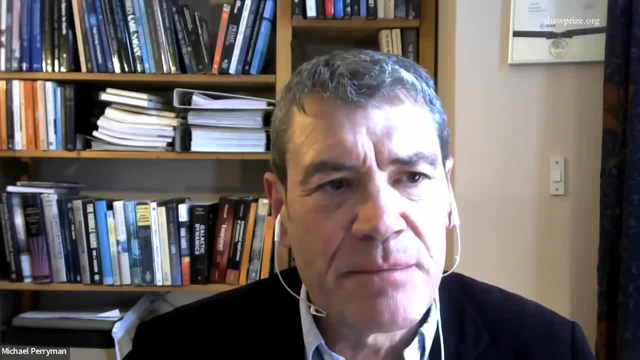 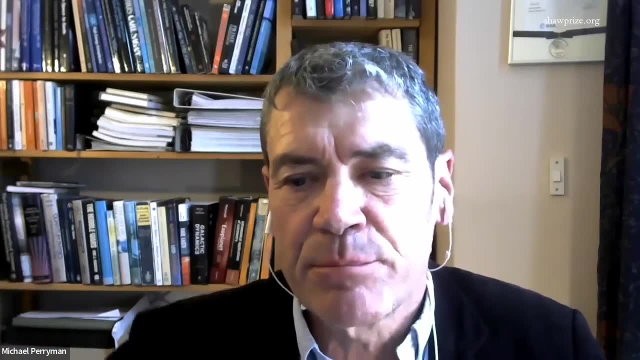 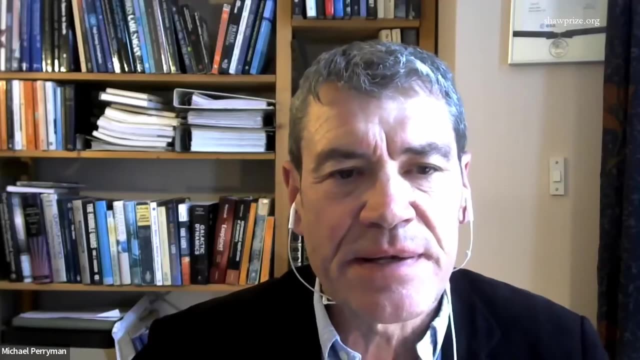 What we can only measure with a mission like Hipparcos and Gaia from the astrometry is how the stars move on the plane of the sky, projected on the plane of the sky. So we measure that using these astrometric measurements and you can think of that in two coordinates. 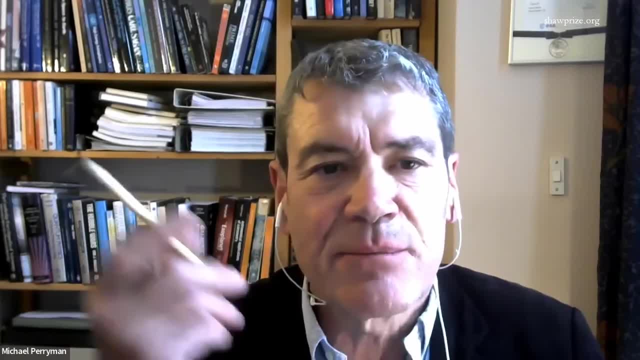 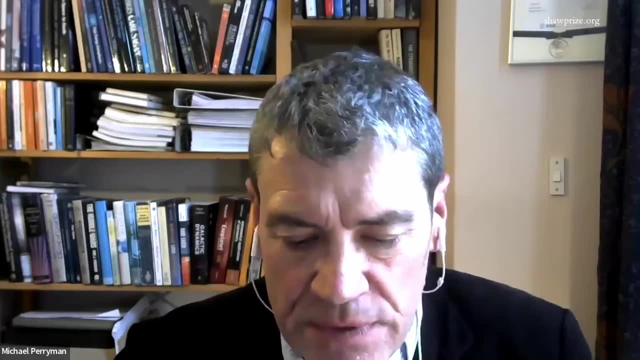 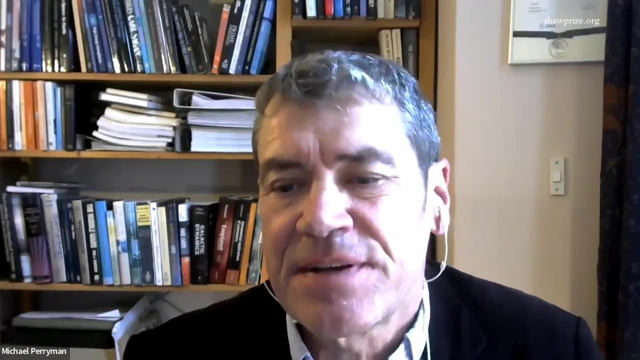 I think it's simply stated like that. Ideally, we'd like to measure the radial motion of the star as well, And there is a separate instrument on board Gaia called the radial velocity spectrometer, which measures the radial velocity of a subset of the stars. 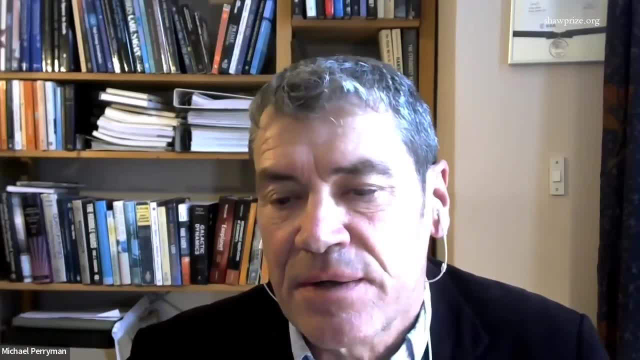 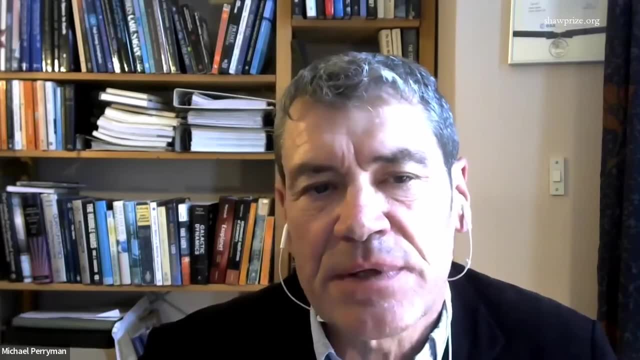 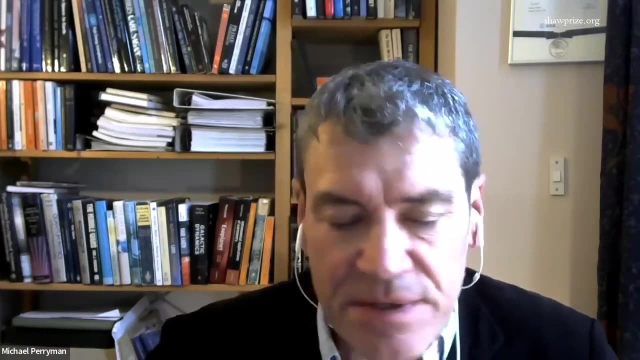 the brightest stars in the radial direction. So when you combine these astrometric measurements made in two directions on the sky, with Gaia, with radial velocity, you get the full space motion If you don't have these radial velocities available, so we don't. 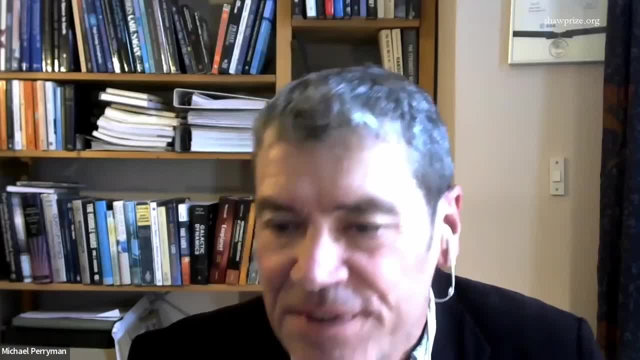 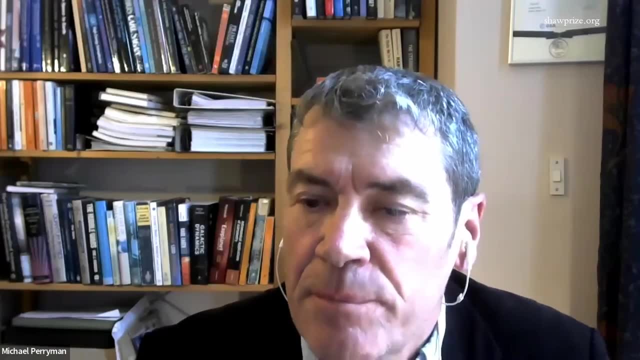 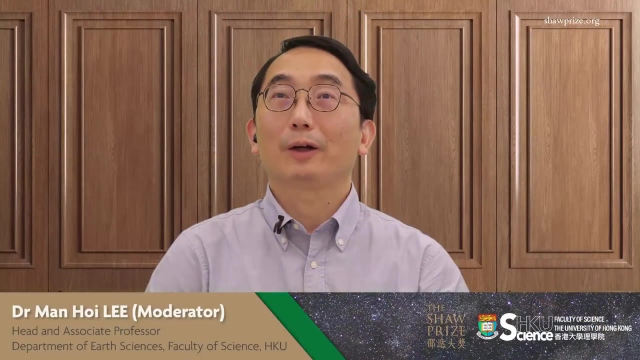 have those for the fainter stars. there's not enough photons, the stars are not bright enough to measure this. then you just have a projection of the stellar motion on the plane of the sky. Okay, thank you. So we have another question in the chat. 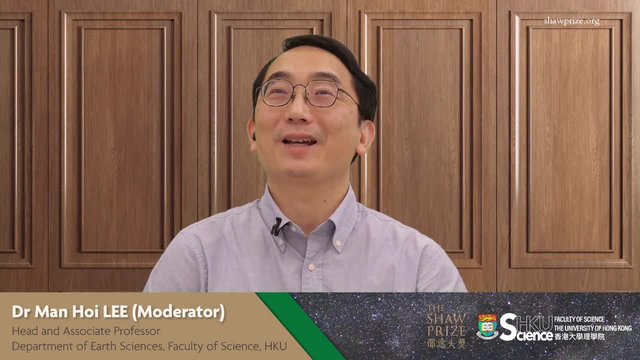 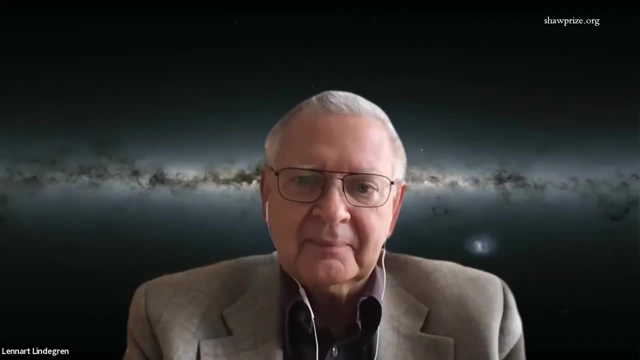 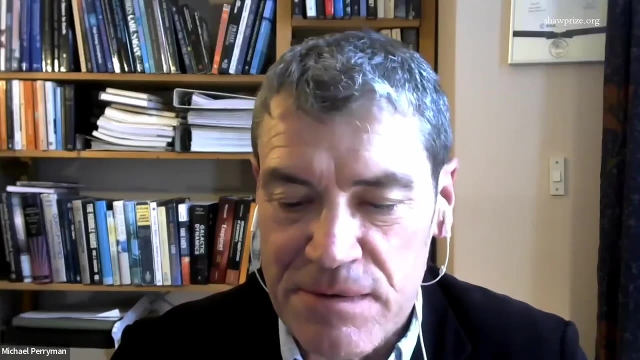 room. Someone's daughter was asking why it's called Gaia. Do you want to take that, Michael? Yes, when you come up with any experiment, you have to come up with a good name that will attract attention to the funding authorities. 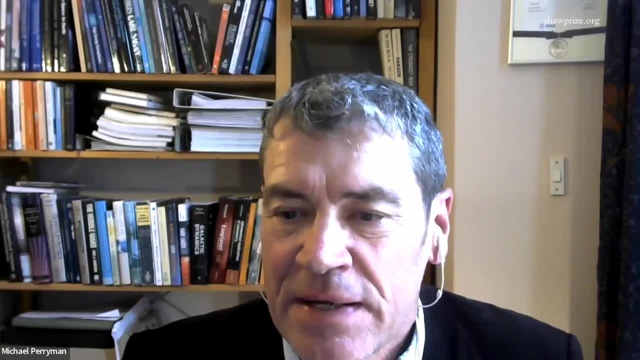 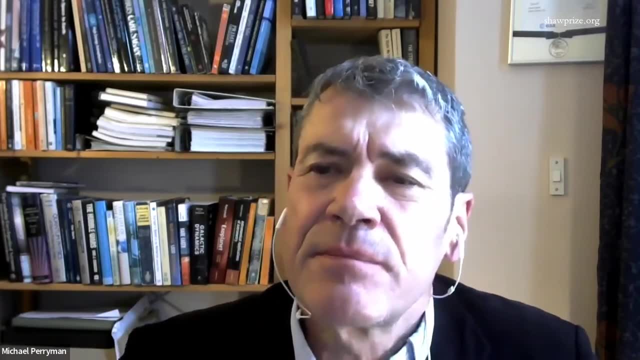 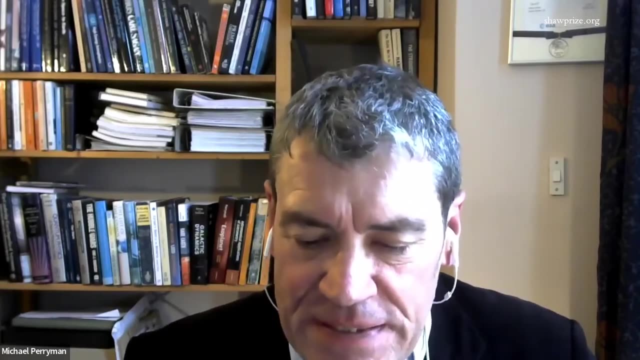 That's part of the answer. We liked the name. So you come up with a name and then you think about an acronym, And in the early days we thought that one of the early ideas was to make these measurements using a technique called interferometry. 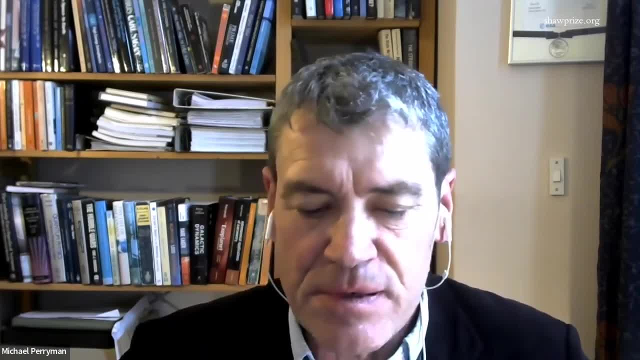 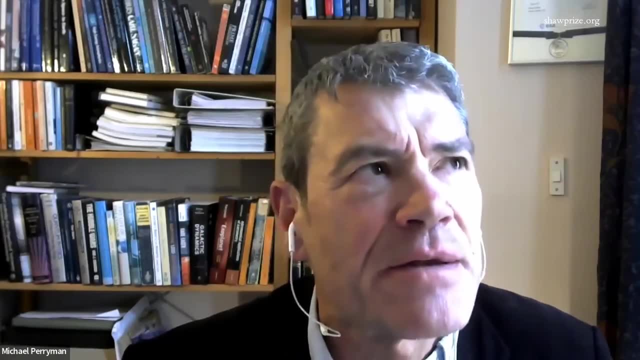 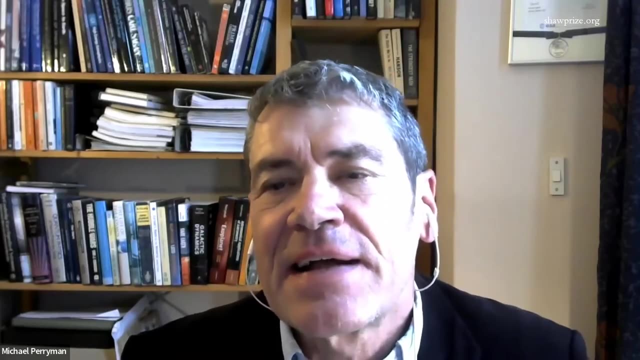 And we dreamt up this name, this description: global astrometry, global astrometric interferometer for astrometry, Global astrometric interferometer For astronomy, And abbreviated Gaia As the design of the satellite developed the interferometric. 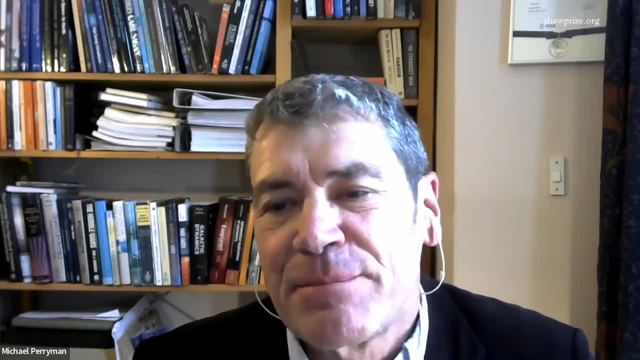 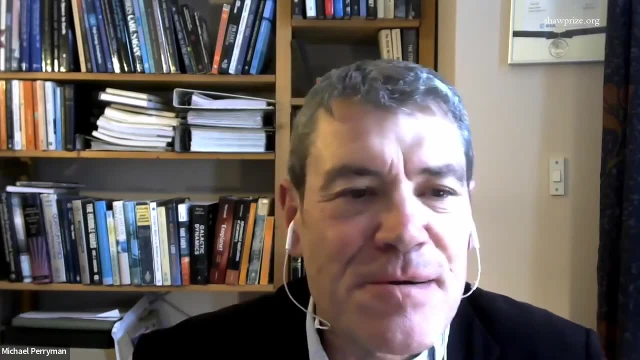 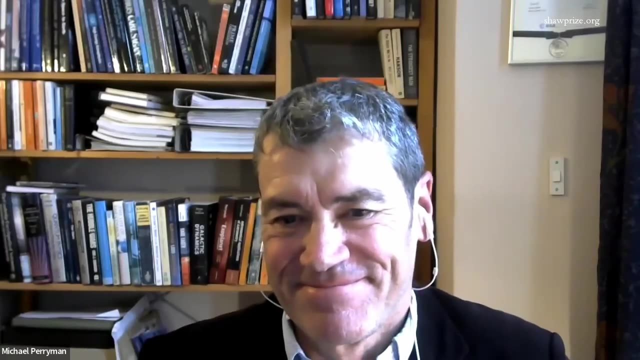 principles was dropped, but we kept the name and we just called it Gaia. So it's a nice name. It's some kind of tenuous relationship to the goddess of the Earth. It's just a nice name. Okay, We can take more questions. 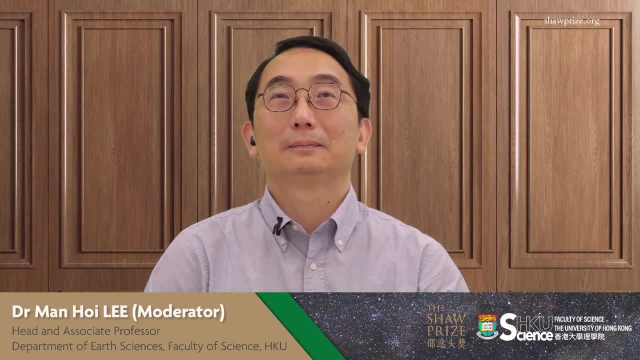 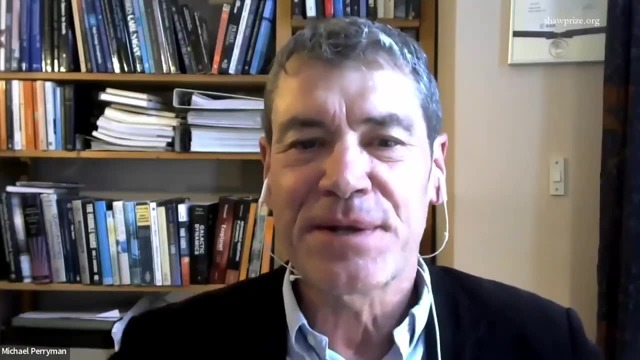 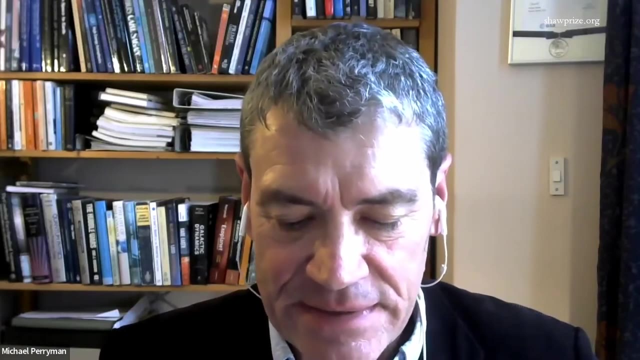 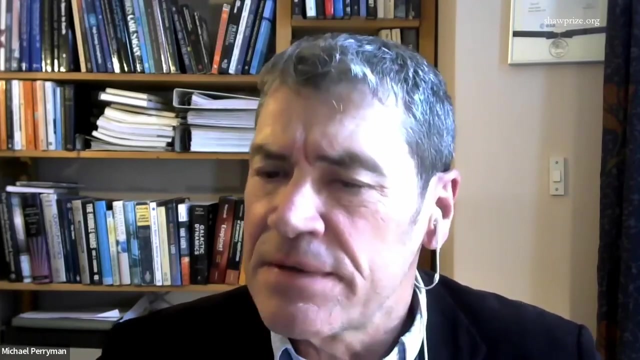 What's next after Gaia? That's a problem for young people. The world is open to the new generation of astronomers to think of how to do it better, and what we know from our studies with Gaia is that you can make these measurements far more accurately than we could. 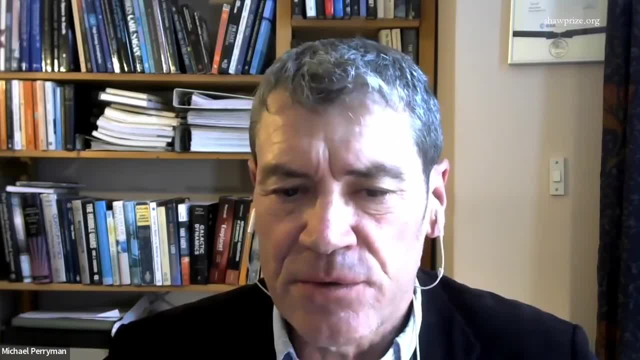 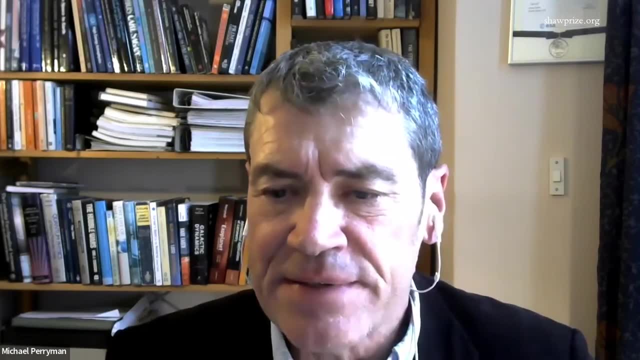 even with Gaia. In principle one can go to much, much better accuracies. There are studies being carried out. I mean, maybe Lennart would like to say a little bit more on that. There are some ideas being pursued in Europe and elsewhere. 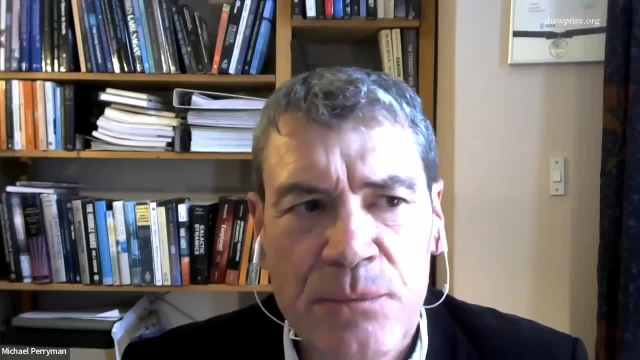 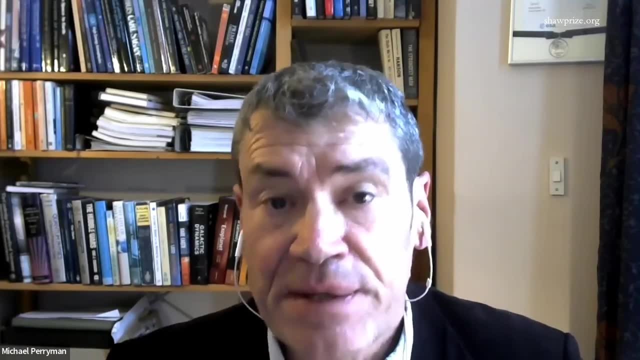 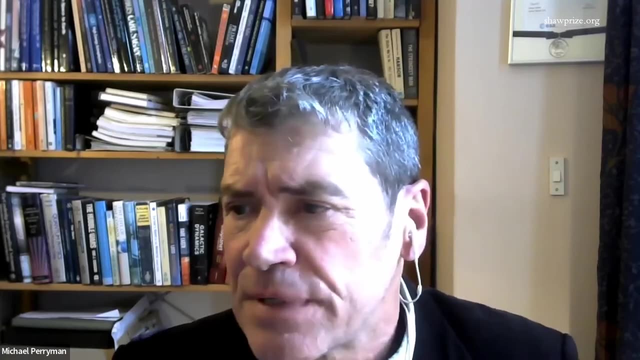 for the next generation. But I think what we, what has been demonstrated with Hipparchos and Gaia, is that this is a very, very clever, robust way of making these measurements. The scientific information available to us about the way our galaxy is formed and the way 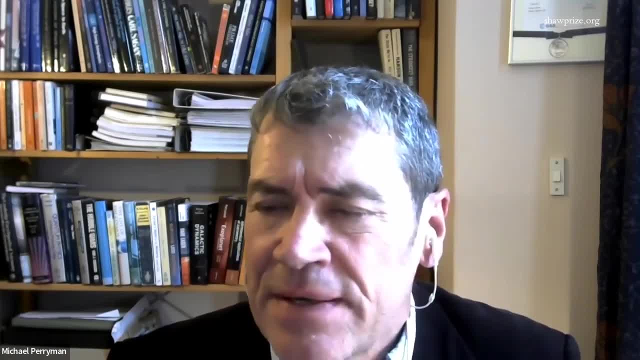 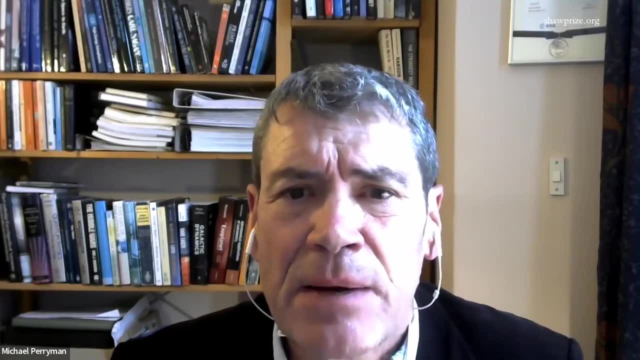 our universe is structured would benefit from even more stars and even more accuracy, And I think that's a possibility and it's a challenge for the next generation to come up with the best way of doing that. Lennart, maybe you could add a few words about what's. 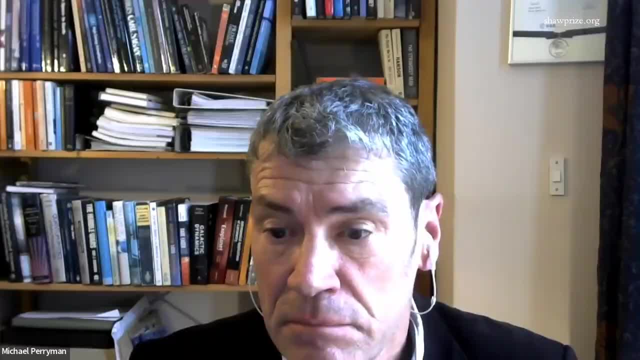 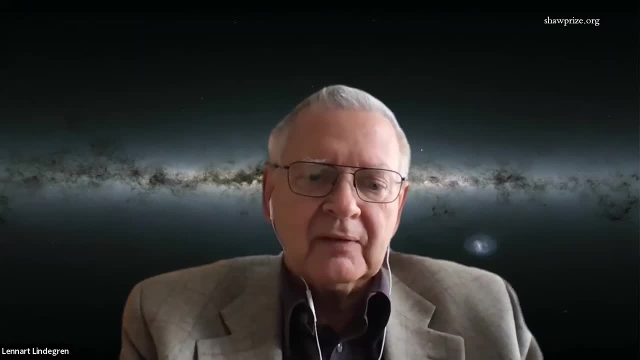 being done already. Yeah, it's not completely obvious how you should go forward here. There has been a discussion about various directions. For example, you could go towards a pointed mission, that by being pointed, you can have much longer integration time on each object, which means 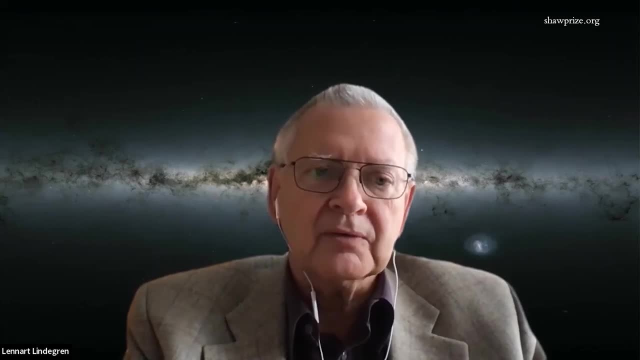 that you can do it more accurately and also reach much fainter objects, And that would perhaps open the possibility to detect Earth-sized planets around stars using astrometry. Another possibility is that you can extend the wavelength range. Gaia is essentially sensitive to visible. 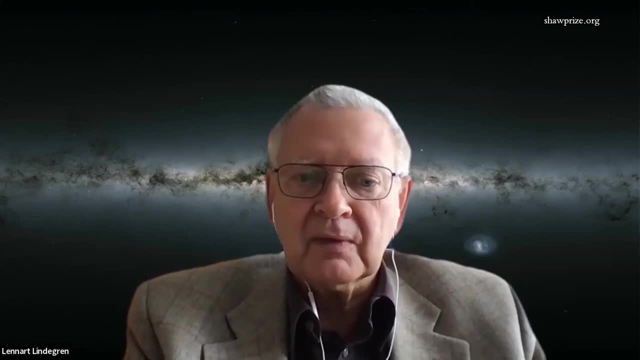 light, but we know that a large part of our galaxy is hidden behind dust clouds, and it would indeed be interesting to be able to penetrate these clouds a little bit better, which you can do if you go to slightly longer wavelengths into the near infrared. So that is also. 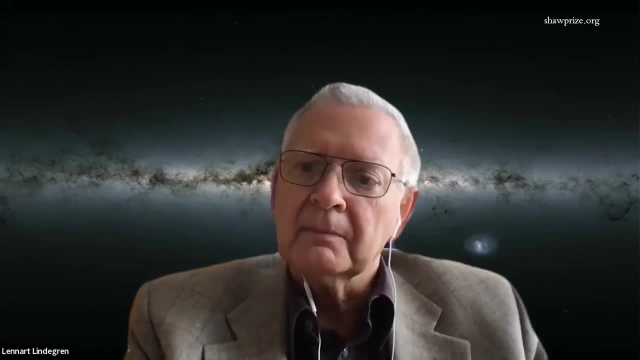 a possibility And there has been proposals for such missions, including the Japanese Jasmine mission and the European mission, which is currently called Gaia Near Infrared. As Michael said, we have to come up with a better name that captures the imagination of those. 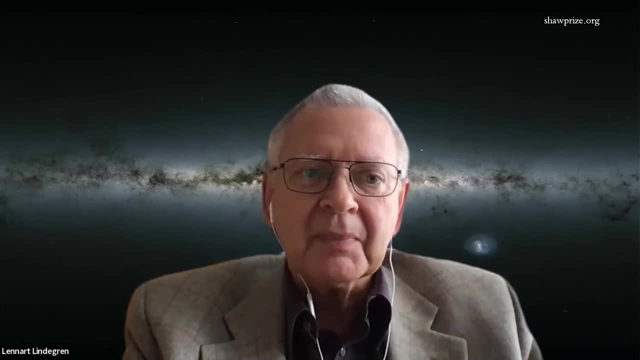 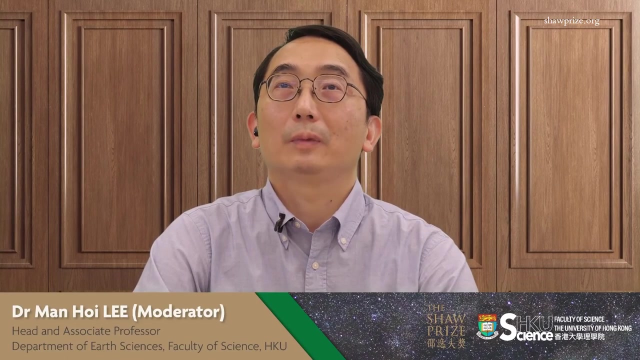 who are going to give us money for it. But these are some of the possible directions we could go with future missions. Okay, thank you. We also have a question on the chat room asking. it says that you both mentioned the measurements of very distant objects, including quasars. 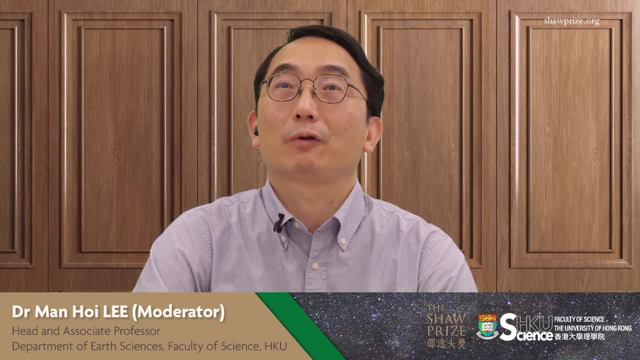 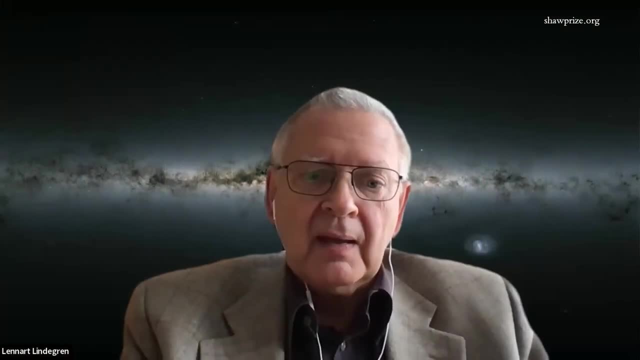 Can you explain the importance of using these measurements for the identification of the proper reference frame? Perhaps I can answer that also. Well, the concept of a reference frame is that you should define coordinate axes in space that are non-rotating, because it is only in such non-rotating coordinate systems that the laws of mechanics, like Newton's laws or Einstein's laws, apply. As soon as you have a rotating coordinate system, you get strange effects like centrifugal or Coriolis forces and so on. You don't want that. 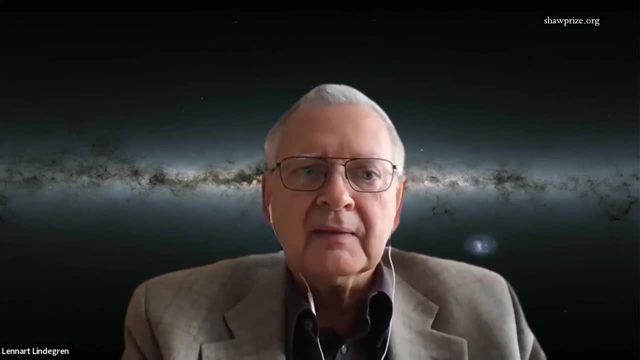 simply, You want a non-rotating system, And the simplest way to get a non-rotating system is to look for sources that are sufficiently far away that, even if they have large motions in space- thousands of kilometers per second- it really doesn't. 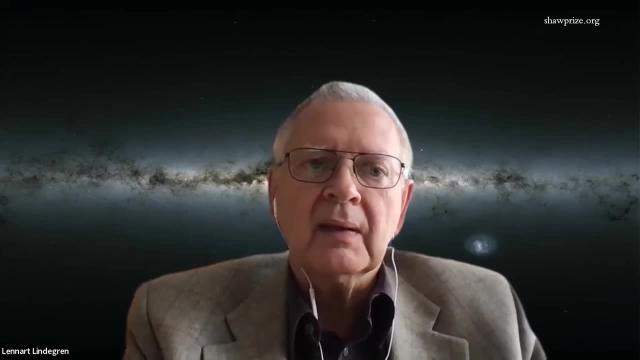 matter. They are so far away that they look to be stationary on the sky, And the quasars are the best objects we have for that, because they are very far away at cosmological distances and they are also more or less point-like. 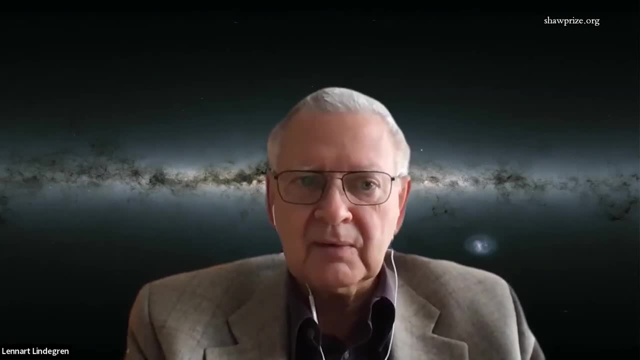 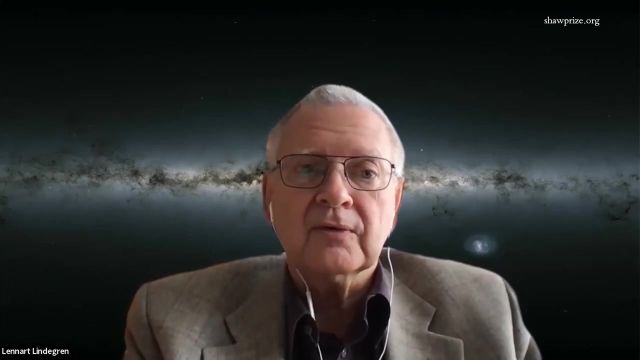 like stars. So if you can observe stars to good accuracy, you can also observe quasars to good accuracy. So with Gaia we observe a few million quasars and they are used to define exactly this non-rotating reference system. 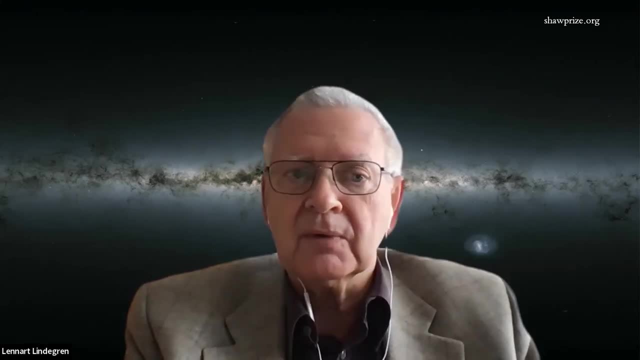 And that is then very important when you want to study the motions of stars in our galaxy, for example, or the motions in our solar system, asteroids, and so on. For all of that, you need a non-rotating coordinate system. May I take? there's several. 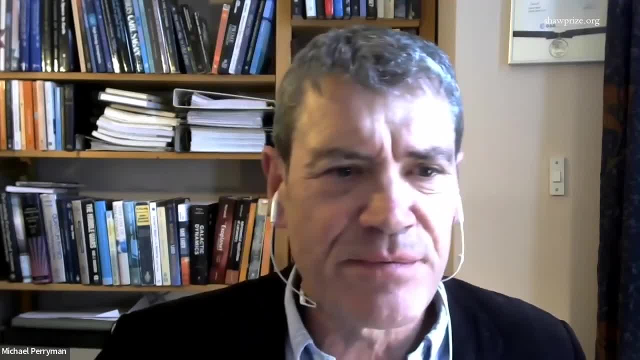 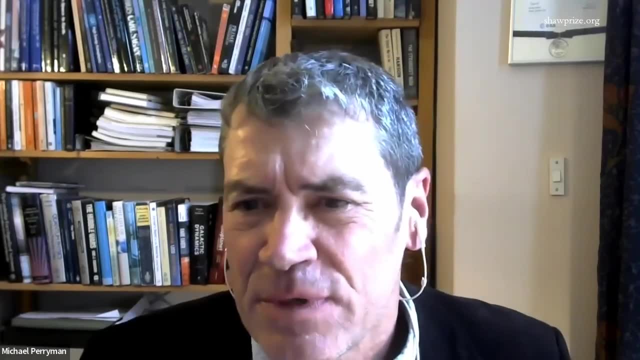 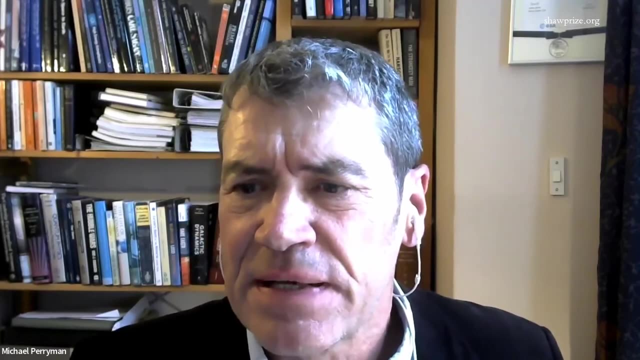 questions coming in and I must say how wonderful it is, when you give a presentation, to have interested questions, which I think reveal the complexity of these missions. Can I see if I can take those three questions together fairly quickly? The first, Pearl Mong, has asked. 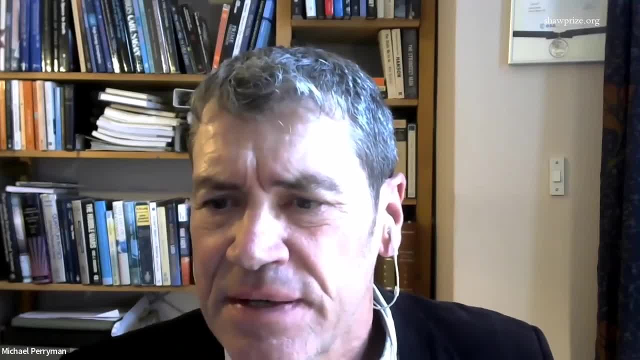 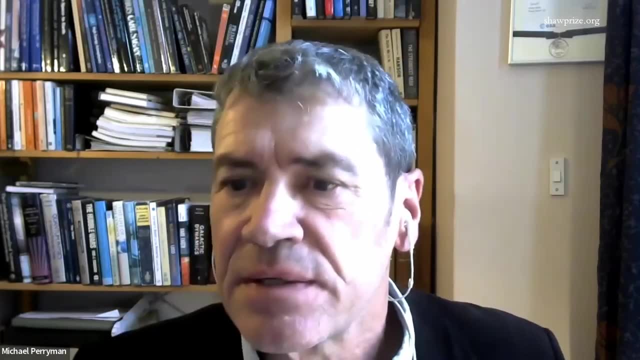 is it correct to say that the definition of target stars, background stars and so on varies according to the location that Gaia is launched and, if so, how is the location picked? No Pearl. it's not correct to say that The idea is: you can. 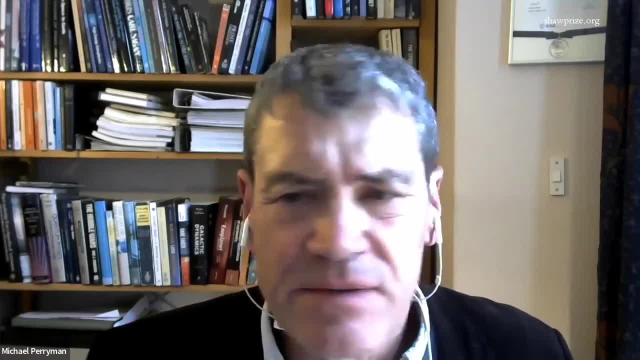 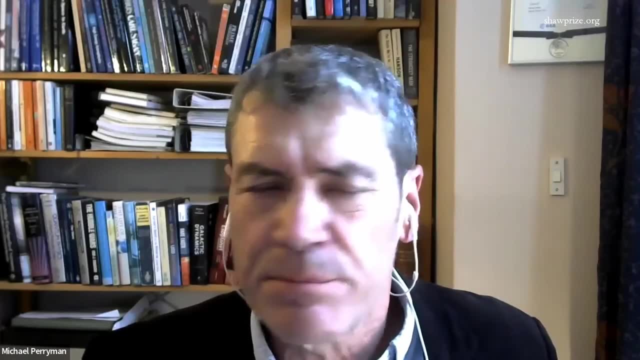 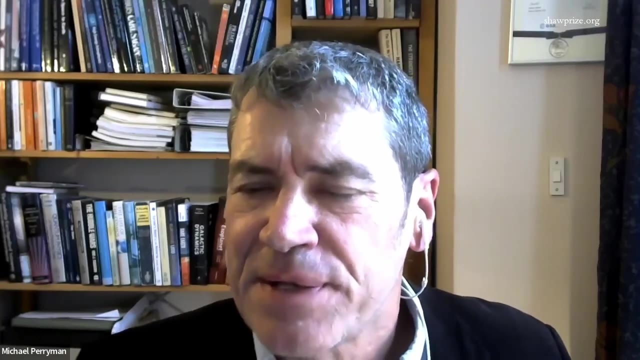 see, because the satellite is launched in the way that Professor Lindgren has described. you see the whole celestial sphere, you see all the stars, and the question of which- where to launch Gaia and where to place Gaia- was just dictated by how the best possible. physical location to place it and we wanted to get away as far away from the Earth as possible to avoid several problems with radiation from the Earth and so on, and Gaia has been placed in something called point orbit beyond the Moon and we see the whole. 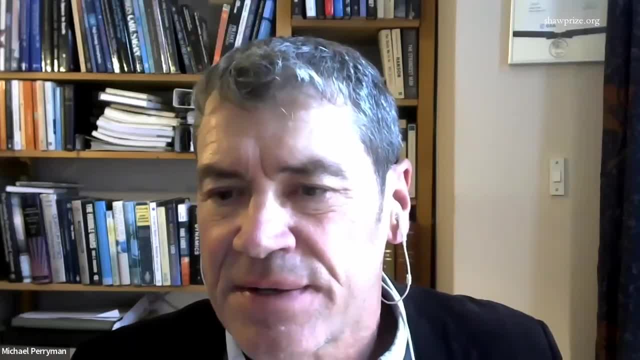 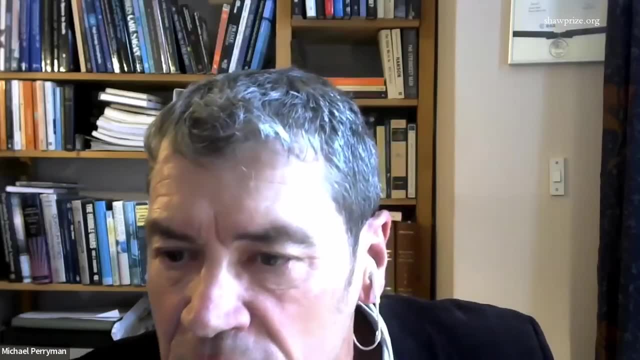 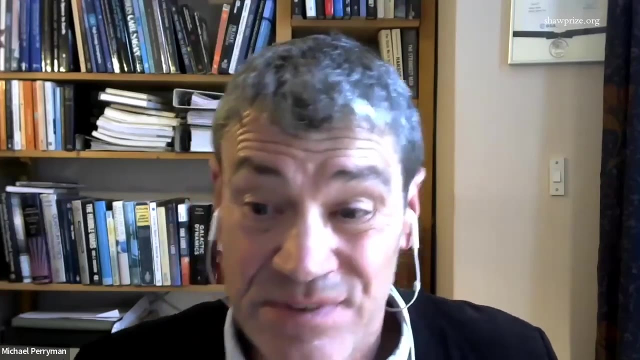 sky from there. so the idea of target stars, background stars, doesn't depend on where we place the satellite. So Leung Chung has come. I think, a very important question that we didn't touch on at all, which is what's the main difference. 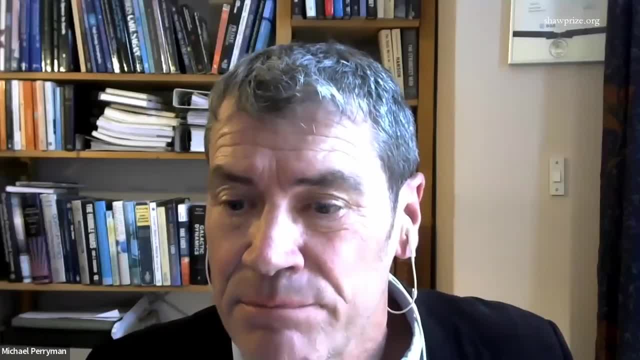 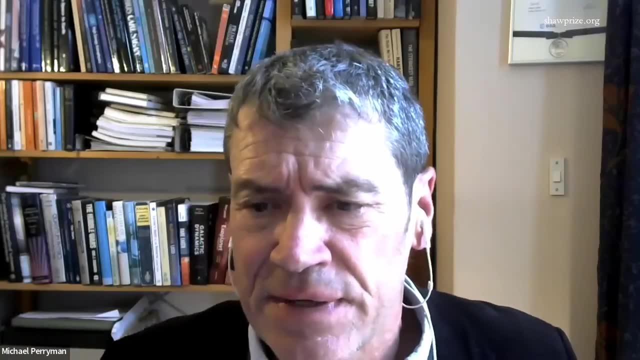 between different data releases of the different catalogues? Are they mainly the time difference, or new data analysis, or correcting mistakes? Well, it's a combination of all of those. in fact, The idea is that, as both of us have explained, 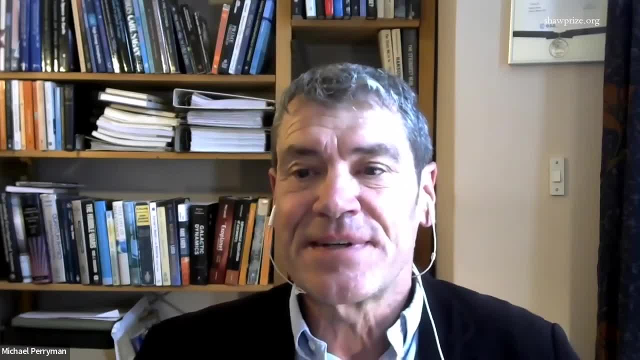 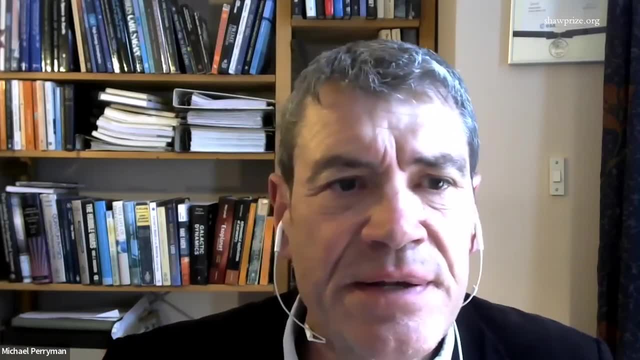 Gaia will be operating for about 10 years. We didn't want to wait until the. in fact, I should point out, there's several people tuned in. Anthony Brown is listening into the Zoom meeting. He's actually chairing the entire data analysis. 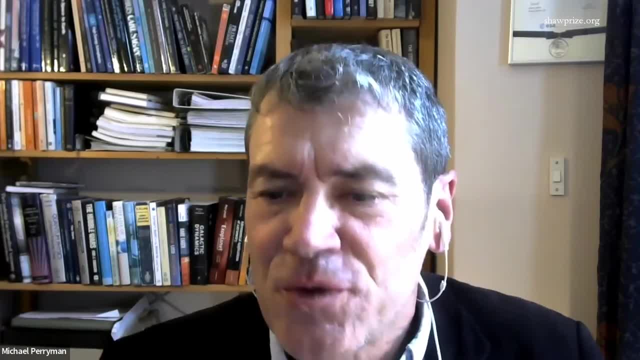 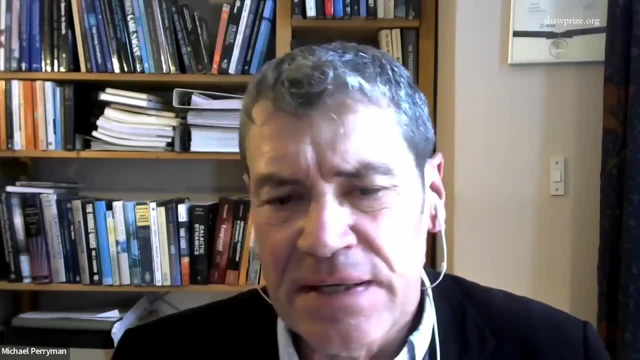 consortium at this moment. The idea is not to wait for the full 10 years until you have all the data and then give it to astronomers sometime in the 2030s. The idea was to take data in bunches, in packets, as it comes in, And the difference. 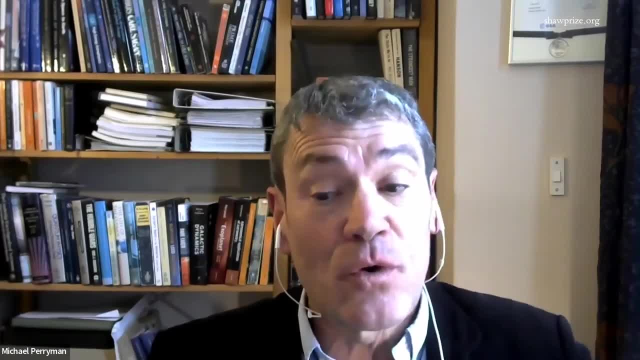 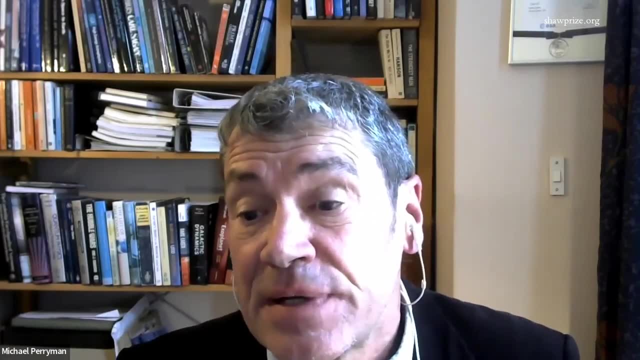 between the different data releases is just the addition of more and more data with time. So the current best data, current latest data release- DR3, data release 3, is just based on the first 33 months of data. Data release 4 will be based on something. 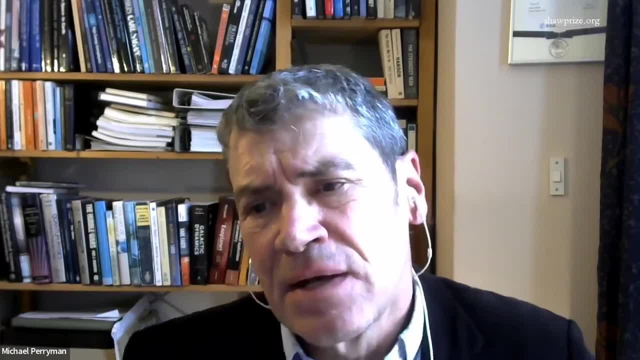 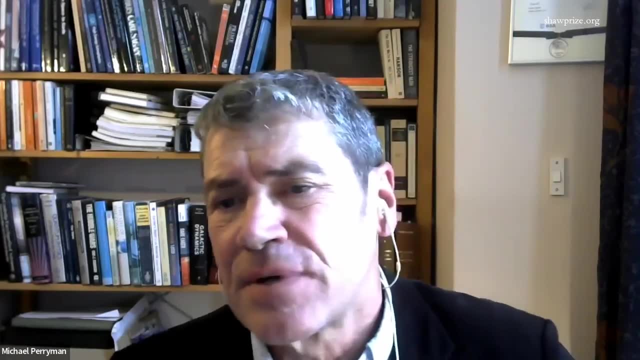 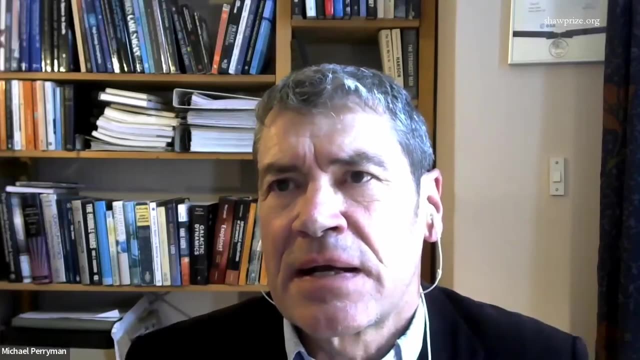 like 60 months, 5 years of data, And what happens is you're bringing in more data, completing more iterations and completing more interactions between, say, the photometric data and the astrometric data. So it's trying to come up with.